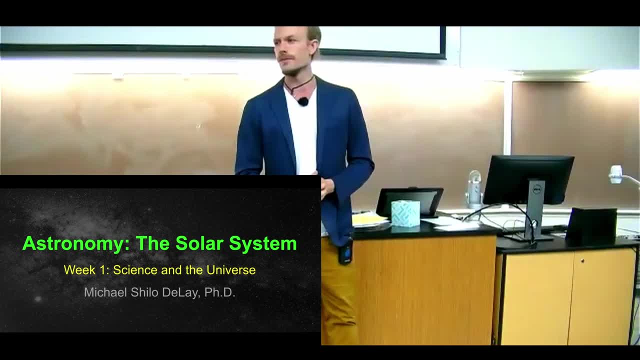 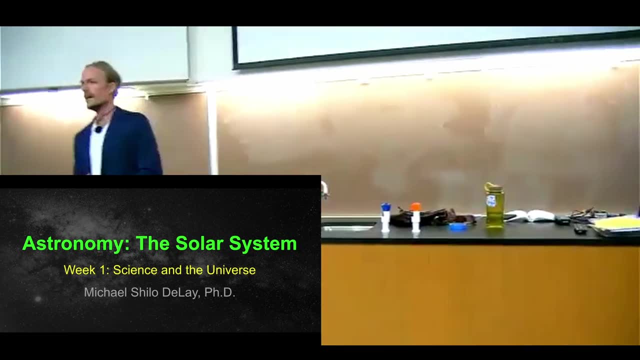 will almost certainly be superseded in the decades to come. Some of them are on the rocks right now, And that's really important. They are, however, the best way that we have of getting to know how the world works, And they've proved out that way, So we're going to talk. 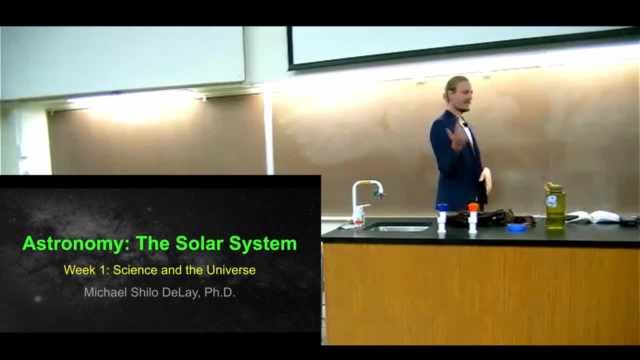 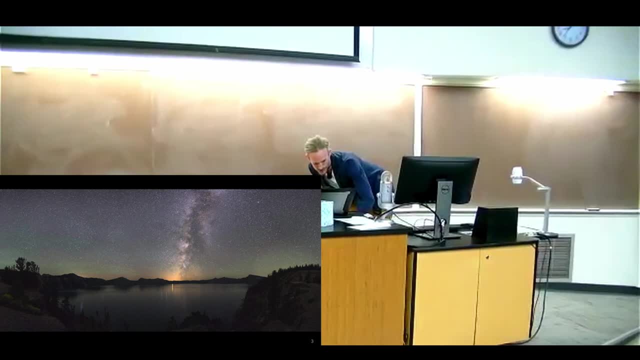 about all of those things. Can you guys see this projector very well? It seems a little light right now. You should see a nice night sky up there. Let's see if I can turn this down a bit. Let's turn it back down a bit, All right? OK, cool. 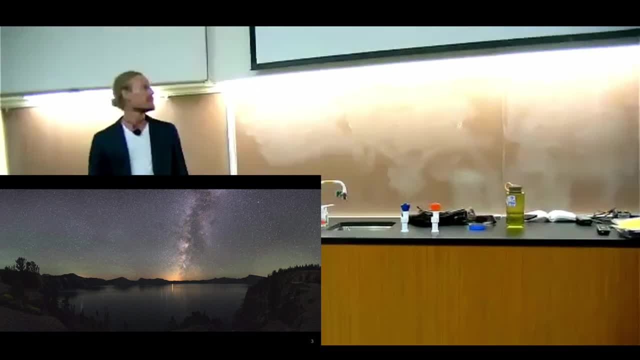 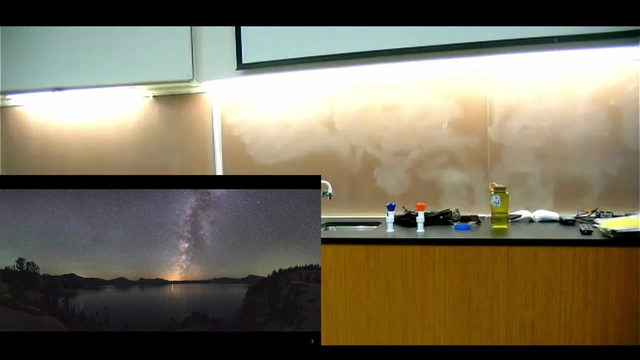 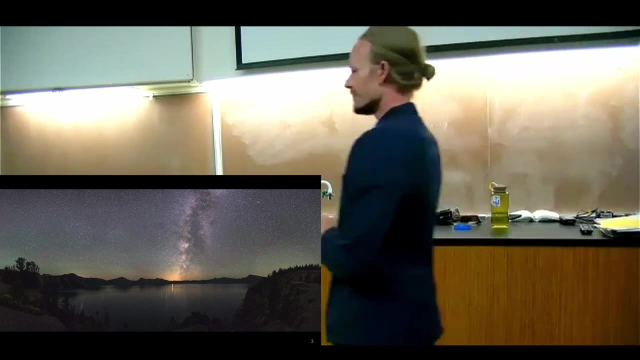 So this is Crater Lake. Anybody ever been there? Yeah, It's beautiful right Now. how many of you have gone outside and seen something like this? Yeah, A few of you, right? So people have been seeing something like this forever. So for hundreds, if not for. 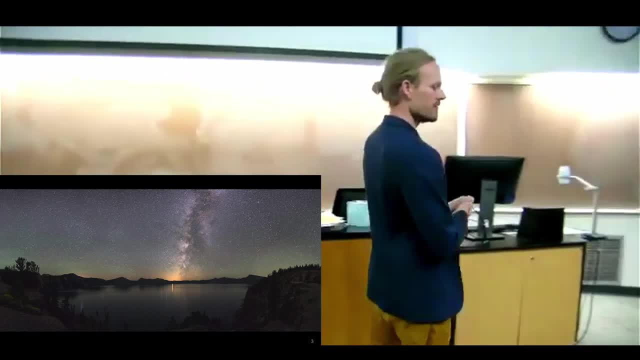 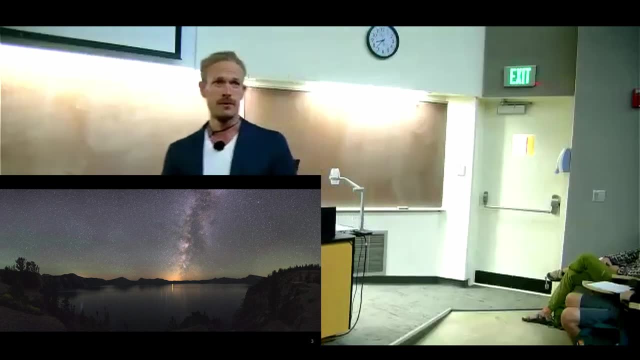 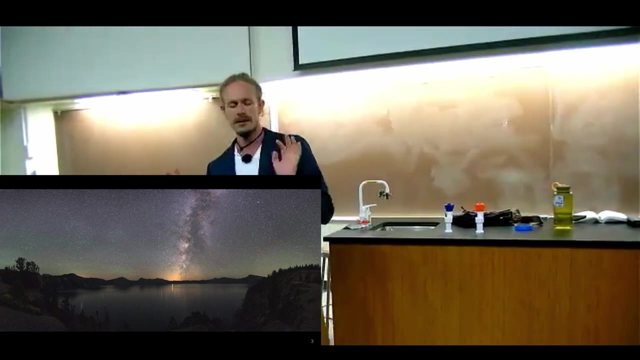 hundreds of thousands, maybe millions of years, as long as humans in their definitive form have been around, And this is a very beautiful and wonderful thing to see when you walk outside. But it's kind of strange to think I want you to do this, I want you to imagine forget. 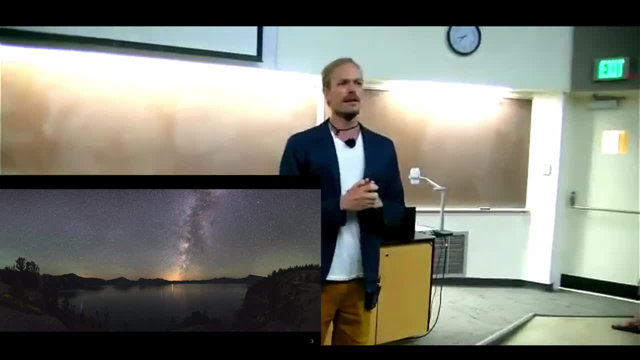 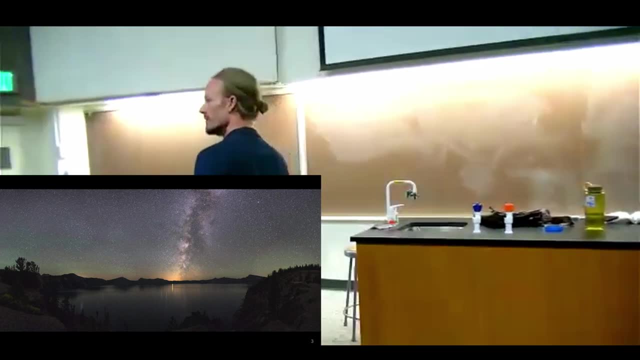 everything you know about. I want you to think about science. Forget that you know that gravity is a thing. Forget that you know that a star- anything you think you know about a star- that it's this orb of glowing hot material. Forget all of that for a second. Imagine that you know none of. 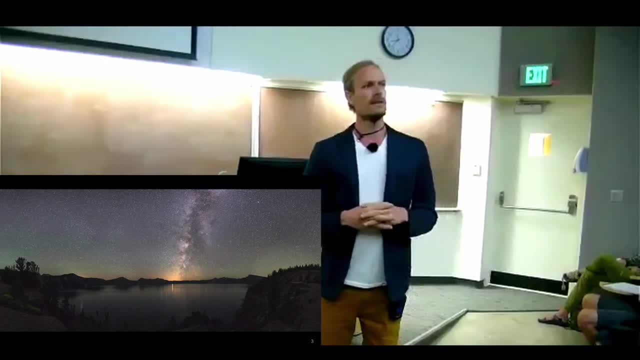 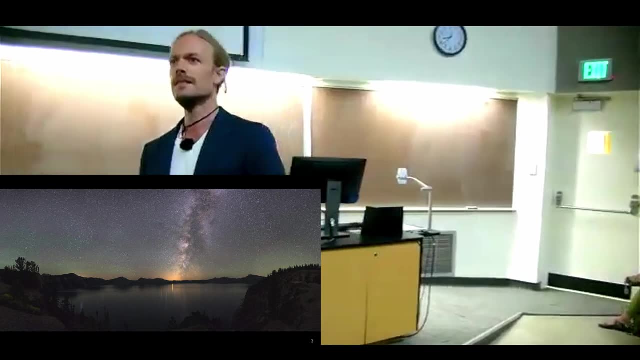 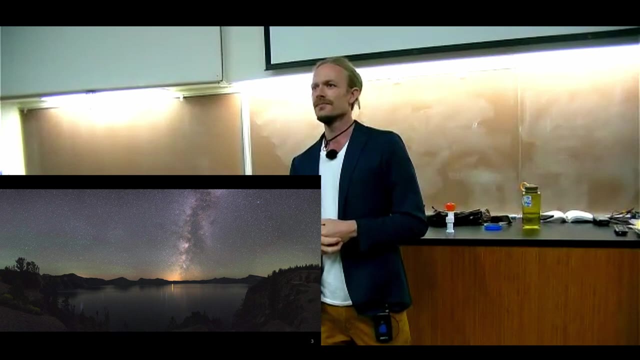 that. Imagine there's no cities to go back, to. Imagine that you walk out into the world and you just and you look up at the sky And what do you make of it? What do you make of it? Right, You have to, I mean, and what is a god really? right, It's some overarching form. 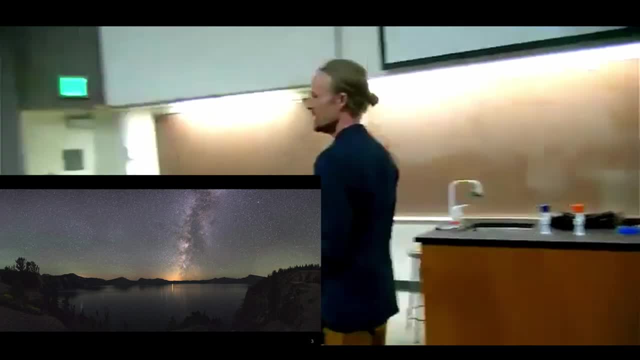 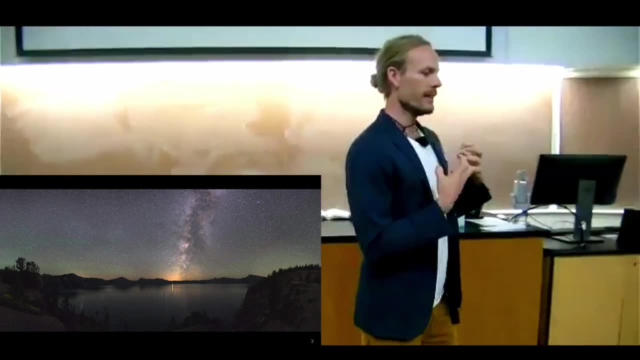 of everything that is powerful, everything that is represented by nature. You're seeing, you know, in our modern society, we don't accustom ourselves to things like the brutal forces of nature. right, We have roofs over our heads, We have climate control, You know. 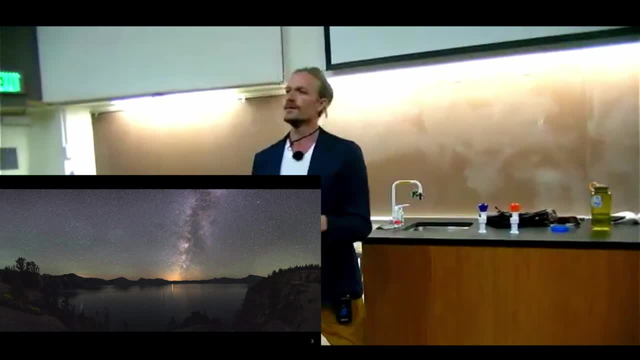 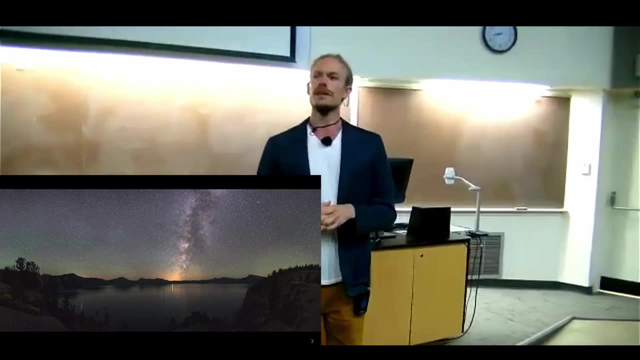 when someone dies in our society, they're immediately taken away, And these things weren't the case for thousands, maybe millions of years. this wasn't the case. Nature was a very brutal and ruthless force, and it wasn't clear exactly how you navigate. 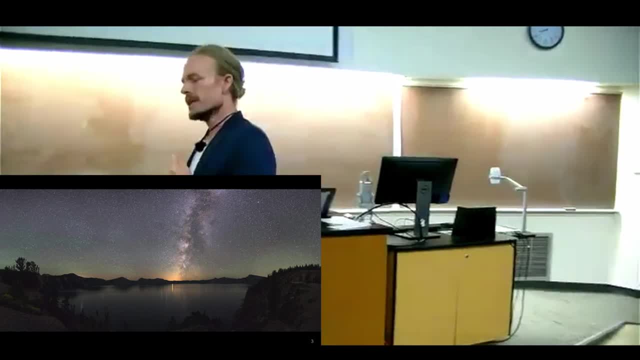 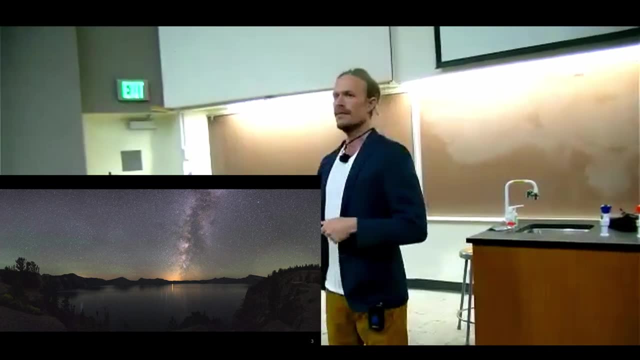 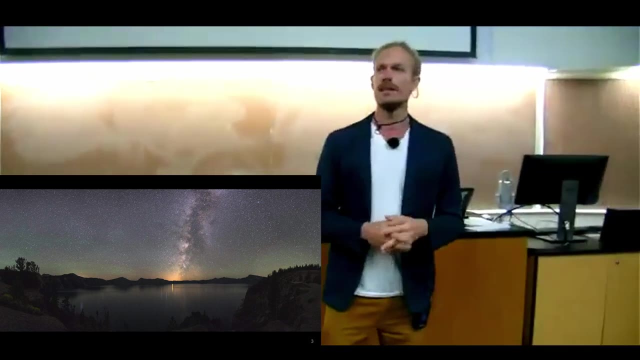 that okay, But one of the most comforting things, I believe, for the people who were around at that time, was that this happened every night and it happened in a very predictable fashion. right? You didn't have TV or Instagram or TikTok. You didn't have Facebook. You didn't have 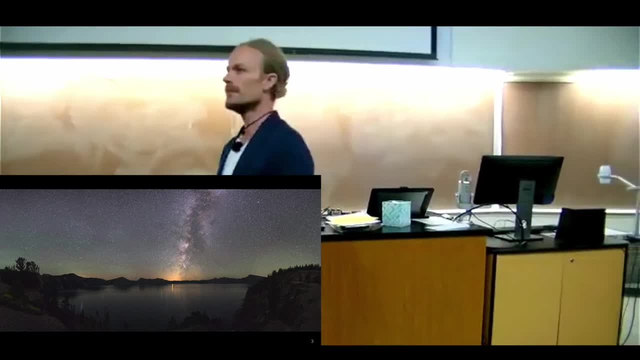 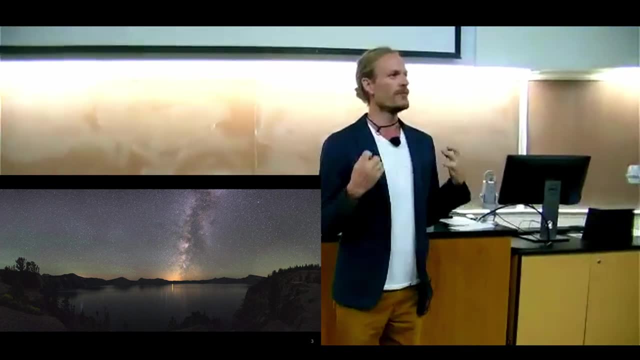 TikTok right, You just had the night sky, And so people would sit around and they would look at this, and this was their entertainment. Not only was it their entertainment, but it was also something reliable that they could reach to. they could pin their existence to. 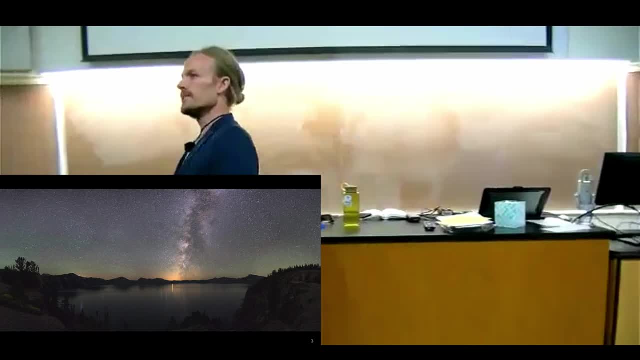 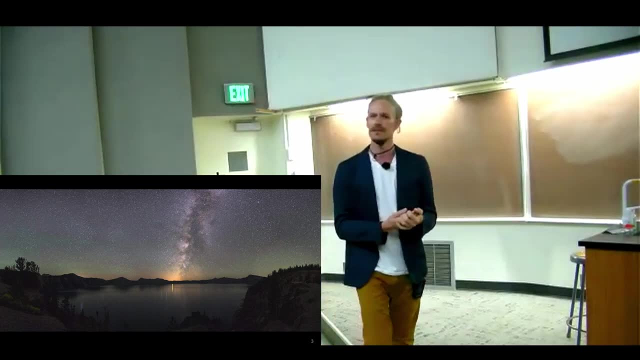 And, as we'll see, it was very instrumental from a technological standpoint, because it allowed people to survive right, They were able to time the planting of their harvests, They were able to perhaps time their fertility cycles so that they could actually generate and make more people. 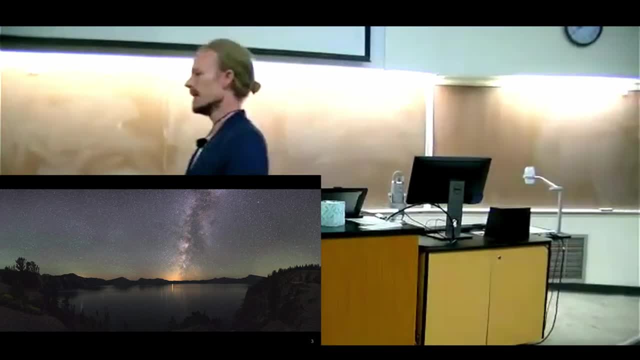 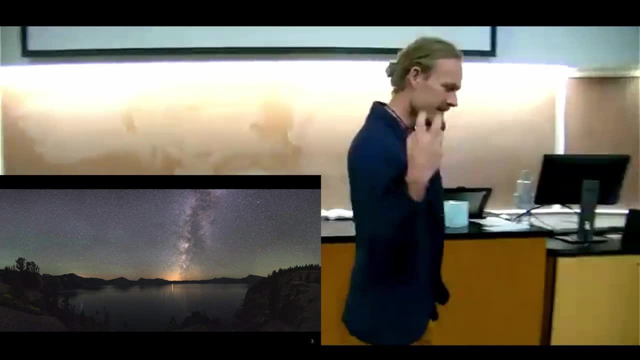 And that was really important when something like you know, one out of ten children survived to adulthood. right, which was the case for most of human history, which is inconceivable to us today. right, You have a problem, you go to the hospital. There was no hospitals. 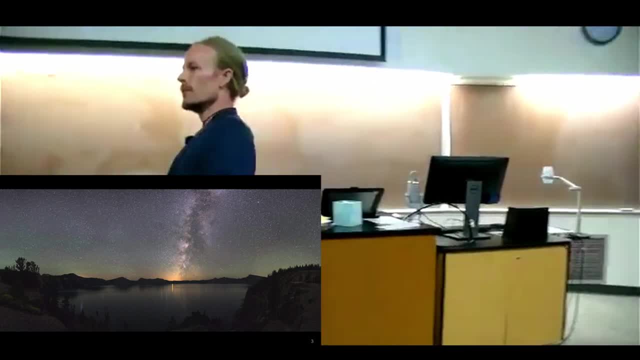 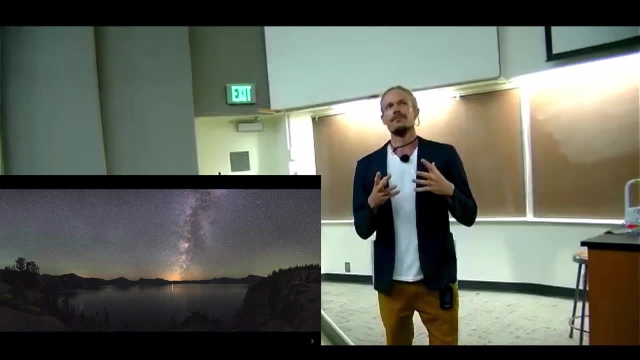 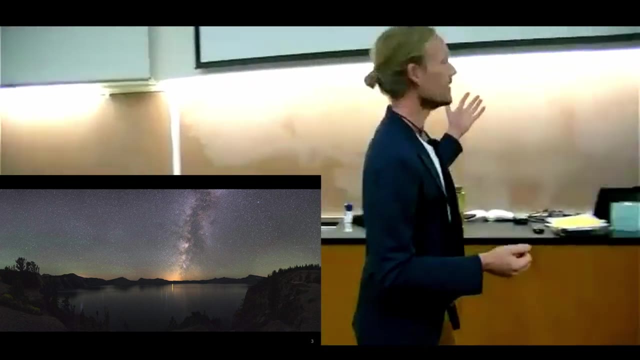 back then, right, So this is a very different world for 99.9% of human existence. It was a very scary but also a very wonderful and wondrous place. right, We didn't have answers. So what was your name, by the way? Thedo? So what Thedo mentioned? 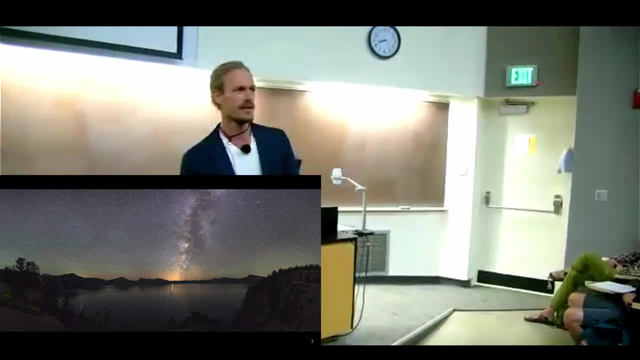 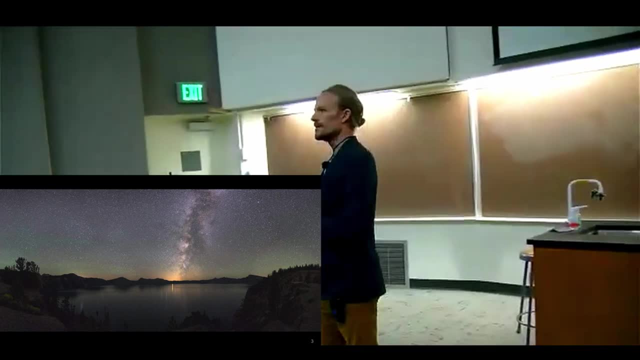 was that people probably thought of these as gods, and that does seem to be the case, and we'll get into that more- And it's not an entirely unreasonable assumption, right, And I think that's another thing that we have to start to accustom ourselves to is these: 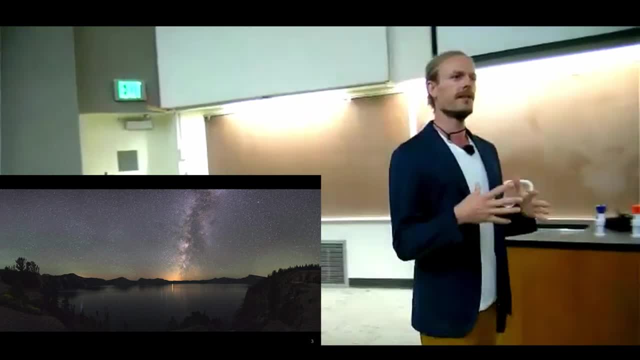 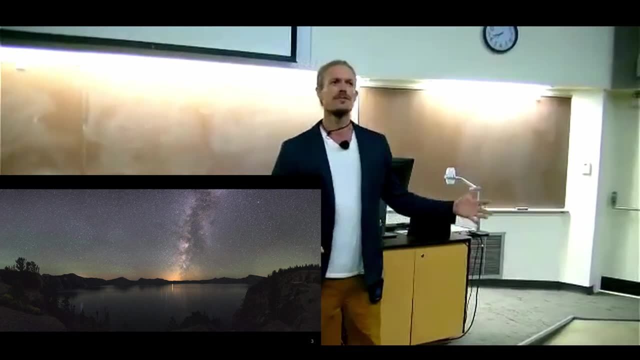 weren't idiots right? It's very easy to look back into history and think: well, these people didn't understand the laws of gravitation, they didn't understand you know how quark works, or protons, or anything like this. They must have been morons And it wasn't so clear. 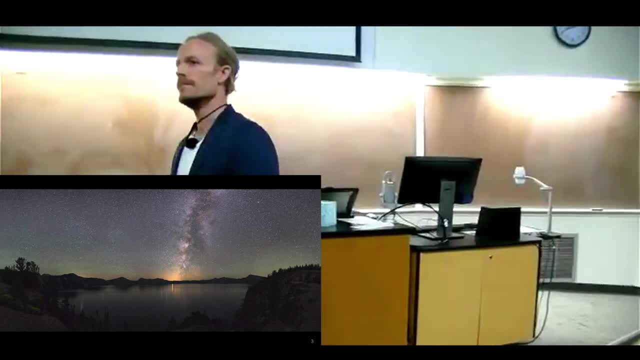 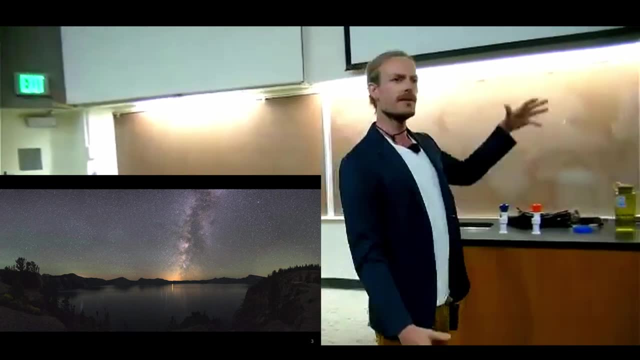 that this is the case. In fact, I would say it was much more the opposite. Their solutions to what was happening in the sky were very much informed by what was happening on Earth, And so the stories they told about these places often reflected what they idealized to be. 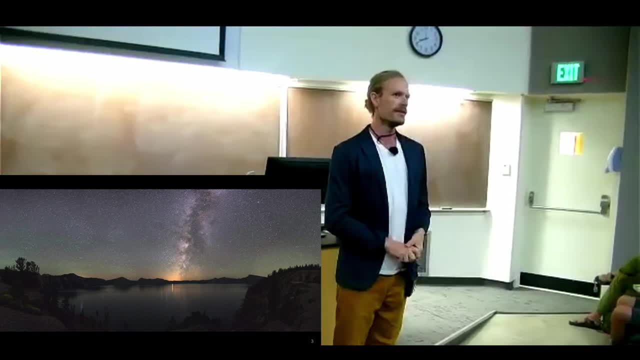 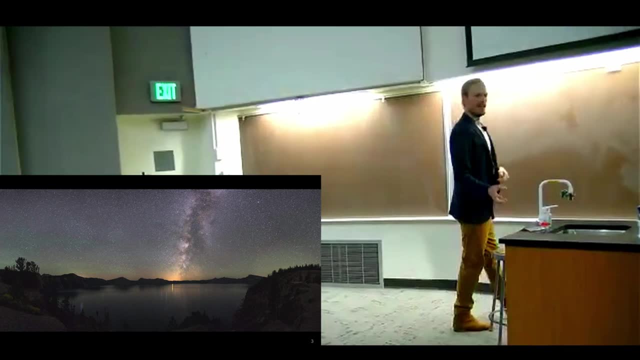 the case on Earth and the way that they wanted their civilization to unfold. And that's really, really important Because, you know, in our modern society it's not always the case. It's not entirely clear how you're supposed to behave at all times. right, It's very difficult. 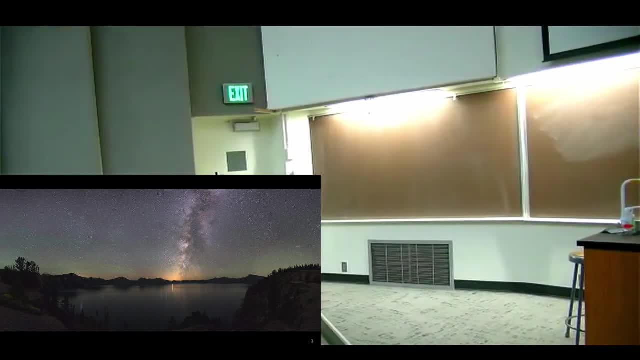 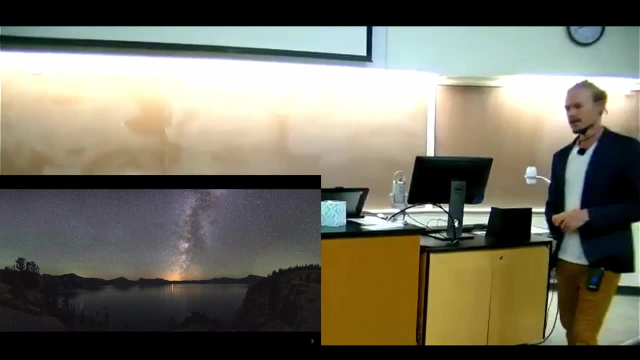 actually I have a lot of sympathy, especially for the younger people coming up in this world. right, You know, you wake up into a world where people say you can be anything, you can do anything. but this wasn't the case for hundreds of thousands of years. It was. 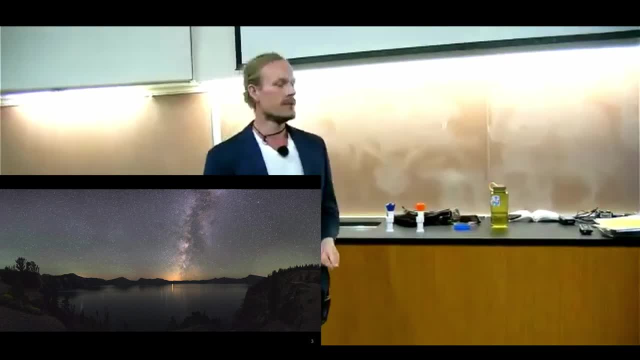 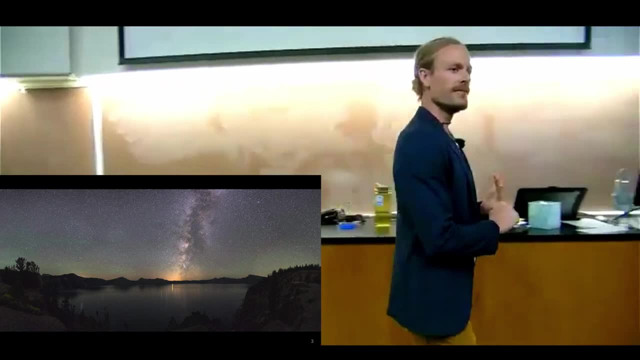 exactly clear what you were going to do. You were going to model yourself off of the various celestial role models that you had And you were going to go forth. you were going to make a family and you were going to succeed. And you were going to make a family and you. 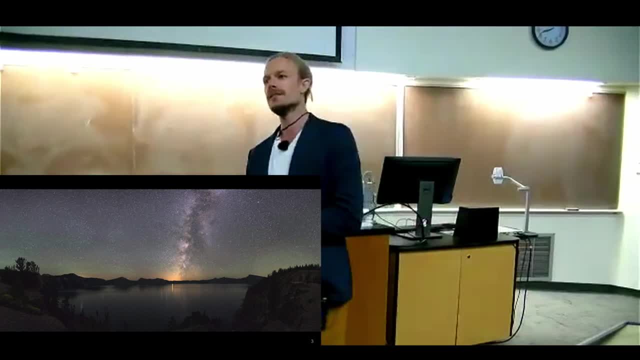 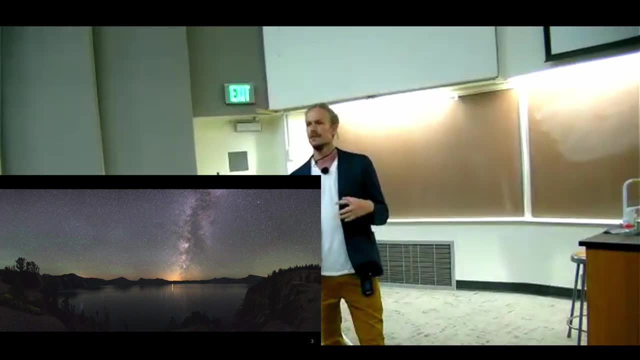 were going to sustain that family, and that's it for hundreds of thousands of years. It's very confusing today, And these people had developed very rigorous systems to be able to instruct the young to how to go forth and actually make this life, And so the story. 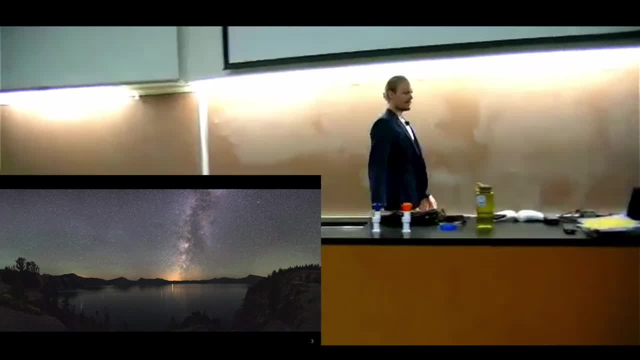 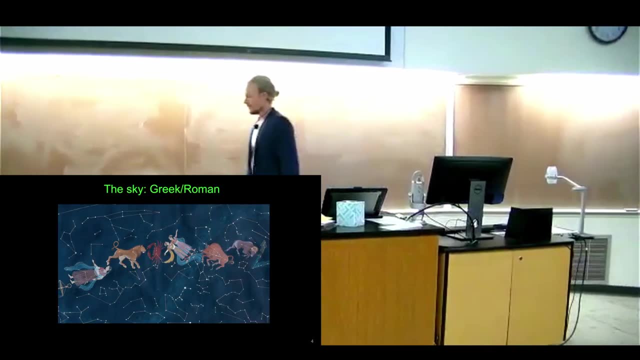 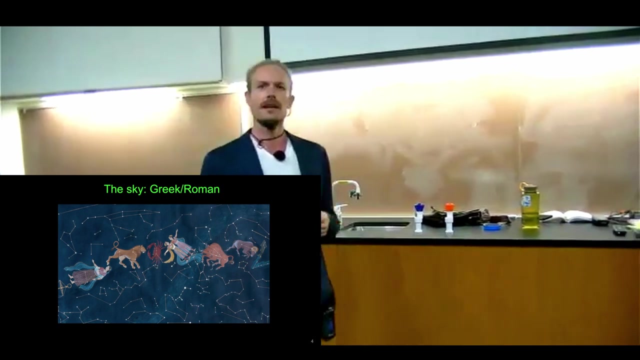 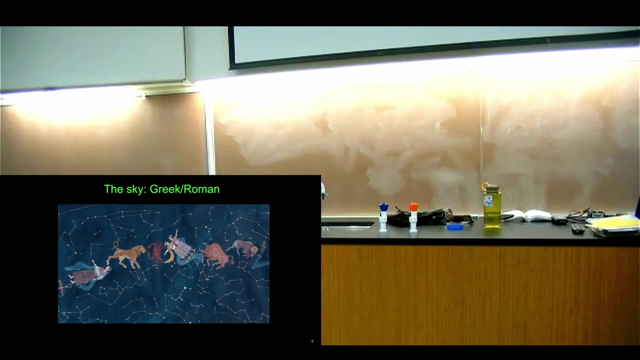 of the gods was really important. okay, Now, when they looked up, you know, perhaps you guys have seen some of these pictures, Right, These things, constellations, right. And you might think to yourself, you know, the first time someone showed you a constellation, they were like, ah, this is the Gemini, right. 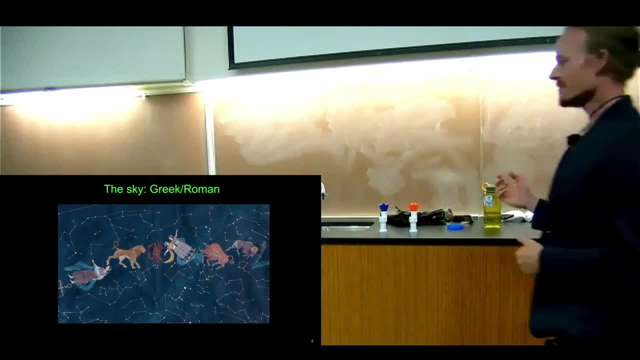 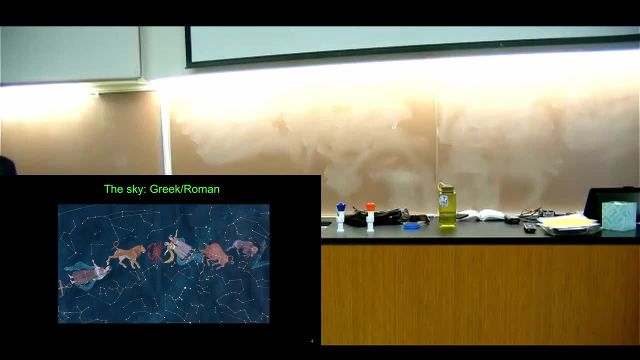 They don't look anything like that, though, right, And you're like what's wrong with these people who came up with these ideas? This looks nothing like two twins, right, But that's not the point. The point isn't that they look like the twins. The point is: 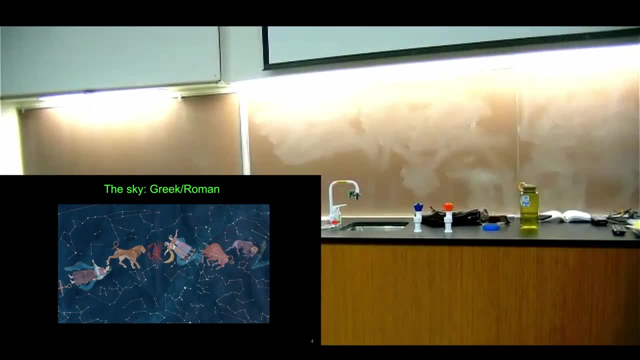 that they're gods. The stories they told of how to conduct themselves on Earth, they're born on Earth and how to survive into the next generation were reflected by these characters. So they had these stories and they needed to use the stars to tell those stories. It's. 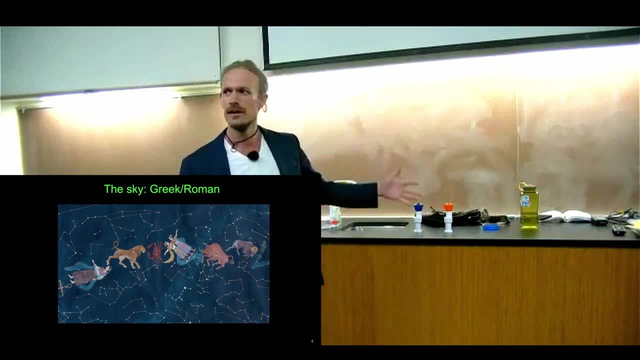 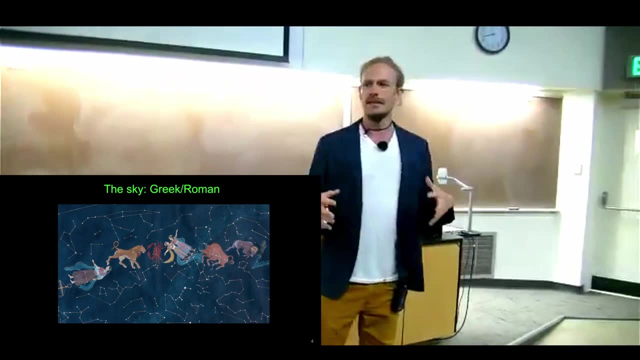 sort of like having a projector on the screen. People would gather around, almost certainly, and they would tell these mythological stories that were archetypical, right? They contained all of the necessary information for the people to be able to go forth and succeed. And what? 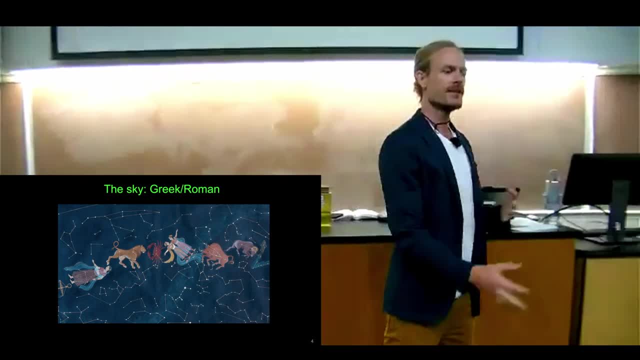 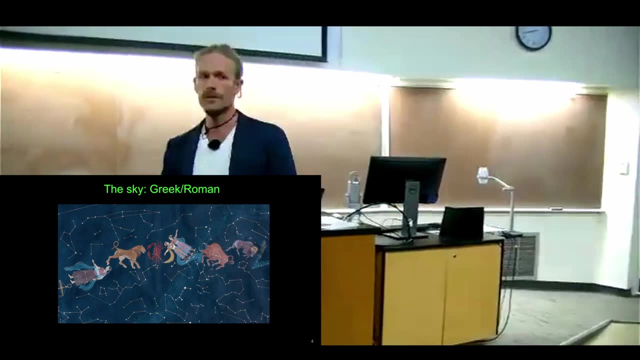 does it mean to be archetypical? It means you can't push past it. It means all stories converge on that story, right, And so there happens to be a myth for each one of these characters. This actually happens to be the Greco-Roman tradition, which 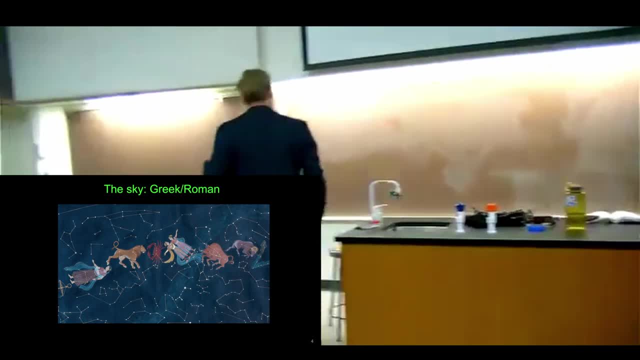 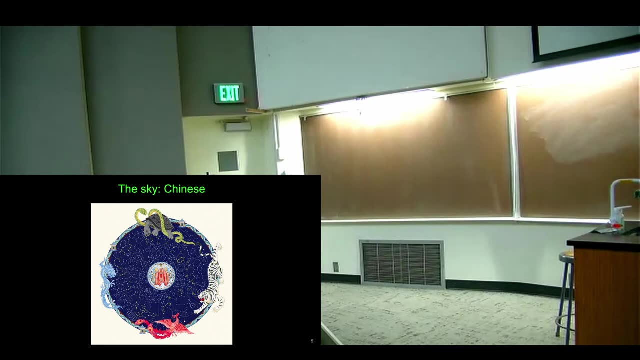 is the one that you're most familiar with. But as you look around the world- and we're going to get more into this next week- We'll go through all the different cultural interpretations of the constellations. But perhaps if you were born in ancient China, you would have. 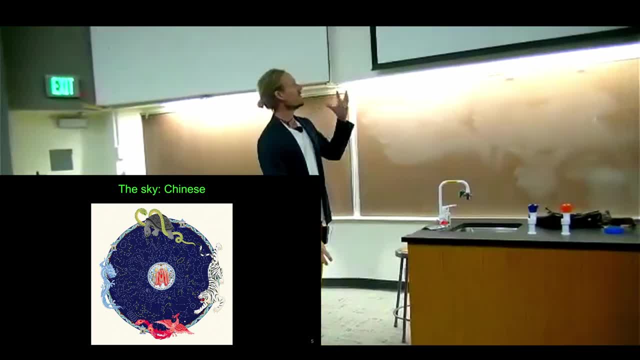 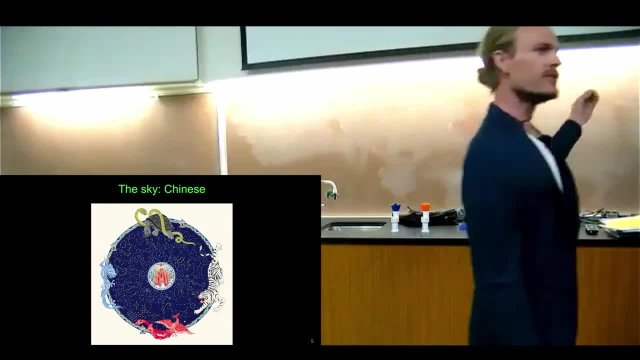 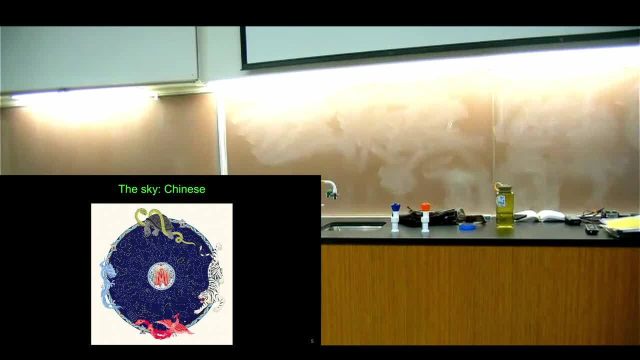 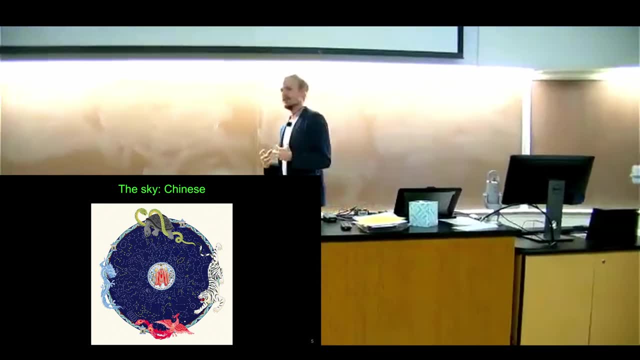 universe on Earth, And so you pin them to something that you see in the sky. this is really important: that you you understand that the constellations are actually symbolic, They're Archetypical, They're not actually supposed to be pictorial representations of. 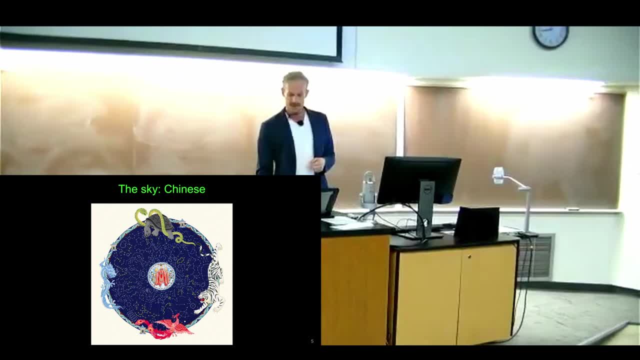 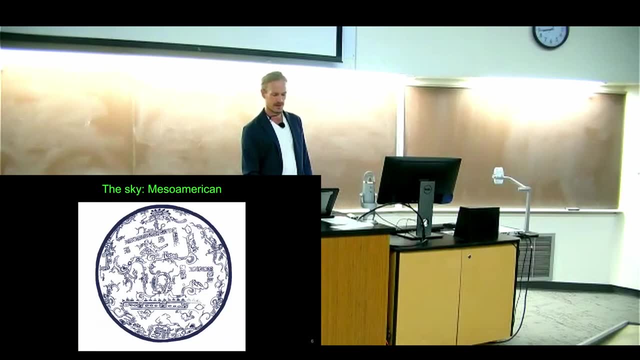 what's happening, And actually they're quite useful, even today. Obviously, we still use them, And we're going to talk a lot about that in terms of how to figure out where you are in the sky. so again say, if you were born in, uh, into like a. 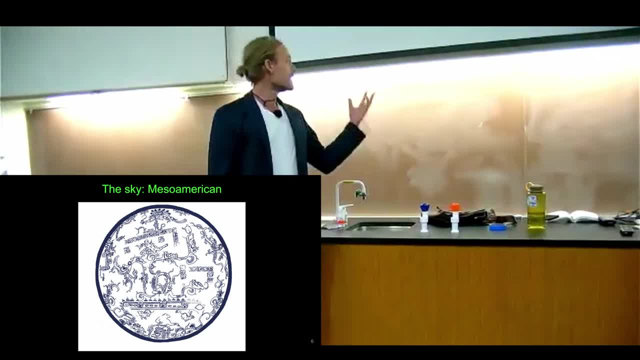 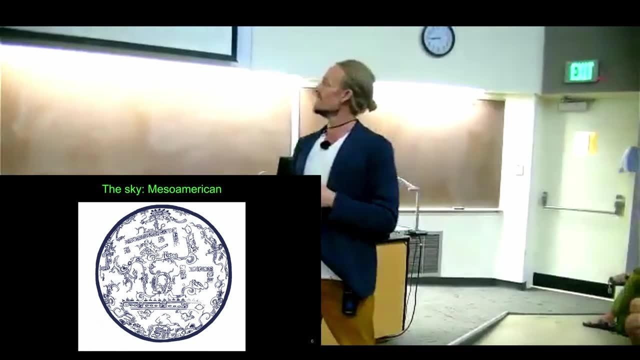 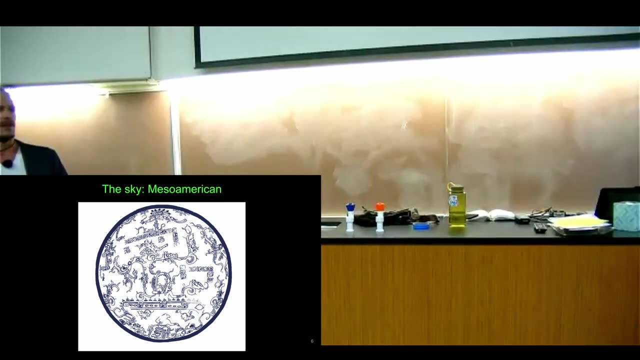 pre-mayan civilization or somewhere in mesoamerica, perhaps you would. you would explain things in terms of of giant, uh, giant feathered serpents, or or in terms of, uh, of of ruthless gods or serpents, or or whatever. right, you would see things very differently and and we'll talk about all those. 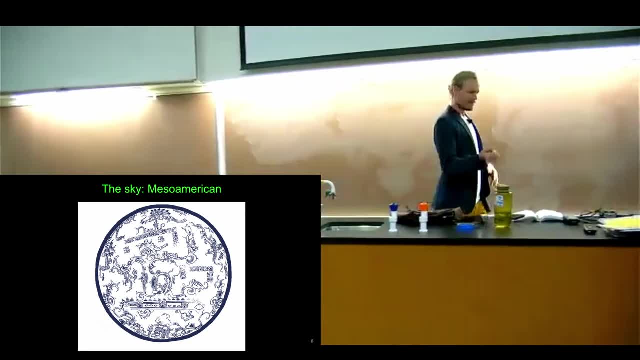 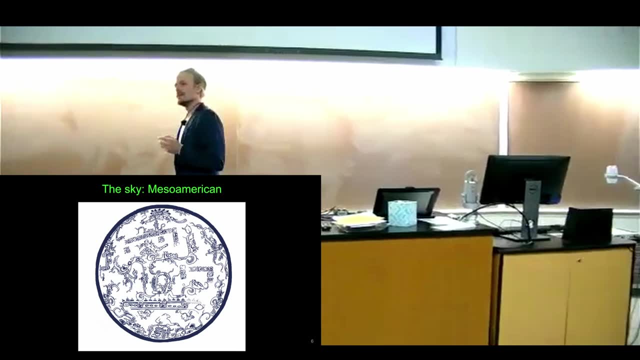 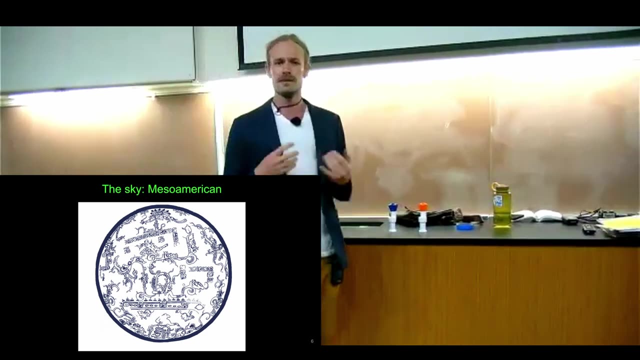 traditions, and i'm really stoked on that, because so often we think of, we think of science as being this homogenous western rational enterprise which it very much is today. um, but there's a lot of different traditions and nowhere are they more important than in astronomy and in cosmology. 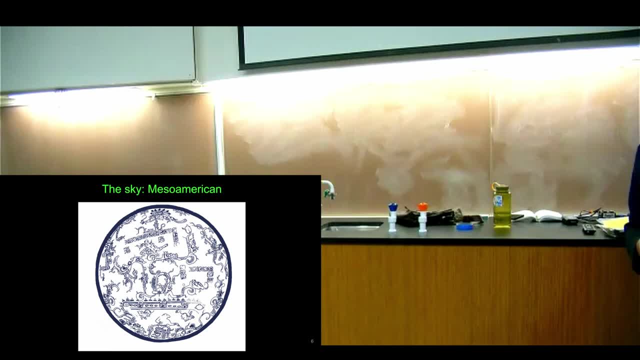 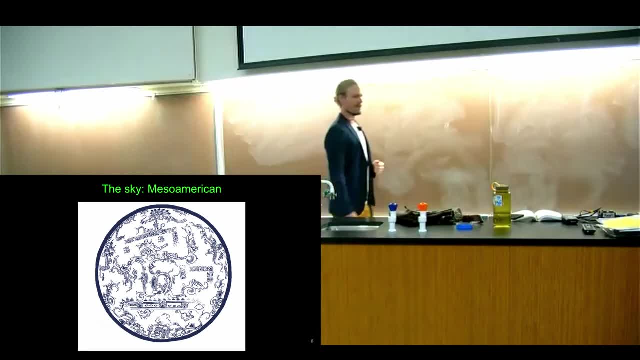 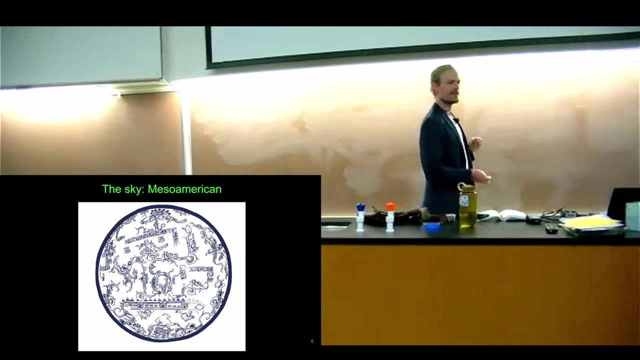 and how to make sense of it, but we'll overlap the two a little bit in this course. but what do you find is that each civilization has its own cosmology and there's not necessarily, you know, it's, it's hard to say with with any degree of certainty which cosmology is. 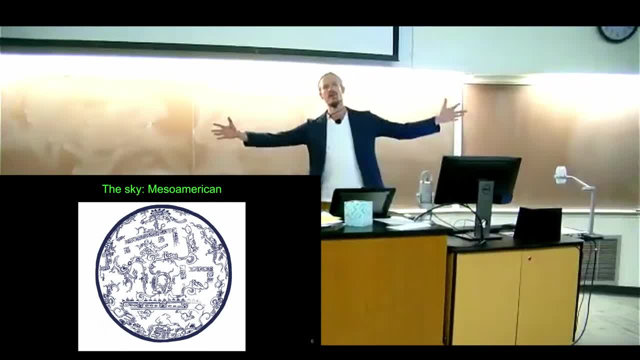 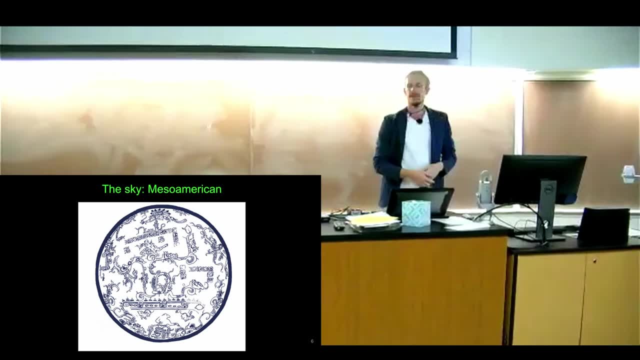 appropriate. the cosmology has to do with your own existence in the context of everything else that's happening around you. if you're born in the far east, your existence might be wildly different than if you're born into the mayan civilization. you have a totally different. 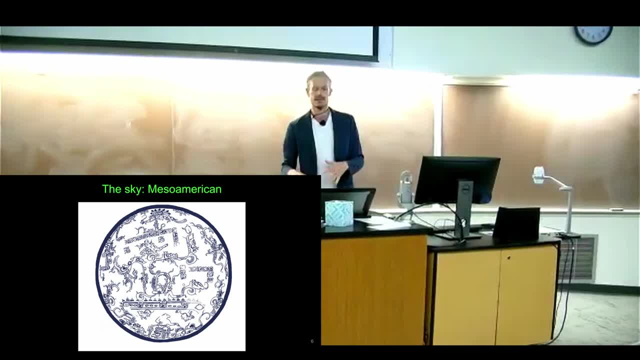 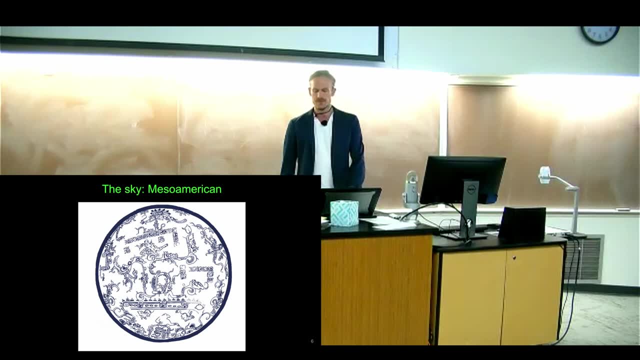 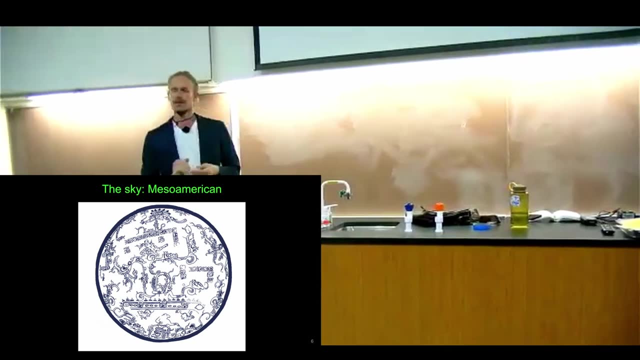 cosmology, and it might be more appropriate for you, honestly, in terms of surviving, and that's really the points of cosmology, uh, from an ancient standpoint. so people have been looking up at the sky for a very long time, they've been making stories about it and, like i said, the most 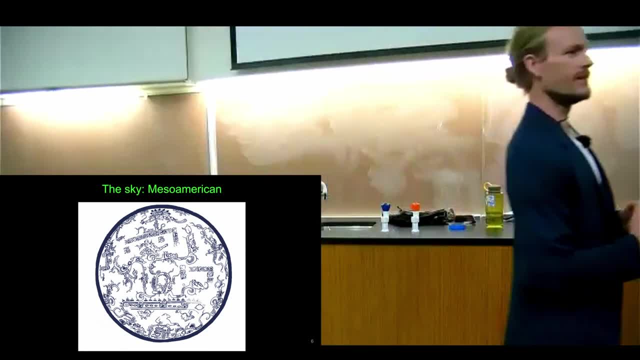 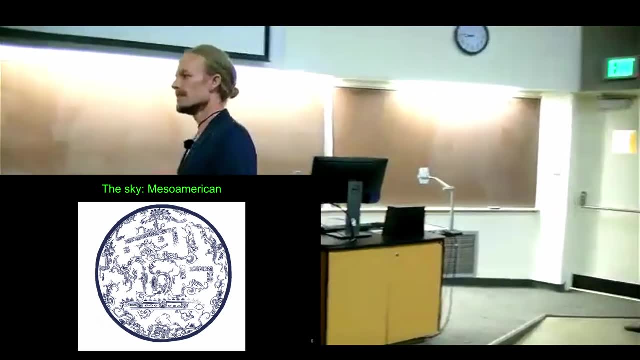 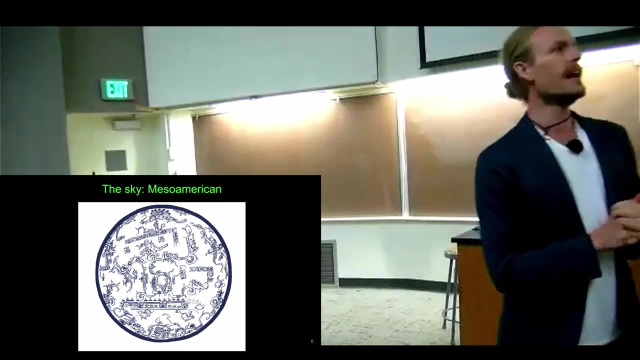 reassuring thing about this was that it appeared to be predictable. and if you, if you, don't understand how reassuring it is for things to be predictable, try to shake up your routine sometime, right, try to try to imagine not knowing what's going to happen to you tomorrow. you 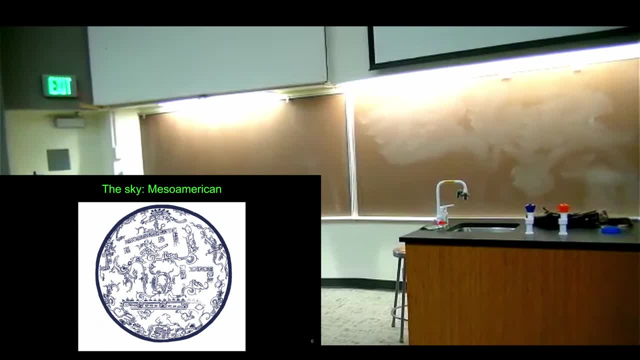 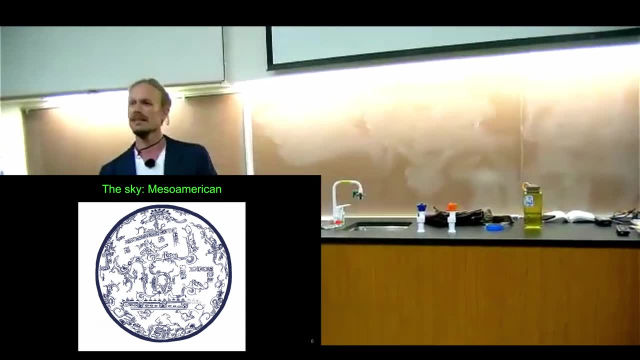 all know you're going to go to this class or the next class. without that, you're thrown into this, this real chasm of darkness where everything like who do any of you have cats? i, i'm a cat person. i have a cat. her name is mingus um. 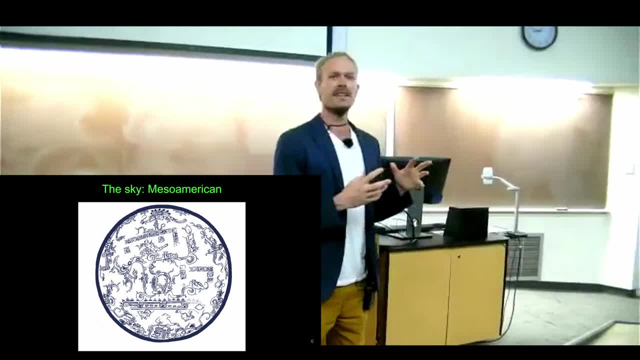 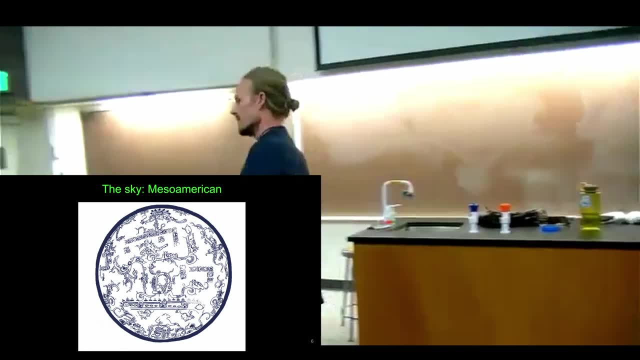 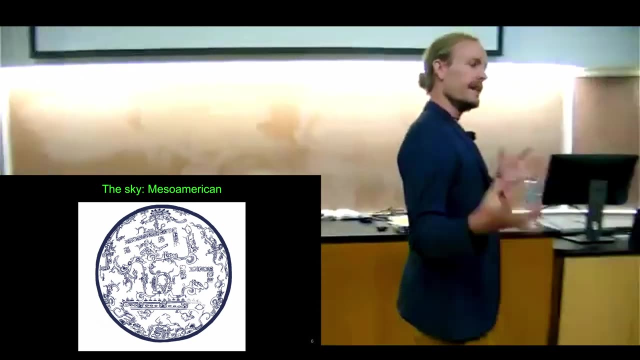 mingus is constantly alert, right. if there's a sound in the other room, she's like: oh, what was that right? she doesn't. she doesn't have this conception of what's going to happen five minutes from now, let alone what happens tomorrow. but- and the ancients started out this way too- the deep 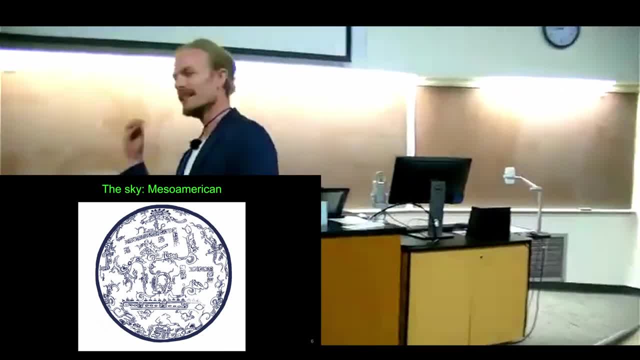 prehistoric humans. but the sky gave him a sense of regularity. it gave him a sense that maybe things are under control and actually if we pay attention to the sky, it gives him a sense of regularity. it gives him a sense that maybe things are under control and actually if we pay attention to the 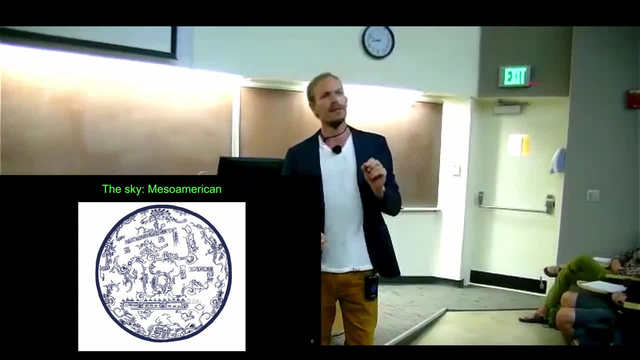 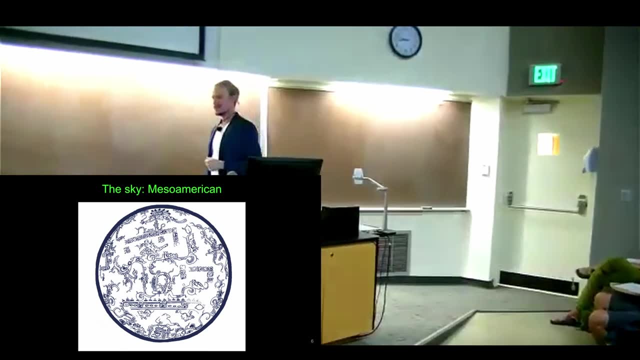 sky. it gives him a sense that maybe things are under control and actually, if we pay attention to it really well, we can come up with a pattern that will guide what happens to us in the future. this is really, really, this is really critical for understanding what it means to be a human, which. 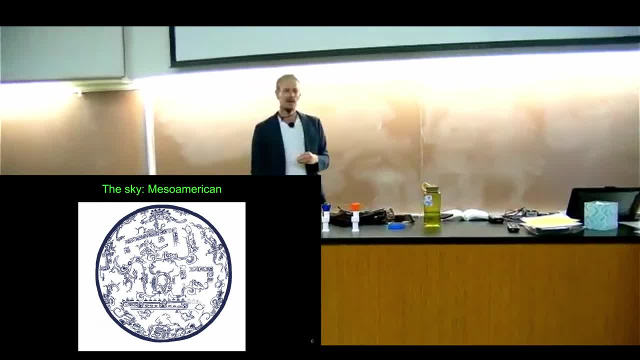 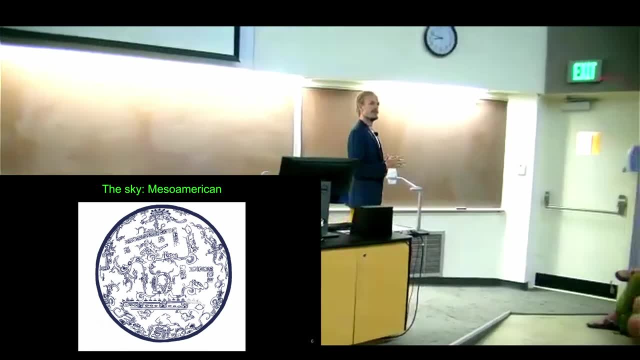 is having this ability to plan, which is having the ability to take control of our environment right. we're not just like, like. this is the primary difference between humans and other animals is that we can. we can reshape everything. we don't have to suffer the consequences immediately. 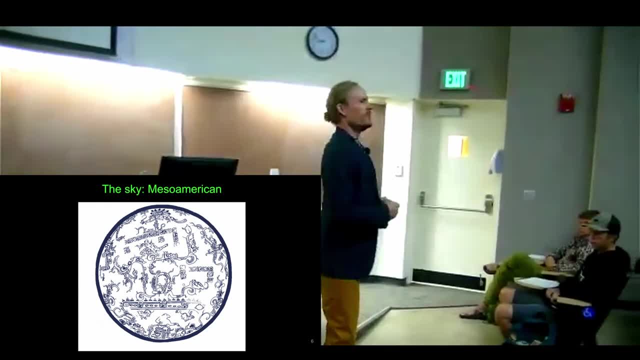 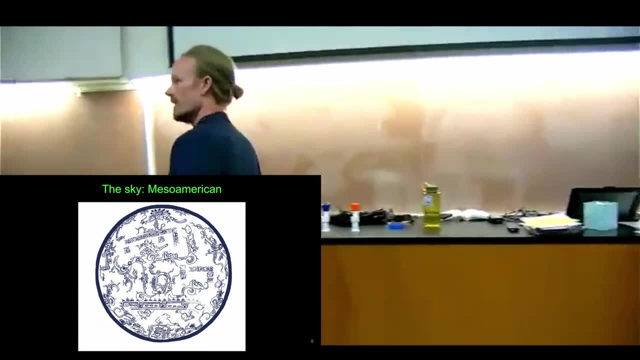 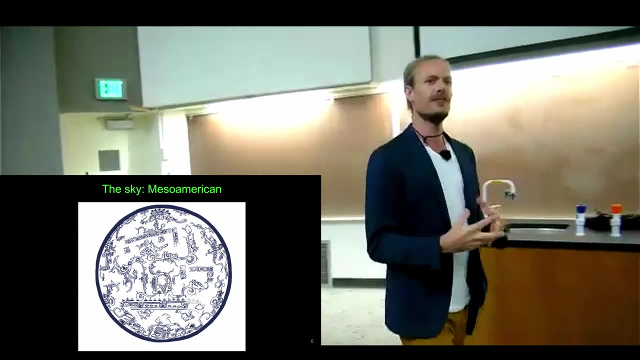 of what's being pushed upon us, and I really firmly believe that astronomy had a huge part in the developments of that concept of technology, right, the idea that we can make things to make our lives better because the world has predictable behaviors. alright, if I change the shape of this arrow in just 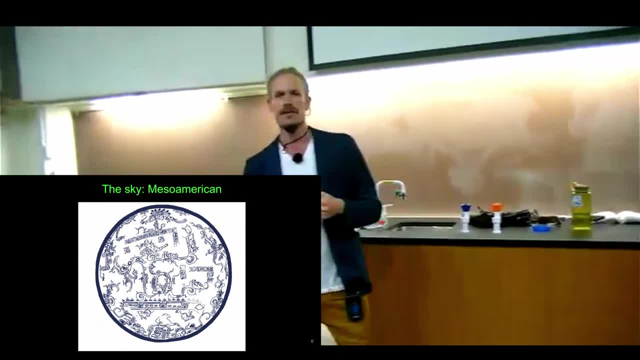 a little bit, then it's going to change the behavior of the arrow, and this is the root of how technology works. it's right, it's the root of how technology works. it's really, it's really the root of how it's really. it's really the root of how technology works. it's really, it's really, it's really. 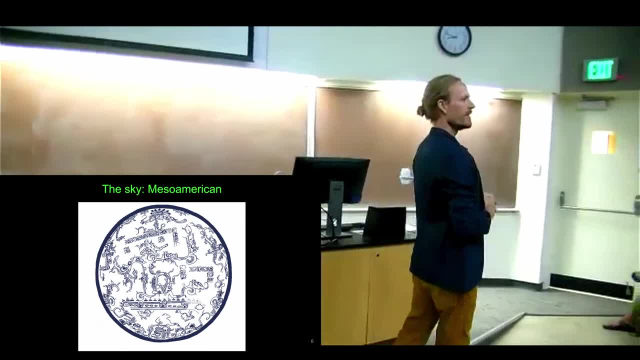 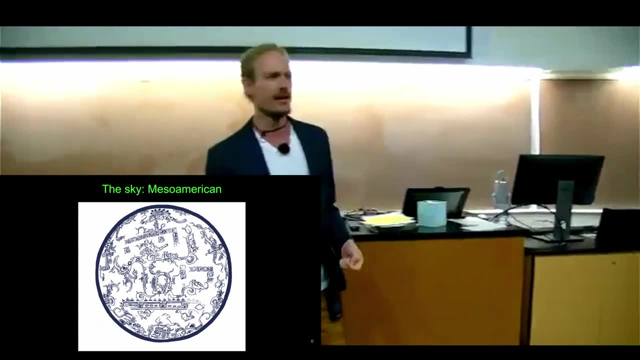 embarrassing to say that technology works through trial and error like this, but it is the case And we can come up with laws- which we'll talk about in a minute- that describe the path of the arrow right, And we can, we can. 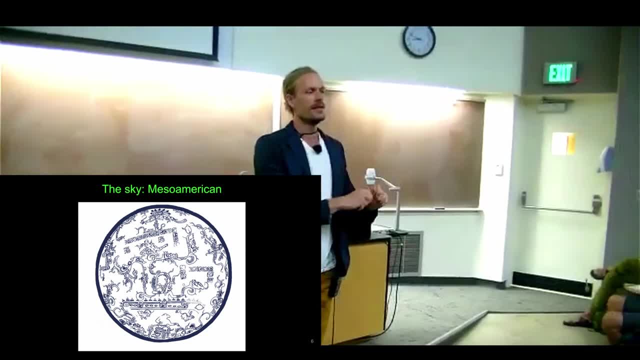 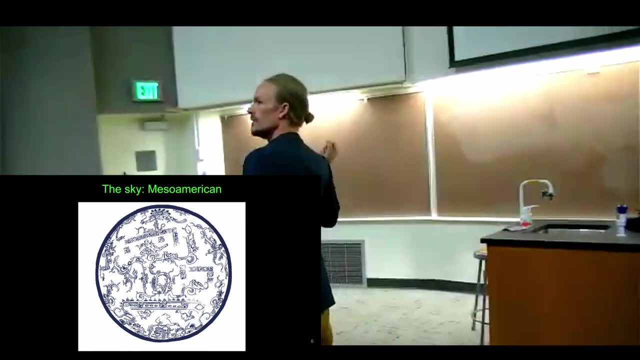 parameterize it and we can say, okay, if I change the fins this way, the arrow will change this way. This is really the harnessing of that predictive ability that all started with astronomy: Looking at the sky and saying, okay, tomorrow that Sun is definitely going to come up over there, just like it did the day before. 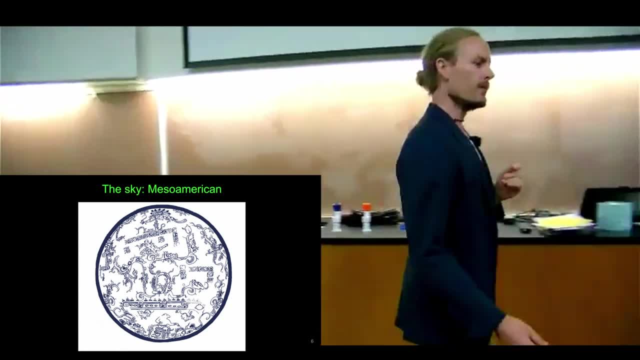 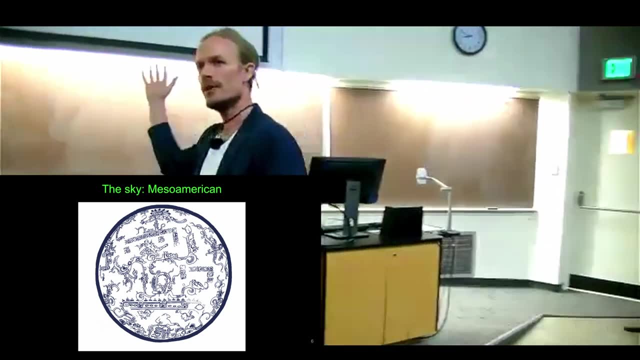 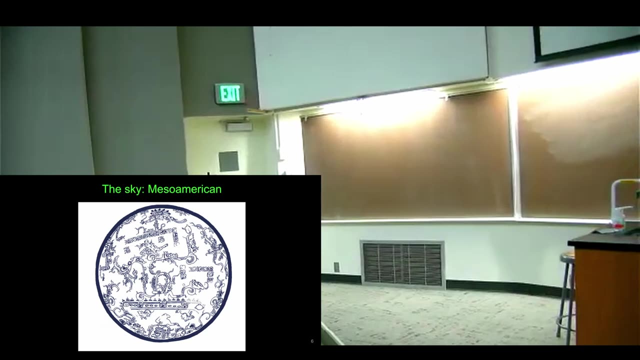 and the day before, And if we look really carefully, what we're going to notice is that actually these, these characters which we've assigned to these star groups, they come around in a predictable time every year. This is extremely reassuring, So we have evidence that people were taking note of this, for 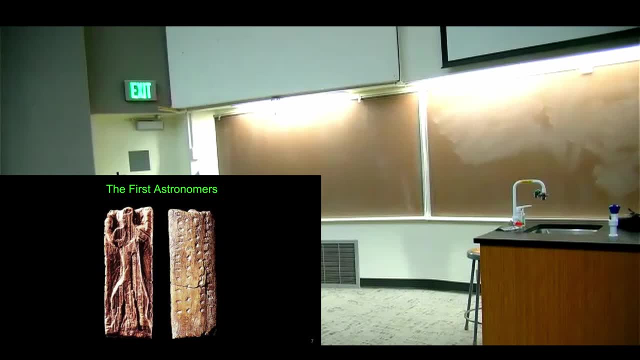 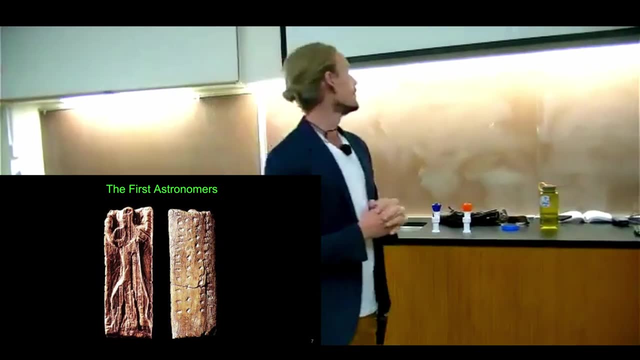 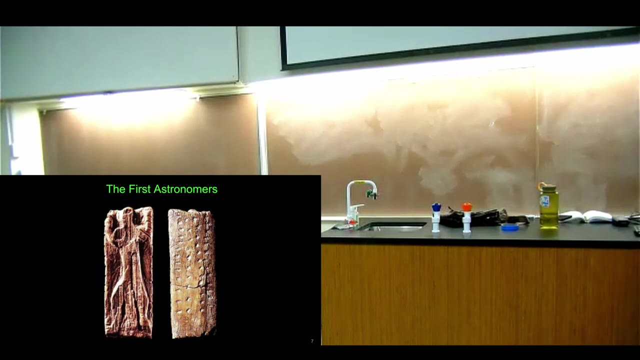 quite some time, And what's interesting is that artifacts were accumulating for the last hundred two hundred years and people would look at these and they'd be like, oh, it's just a, you know, it's a totem God, representation of this primitive culture. I want to say that 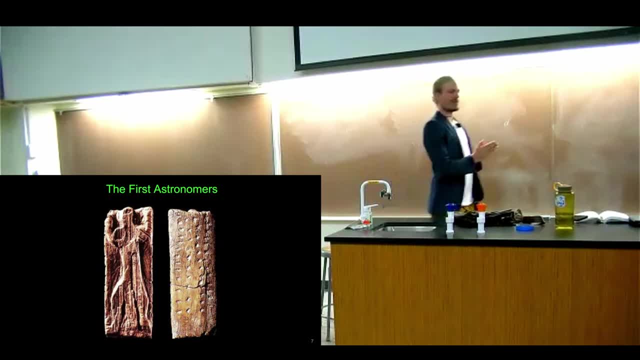 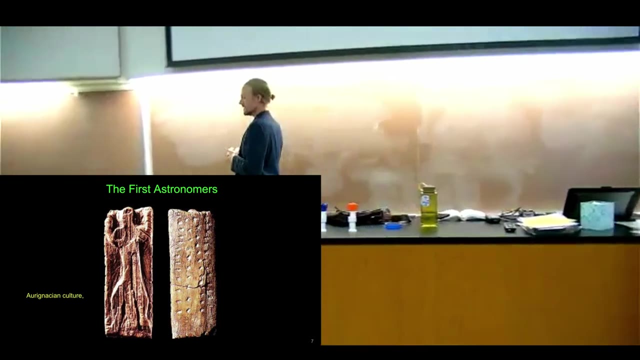 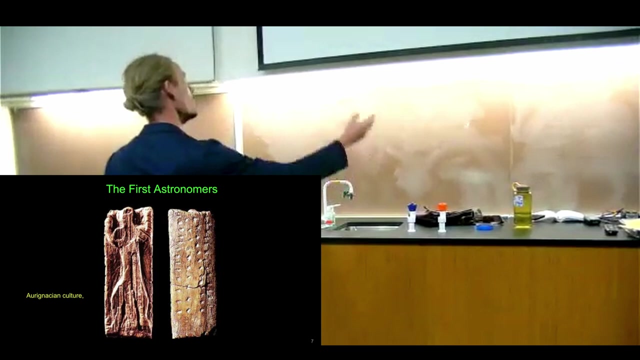 this actual carving. let me see, this is about 30,000 years old and this is from the Near East- sorry, yes, the Near East. somewhere in the Arabian Peninsula this was found And it turns out that when astronomers overlaid some of the, you can't really see them too well, but there's a couple of. 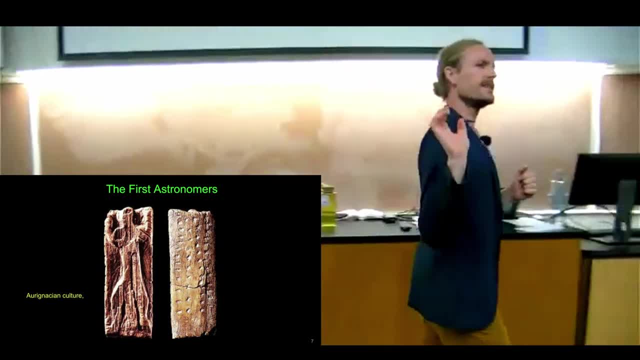 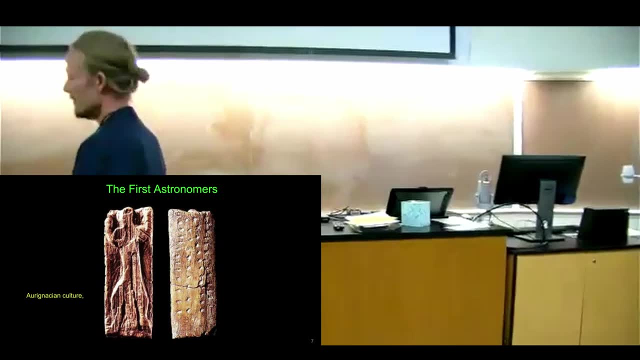 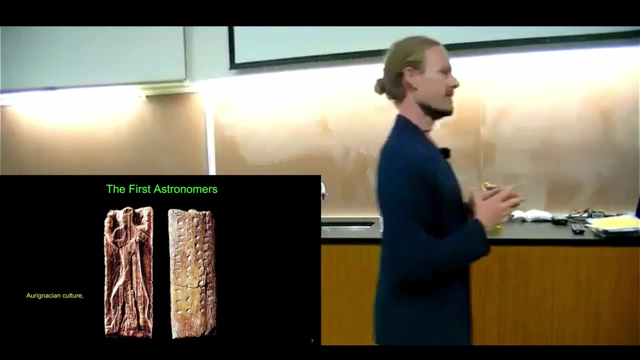 little dots on the chest. Turns out that these dots actually overlay perfectly with the constellation Orion, And they didn't discover this until quite a bit after they had found this artifact. But people were making notes of the locations of those stars for tens of thousands of years, And this has not. 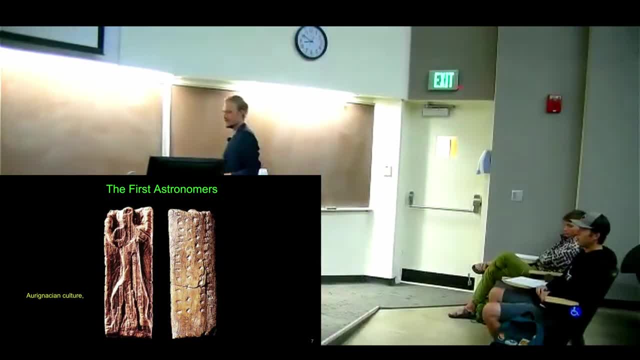 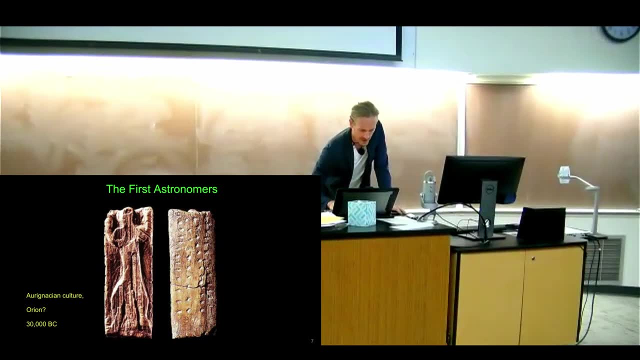 happening only in the Near East. this was happening all over the world. Let's see what else we have. Sorry, 30,000 BC, so 32,000 years ago. Here's another representation. perhaps you've seen this. This is a cave painting. 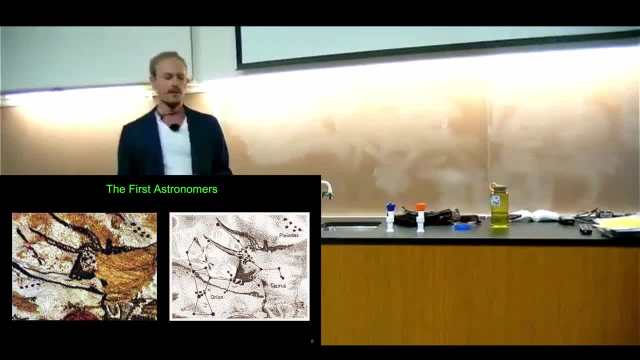 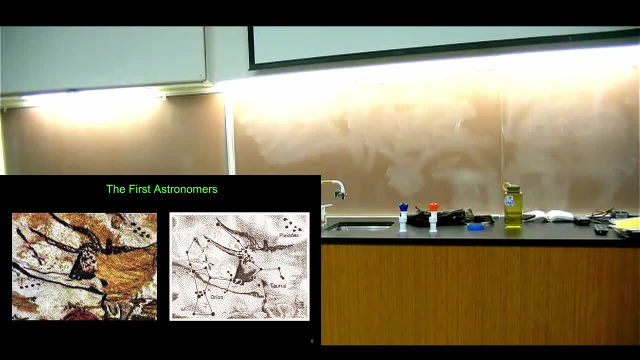 from this cave in France. There happens to be a number of cave paintings preserved in France. You can actually go there and look at this, although I think they they make you look at a replica of it now And for years they thought okay. 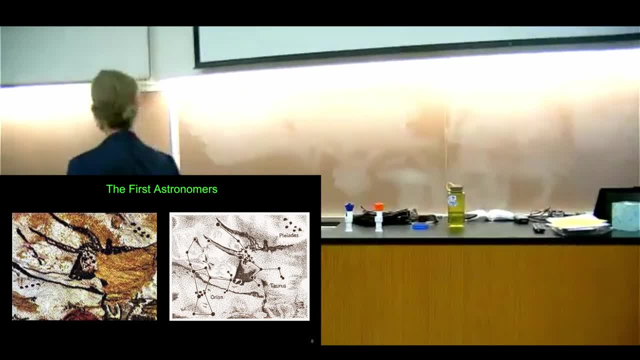 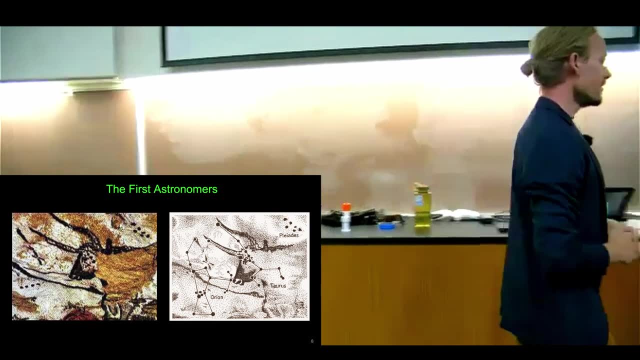 this is a beautiful drawing of some sort of bull, right? And aren't those some cute dots next to it, and so forth? Well, it turns out that couldn't have been further from the truth. This is actually a map of what's happening in the sky. 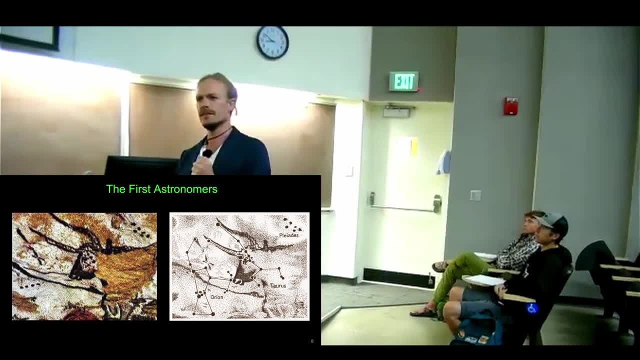 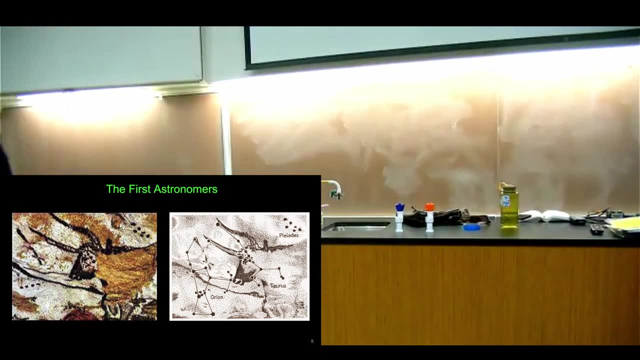 And this was. I think there's another aspect to this as well. right, There's the predictive nature that every year, at a certain time, we can see this constellation. It's in the same place. We measure its place with respect to where the sun rises every year. 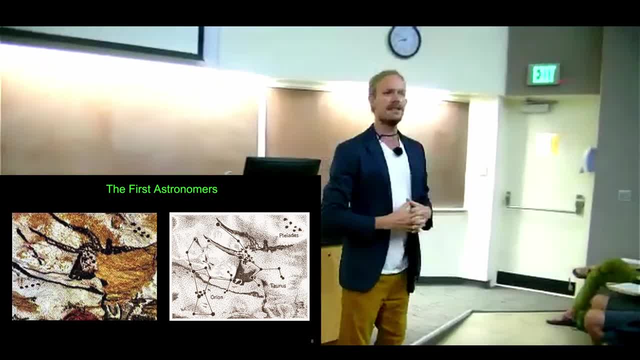 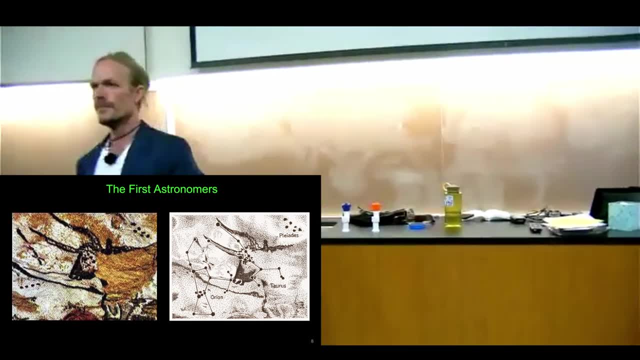 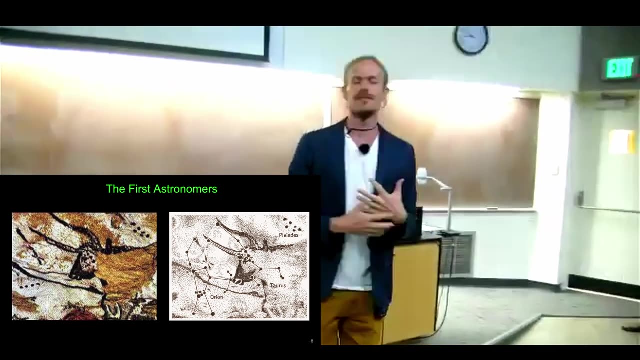 And I think this is where we begin to see the birth of hierarchies and hierarchical structures in society, because in each culture there's a group of people: the astronomers. this sounds crazy, but the astronomers were no different from the ruling class of those civilizations. 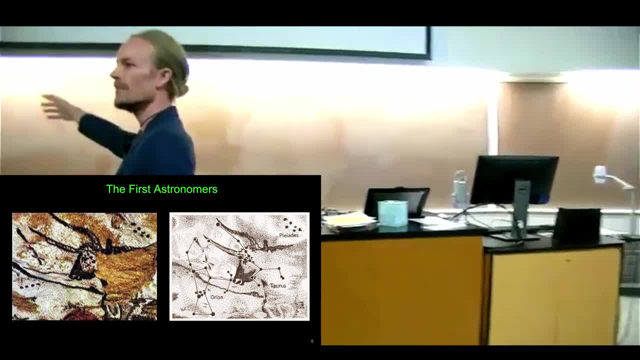 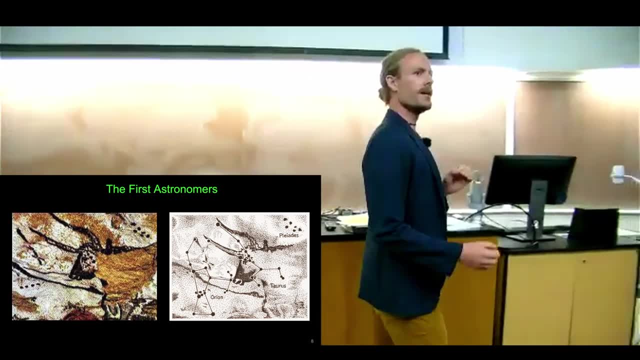 for the most part, They were the people that were able to actually divine what was gonna happen next year, what was gonna happen tomorrow, And they used these to some extent like a parlor trick. right, If I can tell you what's gonna happen tomorrow, 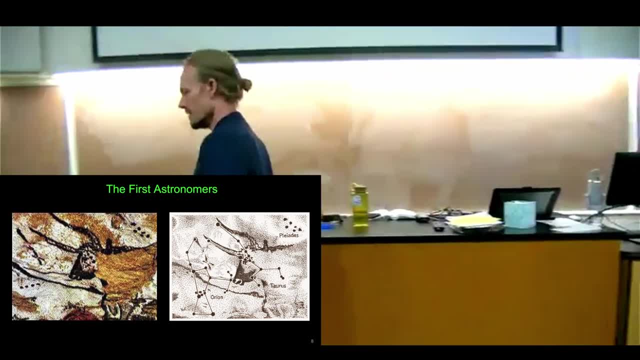 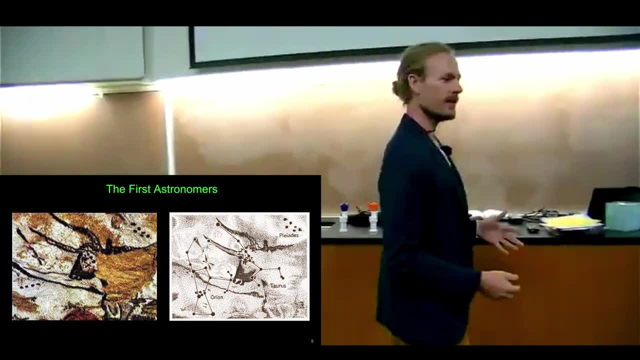 you're probably gonna believe me and follow me and do what I tell you to do. And I don't mean to say that these are like some oppressive, you know, ruthless, fascist ruling class. That's not the case at all. In fact, I would go so far as to say 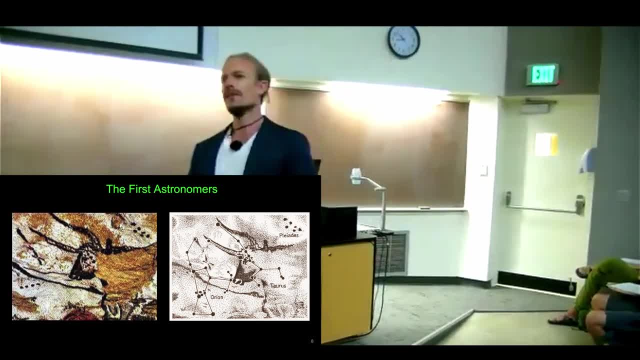 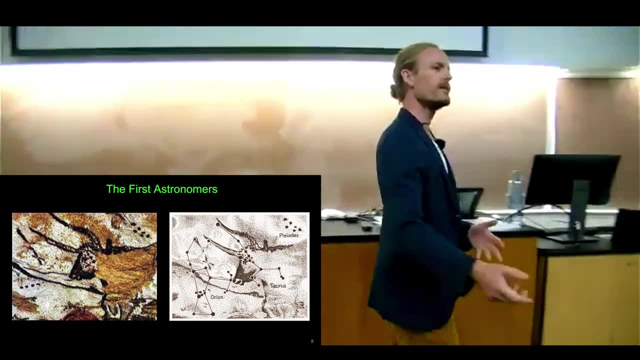 we all very much need authority structures. I would say that without someone to tell us what to do, if no one told you to come to this class this morning, if no one said: hey, you should, you know you probably. oh, you wanna do this with your life. 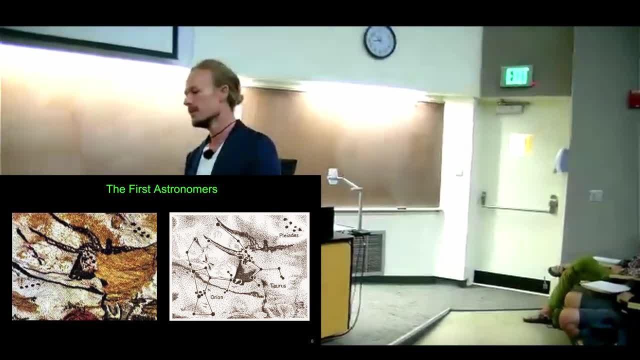 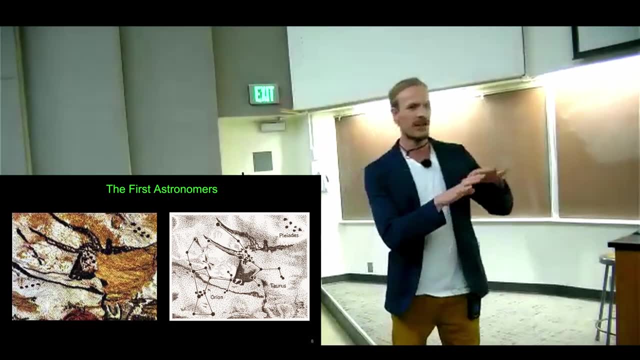 you should probably go to college Without some authority telling you what to do. the world becomes a very shadowy and mysterious and difficult place to navigate And so having this stratification start to appear where some group of people was able to actually inform the rest about what's going to happen. 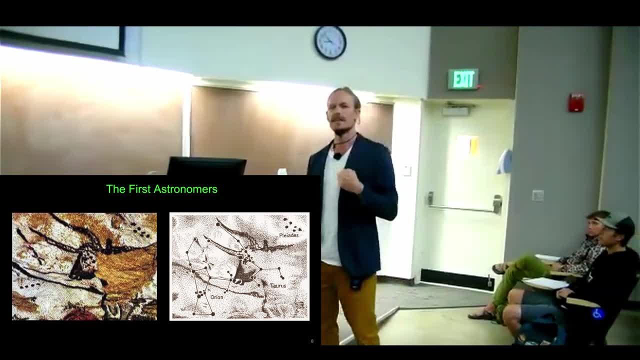 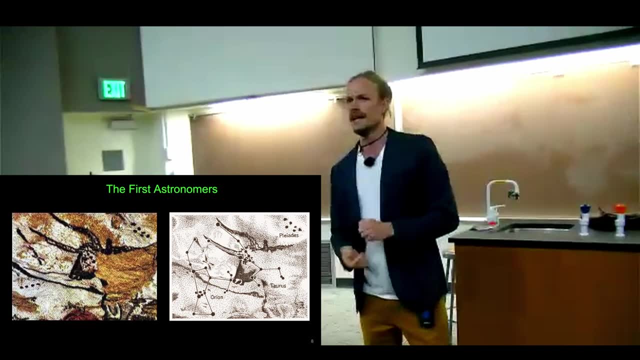 set the stage for this structure that we have today, And we're gonna see that more and more as we go through, especially once we get into the Greek and Roman traditions. It's really really uncanny how little our civilization has changed in the past couple of thousands of years, right. 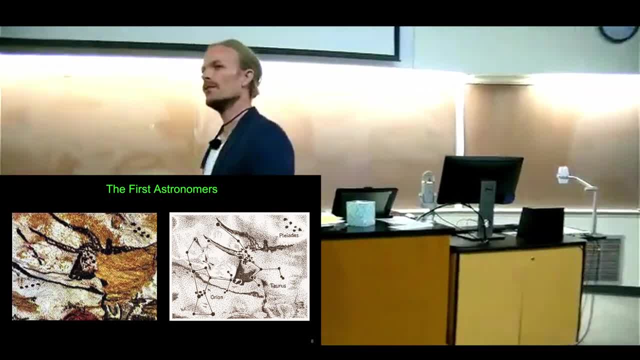 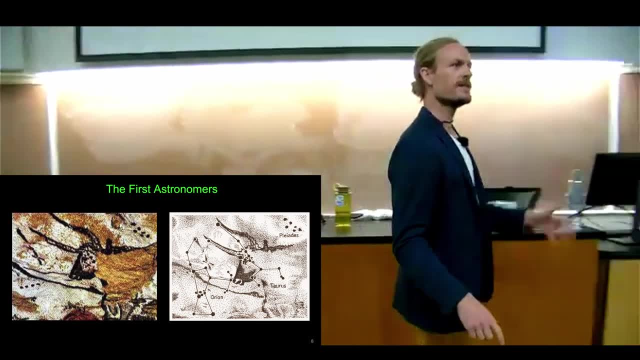 We essentially live in a Greco-Roman society. today. Our laws are largely written in Latin, which is the Roman language. If you go and look at any of the state buildings or courthouses, they're using Roman Greek architecture. This is not that different of a place. 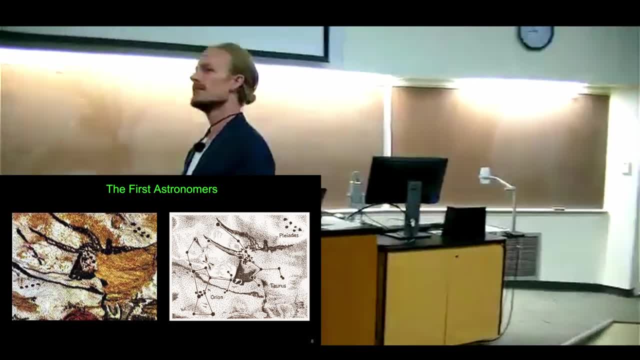 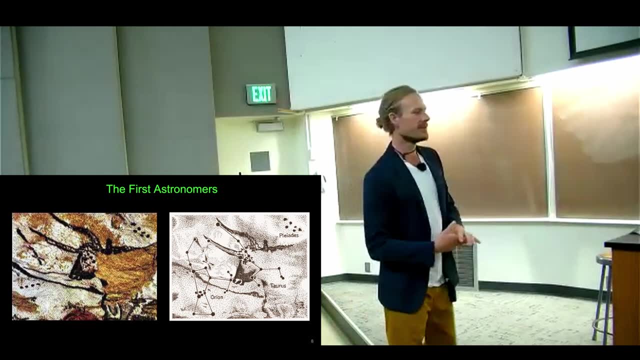 than it was 2000 years ago, And I would say that the Romans and the Greeks inherited their civilization from someone before them, and so on and so forth all the way back. We have records going back to the Sumerians and we're gonna talk about them. 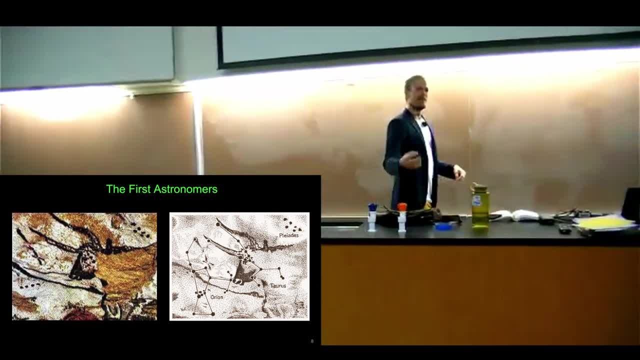 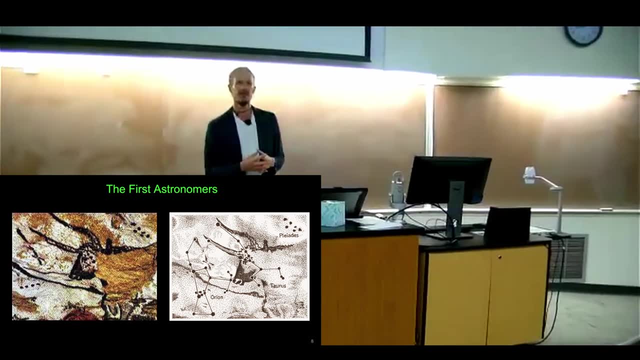 because they're some of our first astronomers. But these were the roots: being able to define what's happening, being able to say what happens tomorrow. These are somewhat magical abilities to the normal farmer who's coming into town to listen to one of these stories. 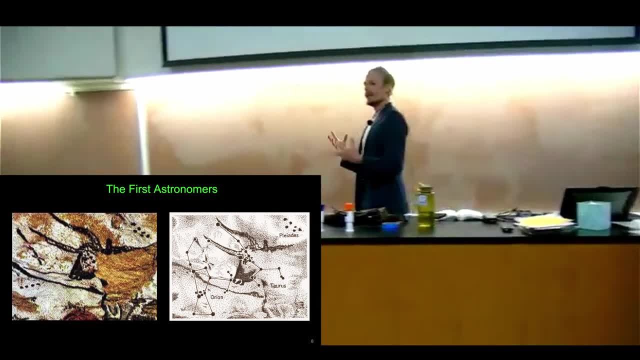 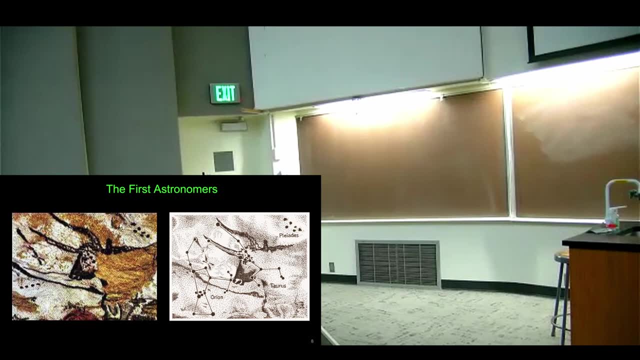 You know, maybe the farmer has inherited some stories from his parents. but to go to a place where there's someone who's cataloging all of these, right, This is essentially. oh, it's not there anymore. Last slide was essentially a catalog of this event. 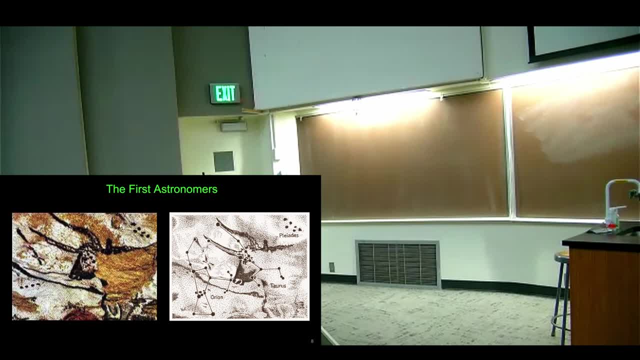 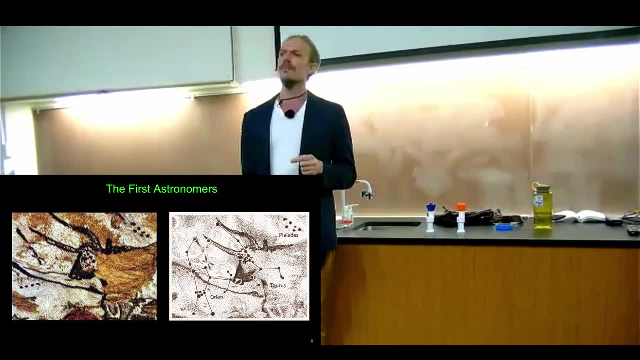 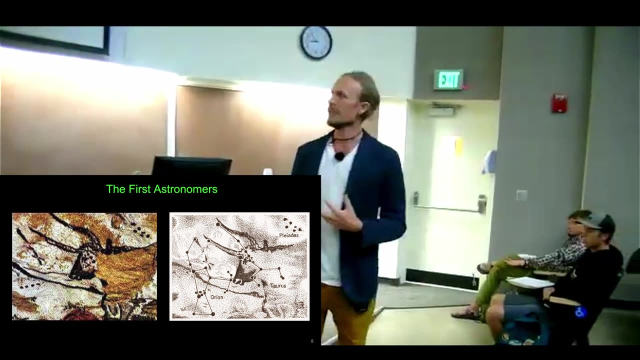 that happened at a particular time. Someone's keeping track of it. In fact, the civilization has at that point gotten advanced enough that someone is able to take their time out of their busy life to stop hunting, to stop planting and to stare at the stars and make catalogs of it. 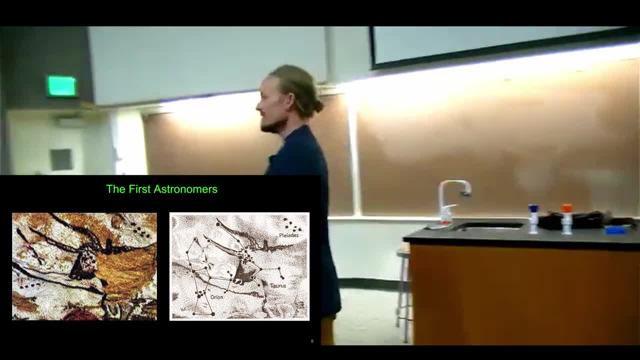 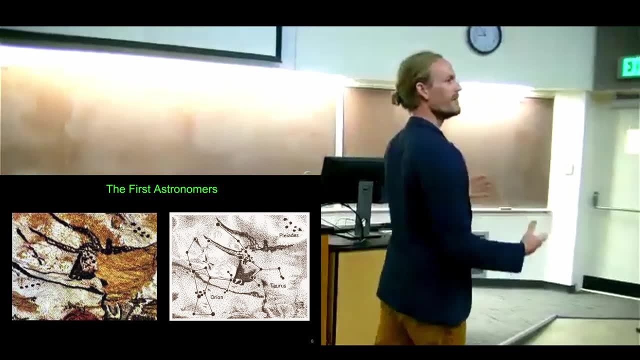 and try to make models of what's happening. So the civilization has evolved with 30,000 years ago. The civilization is already to the point where they're paying for somebody to sit around and think. And that's really crazy because in our civilization today, 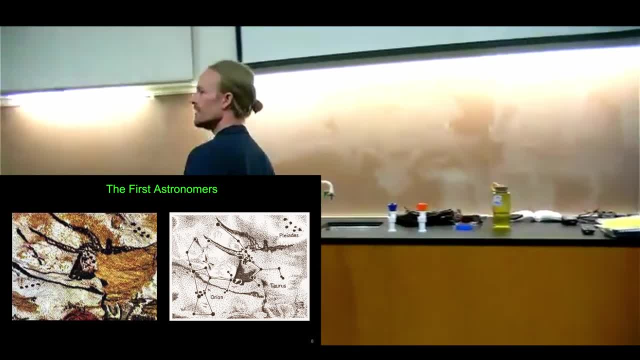 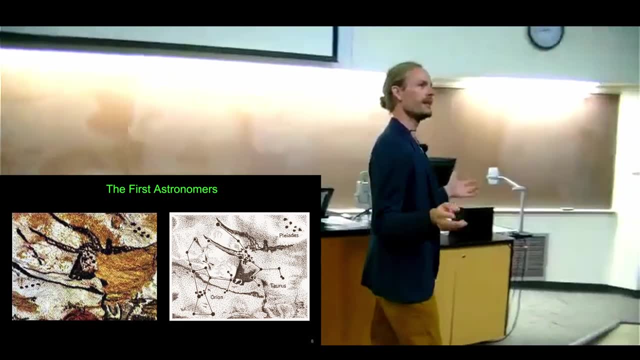 pretty much everyone is paid to sit around and think: right, I assume that's why you all decided to go to college. right, You decided, right. You're like. I don't know How many of you have worked back-breaking jobs growing up. 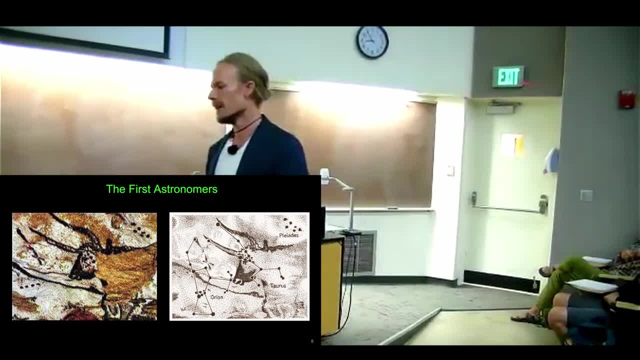 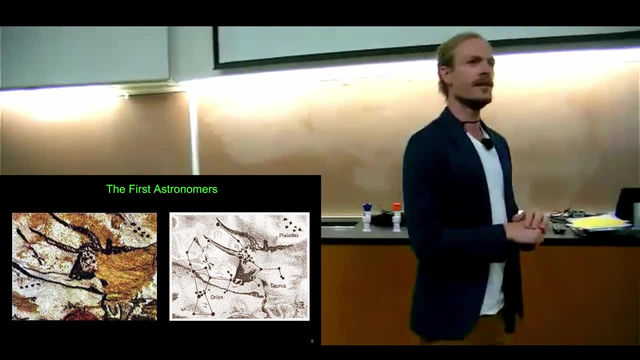 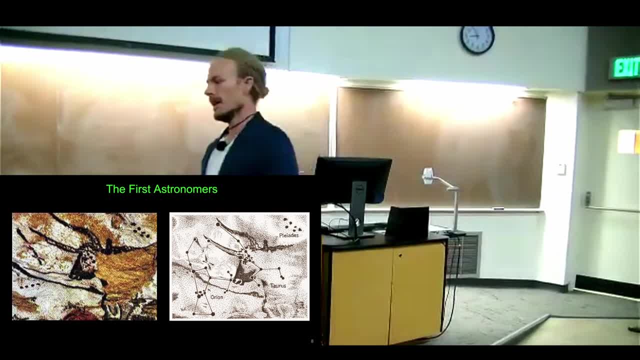 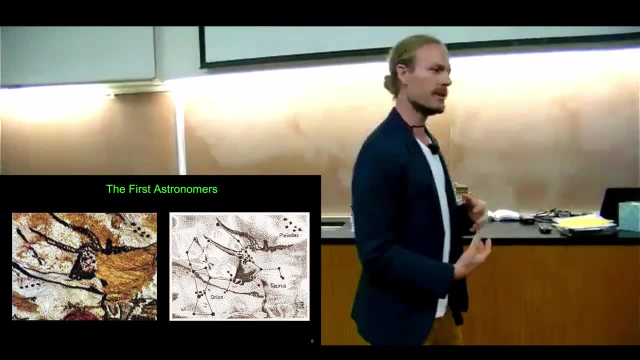 It was the most brutal job of my entire life, for sure, Both of those right, And so the ability to transcend beyond working in the fields and be able to take on intellectual work is a really interesting specialization feature of society, and we see that increasingly more. 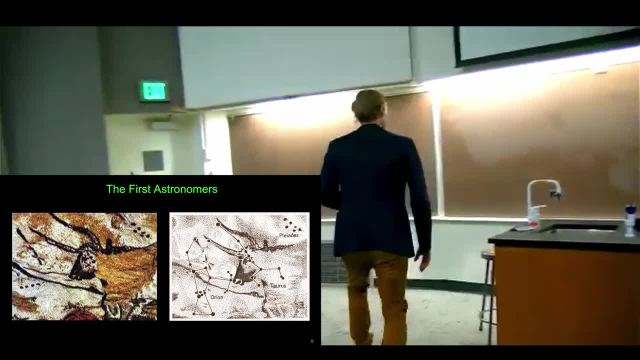 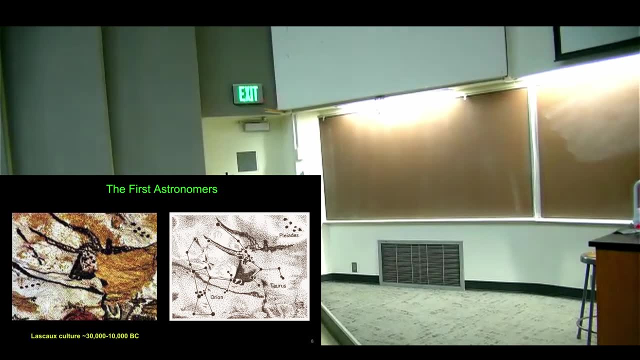 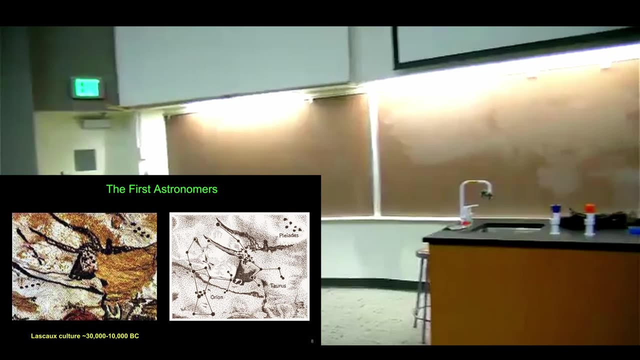 But I think that it started all the way back here with the astronomers, and that's not insignificant. That sets the stage for where everything's headed. So this cave again. the dating's a little rough, but the fact is that dating is a really tricky thing actually. 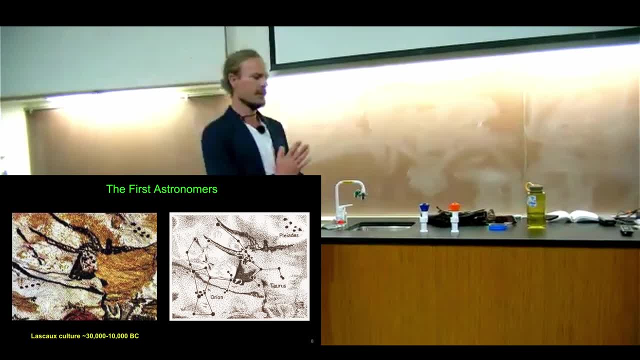 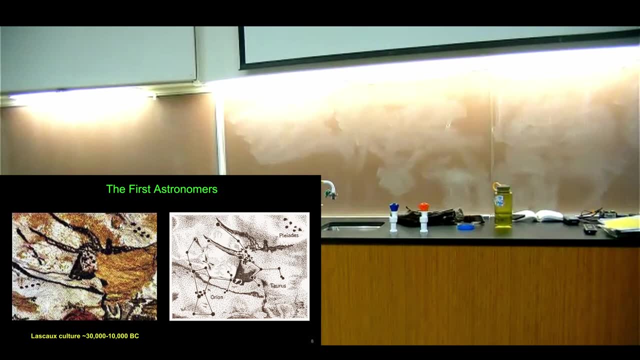 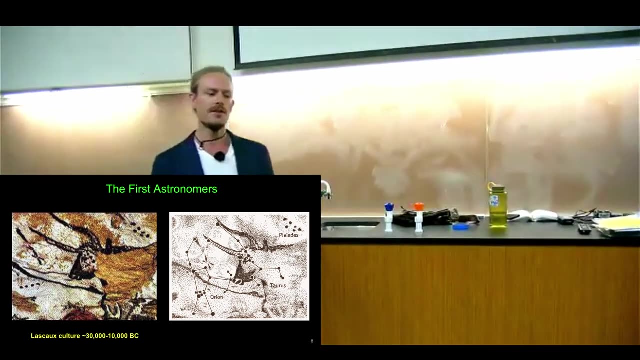 when it comes down, And we'll be talking about this a bunch as we go forward. Dating something is very tricky. You have basically two ways of dating something. You can look at where it shows up in the sediment, okay, Which means that it had to have been either preserved- 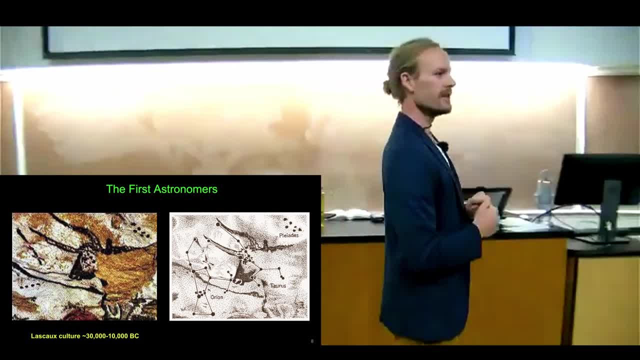 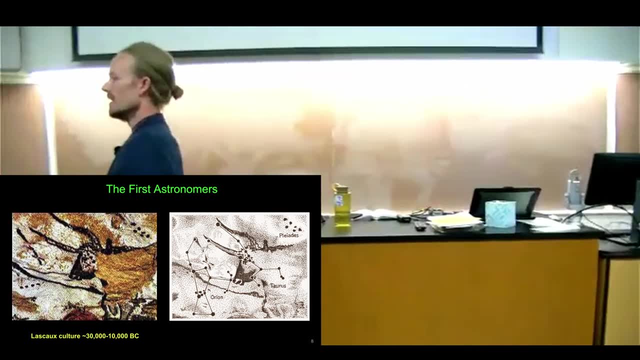 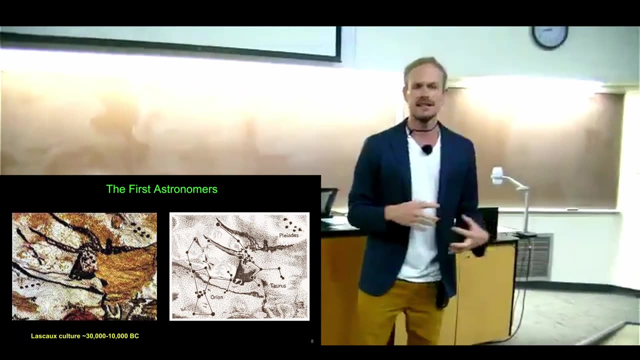 in some perfectly ideal cataclysmic situations. like you know, Something was cast away that had a great amount of information in it. It was covered in a very pH-neutral type of very non-acidic, non-basic mud. It was preserved in this beautiful way, right. 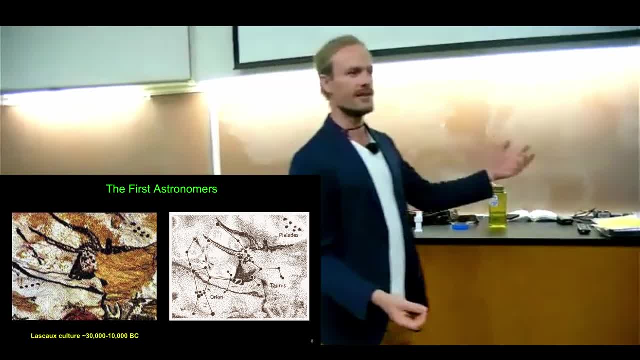 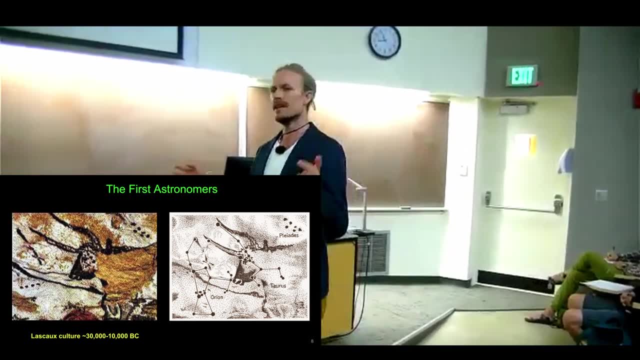 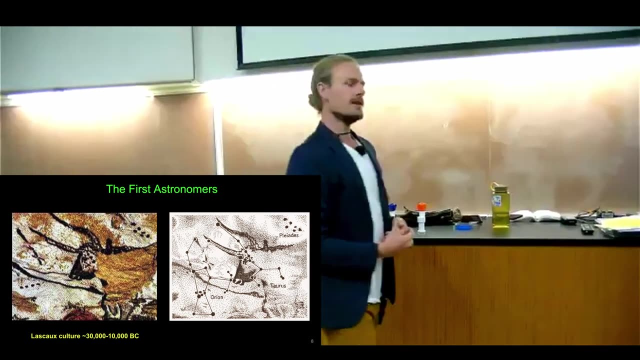 And then we have layers of it. But these records, especially the fossil records too- you hear about fossils all the time- The fossil record is completely absent of massive chunks. There's hundreds of thousands, sometimes millions of years. In some cases there's a billion years missing from the fossil record. okay, 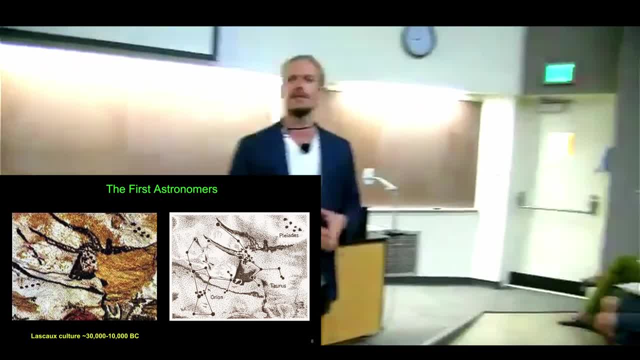 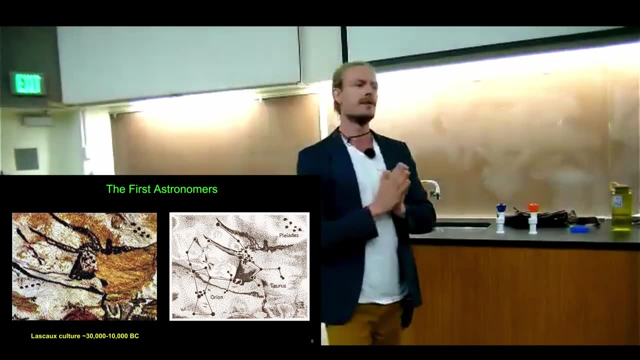 We don't have just this nice continuous story that we can read, And that's why dates are changing and that's why we have such a ridiculously wide range here. Oh, there's also radiometric dating, which does you very little good if A you don't. 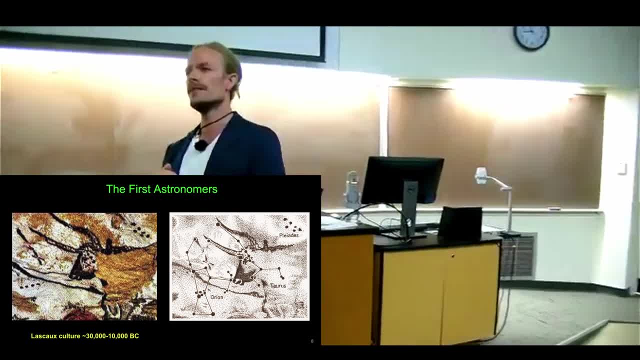 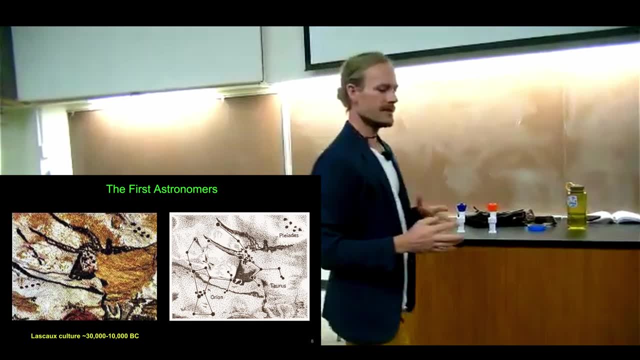 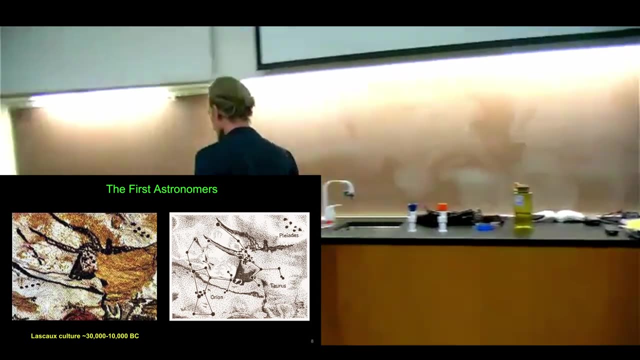 have a particular type of inclusion, that's radioactive, that will allow you to do that dating, or you don't have carbon material, And so the dating as we go through this Is tenuous and it will be changing as things unfold. You know, I think it's a good point right now to mention that as early as, let's say. 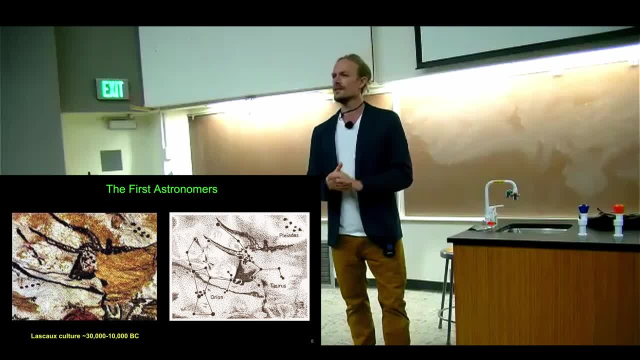 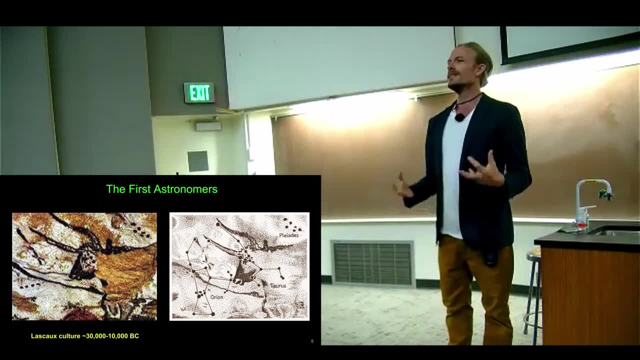 the early 1900s say, like the 1920s, people thought that the Milky Way which we saw above Crater Lake at the beginning of the lecture, that the Milky Way was the entire extent of the universe. That was it. 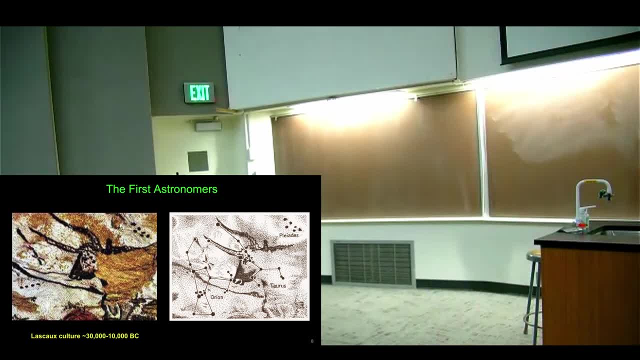 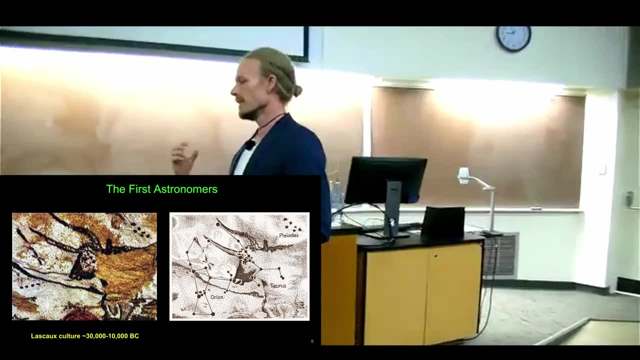 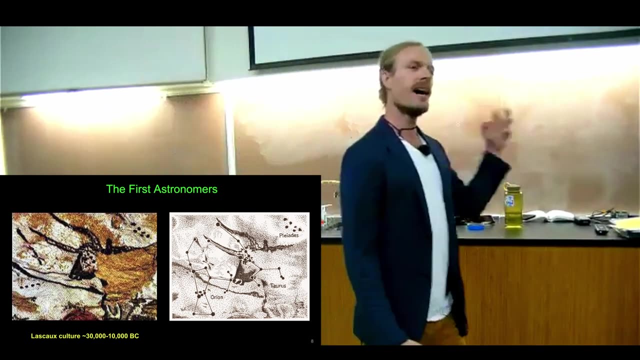 They believed this. They had powerful telescopes They had. They couldn't see anything outside of it. and that was the universe. And, in fact, this model for the origin of our universe that the astronomers and cosmologists are pinning their hopes on today was concocted with the understanding that the Milky Way 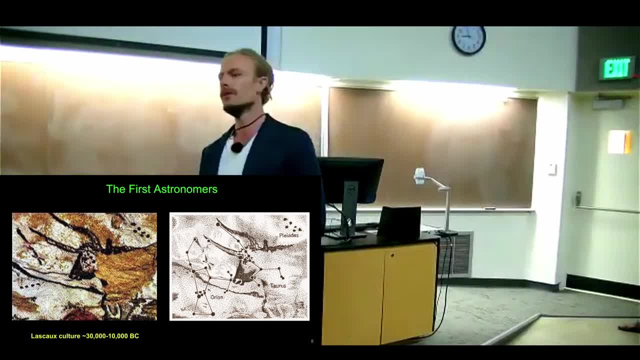 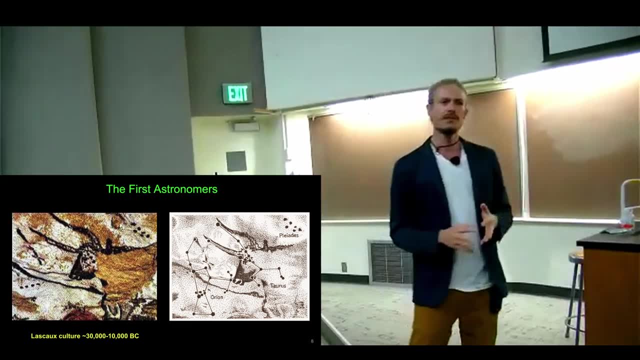 was the only part of the universe, And we know, and we'll see at the end of the lecture- this couldn't be further from the truth. The universe is vast. Of course the Milky Way is vast, But the universe is far more vast. 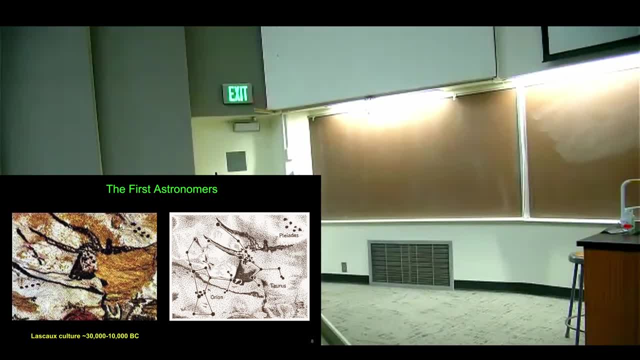 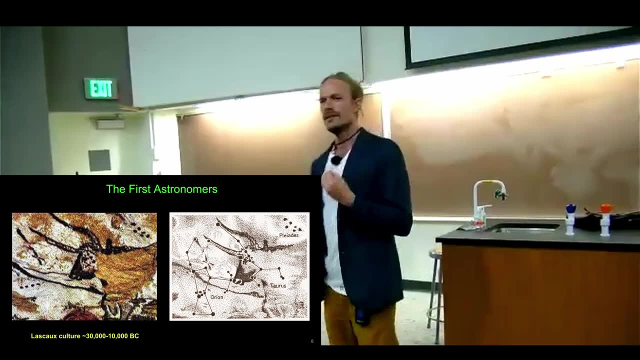 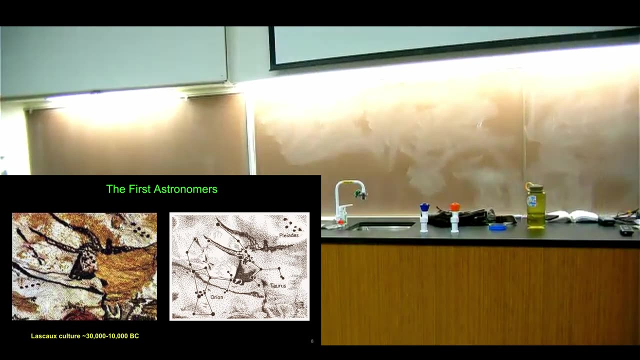 The Milky Way itself, And so that's only a hundred years ago that we thought that the entire universe was inside of this one galaxy. So this is This should give you a sense of how much science changes in such little time. I almost guarantee you that several of the things that are in your textbook will be overturned. 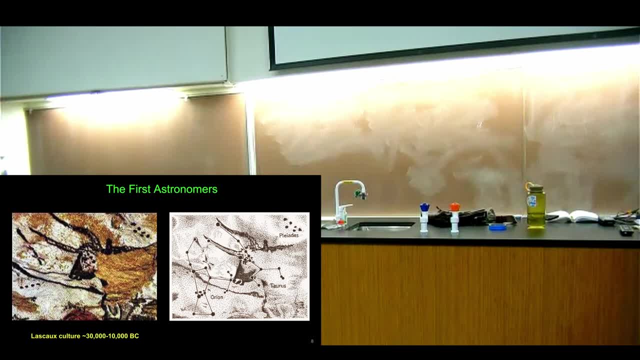 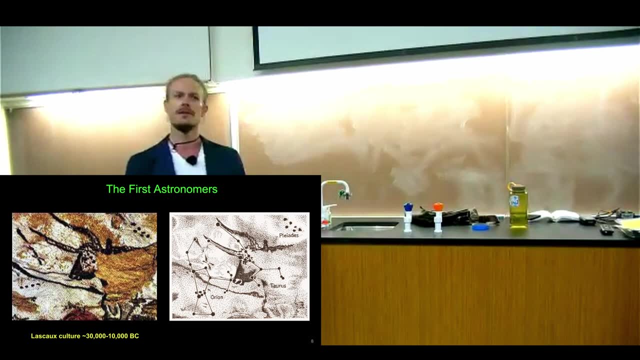 within ten years, And the textbook does a decent job of pointing out a couple of those. I'll probably point out some other ones that will probably change, But I'd love to hear what you guys think too. You know, if you come across something, especially in astrophysics and cosmology, that doesn't 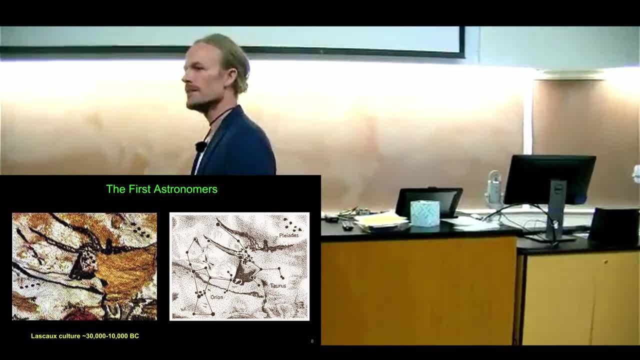 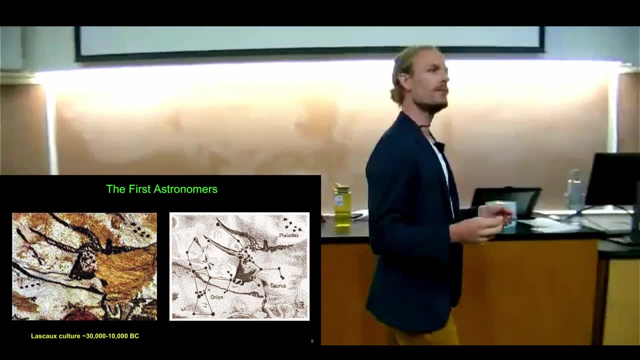 make sense. this doesn't make sense to me. whatever it is. That's because it's probably not right, And I don't mean that it's completely wrong. I mean that it's probably incomplete Or it's an overly complicated way of looking at something. 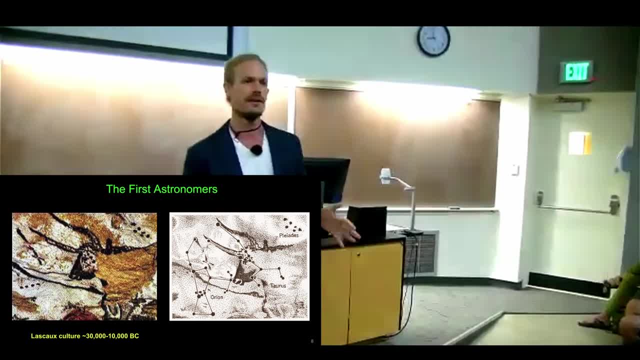 And this has happened multiple times. We'll talk about that with the story of heliocentrism versus geocentrism, which your textbook loves, And I think that it is a very, very complex way of looking at something, And this has happened multiple times. 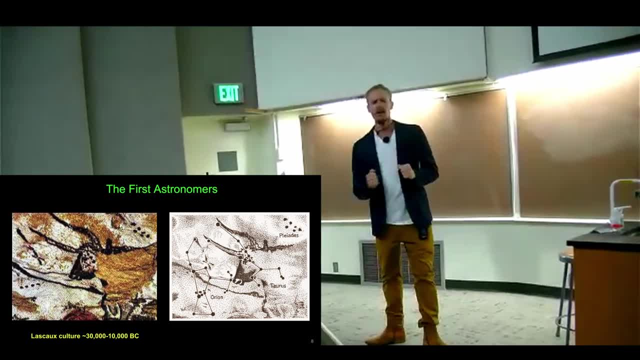 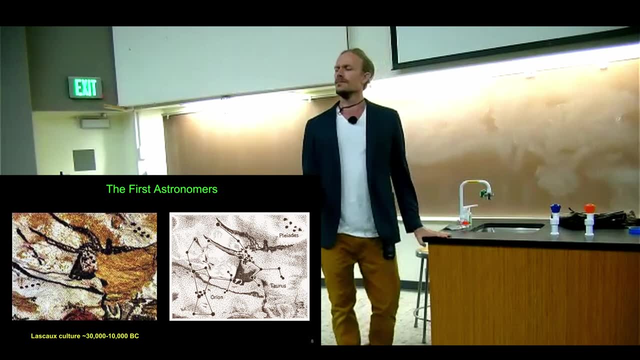 We'll talk about that with the story of heliocentrism versus geocentrism, which your textbook loves, And I think that it is a very, very powerful and meaningful story of how science can change, Because for something like a thousand years we had this model of the solar system that 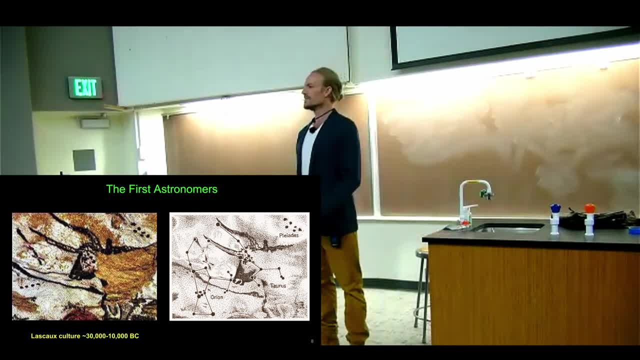 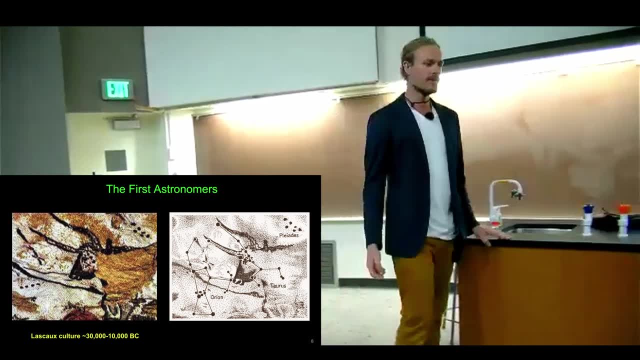 was completely wrong, But what's fascinating about it was that it was also completely right. It worked out mathematically perfectly. So today we have mathematical models that are highly predictive. They tell us exactly how things are going to happen. We can imagine how they're going to happen years from now. 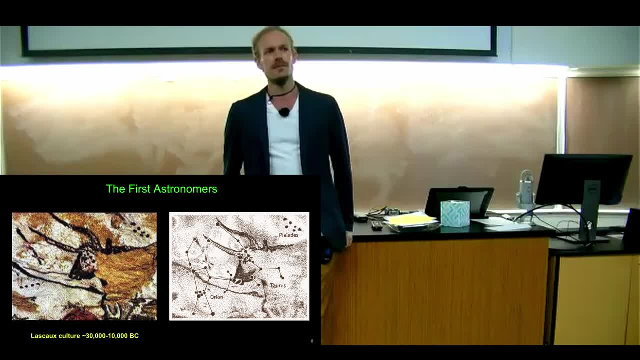 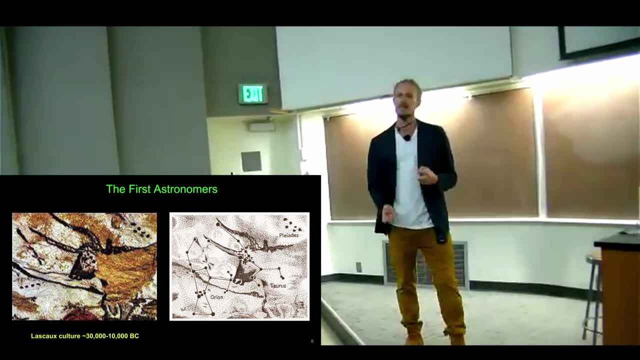 But that doesn't mean that we understand exactly how Those bodies are moving or what those bodies are. just means that we can predict their location. And so there's been this very interesting conflation of prediction and explanation, And I think this has to do with the division of science and technology. 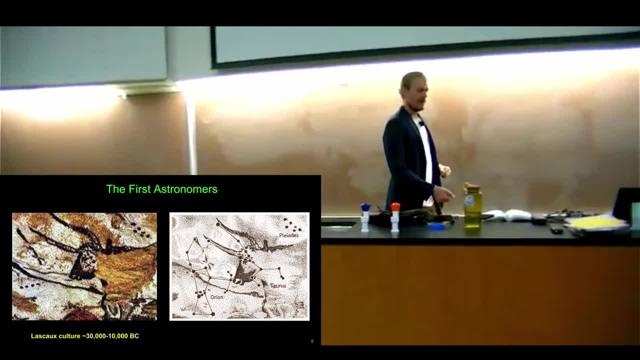 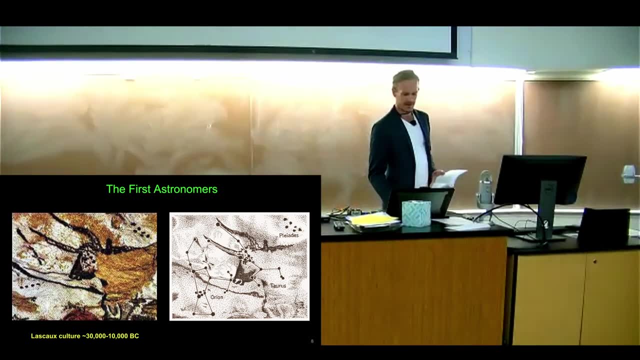 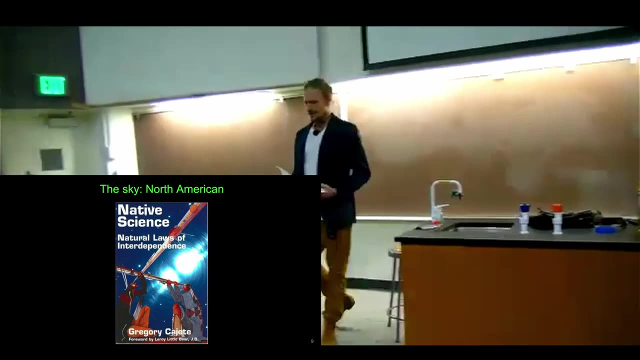 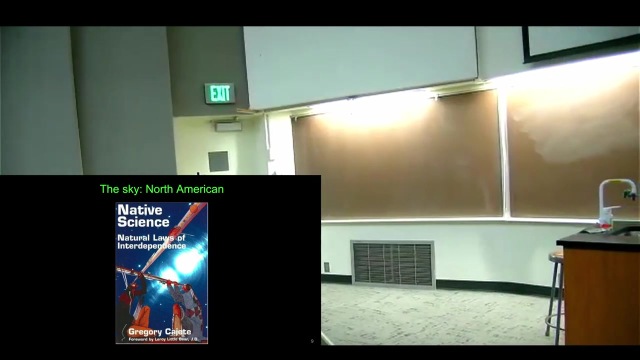 And we'll get into that in a second. There's a, there's a book that I'm going to be using as a companion to this course, which I think is really important. It's called. it's called Native Science, And I think that it's very easy to get sidetracked into the Newtonian mechanical world that. 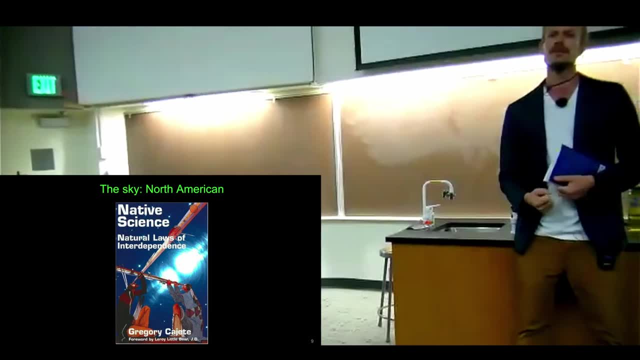 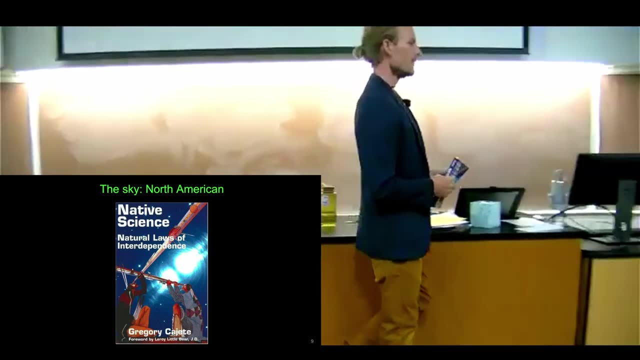 we've impressed upon everything: The one that you grew up with, the one that says how things work, how baseballs travel through the air. you know your high school physics class, your rational, scientific understanding of how genetics work, how heredity works. 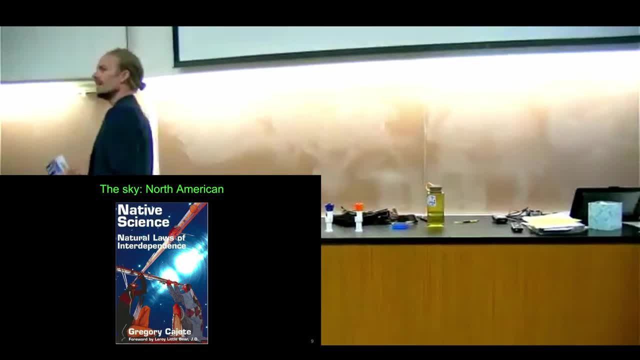 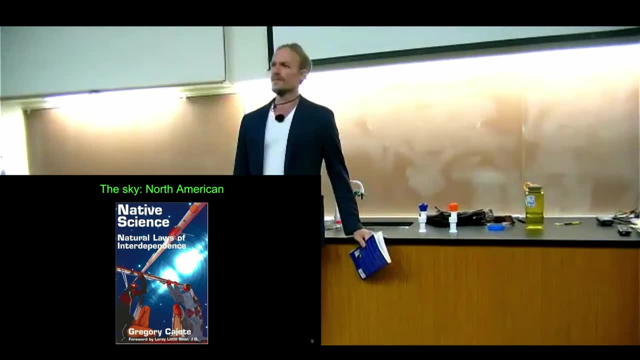 These are, these are. these are perfectly valid. In fact, they're quite useful Again for for producing technology, But they've stripped a lot of the meaning out of these things. right, Like I said, when you're, when you're- an ancient person, what are you concerned with? 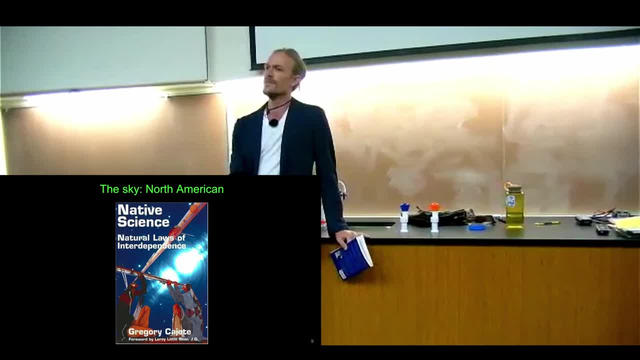 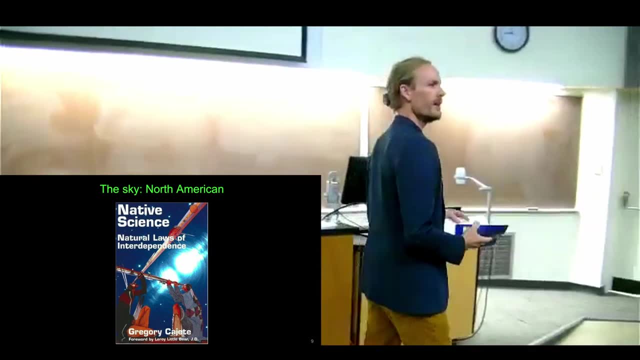 You're concerned with some some very practical matters on Earth in terms of your family life, in terms of your, in terms of your survival, in terms of what to do in order to be around next year, And so I think that, actually, the native people that remain, and some of them are astronomers- 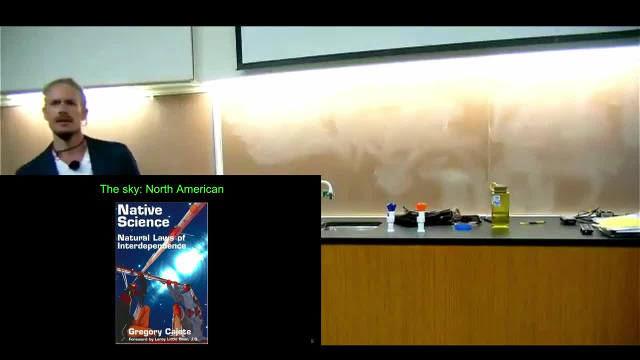 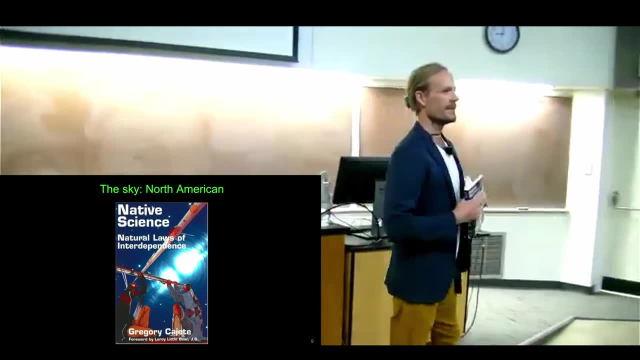 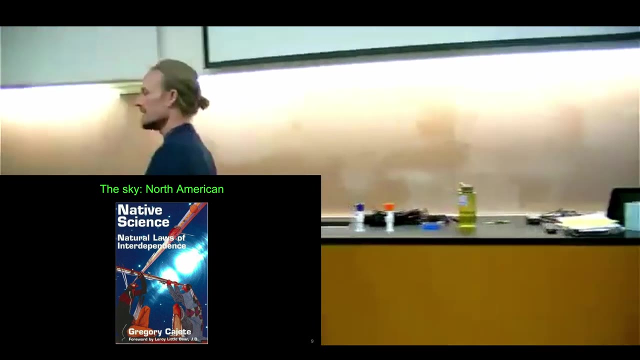 and some of them have Written quite extensively about what they've inherited through their oral traditions. They have somewhat of a better grip on what it all means than we do, perhaps inside of the academy and some sort of hard science. Now if, if you have the opportunity that maybe some of you are outside of the science majors- 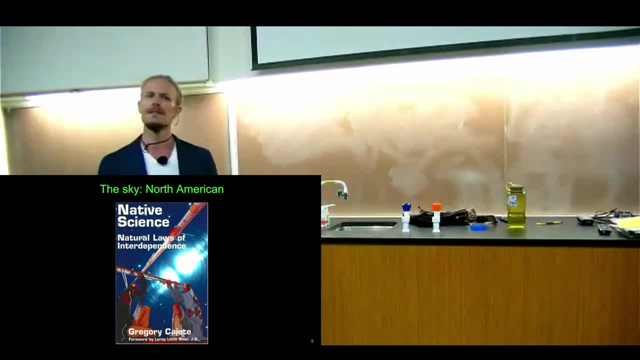 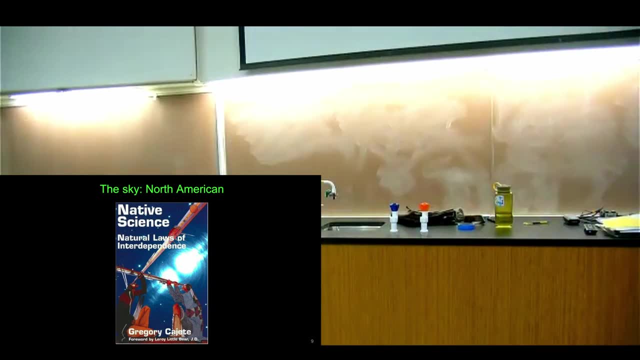 maybe some of you are doing some literature studies, maybe some of you are working in the humanities- I certainly hope so- And you'll bring a lot to this class. You might do some comparative mythology And what you'll find as you go through the mythology is that, again, you start to see. 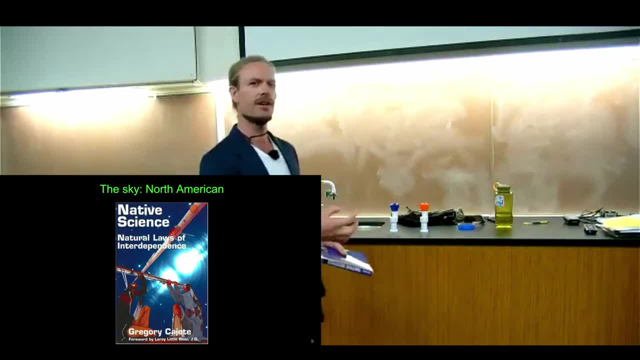 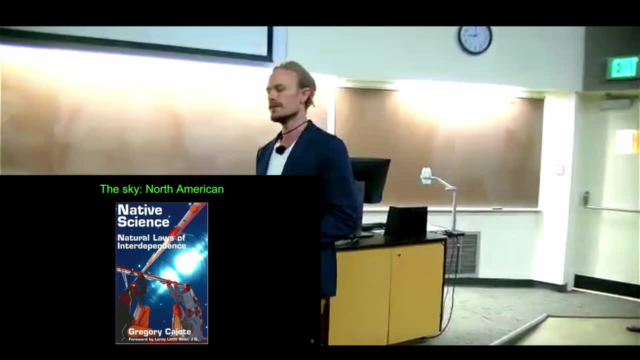 these, these features in each of the myths from different cultures that are saying the same thing. And you might think that's pretty funny that they're saying the same thing. I mean, what a what a strange coincidence. And it's not a coincidence at all. 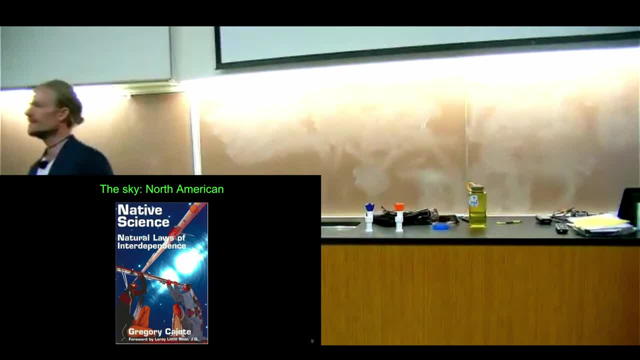 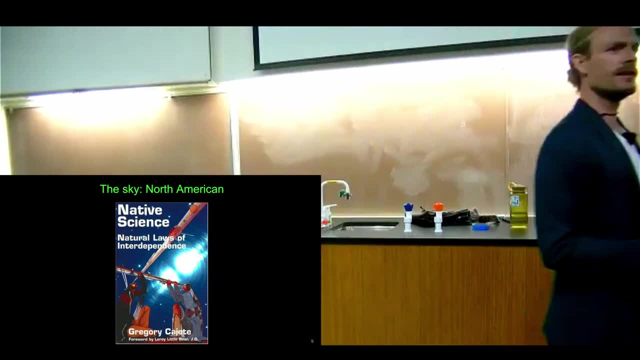 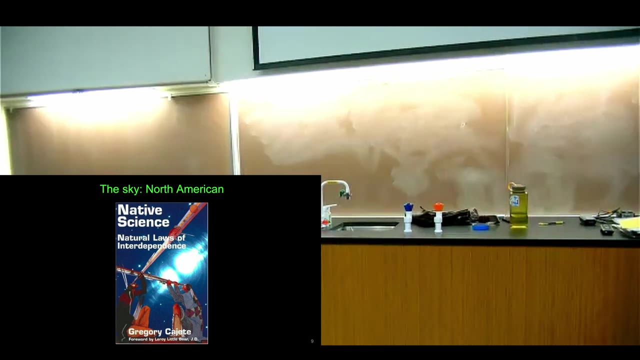 It's that being a human comes along with certain experiences That don't change from culture to culture. There's certain repercussions of your, Of your actions that won't change no matter where you go. You can, we can pick you up, blindfold you and drop you in any culture on Earth. 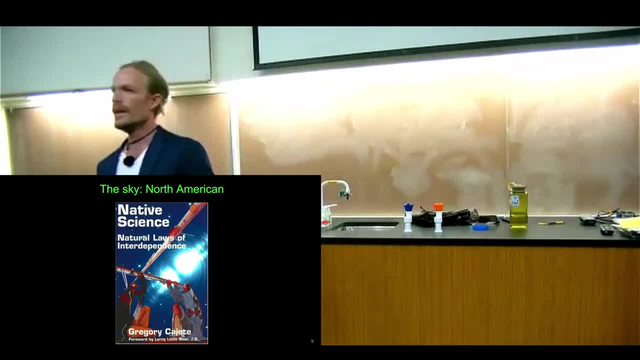 And there's certain things that, if you do them, it's not going to work out for you, And there's certain things that, if you do them, it will work out for you, And that's what a lot of this myth is built on. 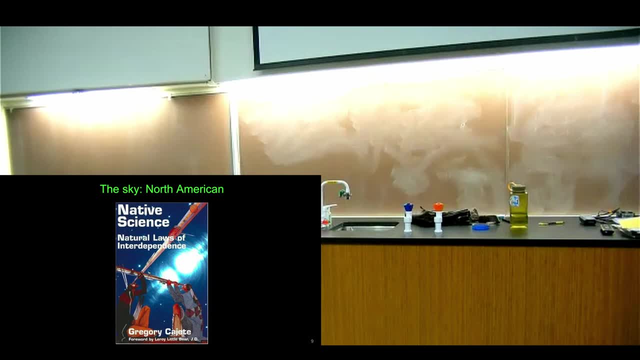 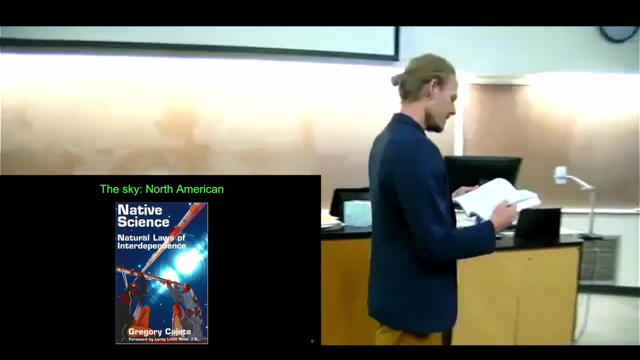 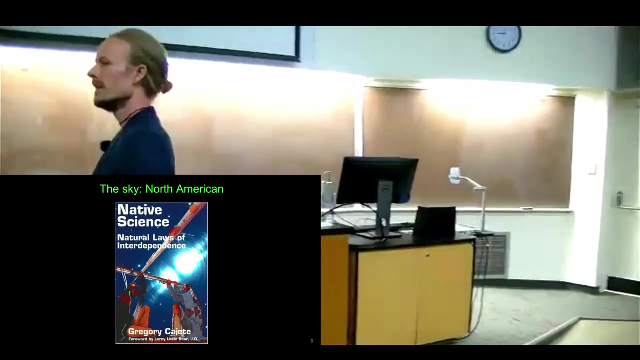 And that's what a lot of the cosmology and astronomy from- excuse me, from the ancient times was built on, And I think I'd like to just read you a short passage from this. This is a Navajo tradition And I think I'll just read you a short passage to give you an idea of how differently the 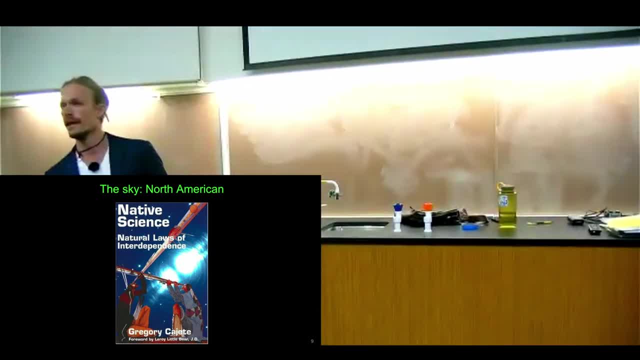 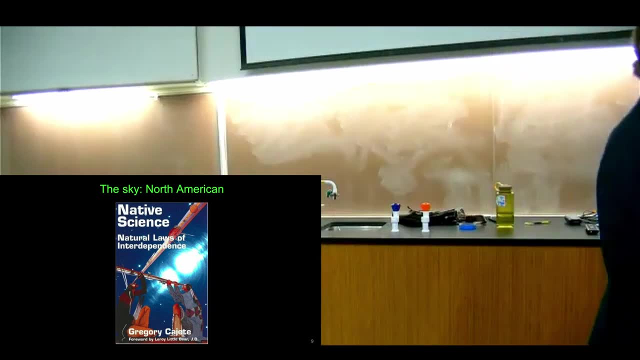 Navajo were looking at the sky from. from how we're looking at it- And I'm going to assume you have some basic background- that the moon is, you know, essentially a sphere, a body of rock that's orbiting the Earth and the Earth is orbiting the sun. 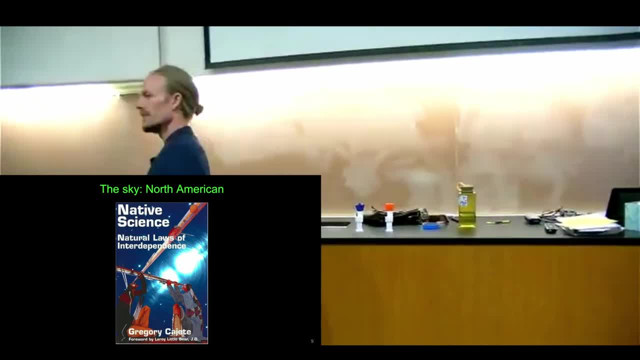 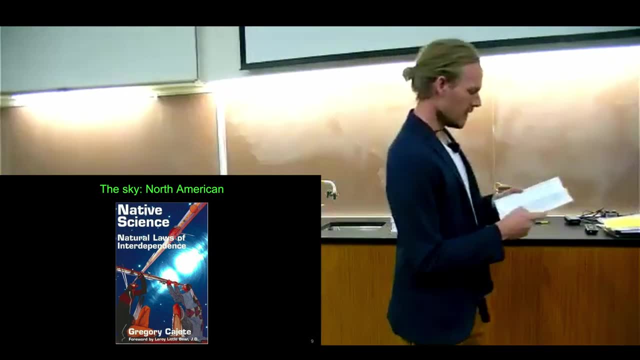 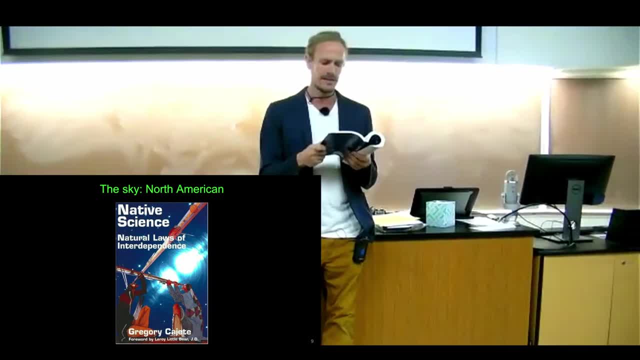 Thank you. The Holy Ones realized that the universe needed light. They also realized that there was no order, direction or sense of time or measurements. The Holy Ones again collaborated to address these needs. First man and First Woman brought the energy of the Sun, Moon and a Crystal Star from. 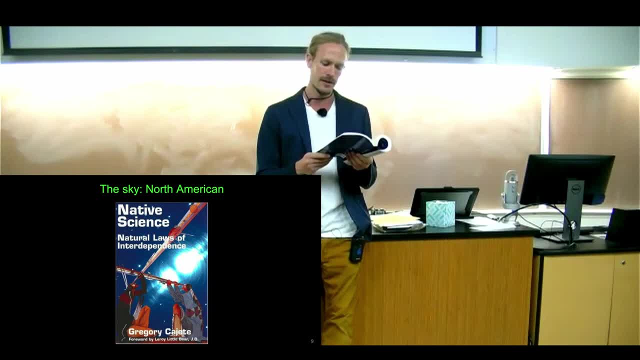 the first world. In the second world, Coyote First Boy and First Girl were created, and together they brought the knowledge of heat and light from the clear crystal to the fourth world. this is our world, all of which was eventually used to produce the sun. 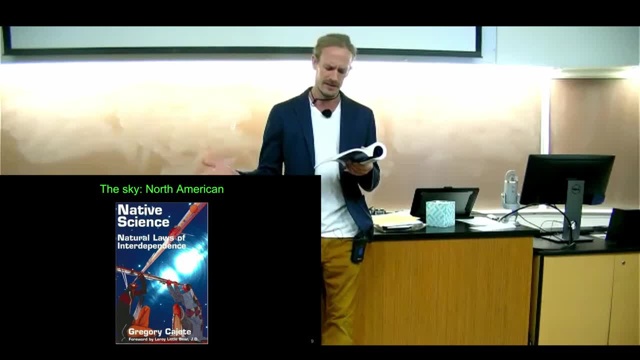 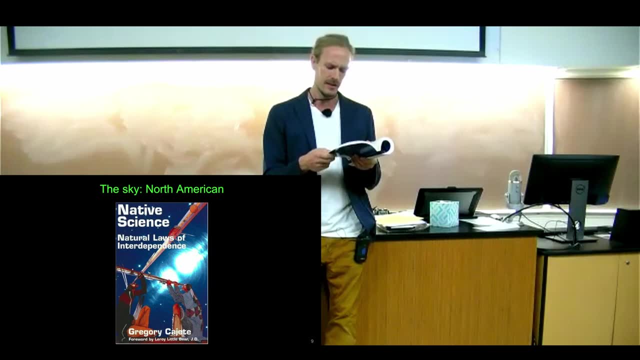 The Holy Ones decided that the sun, considered to have male characteristics, would provide order to the days and seasons, and the seasons are recognized by the location of the sunrise. Referred to as the day traveler, the sun is used to determine time in a general sense. 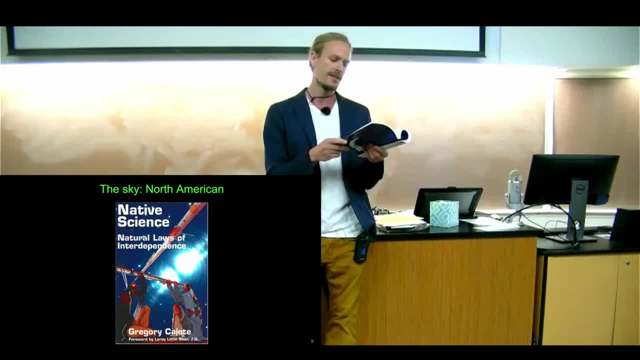 as well as to determine the cardinal directions. The equinoxes and solstices are considered sacred times of year, the end of the sun's journey, making its passage of time and seasons. Ceremonies are held to ensure that the actions of the people and the earth are in harmony. Alright, this is really important. These people believed that if they did not honor these regular occurrences, that they might cease to become regular and that would be cataclysmic. right, Everyone's going to starve to death if they stop being predictable. 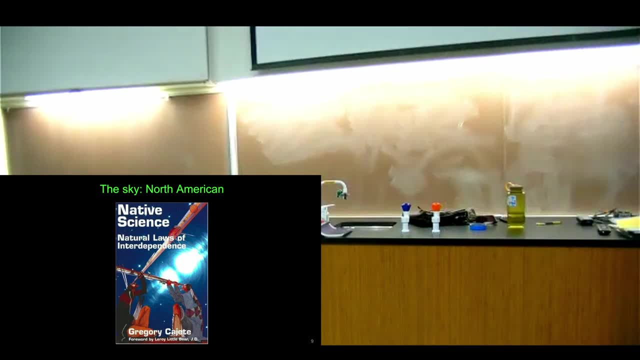 In fact, the only thing we have in the whole world at this point is that this is predictable. in terms of understanding, We don't understand from an atomistic standpoint what this rock is made of, but we do understand that the sky does the same thing every year. 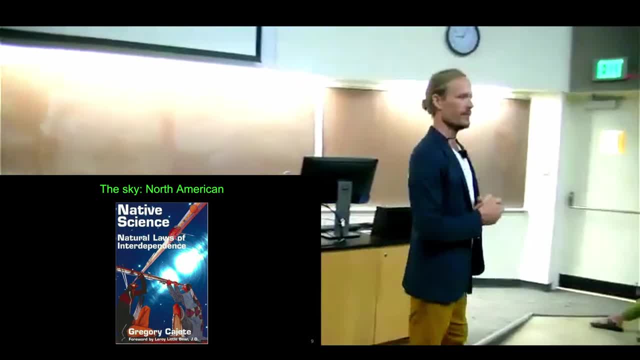 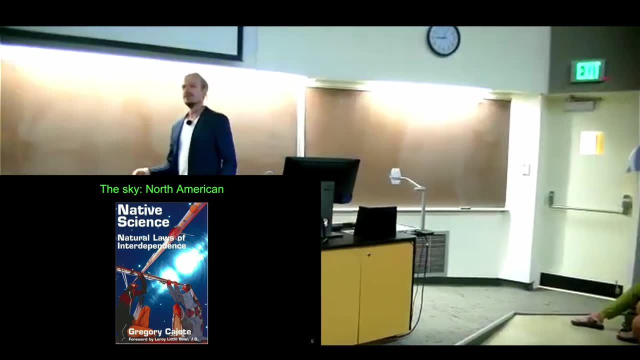 and we better appease whoever is keeping it that way. So this is a perfectly valid way of looking at the world and I think, as we go through each one of these chapters in this book, it's going to be important to go back. 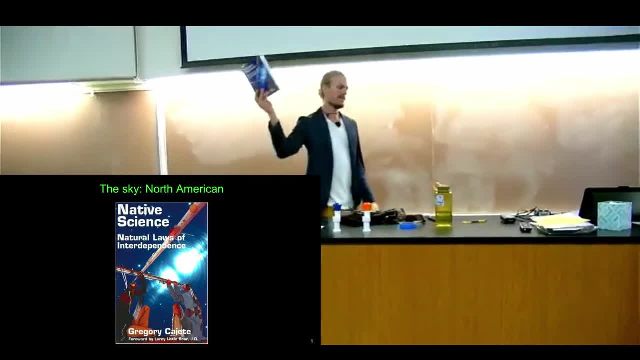 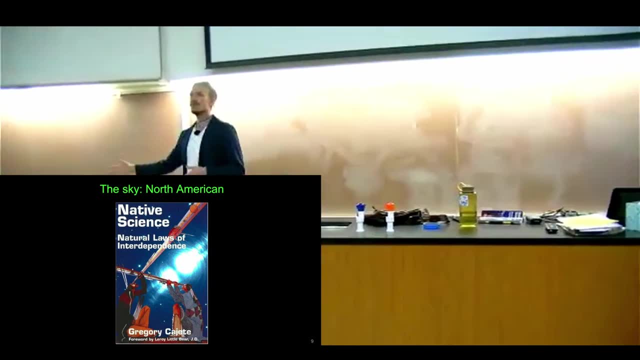 I'm choosing. This is obviously about. This is about Native American perspectives. I think that's perhaps most relevant. since we're here in America, We should perhaps listen to the oldest people that are in America as well, as you know what's printed in our textbook. 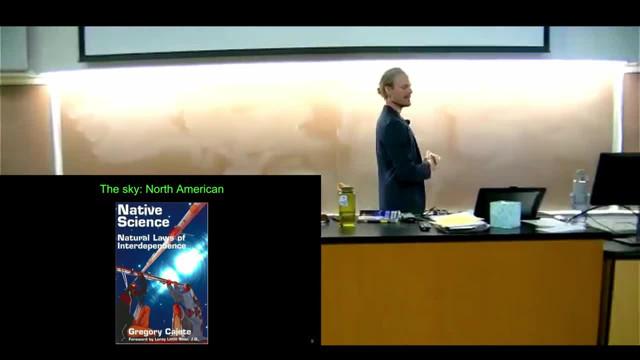 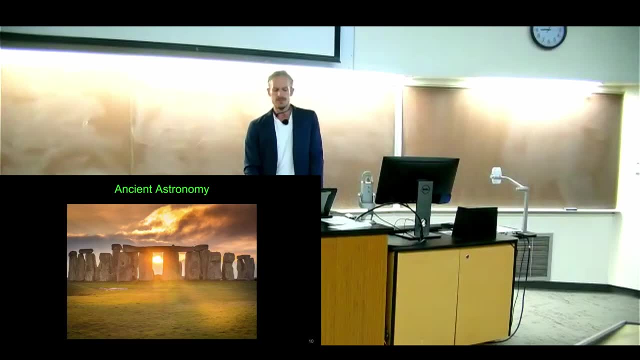 Because there's a lot of wisdom to be gained there. These aren't just silly stories. They actually can teach us a bit about the world. So all around the world, people started to make note of these events. Yes, Stonehenge. 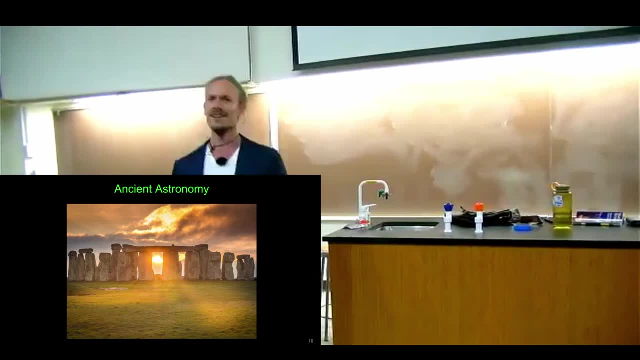 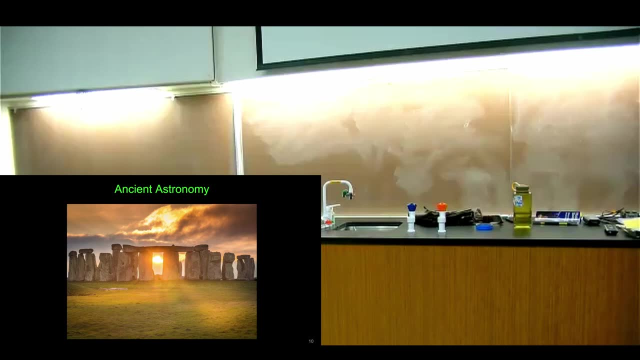 Anybody ever been there? No, All right, Go check it out. if you get a chance, I'm sure you'll have the opportunity at some point. Stonehenge: very quickly people realized that it had the ability to mark the summer solstice. 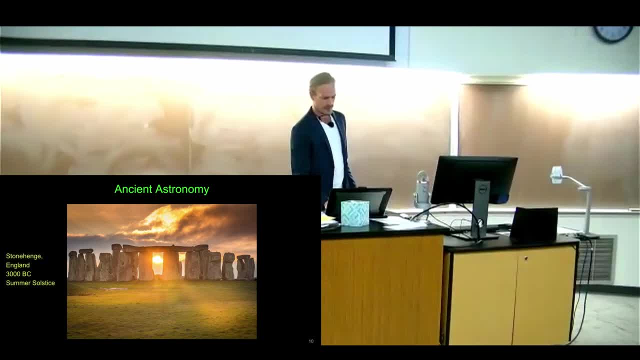 which is, you know, turns out to be extremely important. They built this, let's see, 3000 BC, so about 5000 years ago. They had the ability to move these giant stones into a formation and I don't think that it was a coincidence that they were giant stones, right. 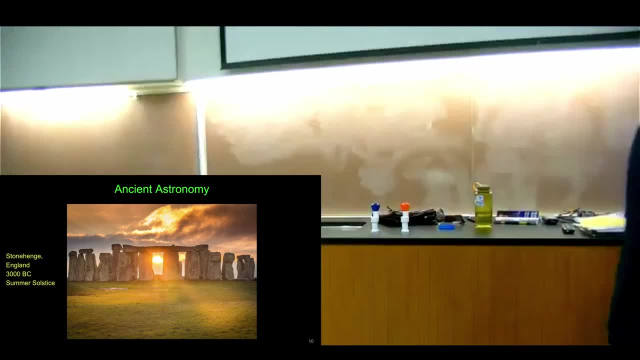 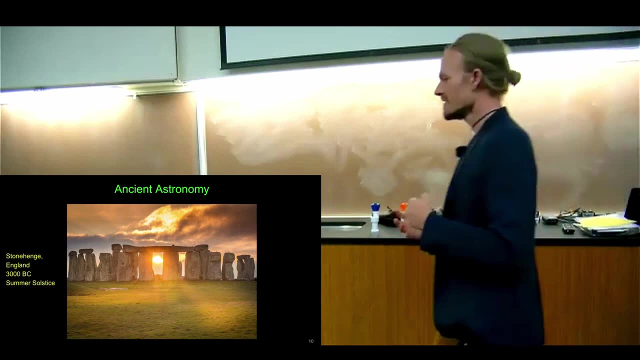 These people believed that their efforts would be in proportion to what they got back. Remember, they're trying to keep the sky moving ultimately, which isn't. it isn't unreasonable, okay. If that sky stops moving, things will go back into the darkness. 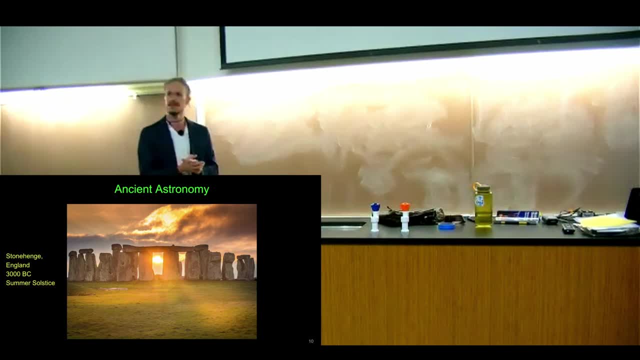 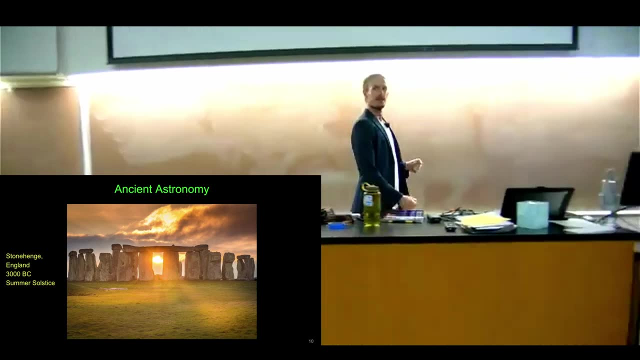 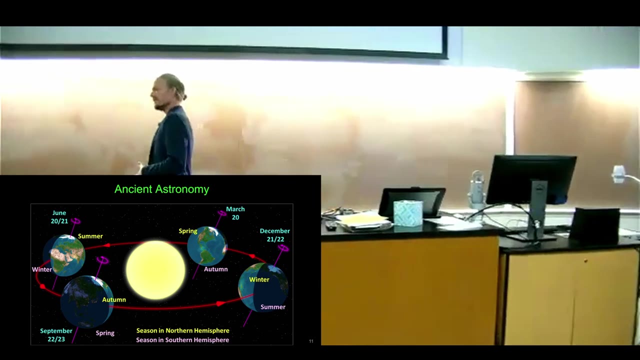 And does anybody know what the summer solstice is exactly? Theodore, It is the longest day in the year. Do you have a sense of why that is? I don't, Okay. so the Earth turns out to be tilted a little bit and as it moves around the Sun, 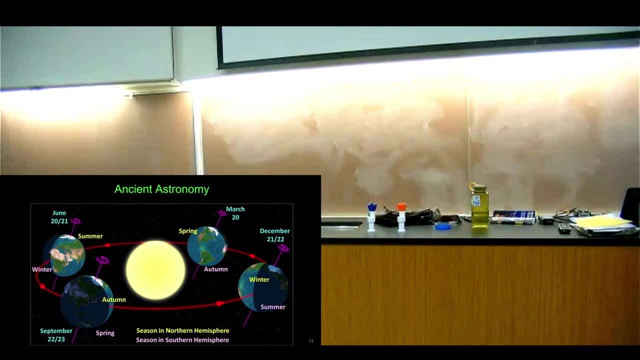 the tilt lets a little bit more of the Northern Hemisphere to be illuminated at one part of the year, and at the other end the Northern Hemisphere gets the least amount of light, And likewise, if you're in the South, you're going to see the opposite. 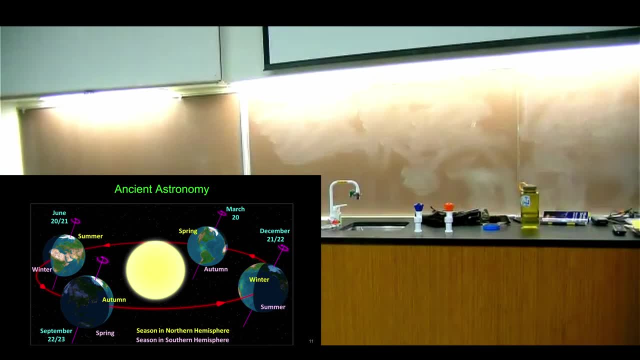 This is why, if it's summer up here, it's winter down there, and vice versa, And so the ancients realized that this was really important and this was predictable, and that when the Sun rose in a particular location, that marked the apex of the year. 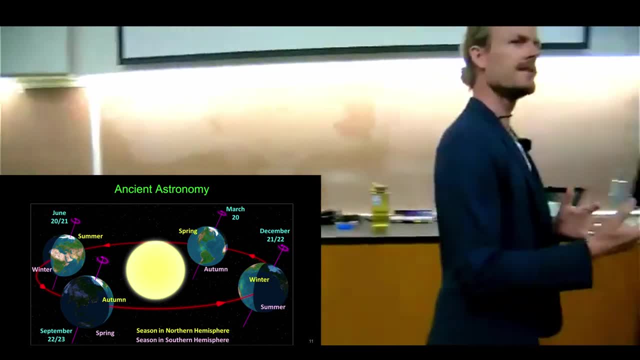 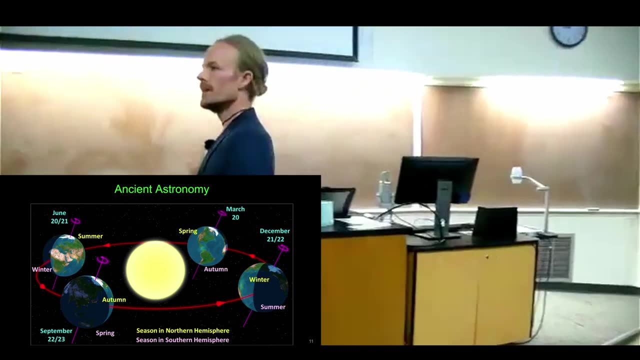 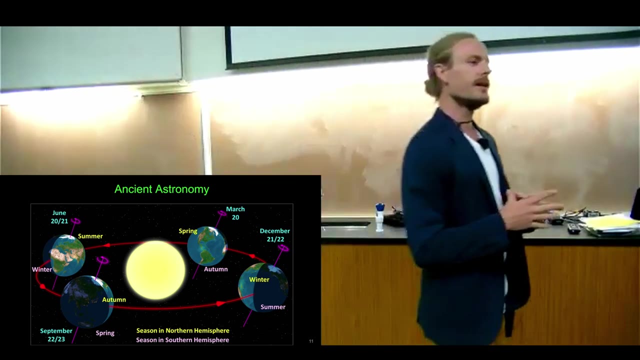 That's when the year was going to begin to turn around. and did they really? did they have this conception? Most likely not. There is some evidence that perhaps the, the Indians, the Vedics in the subcontinent India did have actually a sense. 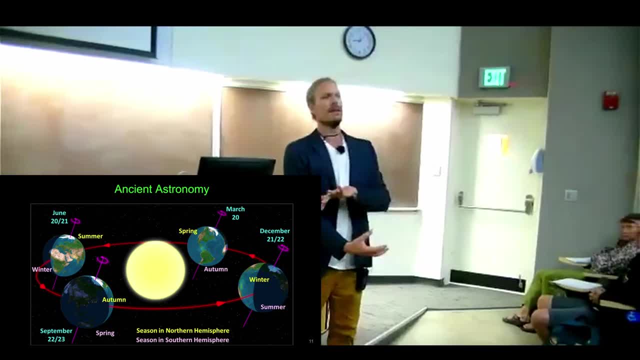 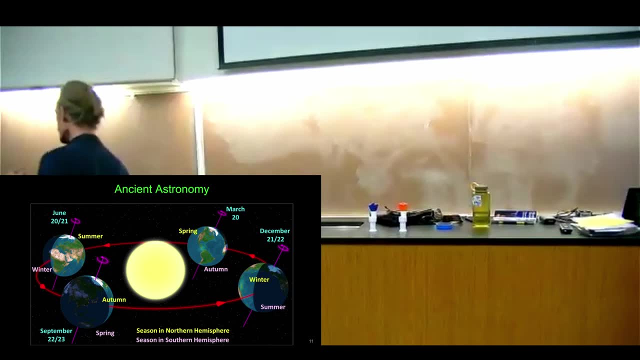 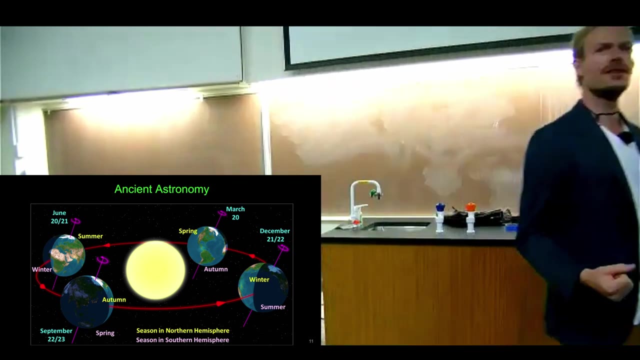 If you look at their gods, you often see the Sun in the center and the planets. There's several pictures of Vishnu that have a Sun like this, And actually the Indian word for the Earth. it means something like round dirt. 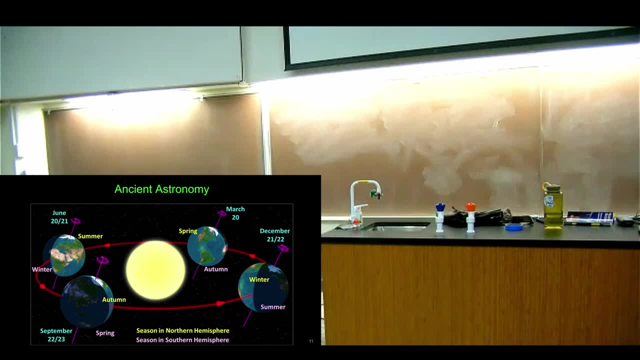 This was from 7,000 BC. These people seemed to have had a sense that they were, that they were standing on something round and that it was moving through the heavens. But most people didn't have that, and that's okay. 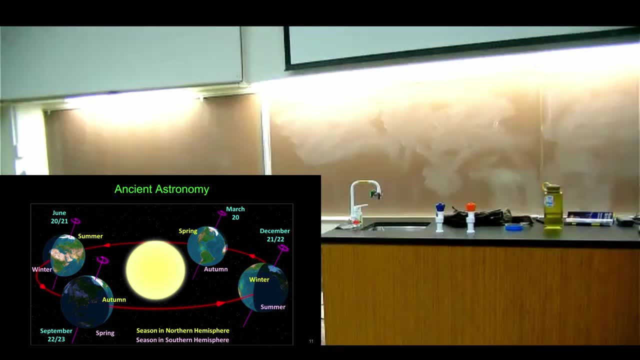 They did know that that Sun was going to be in that exact same place at the same time every year, and they knew that if they built a monument to it, it might stay that way Furthermore, they could begin to time. Let's go back and look real quickly again at Stonehenge. 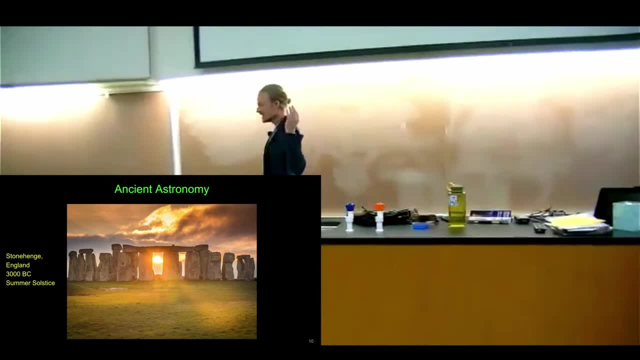 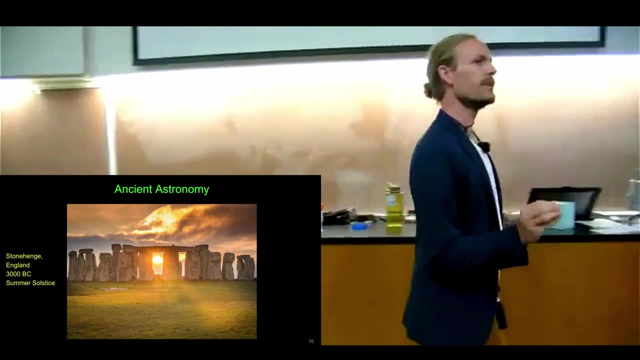 As the Sun moves across the sky, right, It's rising in different, different, different ones of these portals. right You can begin to get. You can begin to get a sense of exactly where you are in the year at that point. 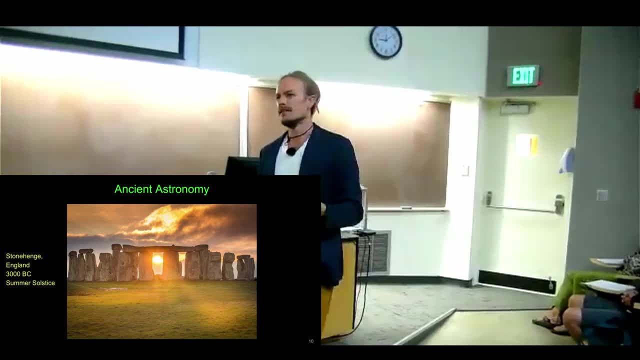 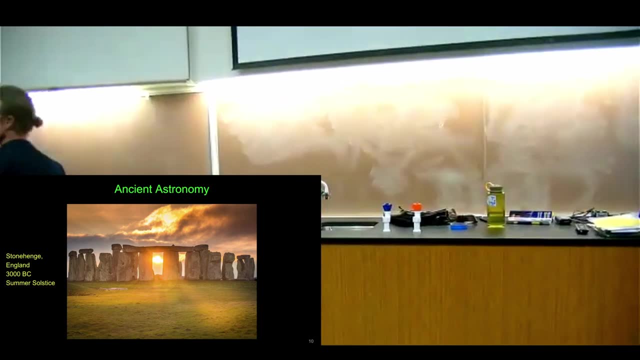 which you know. it's cool to know what day it is and everything, but it's really important to know what day it is if your harvest depends upon it, And I would say that for most of human history we weren't living in civilizations. We were living in very small groups of family And we were, We were just planting. We probably weren't even planting that much, to be perfectly honest with you. We probably tended something like a garden. We did a lot of hunting, We did a lot of gathering. 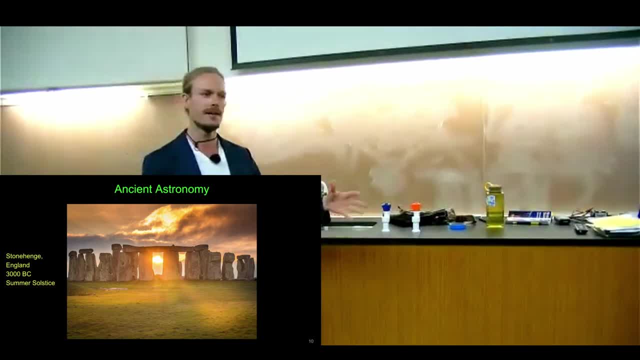 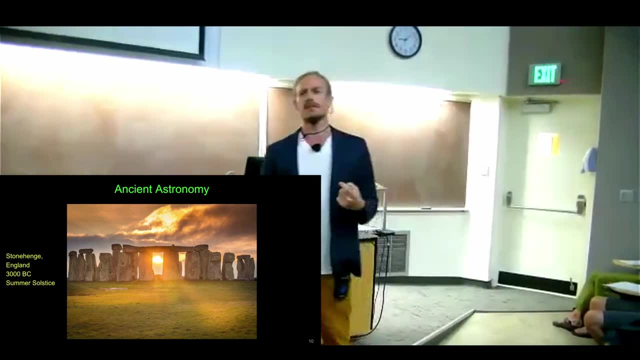 You've heard that before. It sounds so cliché, But really we're out there trying to find food almost all the time, packing it away for the winter. The first features of civilizations, like I said, was that all of a sudden, 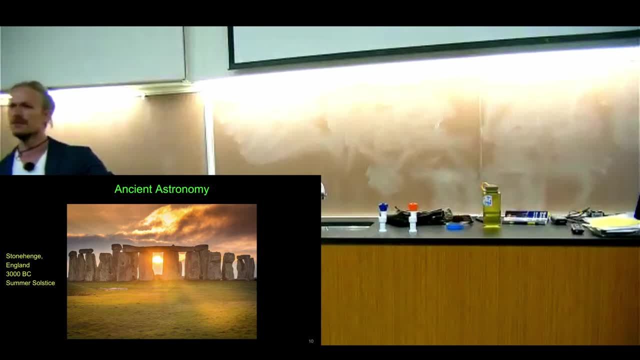 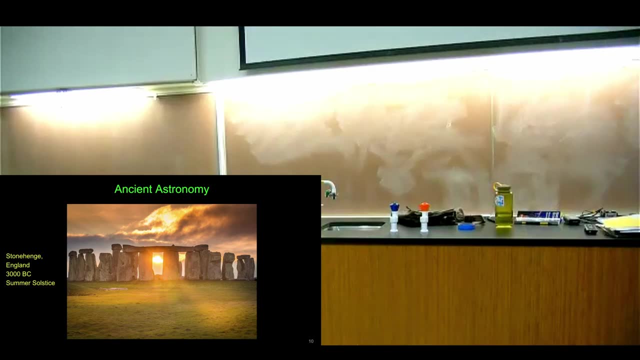 somebody is gathering enough food so that somebody can do something else, And that's really important because that allows the advancement that we have, That allows this auditorium to get built eventually. right, Somebody, This guy, Whoever built this chair over here. 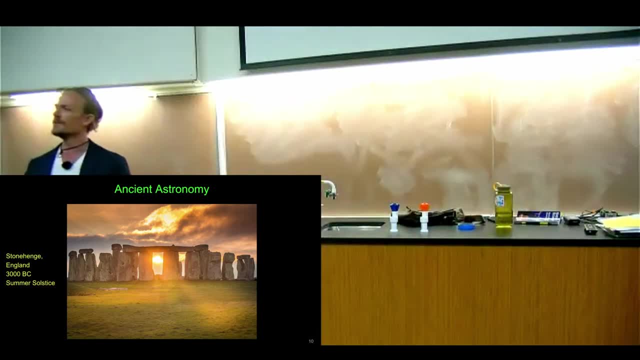 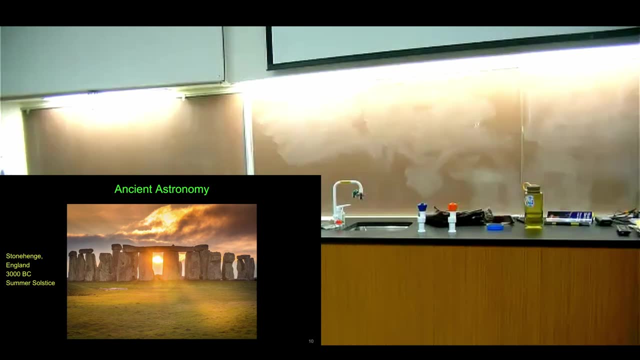 He didn't have to worry about tending his crops in the field. Right, This is really important, actually, You think about it. You don't have to go and hunt your lunch, right? You're going to go somewhere and purchase it. 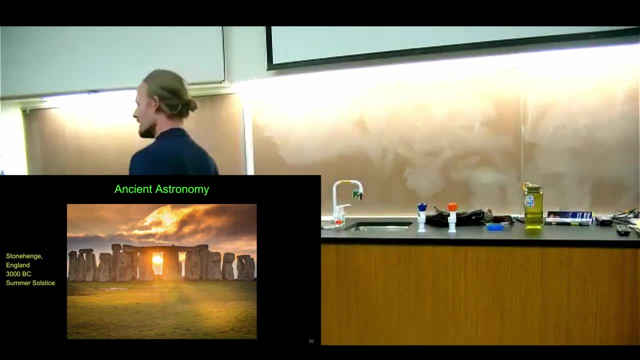 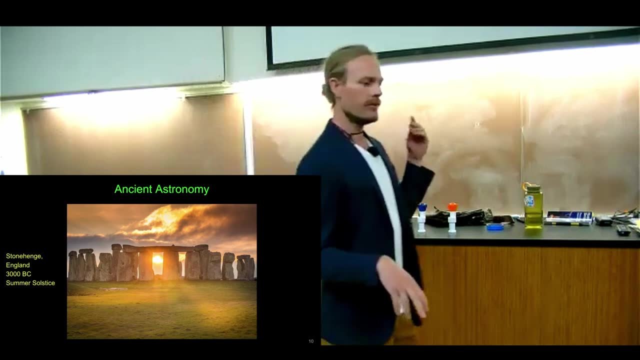 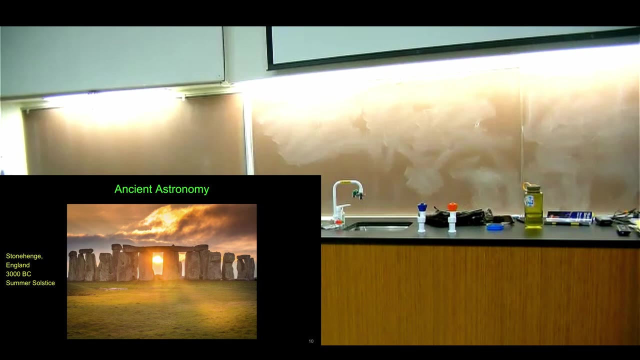 And the ability to keep track of the cycles of the sun allows for that portion of society that's providing the food to be able to do it regularly, predictably and sustainably. If we don't have that ability, If we don't have that ability, we have nothing really right. 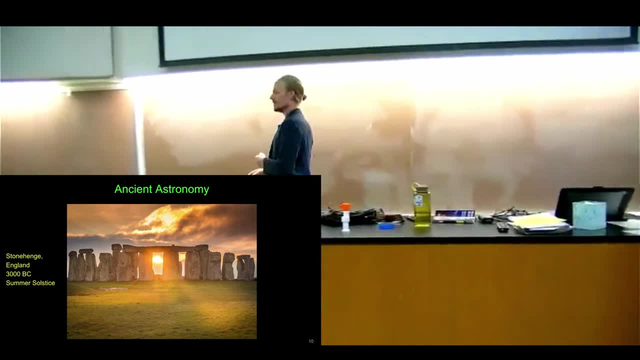 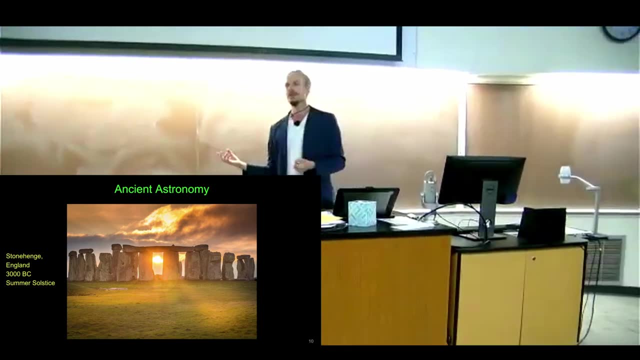 We're back. You're back hunting and gathering all day long. No time for anything. No time for learning how to build chairs, learning how to do anything right: Navigate the seas, Explore the world, Study how things work. I mean science is a privilege, right. 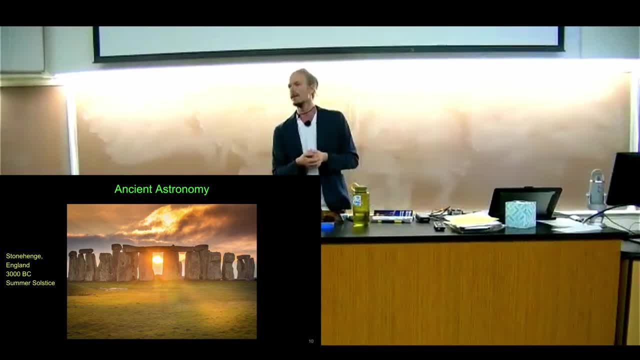 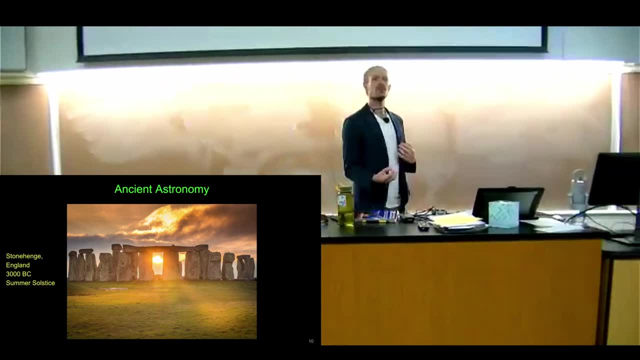 We just get to sit around and think about: how does this stuff work? Quite honestly, a lot of science. It only has meaning in that it's. It's important to know how the world works, because without it it's terrifying And so. 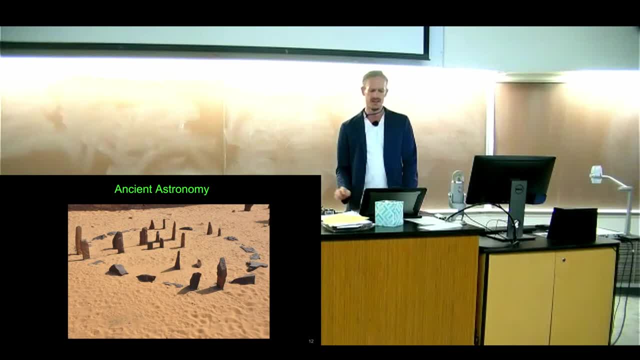 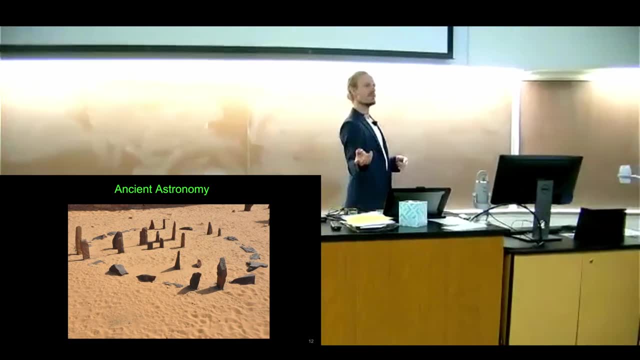 You see this all over the place. This is from South Africa. a very similar arrangement that provided for a calendar for when that sun was going to rise at the solstice every year At some point. Let's see This is Oh sorry. 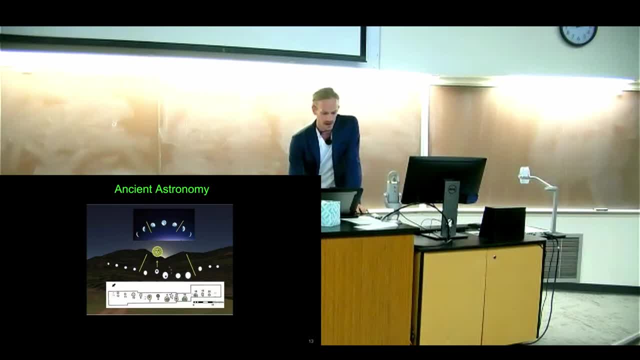 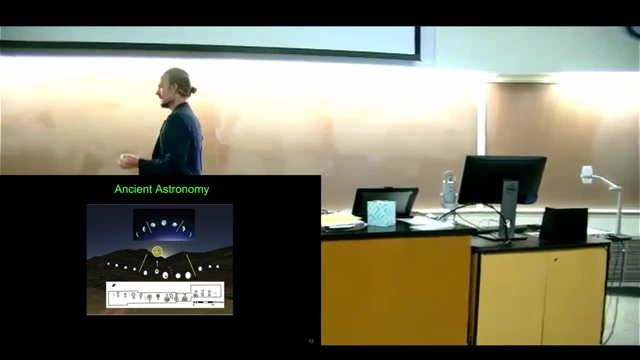 This is from Egypt in 5,000 BC, so about 7,000 years ago. At some point, People began to also try to fit the moon into this. Now the moon's a really tricky, A tricky piece of this puzzle. See, The moon Has a period of something like 29 and a half days And the sun has a period of Yeah, Now, if you try to do the division there, you're going to find out it doesn't fit in quite evenly. 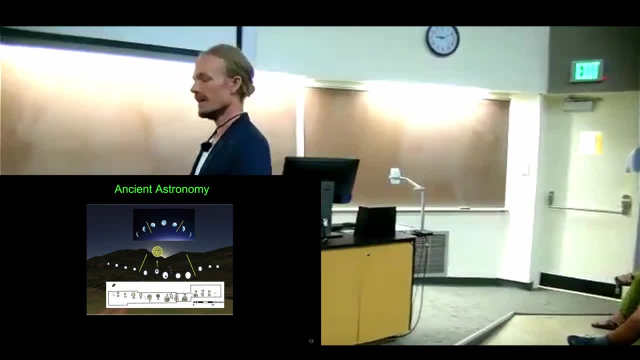 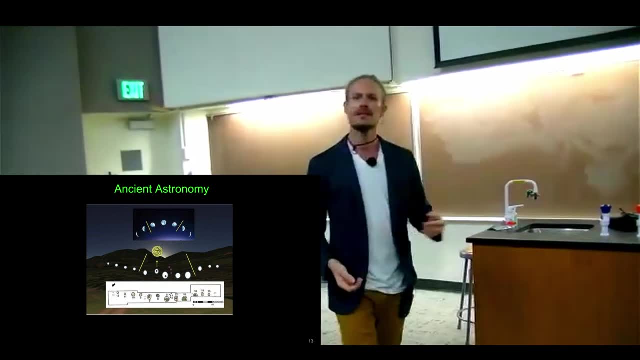 It's very close But it doesn't work out, And this drove people mad in every civilization for thousands of years And, honestly, it still drives us mad And we have these things called leap years every once in a while, which are very cumbersome and annoying right. 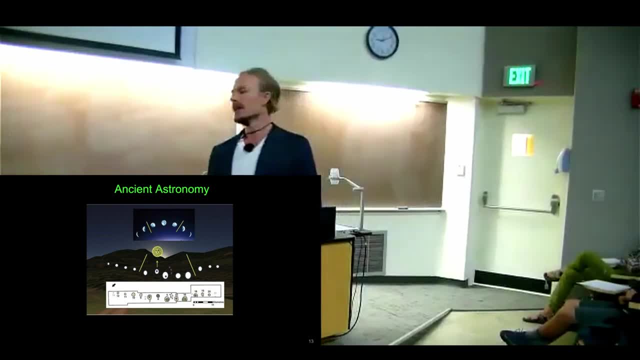 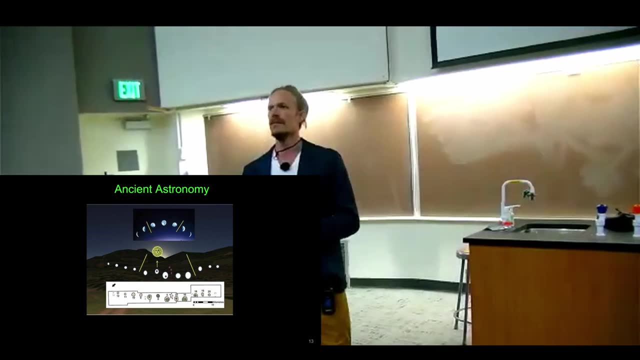 You just have like an extra day tacked on right And people, People bashed their heads against the wall trying to figure this out. I mean, people could not believe that. it didn't line up perfectly. It drove them mad, right. They thought the gods were playing tricks on them, But they studied it And they devoted a large amount of their intellectual resources to figuring out how to time that leap event, And they had different versions of this leap event in every culture, And so this is, I believe, from Northern Europe somewhere. 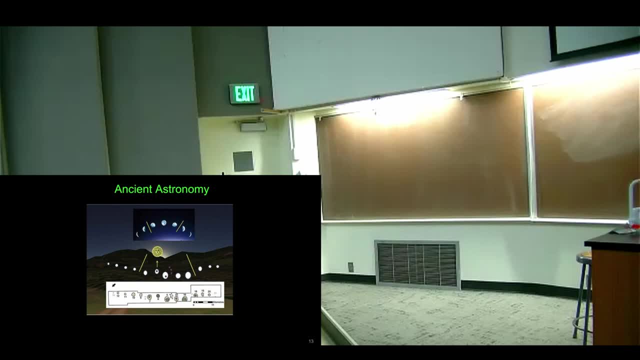 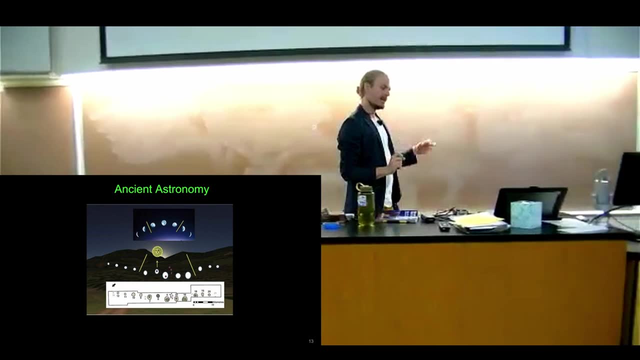 Which was one of the first slots that actually allowed them to time the phases of the moon with the summer solstice, as it happened And they were able to, They would note, after many, many decades of observing this. So the moon would show up in one of these slots. 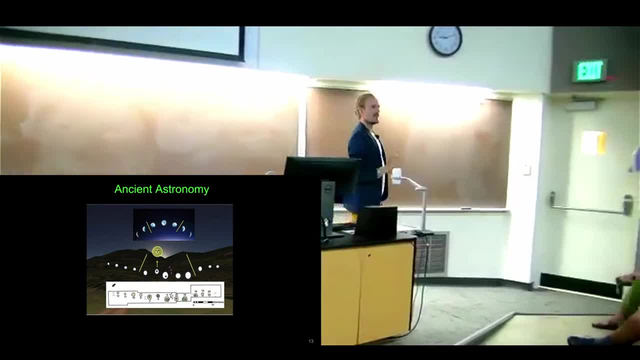 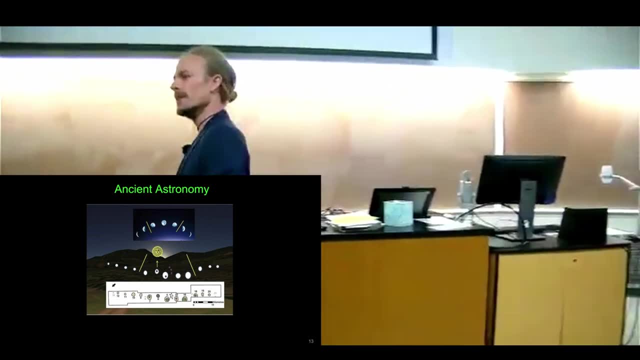 The sun would come up between this mountain And they would note exactly what phase of the moon was occurring at that solstice And they would see how it shifted year by year. Does anybody know what the phases of the moon are? Is that a reasonably familiar term? 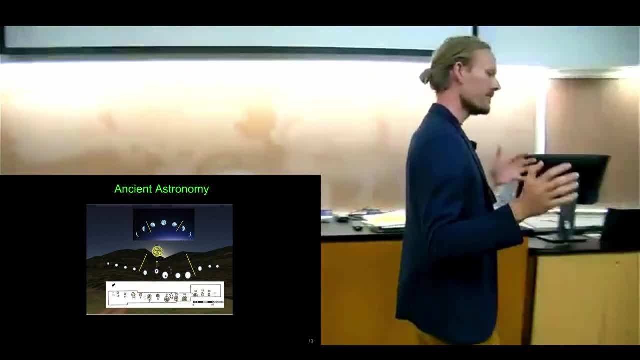 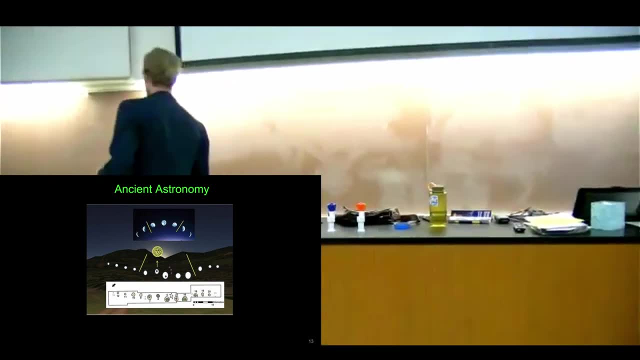 Right. So obviously the moon is a crescent. sometimes It's full, other times They would see how this would shift And they would use this To time their leap events. Some of them had leap months. Most of them had leap months. They would just tack an extra month on every once in a while And you know this appeased them to some extent. This made the world even more predictable, Because now you could use the moon to actually predict how close you were to the solstice. 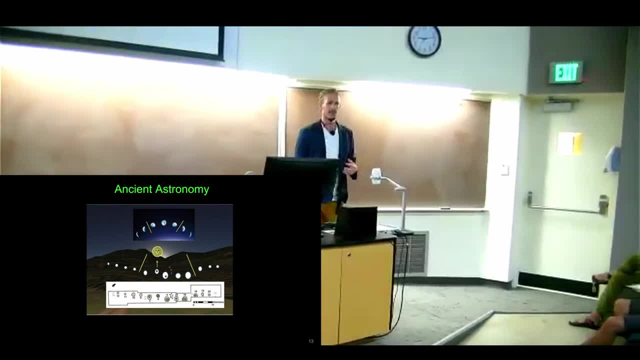 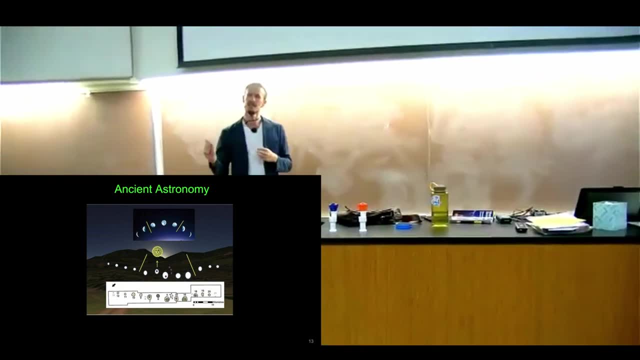 You could use the moon to time when your planting interval came around, Because obviously the moon, If there's only 12 or 13 of them a year, It's a lot smaller interval. It's going to allow you to actually get a little closer to precise. 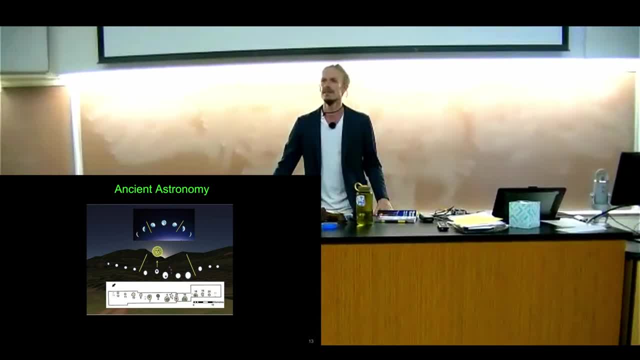 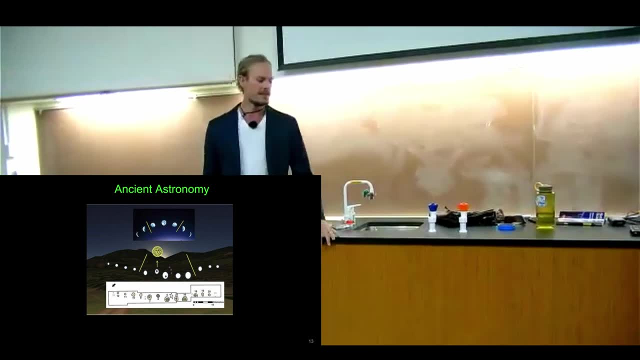 Does anybody here have any experience growing things? Yeah, a couple. I'm trying to grow things. this year I grew some amazing tomatoes for the first time. I used to live in the city, So this is all new to me. It's terribly difficult. 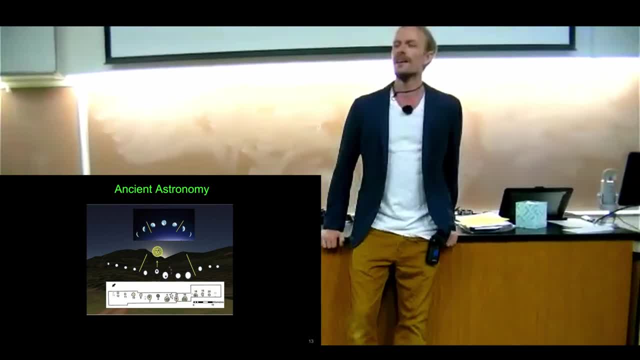 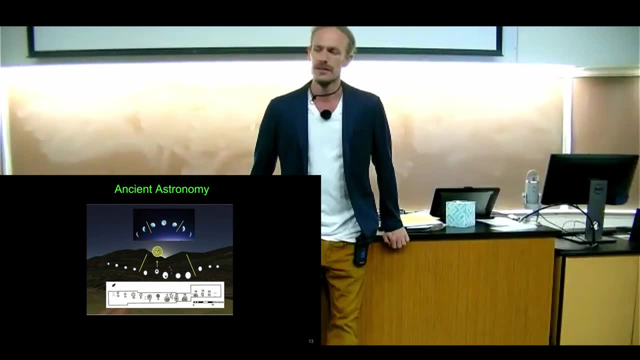 It's very difficult, But it's quite rewarding too. I highly recommend- even if you can- just, you know, grow a flower in your dorm room or something- There's something about taking care of it And the regularity that it requires. 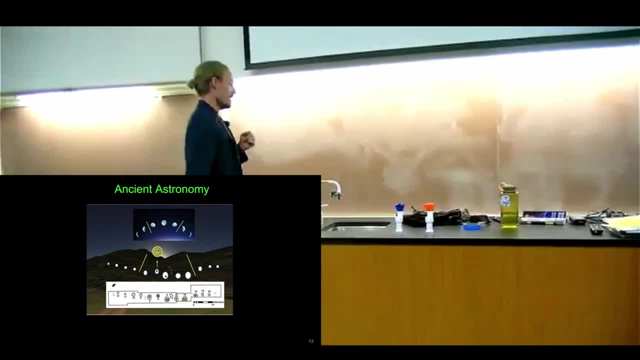 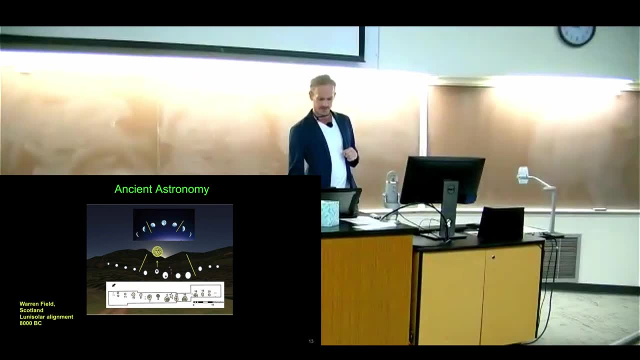 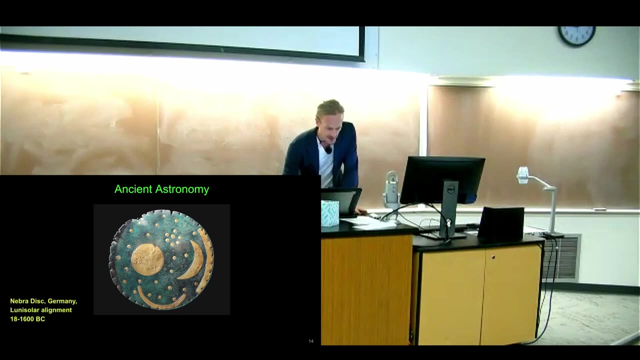 It's very good for the soul, So having this ability to time those events was really critical. Now there's something else about the moon as well. Again, this is. another example of This is the Nebra disk. This is found in Germany. 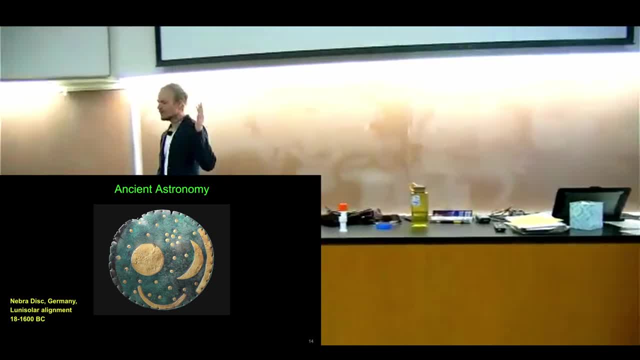 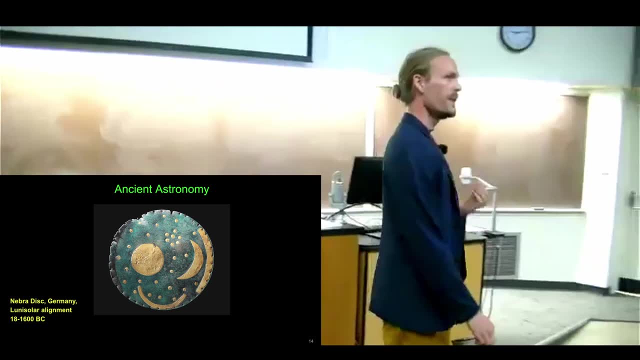 This is from maybe 10,000 BC. I'm told that this disk actually shows the constellation, the Pleiades, And it tells you exactly what phase of moon to expect When you need to add that leap month in to the calendar in order to time it up with the summer solstice. 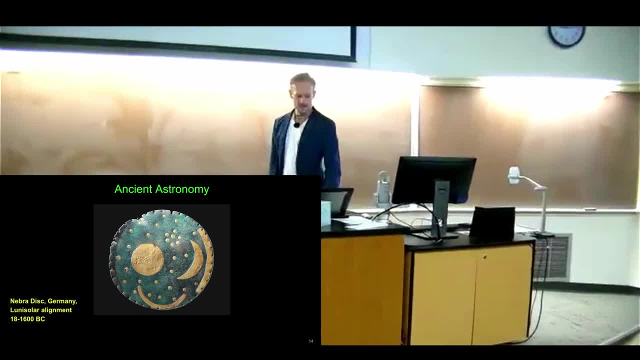 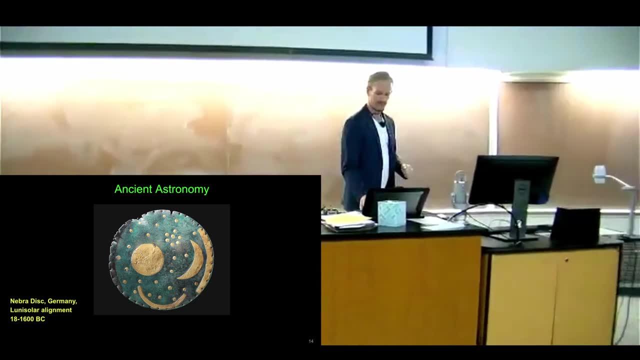 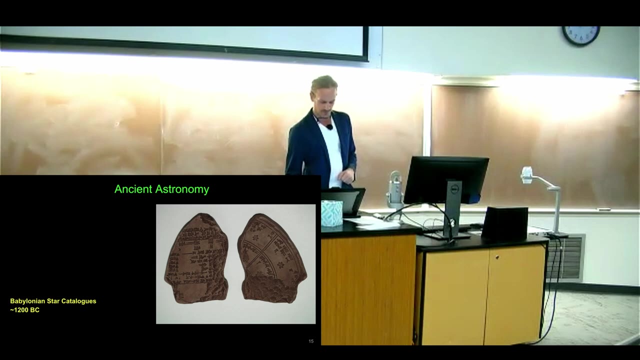 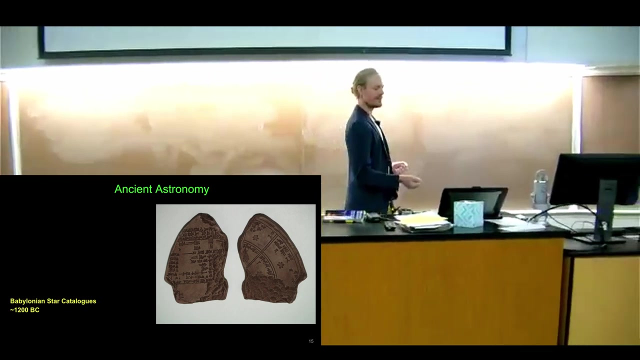 So people have been concerned with this for thousands of years. right, Like I said, it was driving them a little batty And people began to write it down. So, again, This priest class that was able to divine these characteristics. 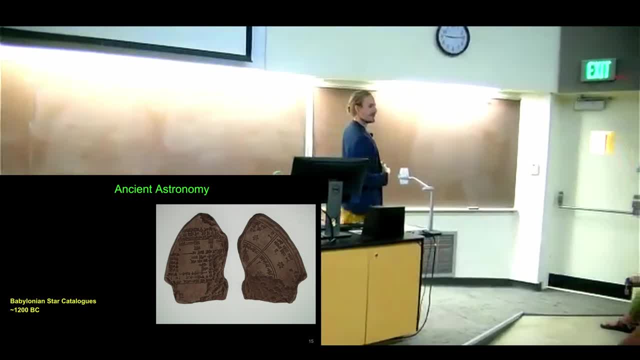 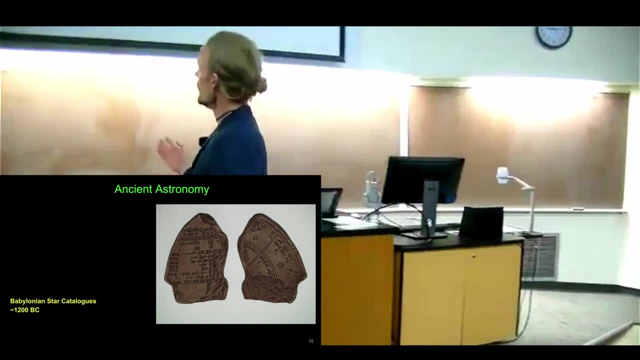 They gained stature. Some of the earliest records we have, in the West at least, are from the Sumerian tradition And you know this is Babylonian star catalog. This one's from 1200 BC. It seems apparent from the record that they were doing this for many thousands of years before. 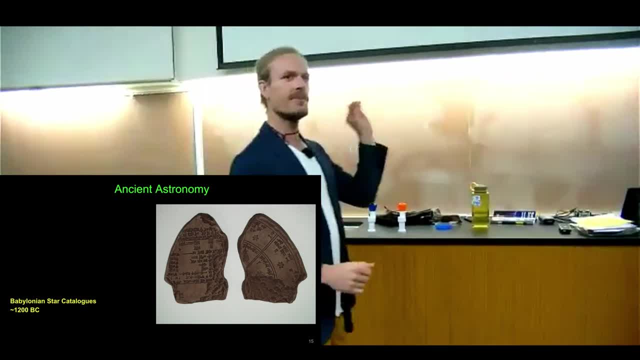 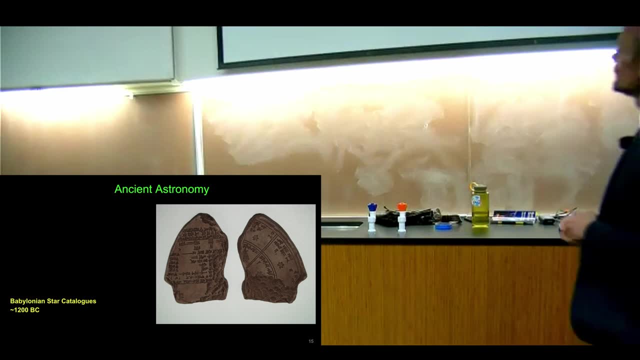 These clay tablets. These were surmising the exact position of different constellations in the sky. This was a full-time job. Now It might seem like the Babylonians- Like who cares about the Babylonians? right? We know so much more about the stars today. 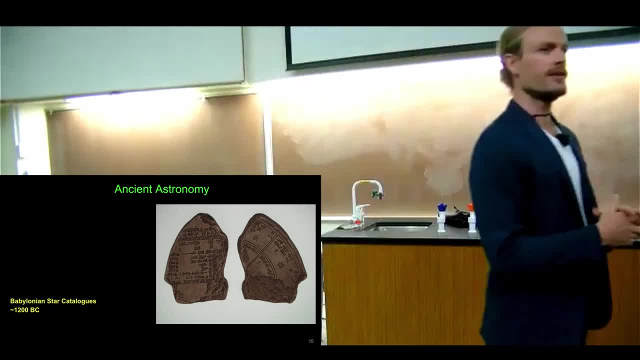 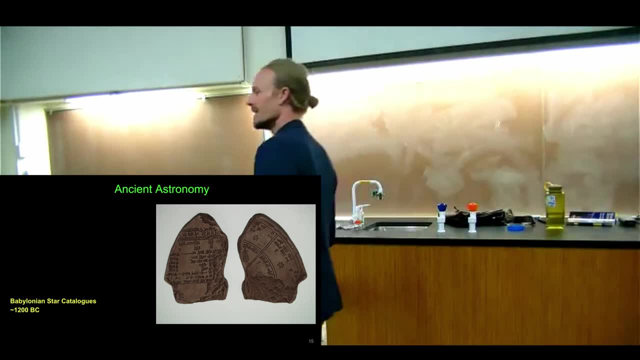 We use a lot of their work. okay, You might ask yourself, why are there 360 degrees in a circle? It's kind of a weird number, right Like where did we come up with that? What is this degrees thing? 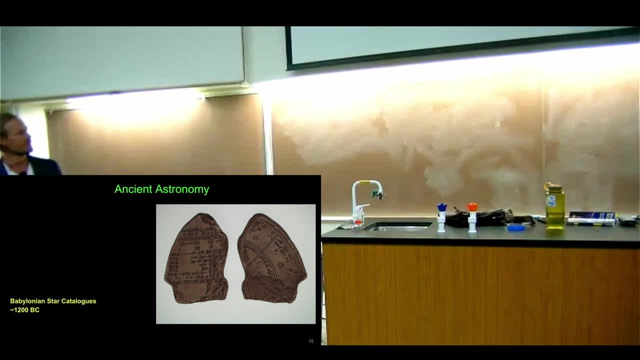 Well, the Babylonians? They actually did not have the same base 10 system that we have. What do I mean by that? Well, When we count, we count to 10. And then we start tacking more units onto that 10.. 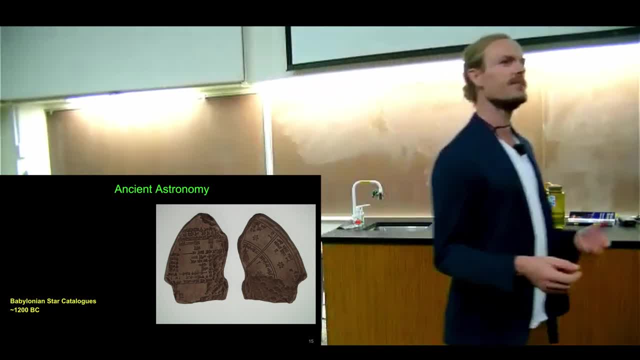 And if we want to go into the hundreds, we just add zeros. And when we add zeros, it means that, Well, there's another 10. The Babylonians didn't do that right. Theirs was in units of 6.. 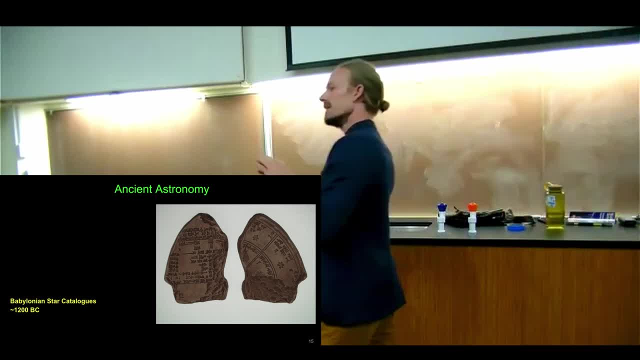 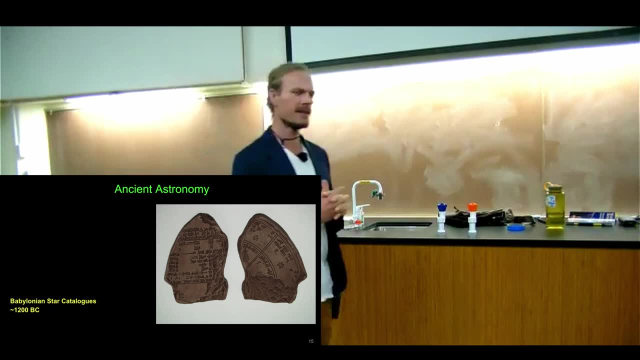 And 60. And this is how they divided the circle as well, Into units of 60. Why did they come up with 60?? It's a strange number if you think about it. Six even It's a strange number. 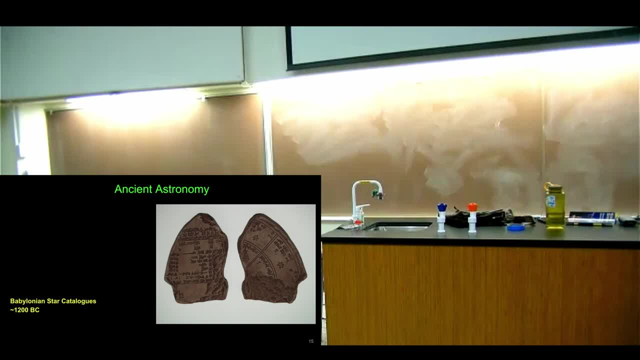 Obviously, it's easy to understand why we came up with, Why we use 10, right 10 makes sense because you can count on your hands right One, two, three, four, Six. though Where did this come from? 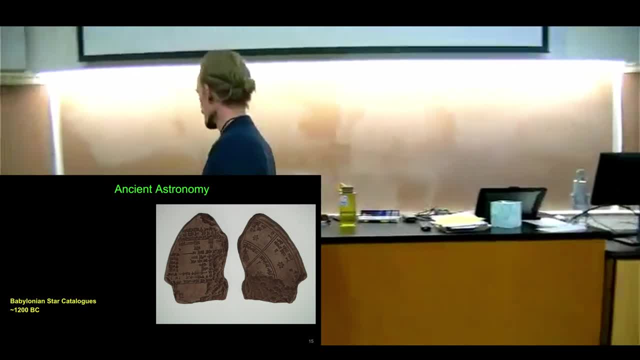 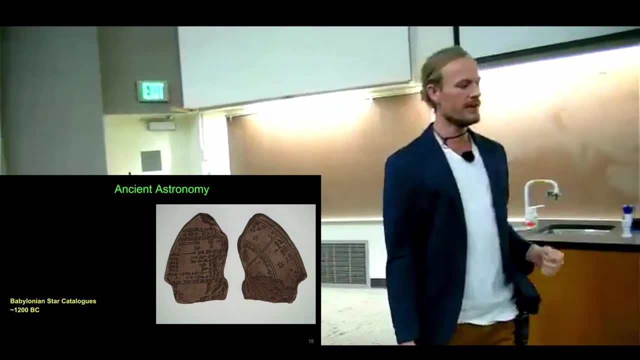 I'm not sure. I don't know the answer to that, But we do still have the relics of it And we are going to use it in modern astronomy in order to gauge the positions of the stars. We're going to be looking at angles between the different stars. 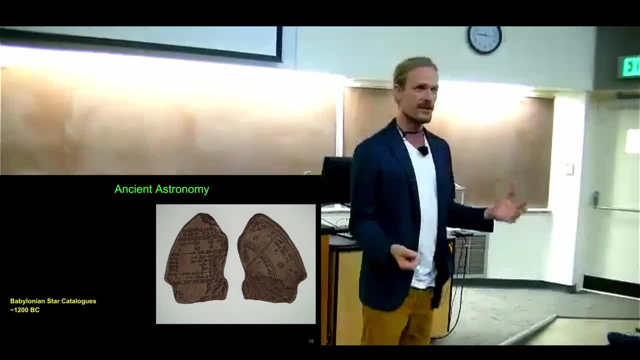 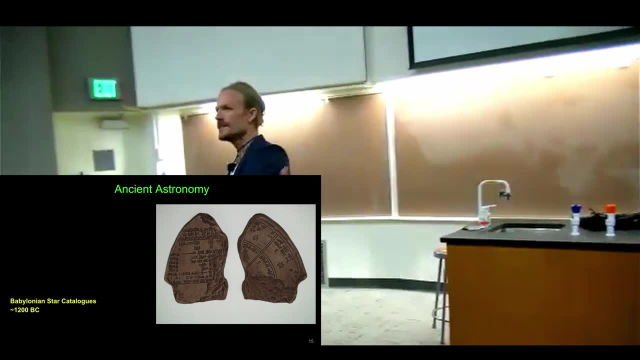 which we'll use to geometrically calculate the distance between the stars, the distance between ourselves and the stars, and so on and so forth. So whenever you hear someone say, ah, this galaxy is so many light years away, or whatever, 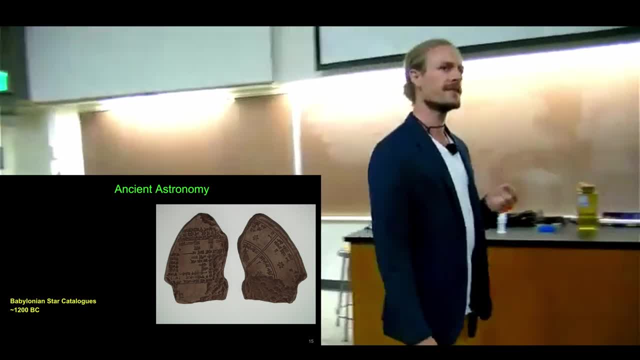 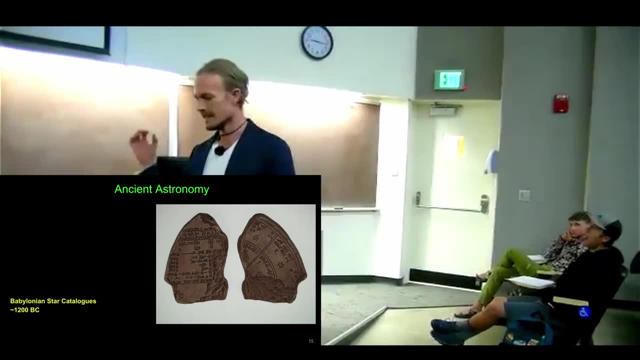 how do they know that? They know that because of the angles in the sky, in addition to some other characteristics that we'll get into later about the light itself. But largely this idea comes from the Babylonians. These are not primitive people. 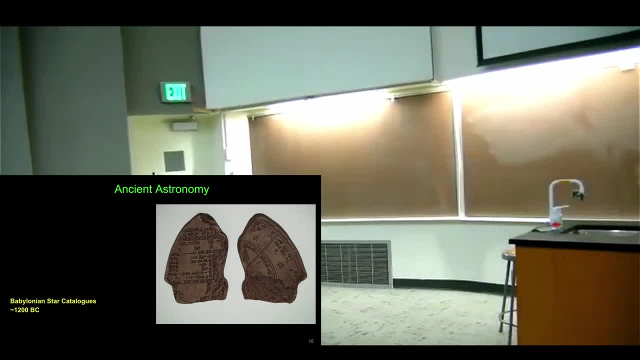 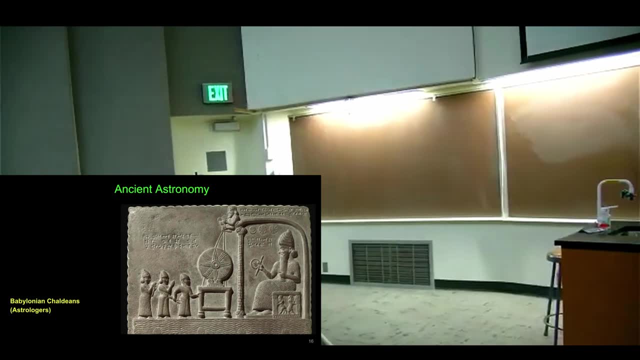 They're very sophisticated. They had an entire class of people devoted to this. In fact, these people were called the Chaldeans, All right, So this is really interesting. There seems to be a group of people in Sumeria. 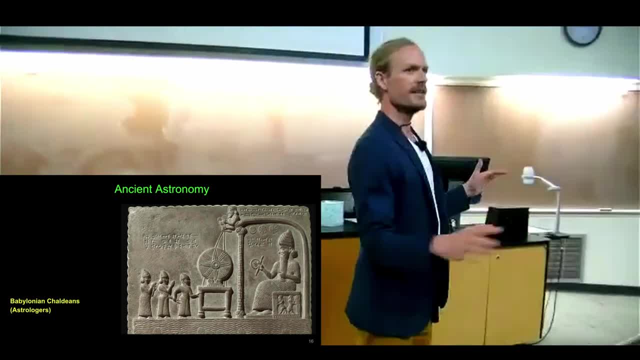 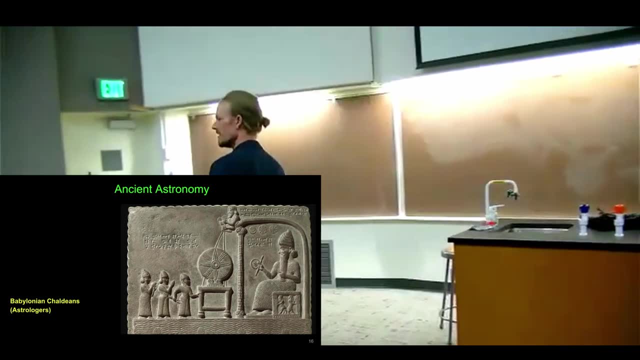 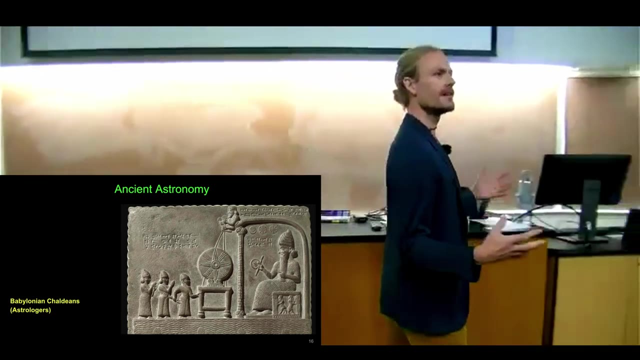 So let's back up a little bit Sumeria. It's essentially where Iraq is today, Which, if you think about it- this is the roots of our modern Western civilization- is in Iraq, And it's a bit of a tragedy what we've done to Iraq. 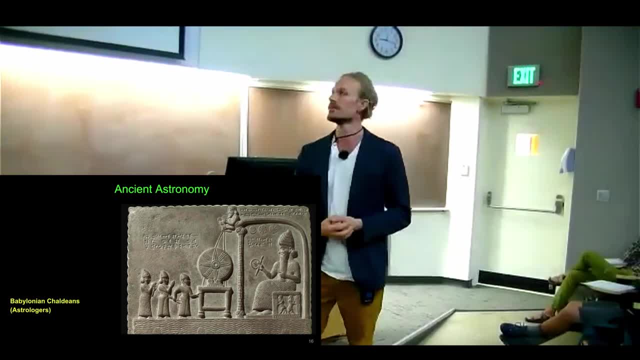 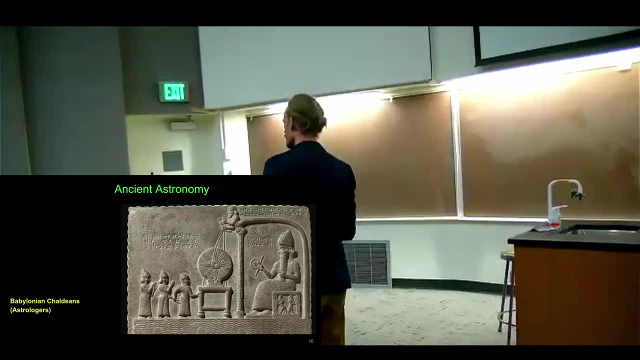 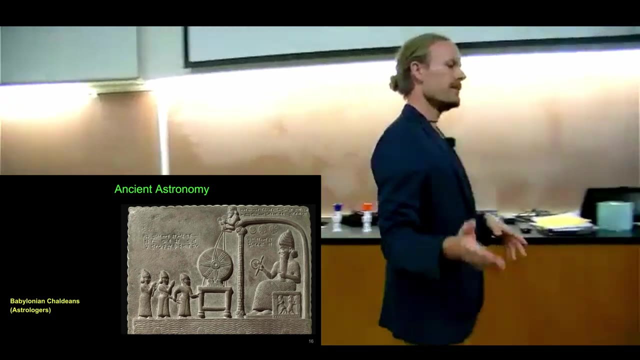 because it's our birthplace. to some extent Now there was a little Iraq. used to extend further into the water than it does today. It was The tides had pulled back. The glaciers were still melting From the previous interglacial. 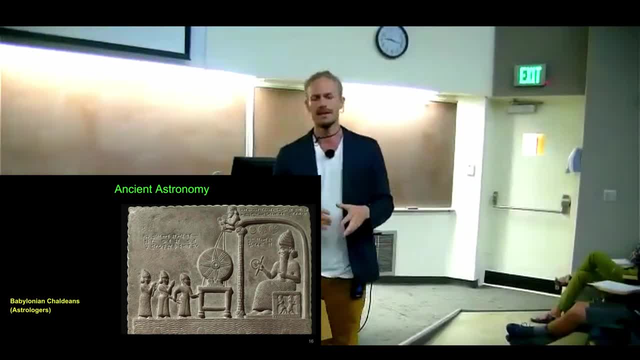 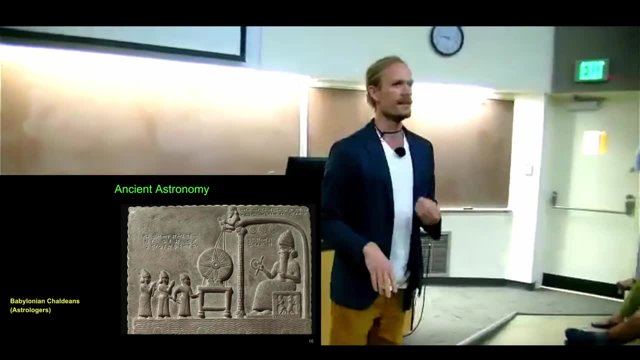 the previous glacial period there was a little strip of land on the, let's say on the western bank of the Tigris, which was called Chaldea And, for whatever reason, the people of Chaldea were the astronomers for the Sumerian Babylonian people. 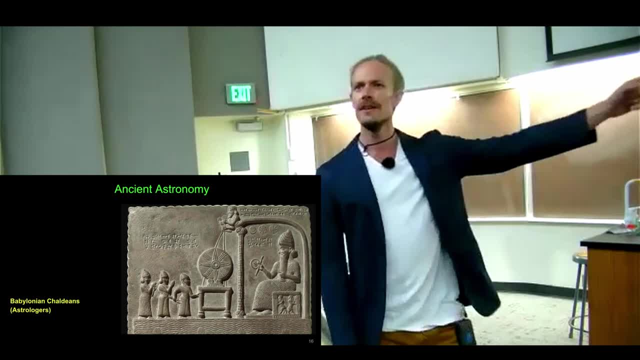 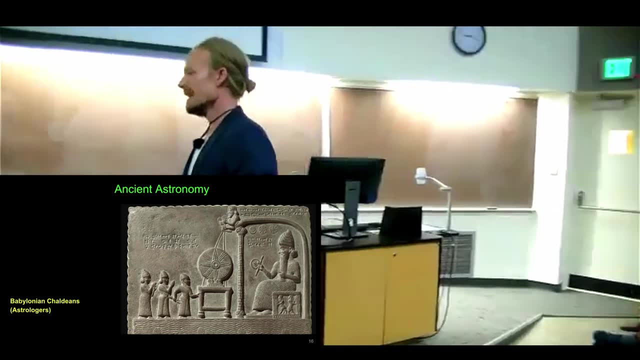 Now that's pretty wild if you think about it. That's like hey, there's a neighborhood on the west side of Ashland where the astronomers live. Pretty weird right, And they didn't. just It wasn't. It wasn't like people moved there and became astronomers. 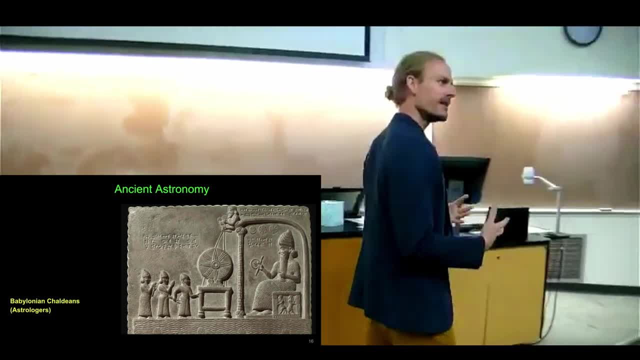 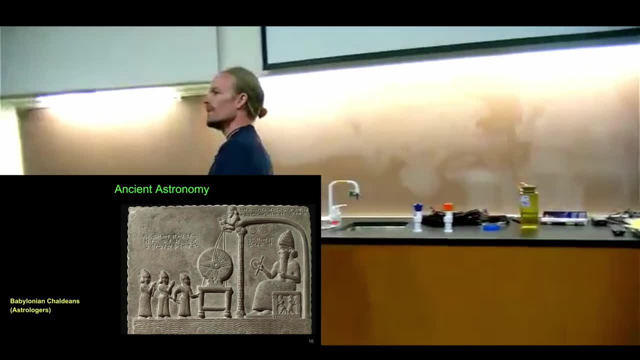 This was an ethnic class of people that were the astronomers. Their fathers were astronomers. They ascended into this role, They were born into it for some reason, And the Babylonian civilization depended on these people. They didn't appear to treat them very well. 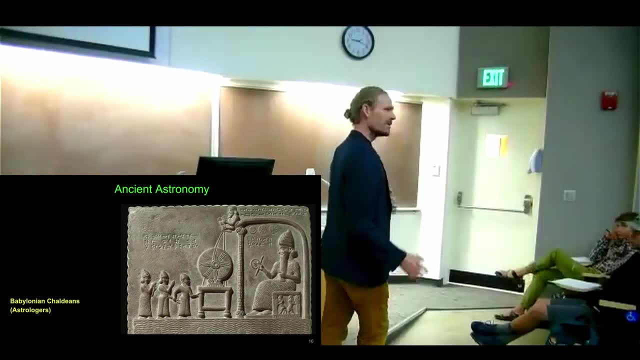 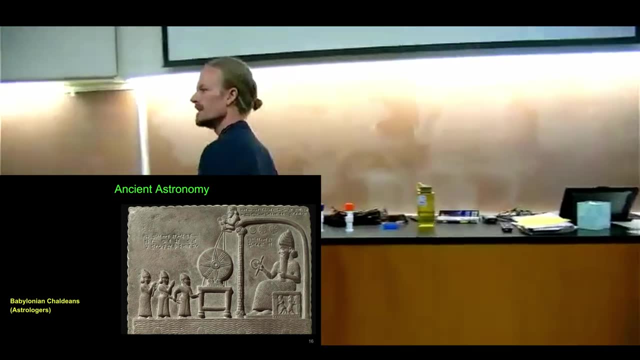 which is really interesting, actually. So Babylonia was a giant bureaucracy, much like today, And we'll see this over and over again. In fact, the state, if we think about it, what the state really is- is a giant bureaucracy. 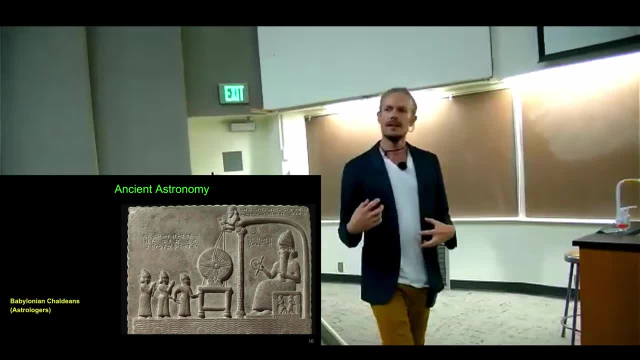 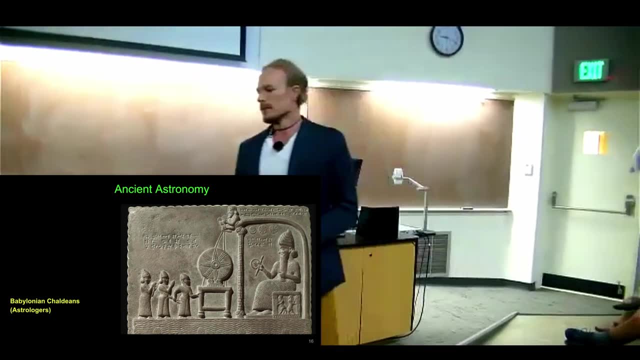 It's a way to get things done so that we don't have, You know, when we have conflicts with people, we can resolve them without starting a nuclear war. Right, I mean, You know, if you're with me for a minute. 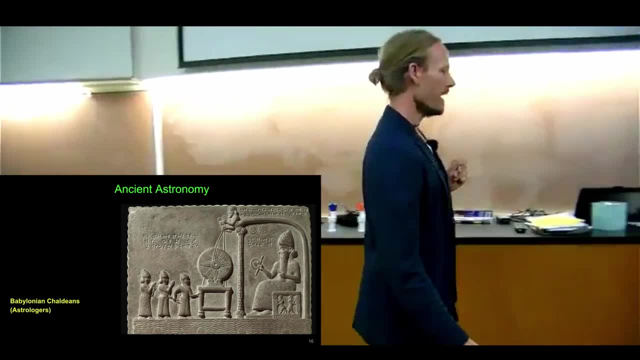 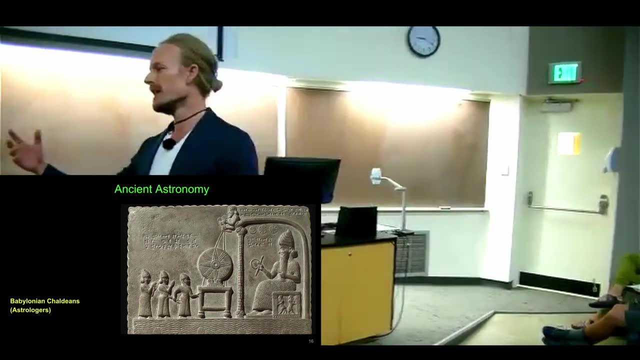 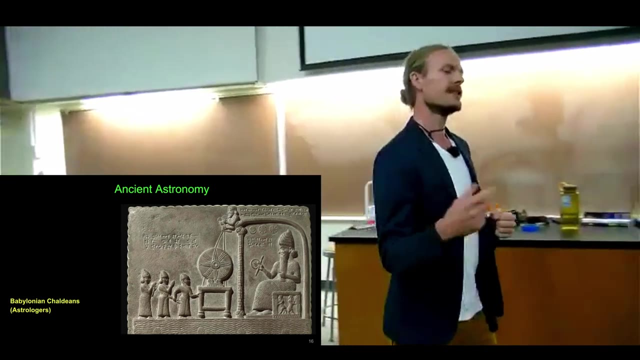 if you don't have a bureaucracy, if you don't have a state, what happens if? What happens if you? You know What happens. if your neighbor has a dog and you have a goat and your neighbor's dog kills your goat, What do you do? 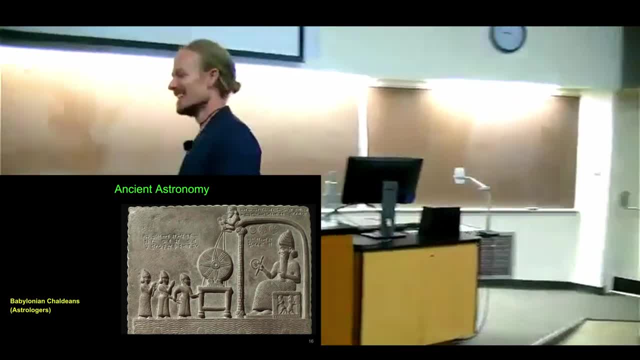 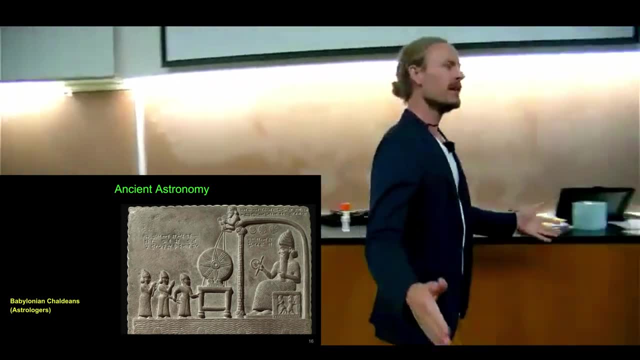 Right, Shoot the dog, fight the neighbor. I'm hearing. Right, But now what happens? Okay, fair enough, fair enough. Okay, let's say you shoot the dog. Let's say you go talk to the neighbor. Hey man, your dog ate my goat. 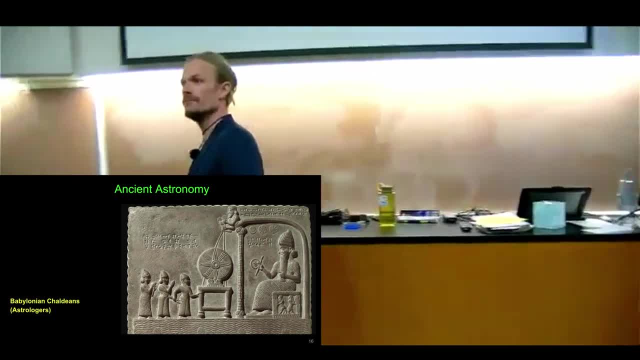 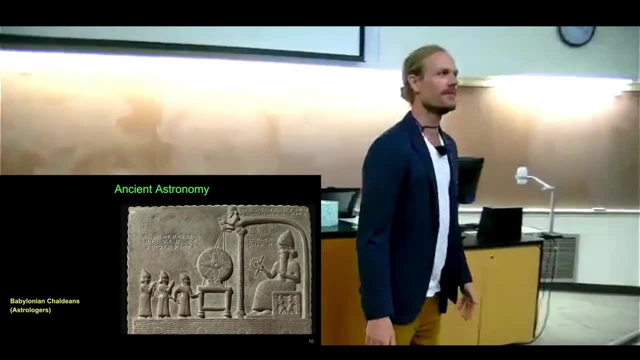 The neighbor is- Let's say he's a decent person. He's like: okay, I'll buy you another goat. Okay, cool, But what happens if the neighbor doesn't want to buy you another goat? He says, eh, not my problem. 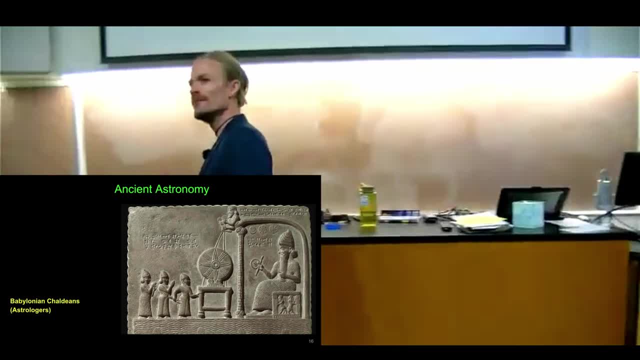 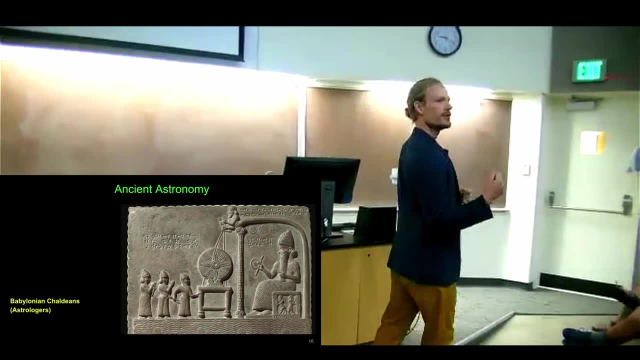 Well, maybe you shoot the dog. Well, maybe you club him or something, right? He didn't have Glocks back then, All right. so What if you shoot the dog? What if you club the dog? Well, the neighbor might decide that he's going to. 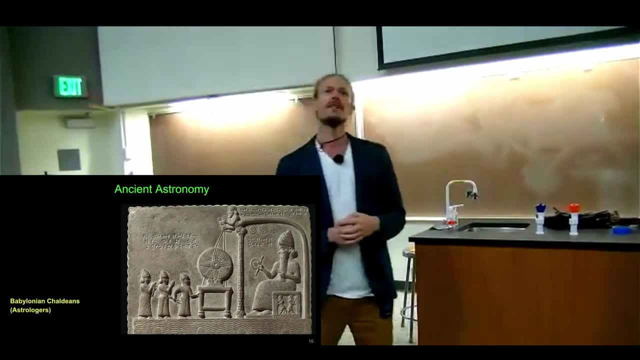 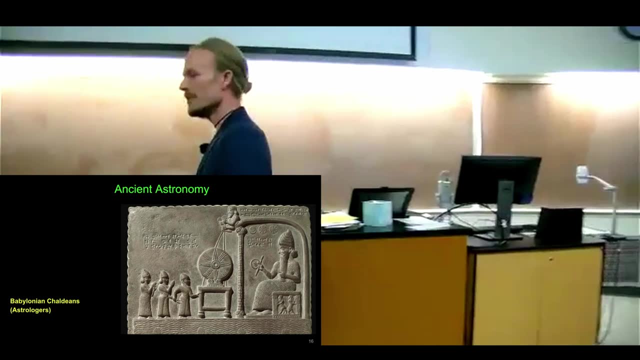 He's going to club three of your goats. What do you do if he clubs three of your goats? Well, at some point you're going to start shooting his family. And what happens if you shoot his family? Well, at some point he's going to start killing your family. 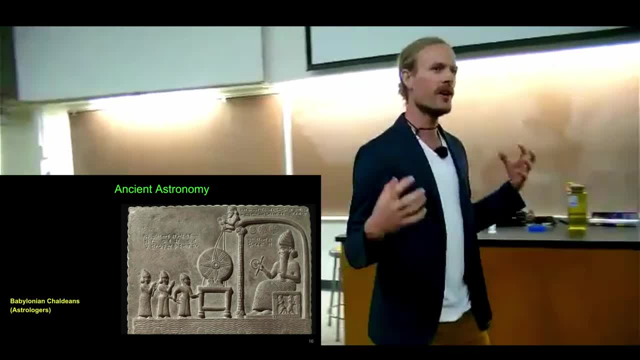 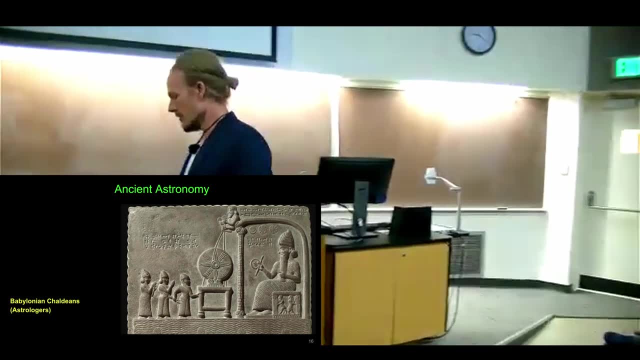 And this gets out of control really quickly, to the point that people are amassing armies against one another, And this is not a joke, right? So anytime you hear people saying like, hey, if we just, you know, got rid of this government, 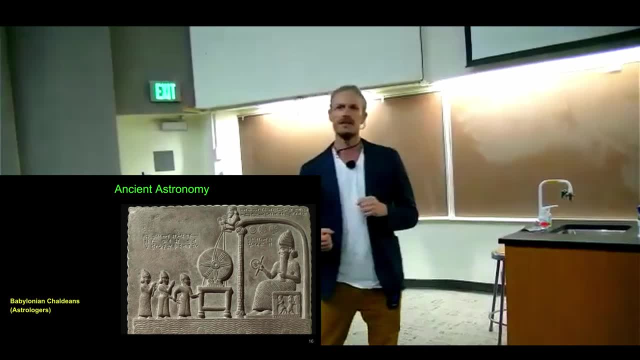 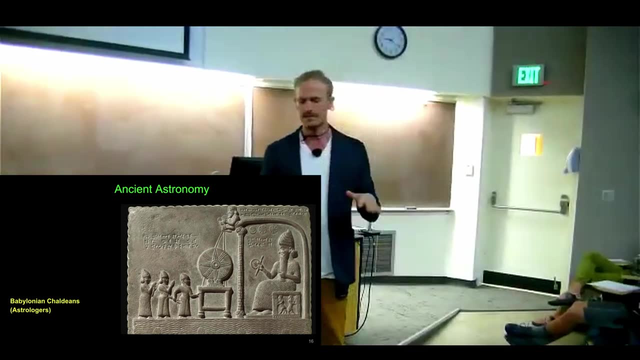 everything would be fine. It's not so clear that that would be the case actually, right? Because? Not because you're not tougher than your neighbor. Maybe you are. Maybe you'd have no problem putting your neighbor down if he's misbehaving. 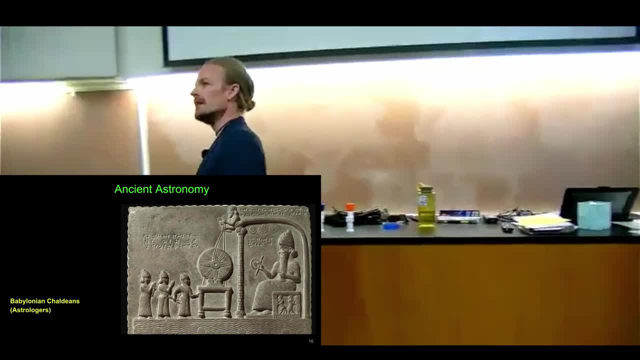 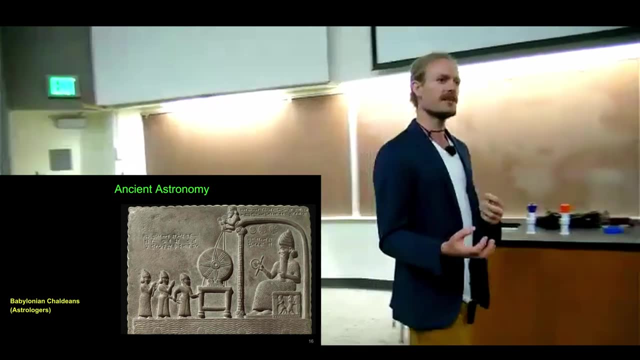 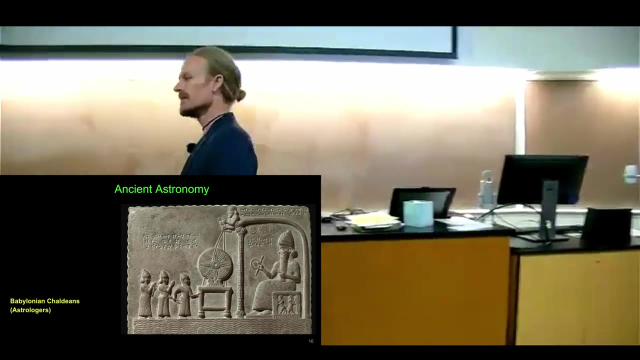 But it very quickly. And this happens in different civilizations around the world, in prehistory especially and, honestly, to this day, in situations where we don't have giant bureaucracies. You see this in Afghanistan, You see this in rural parts of the developed world even. 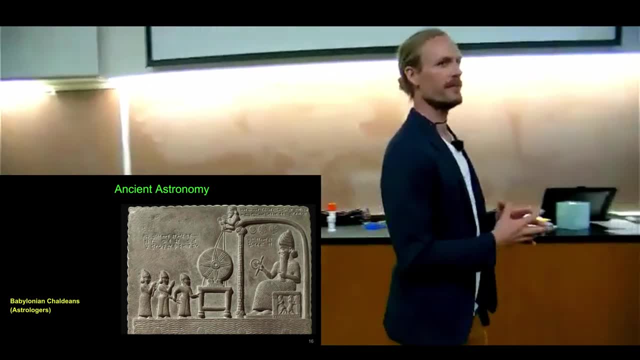 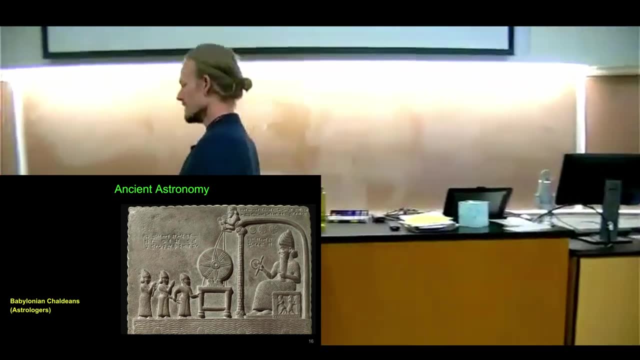 where the tribes will actually band up and start feuds with one another. This is no joke, right? We're talking about 100-year wars, very devastating things. So the state- the reason we have a state- is so that that doesn't happen. 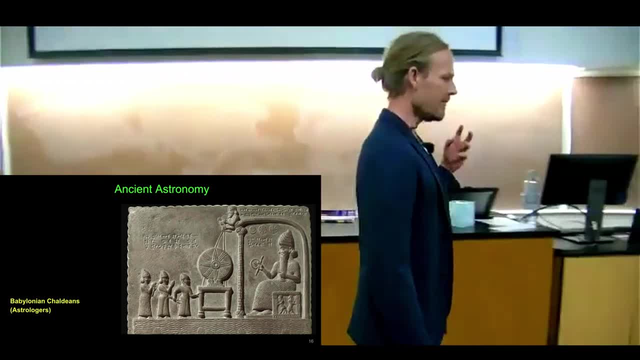 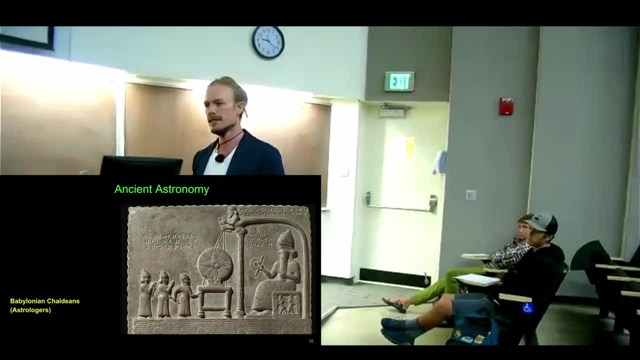 That's essentially what it comes down to, And so the establishment of a king is really just a figurehead. right, that symbolizes everything about the state that we deem to be worthy. right, Everyone's going to make a judgment call When my neighbor kills my goat. 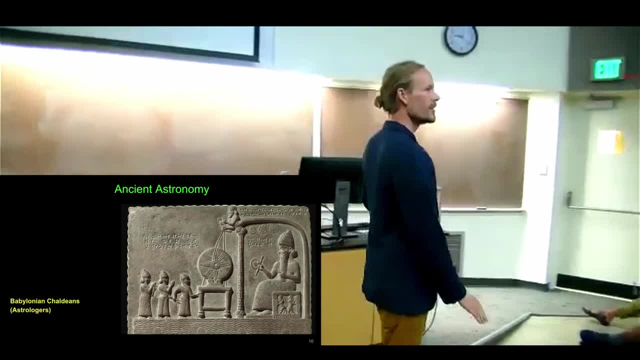 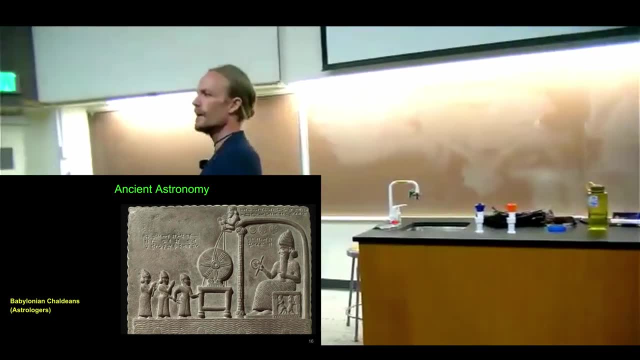 somebody's going to tell me what to do about it And that's the final word. right? There's no more killing goats after that. He's going to decide. you know, the bureaucracy and the king are going to come to a conclusion about what's going to happen. 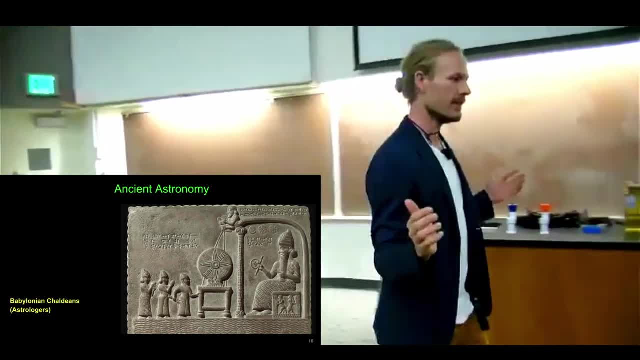 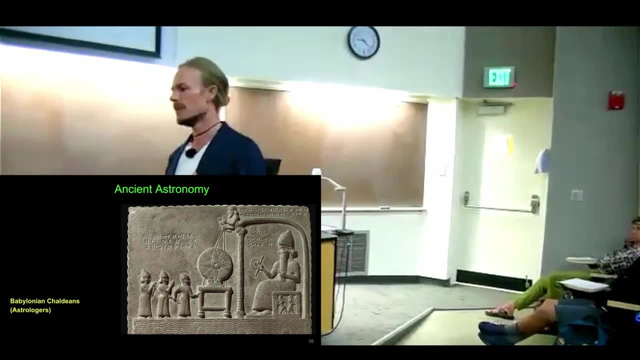 and then they're out of here, right? Then it's over, It's done. There's no more goat killing after that, And so this is really really critical, right? If civilization disappeared tomorrow, it wouldn't be a fun place for most of us, right? We'd almost certainly have to get together with people around us who would be tough enough to defend us against the people who wanted to cause us harm. And, honestly, every time that civilization has collapsed, guess what it does? almost immediately Forms another one of these: a state right. 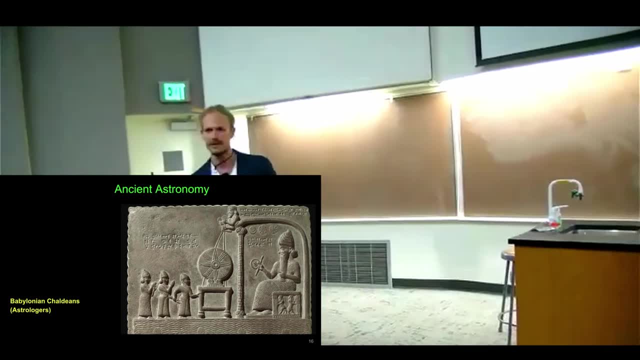 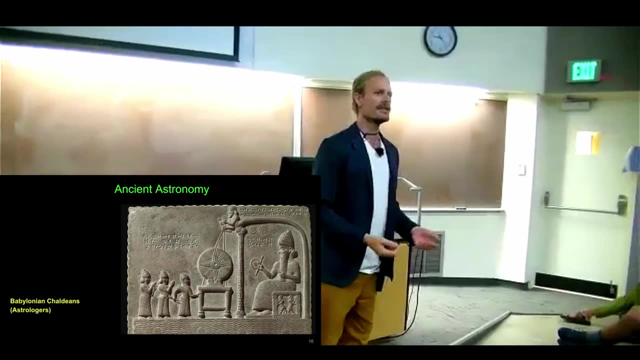 Because it's the proper solution to conflict resolution. The proper way is a very slow, painful government that gets things done. but it's arduous, right? It's not very fast to act, It's not going to immediately make snap judgments. 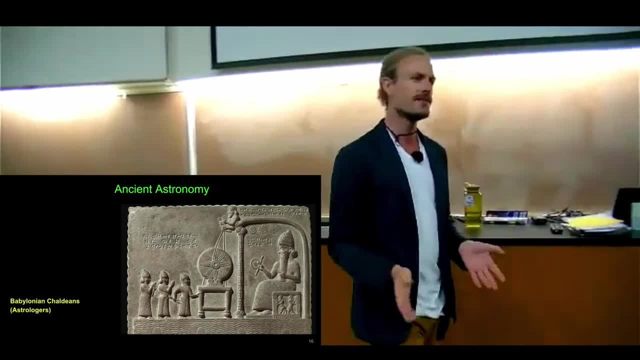 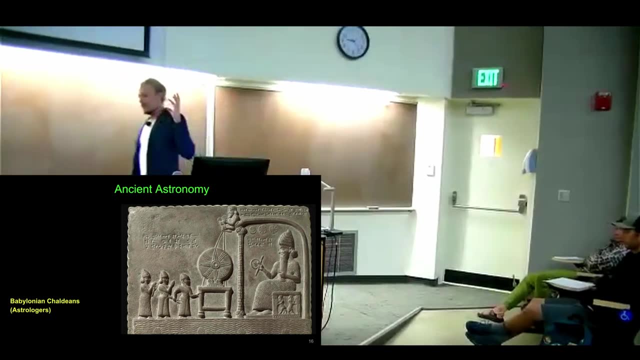 like go kill four of his goats, It's going to be all right. we need to investigate this. We need to figure out what actually happened with the goat. This is really, really important. Okay, so part of that bureaucratic structure in Sumeria. 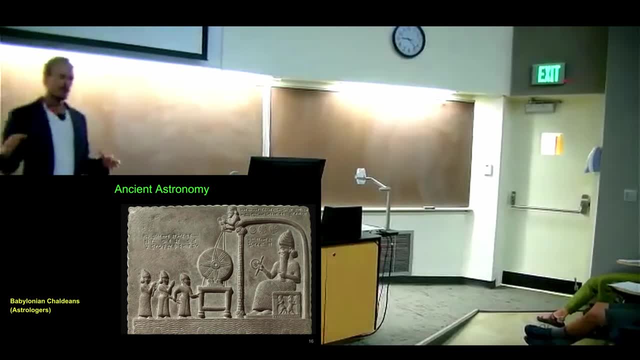 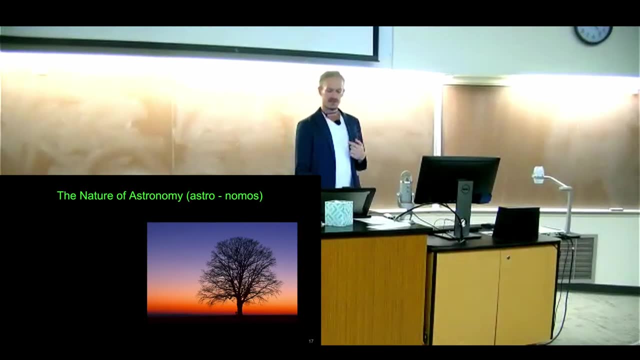 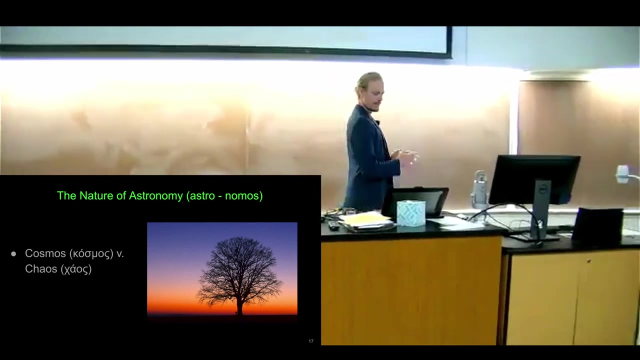 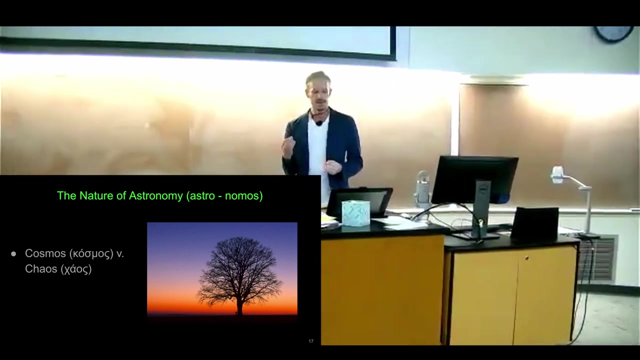 was this use of this astronomer class, which was totally dedicated to this enterprise, And the job of the astronomers was to navigate the cosmos. So I really want to talk about this word, cosmos, for a second. So cosmos technically means order and it's a Greek concept. 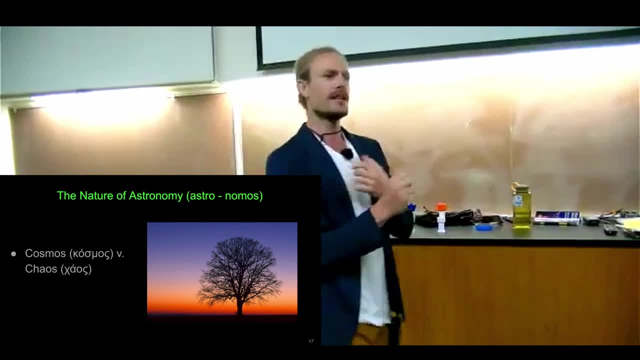 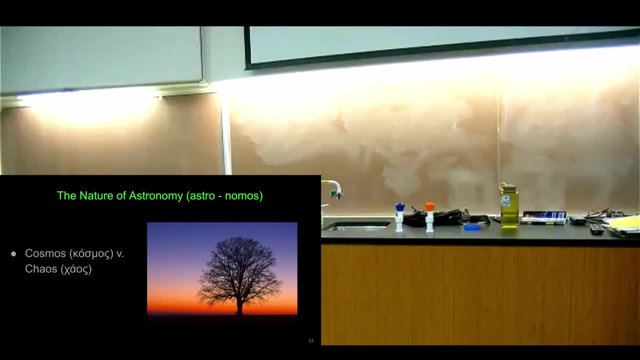 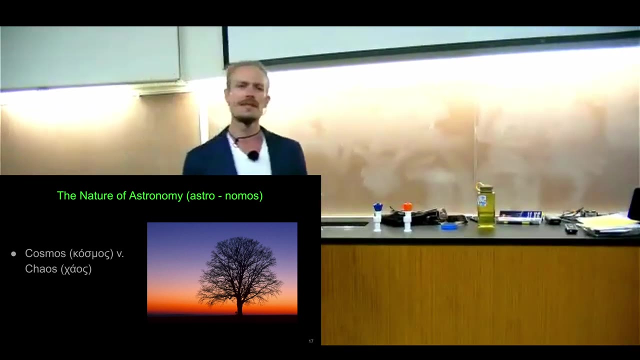 and it's in opposition to a concept called chaos, which you're probably well aware of as well. This is- This is extremely important because, as we go through this, and especially if you take next semester's course, the cosmos is important to us because it gives us structure. 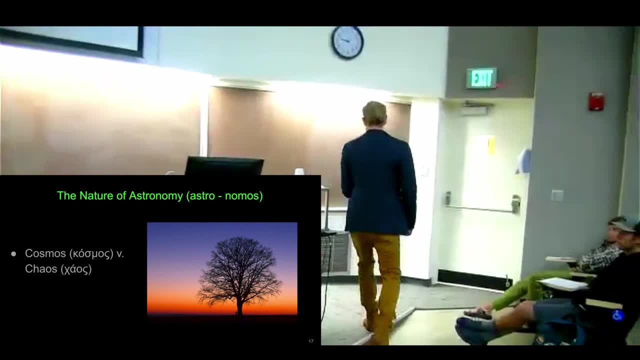 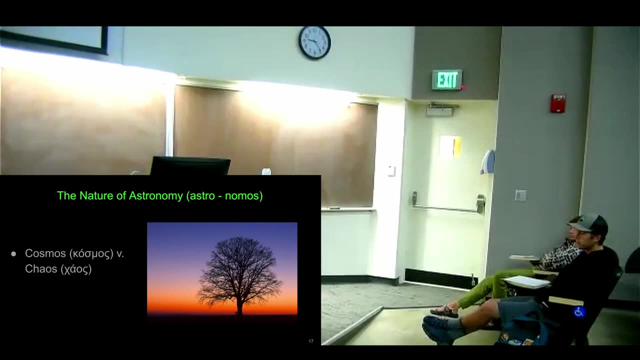 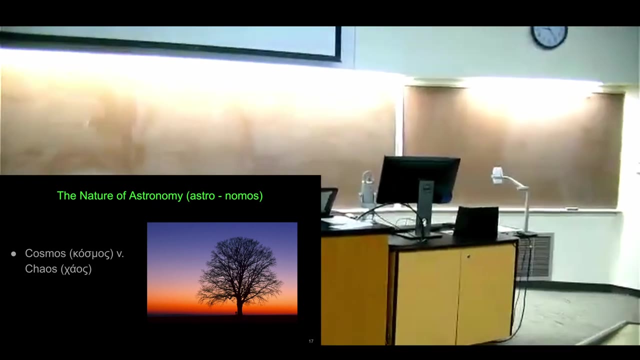 for the universe that we live in, And this was. This may seem sort of trivial, but what is chaos exactly? Well, I would say that chaos is what we don't understand. And if we look up at the sky and we look out at the world, 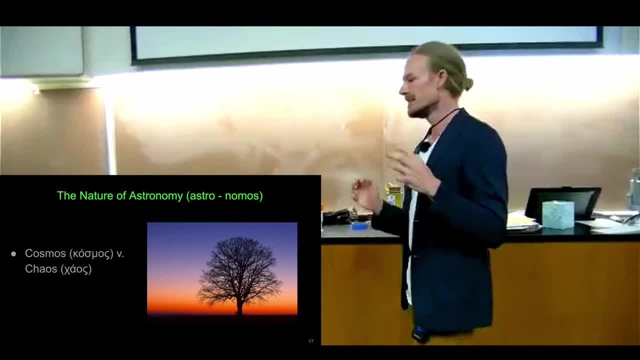 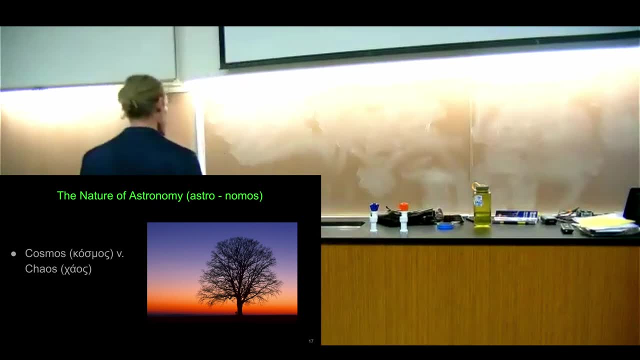 and we don't understand it. this is terrifying, right? Something could be attacking us at any moment. like I said at the beginning, This is foundational to becoming a human that you can trust the world. right? Look, you're all sitting in these chairs right now. 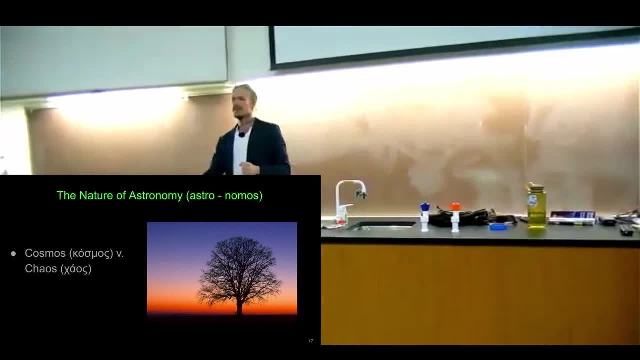 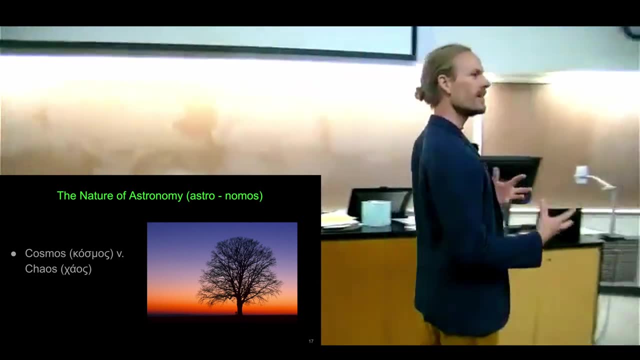 None of you are afraid that the person sitting next to you is going to just stick you with a pencil at any moment. right, Because we have order. right. This is part of our cosmology, as trivial as it seems. Everything about our conduct throughout the world. 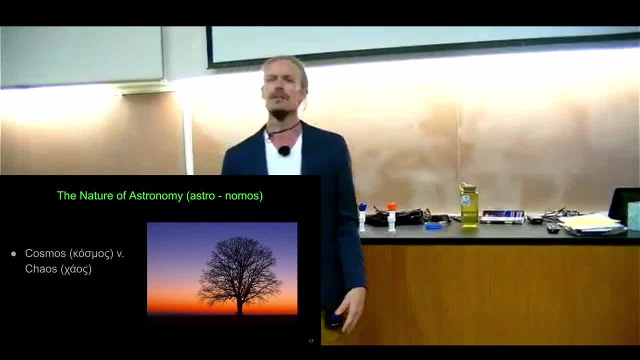 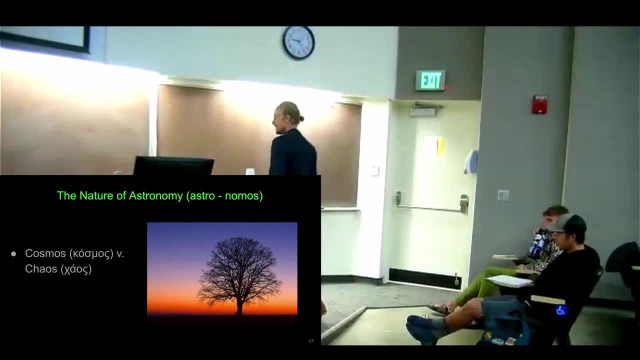 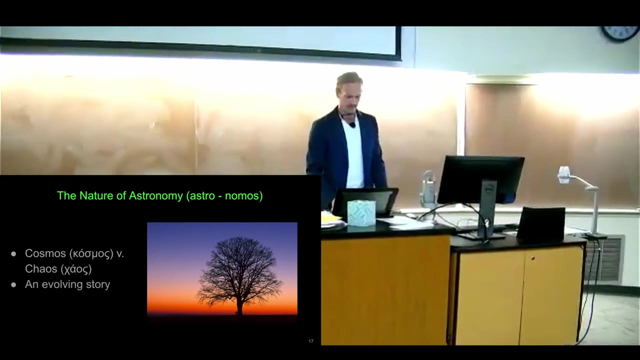 with respect to one another, with respect to the Earth itself, with respect to land rights, water rights. this is part of our cosmology And the ancients appear to have been intimately aware of this And, like I said at the beginning, 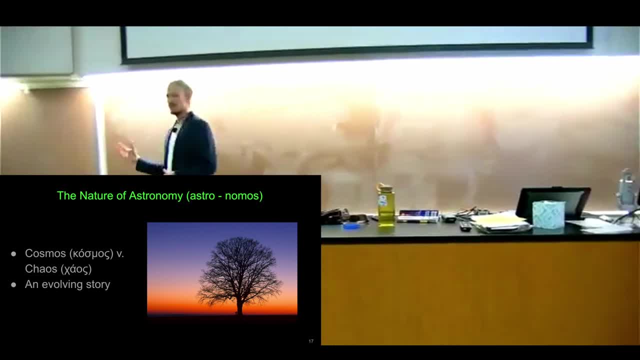 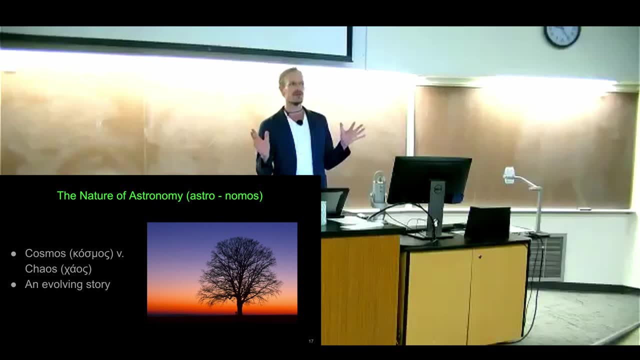 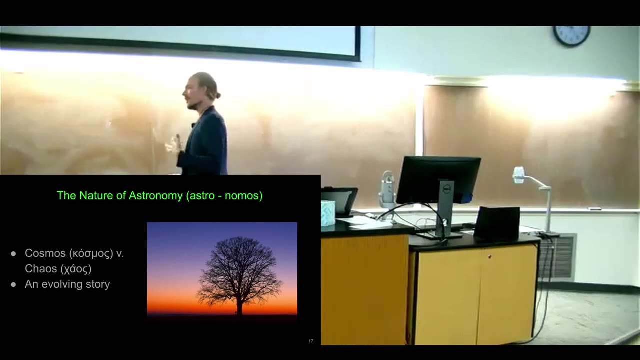 the cosmology, the astronomical stories are never finished And that's important. They're going to be evolving. Astronomy: what does it mean? Astronomos? This is another Greek word. Nomos means law. So law, what is a law? 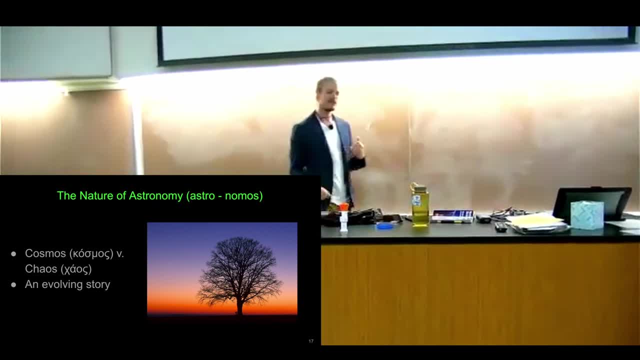 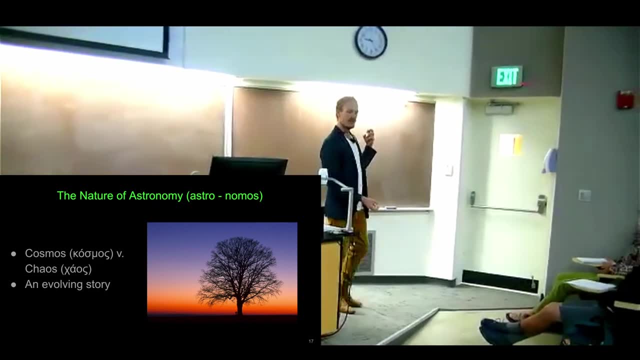 It's something predictable, right? This concept of prediction is just so vital to the astronomers as we go through it, And it turns out that prediction can go really hand in hand with explanation, which is what I would argue that science is, and we'll get into that in a little bit. 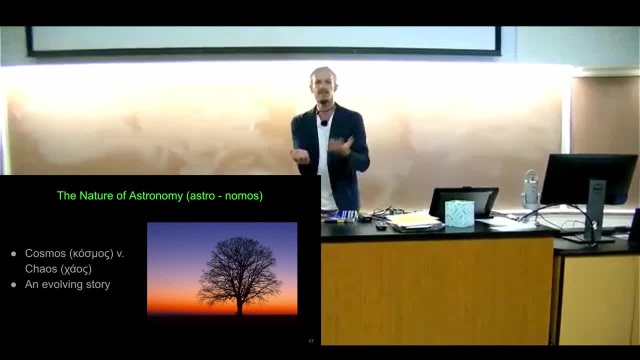 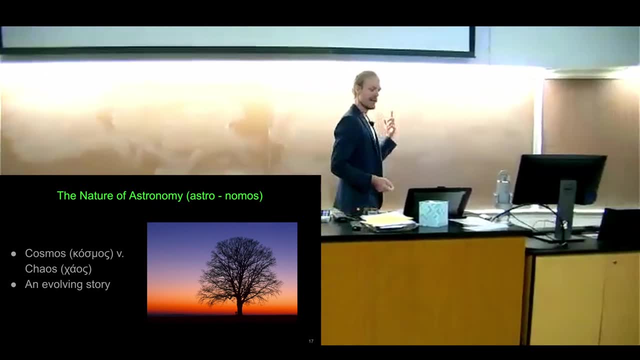 But prediction is fundamental, Not only to science, but also to technology right? You need to be able to say how that arrow is going to travel if you change something about it, And it's a predictable behavior, just like the sky. And so this ability to observe and make predictions 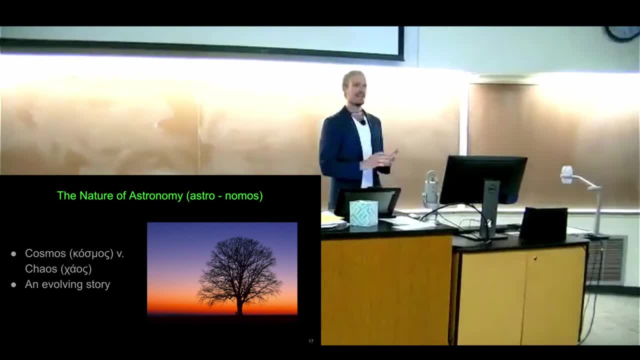 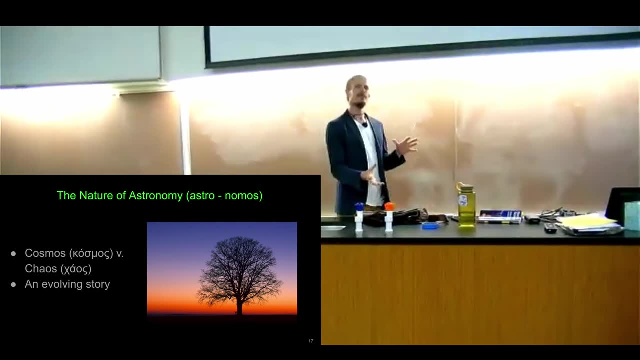 which your textbook is just harping on over and over again. it's not only foundational to science, right? Because I would say that the first step of science is going to be being able to observe some predictable behavior. You need to see something. It needs to be apparent. 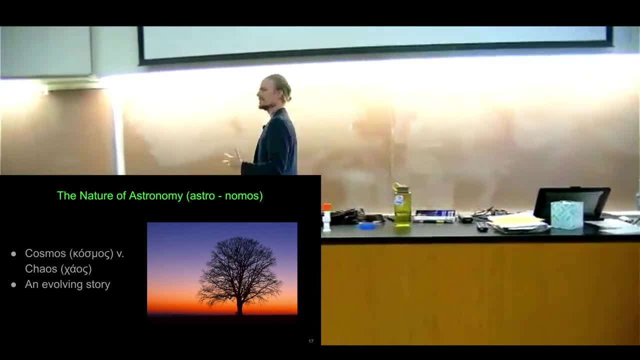 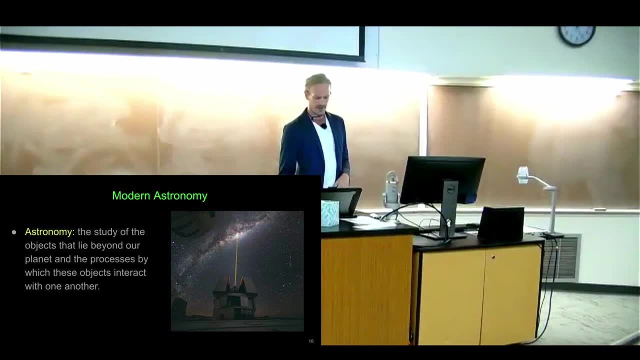 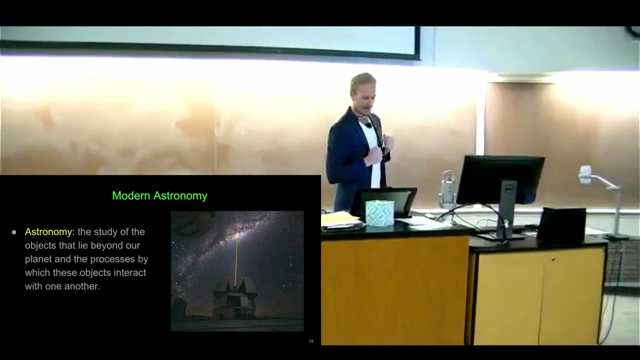 The phenomenon needs to be occurring on its own, And we're doing the same way every time, in order for us to even begin to explain it. But it's also extraordinarily important for engineering, And so, with modern astronomy, we can see that today, what we're doing is we're studying objects in the sky, right. 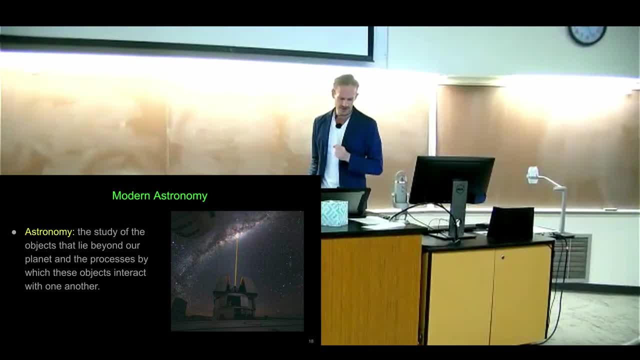 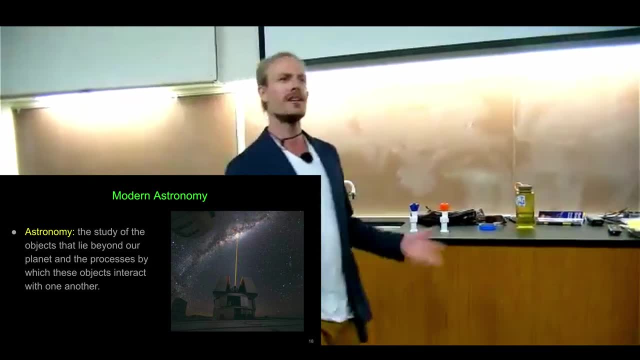 We're looking at them and we're trying to understand the process by which they interact with one another. Now, this idea of an object isn't so simple. Does everybody know what an object is? What's an object? Yes, What else? 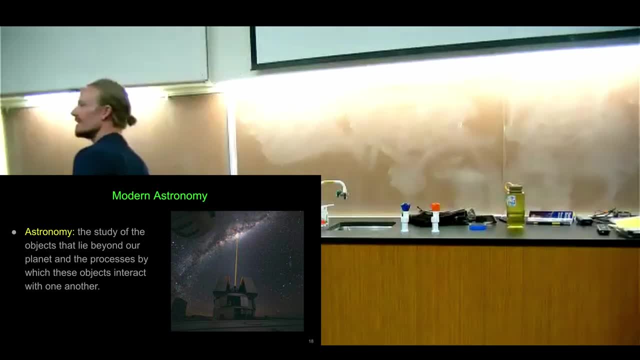 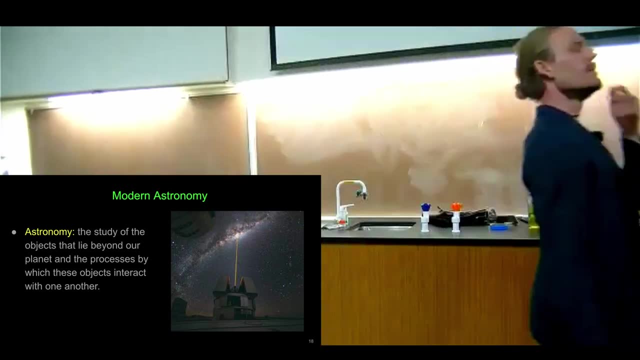 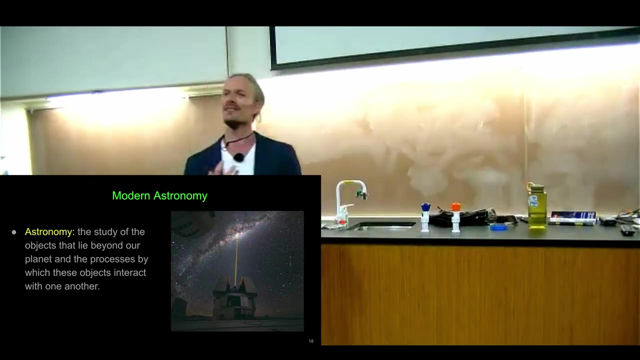 Can you put it in words, though? Can you quantify it? Can you tell me exactly what an object is? Okay, that's close, But something I can hold. What about if I hold a lot of feelings in my heart or something like this: right? 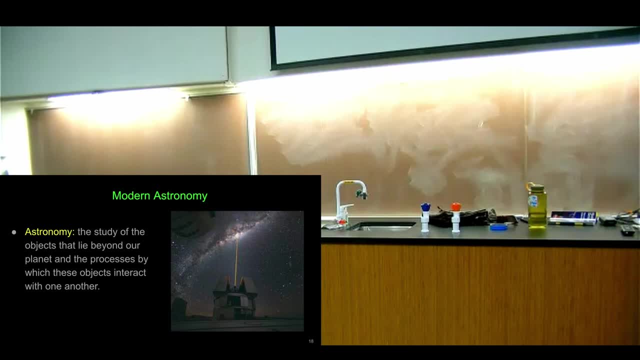 Tangible. Yes, It has mass. What is it? It has mass, It has mass. We're getting into the concept of mass all of a sudden, But yes, I think it's ponderable. right, It's material. I would say. 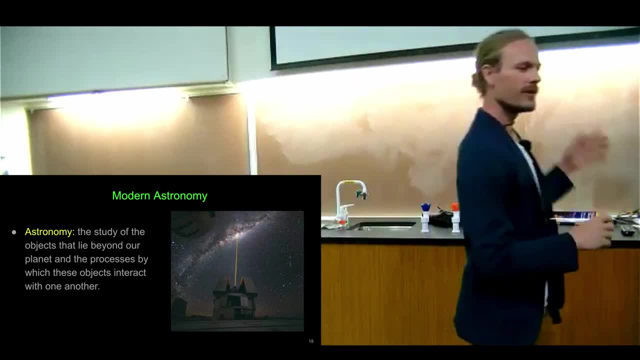 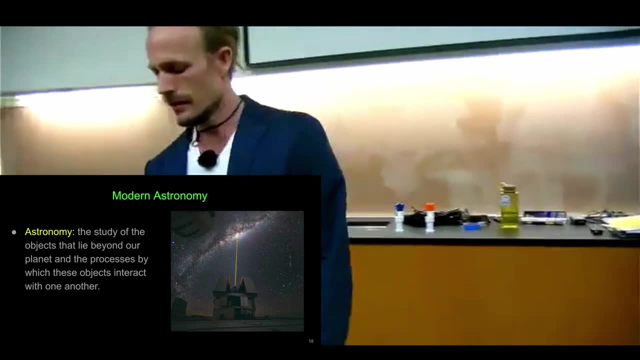 Objects are material, especially ones that exist. We can imagine unicorns and objects that don't exist, But objects have surfaces right And they delineate them from one another. So this chair, this is a chair right, But it's connected to all these other chairs. 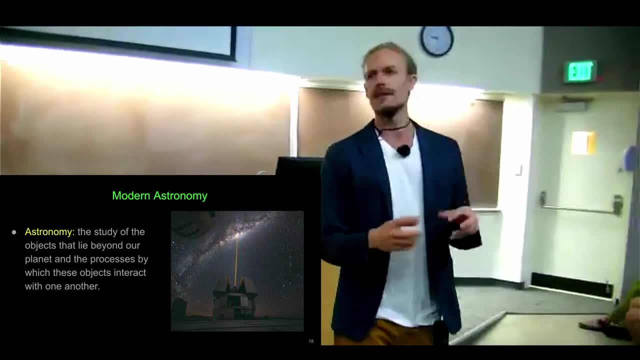 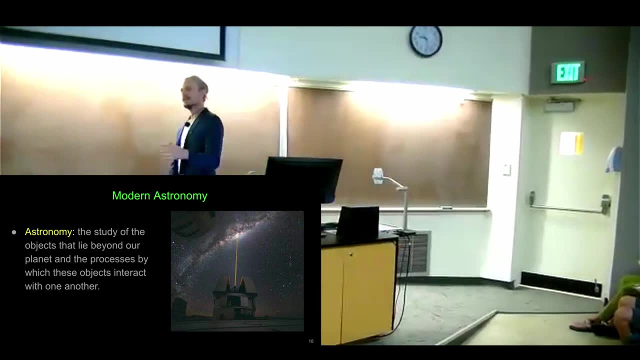 So how do I know it's a chair? Well, that's a really tricky subject, And the objects in the sky and the objects of nature are not so easily separated from one another by the traditional definitions. right, They're all ponderable. 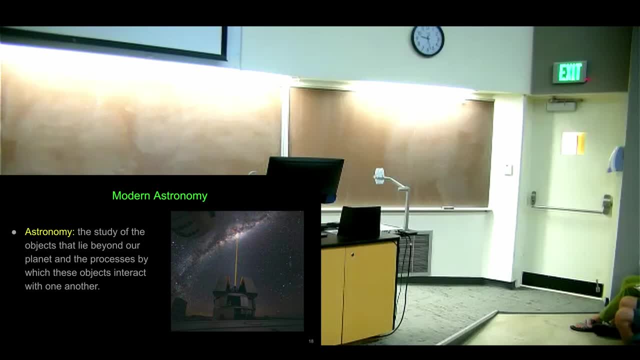 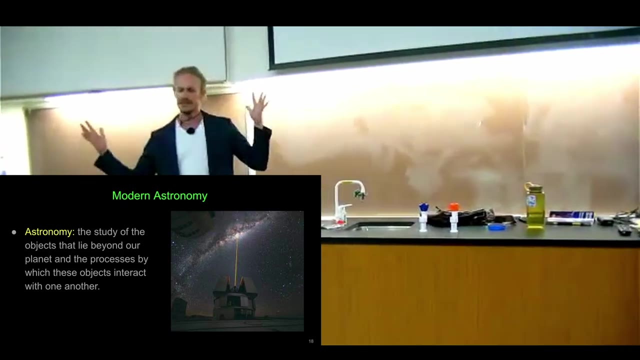 They all have surfaces, But dividing them up seems to be the quintessential scientific problem. Where does one object end and the next begin? Sometimes it's more obvious than others, right? For instance, you might say I'm an object, But it's not so clear that that's the case, right? 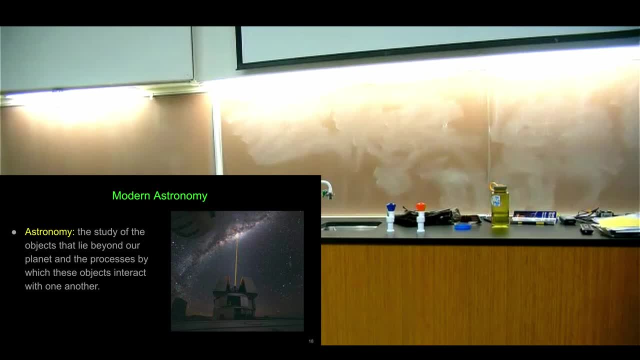 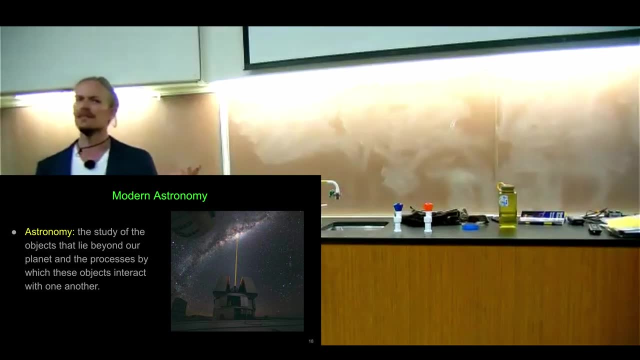 You know, Perhaps each one of my cells, if it could talk, would say: I'm the object. actually, Which one of you are the object? And, honestly, all of my atoms will be completely recycled in seven years from now. No more, no more. 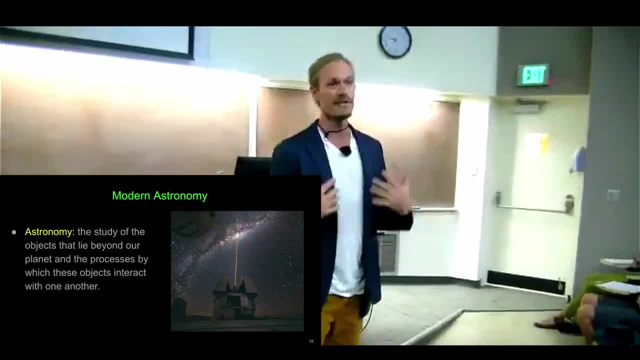 Whatever I'm made out of. right now I will not be made out of it, But I will still be here. That's a really mind-bending concept if you think about it. So we're going to keep coming back to this idea of objects. 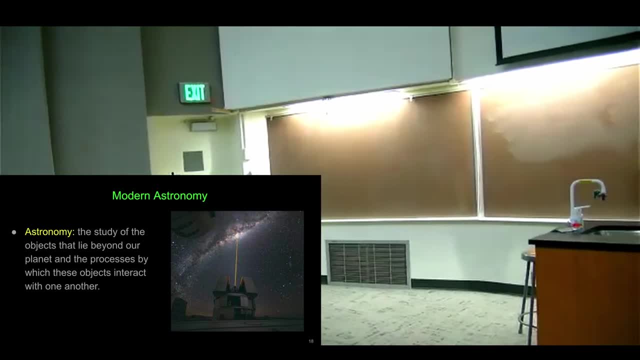 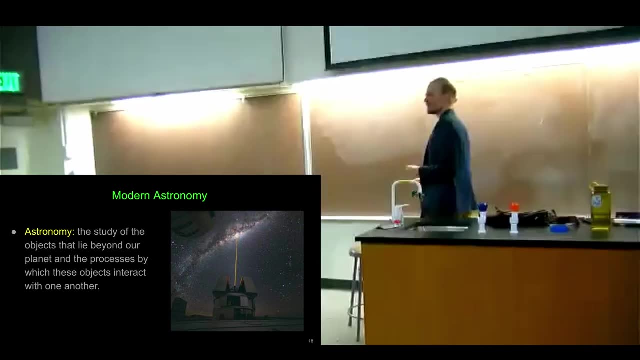 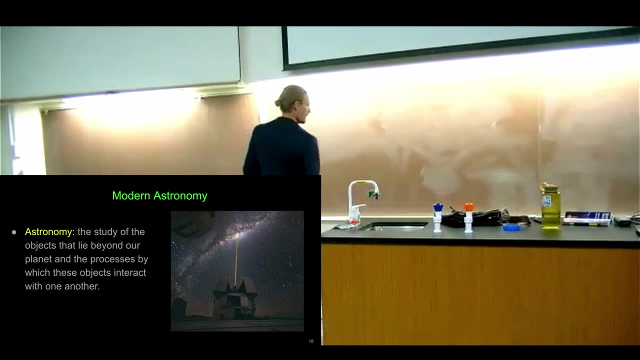 Of course, the opposite of an object, a material object in physics, the opposite is an idea. Every single word that you use all day long represents one of the two. All words represent either ideas or objects. That's something to really think about. 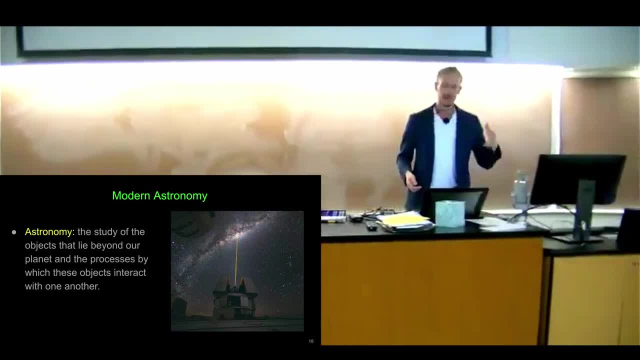 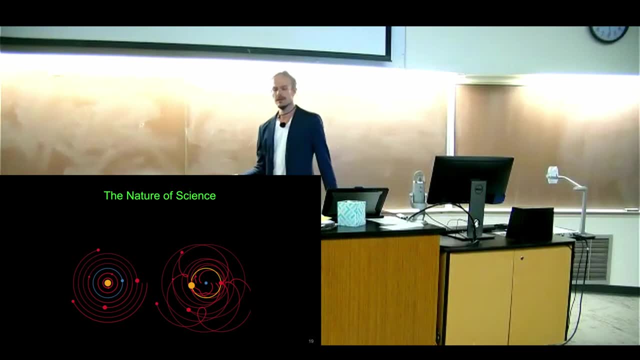 Like I said, the objects might not exist. but there you have it All right. So I mentioned I want to get into a little talk about science itself And what science is. Like I said, I think I mentioned this at the beginning. 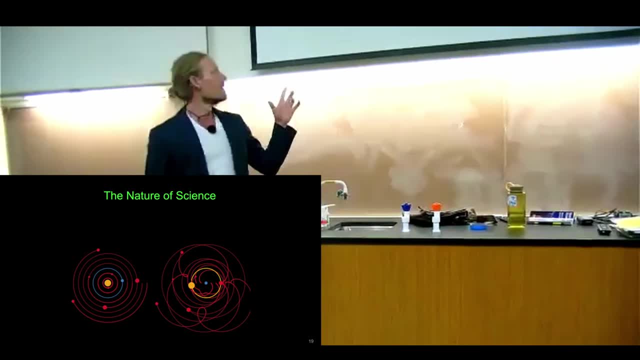 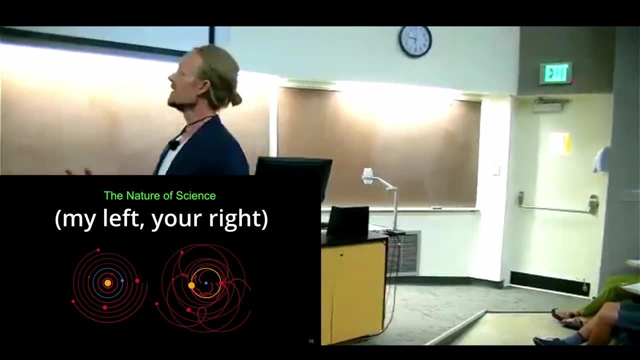 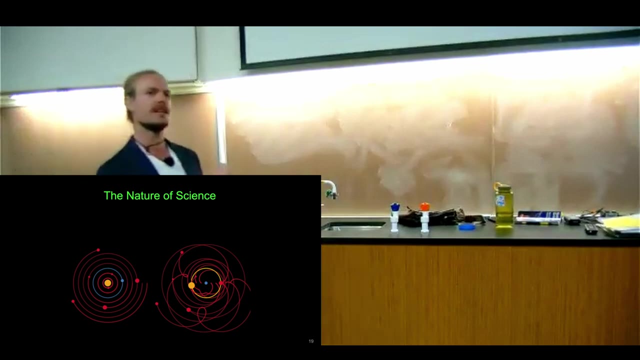 This on the left is the conception that through most of antiquity, all of the classic Greek antiquity, the Sumerian antiquity, Persian antiquity, even- from my read- the ancient Chinese antiquity, everyone believed that the world, that the universe revolved around us. 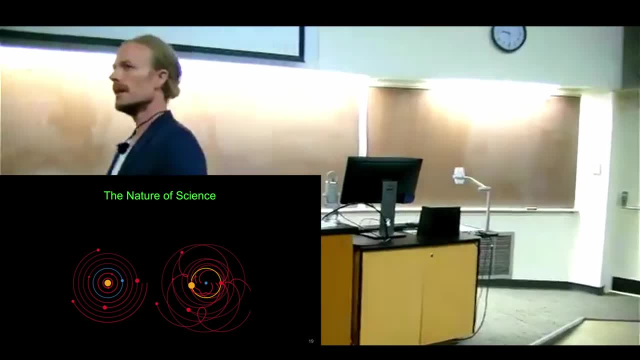 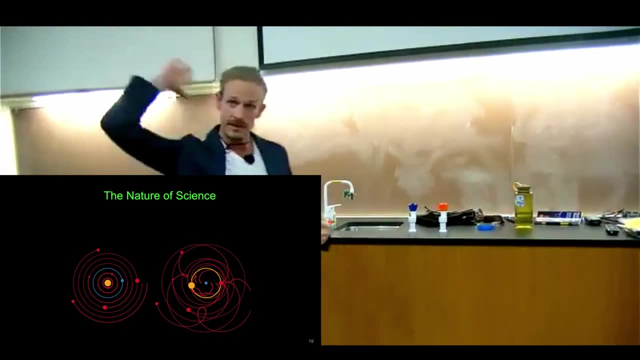 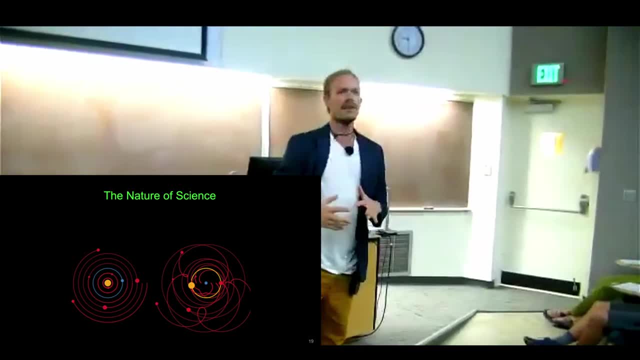 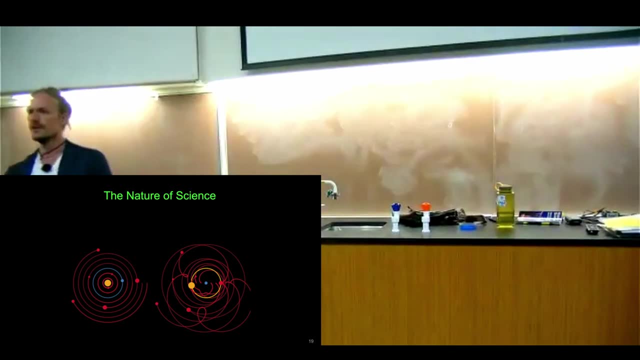 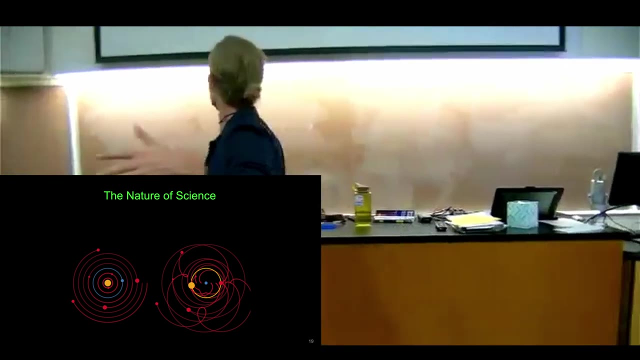 And, honestly, the more we get into modern physics, which is a very relativistic physics, at the moment, it's very much based upon how things happen in relation to the observer, And so this isn't as crazy as it seems, In fact, if you look at these two drawings. 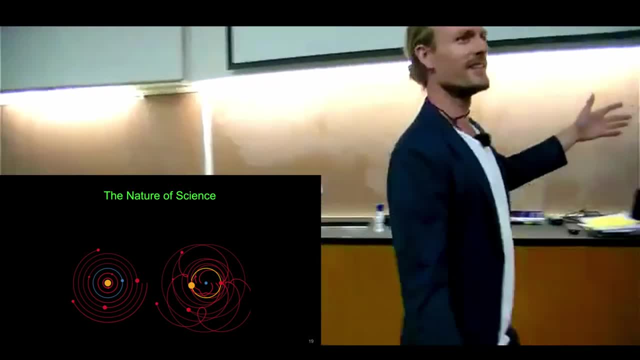 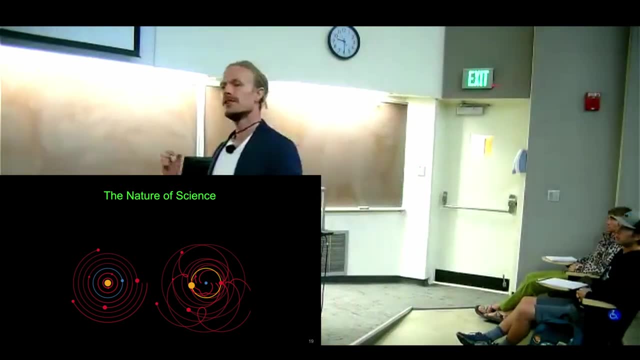 an argument can be made that the one on the left is a little more beautiful actually, And this is problematic because a number of physicists today are convinced that the measure of a good theory is how beautiful it is. But nature is not always beautiful. 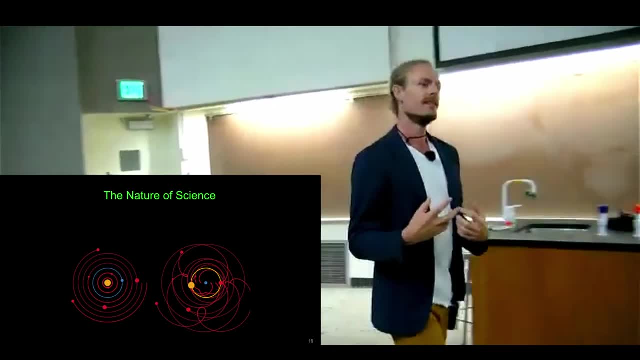 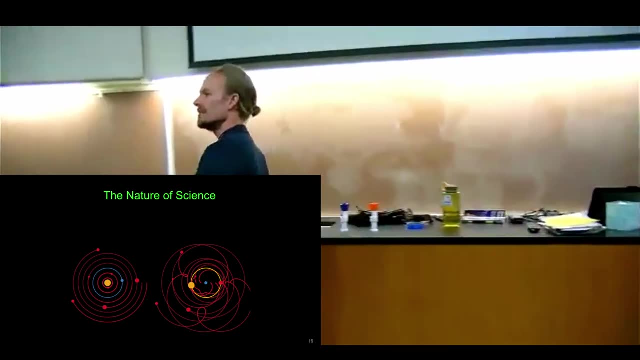 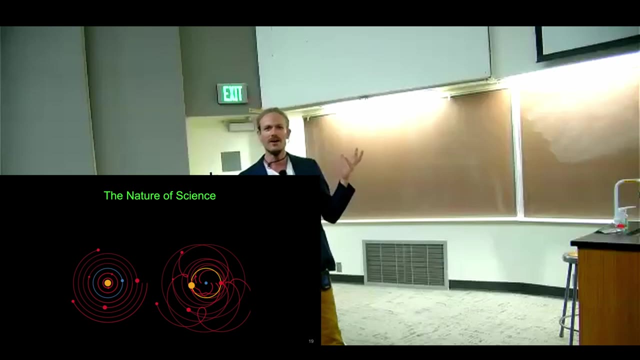 Nature can be ugly, It can be red in tooth and claw. It can be complex, It can be difficult to comprehend. In fact, I would say that the best we can do is approximately comprehend nature at any given time. Well, how did we believe the wrong thing for so many years? Because it worked. From a technological standpoint, this works perfectly- Well, not perfectly- Very, very close right, And the mathematicians and the astronomers of the day were very adept at tacking on new variables to their equations and getting it to line up with the seasons perfectly. 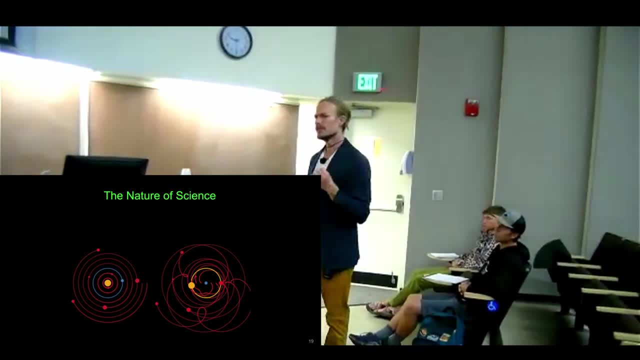 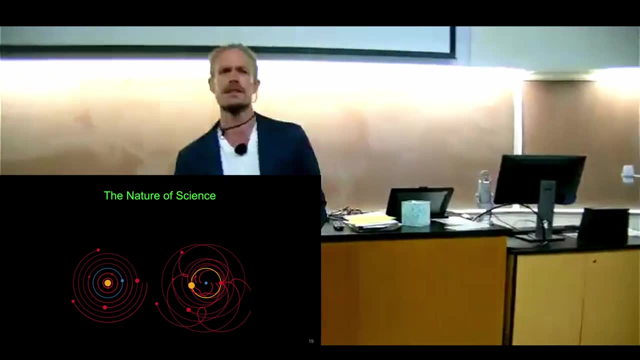 But they were completely wrong And this is extremely critical to keep in mind. as you read about our modern astronomy, as you read about our modern medical understanding, as you read about anything, you need to bear in mind that we've been terribly wrong for thousands of years. 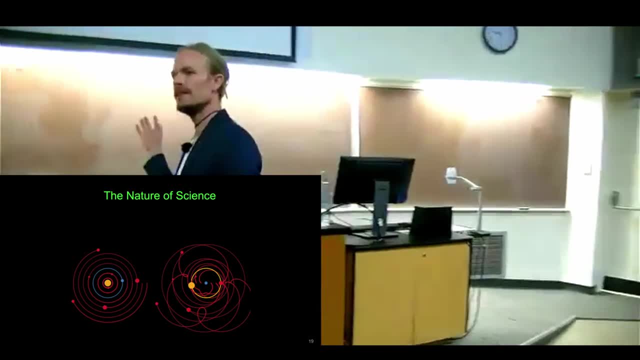 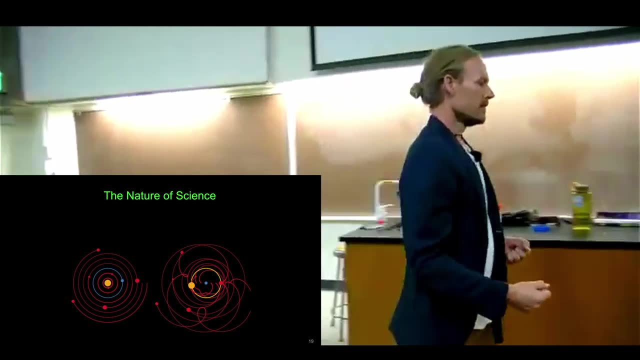 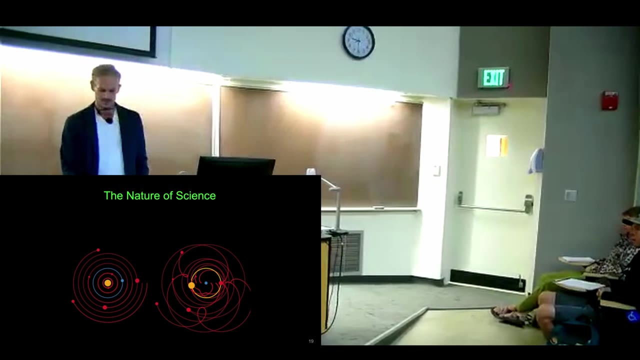 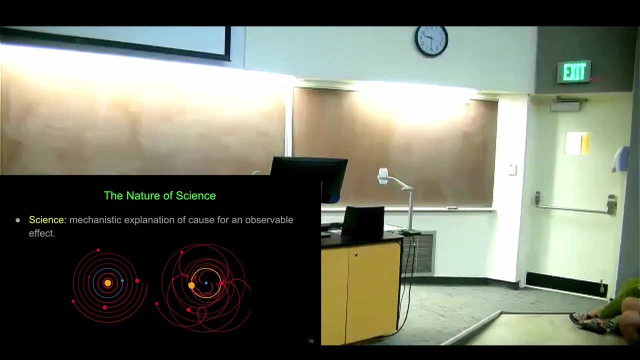 They had a very robust academy with tremendously predictive mathematics. For a thousand years they had the wrong model, But it worked. So what is science And how does it differ from this ability to predict, If we can predict the wrong thing and it works? 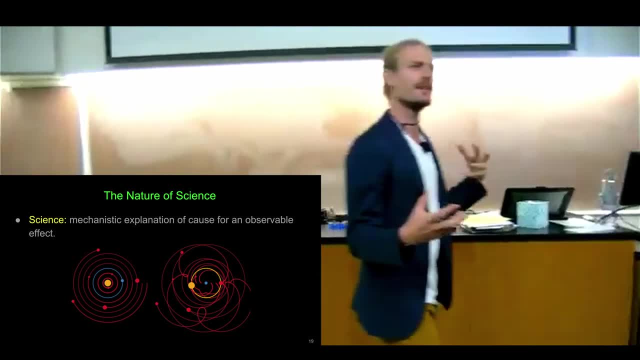 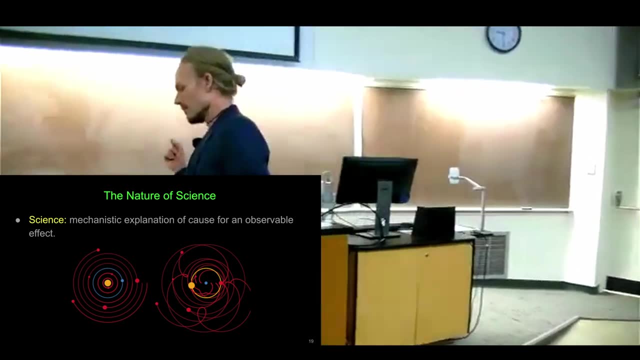 that can't be the basis of science, right? It can't be all there is to it. So you'll find some different things written in your textbook, but I think that it's important to complement these with the concept that I've written here. 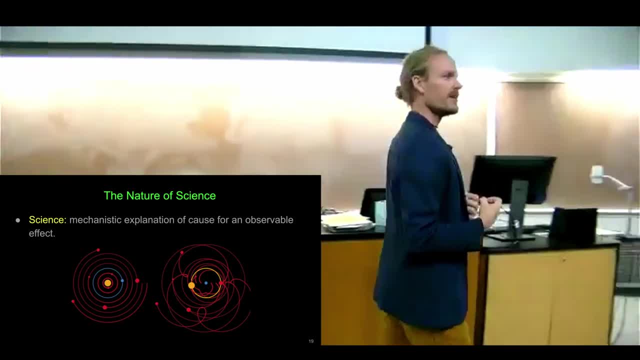 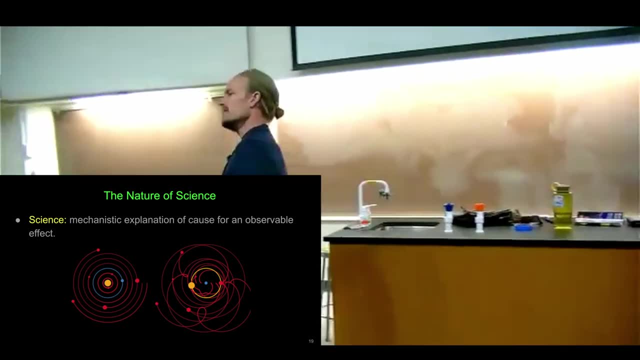 Science is a mechanistic explanation of cause and effect. It's how the objects, the material objects, interact with one another to produce an effect. That doesn't mean that it's right right. It just means that it is an explanation that can be understood. 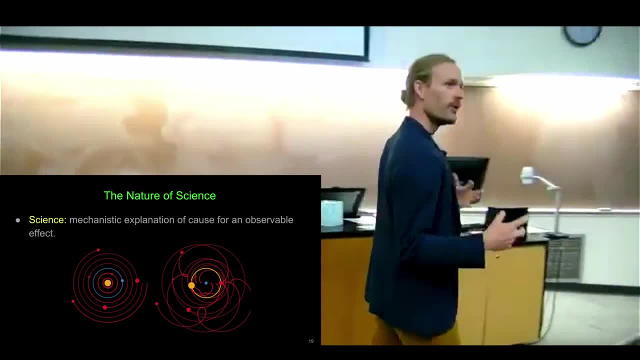 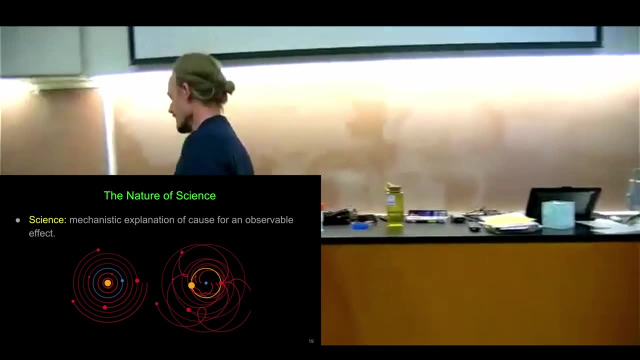 The only way to figure out if it's right is to find holes in it Or- and usually both- to make a new model that works even better, And that's what happened, which we're really going to do a lot of next week. 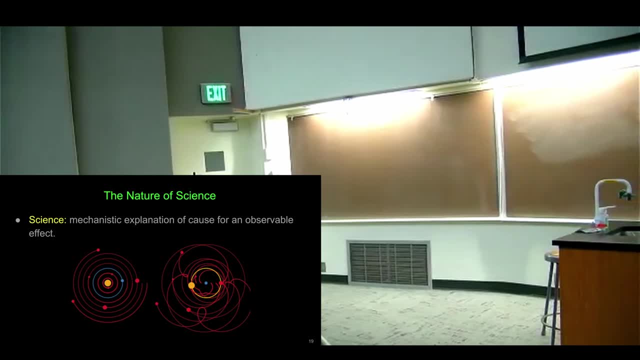 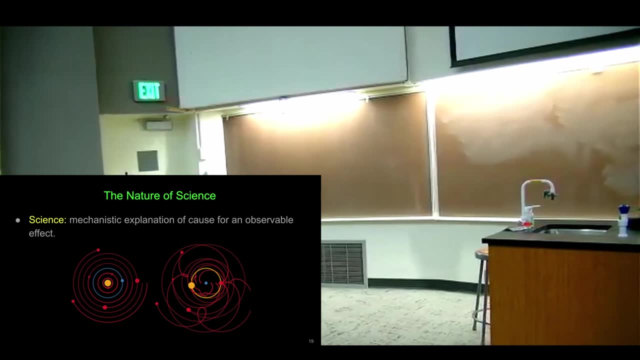 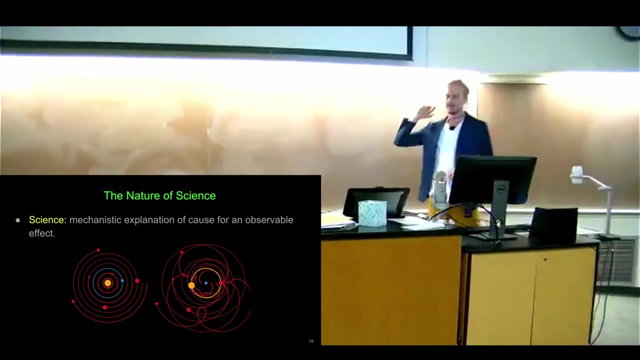 is how we came up with this model on the right over here. eventually, It was easier And it resolved a lot of the tiny little nudge factors that we needed in order to make this one on the left work. So, again, both of these are scientific explanations for how the stars work. 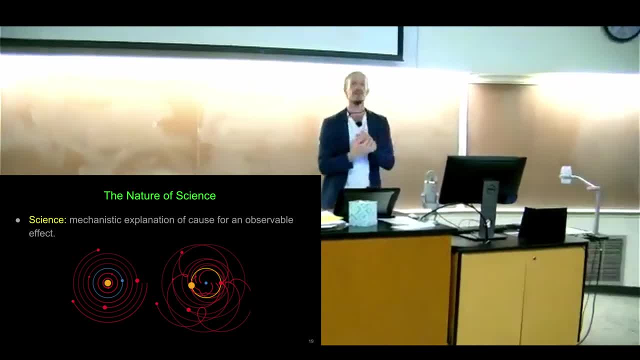 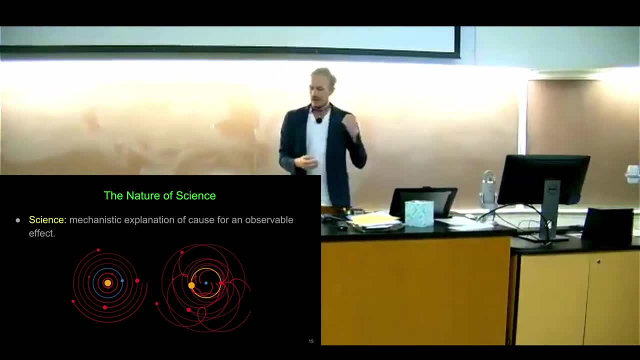 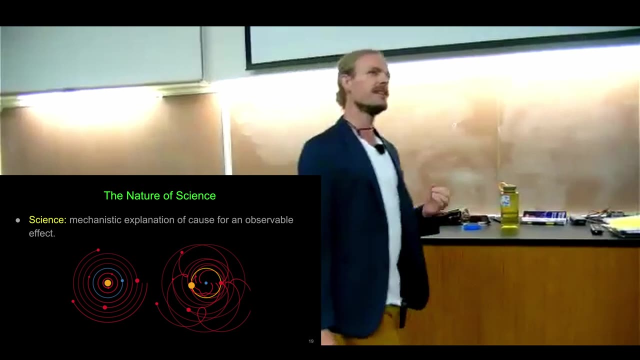 They both involve objects doing things with respect to one another, interacting with one another to produce what we see. Okay, So you know, a very popular phrase has been: trust the science right. It's not so clear that that's how it should work, though. 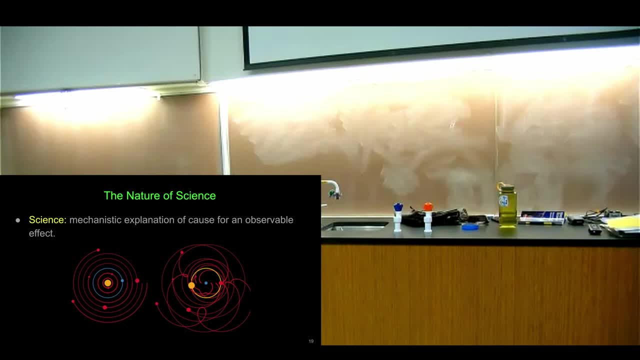 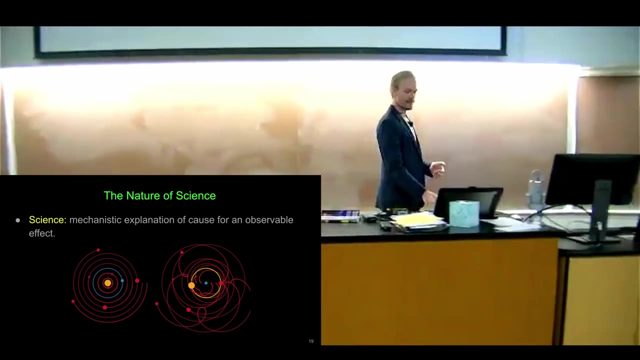 It's much more clear that what you should trust is that this is one possibility. Are there others that you can think of? that would be better. Perhaps Is there a problem with the theory that's before you? Perhaps, And if there is, then it's probably time to start looking for new ones. 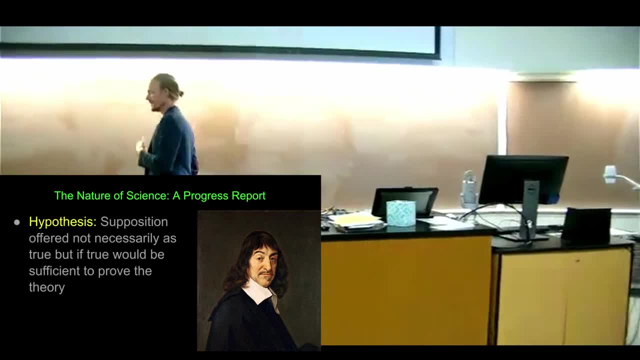 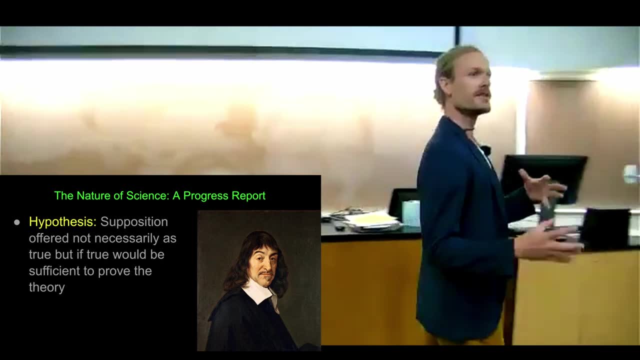 So there's one of these big words that you see here in science all the time And again. I think it's really important to sort this out- One of these explanations, whatever it is, let's say, the geocentric model. 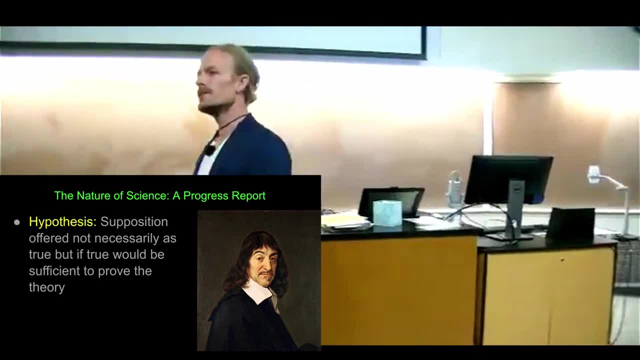 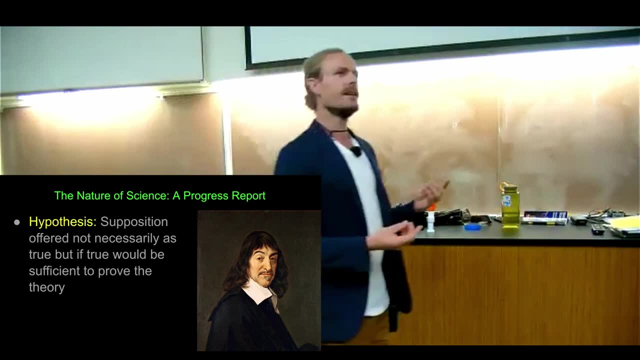 it was a theory. What's a theory? It's an explanation. So, if a theory is an explanation, what's a hypothesis? Hypothesis is what makes your theory work. It's the piece that you don't know of for sure. 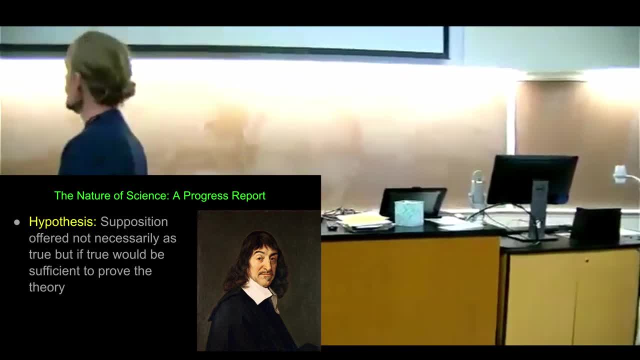 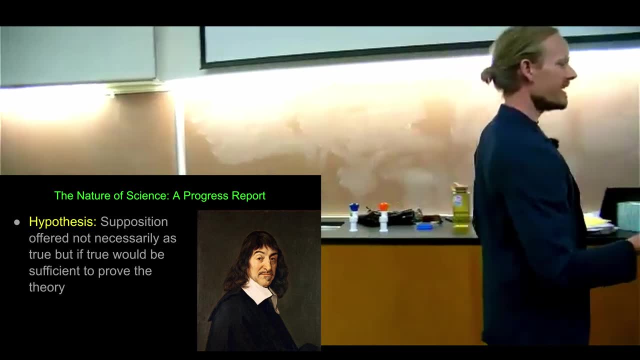 You can't really figure that little corner out. but you say, hey, you know what? I don't know where the Earth is with respect to all of this, but let's hypothesize that the Earth is at the center of the universe. 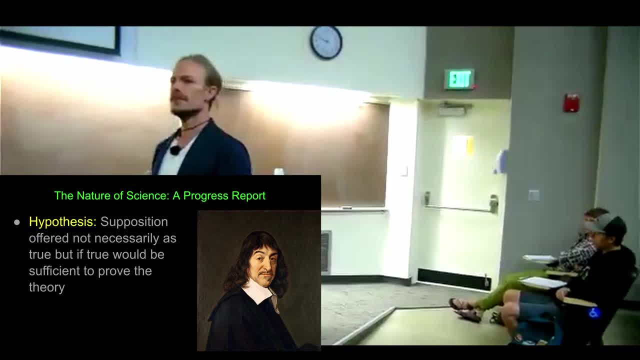 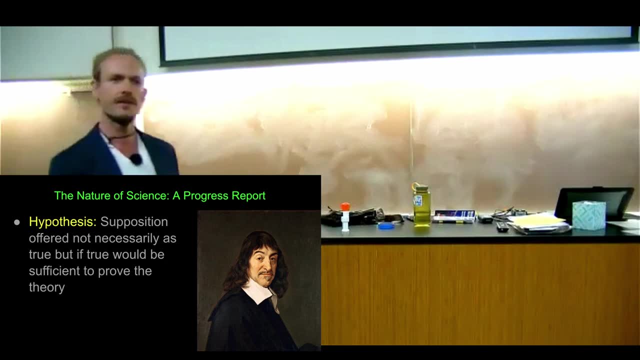 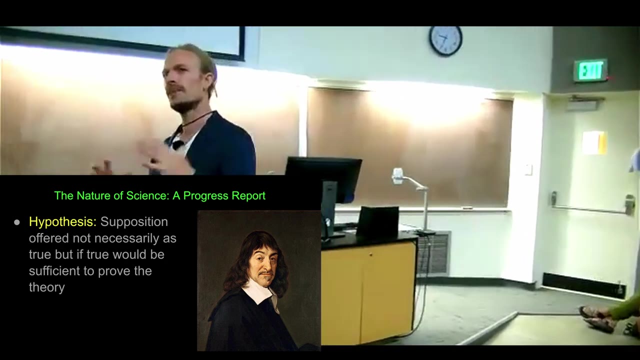 If it is at the center of the universe, then that's sufficient to prove my theory of how the solar system is laid out, which was the crazy looking one in the previous slide. So, the hypothesis being that the Earth is located here, that explains the motion of the heavens. 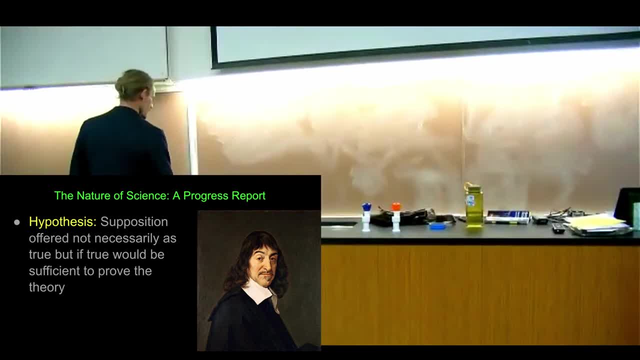 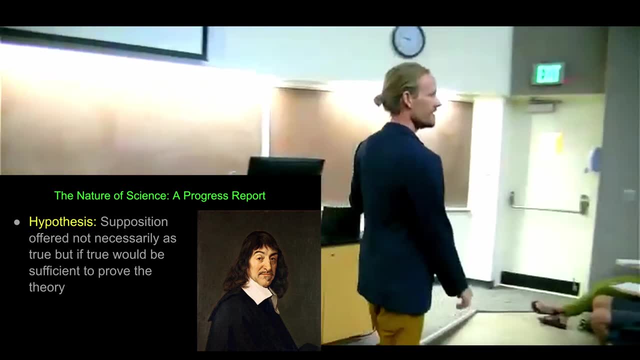 So this is Rene Descartes, who was one of the early Enlightenment thinkers. I quote him. I quoted him here because I think this is a very succinct way of describing what a hypothesis is. You probably won't find this in any of your scientific classes. 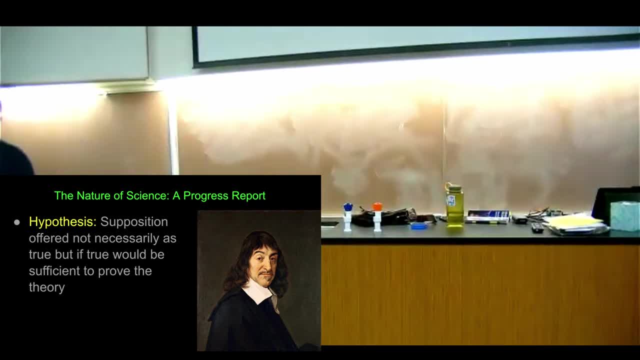 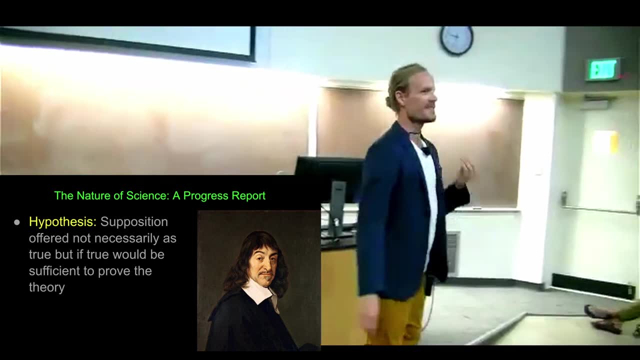 because the idea of a hypothesis has been largely confused with the idea of a theory, and I think that's a terrible disservice to all of you. A hypothesis is a supposition which is offered as not necessarily true. but if it was true? 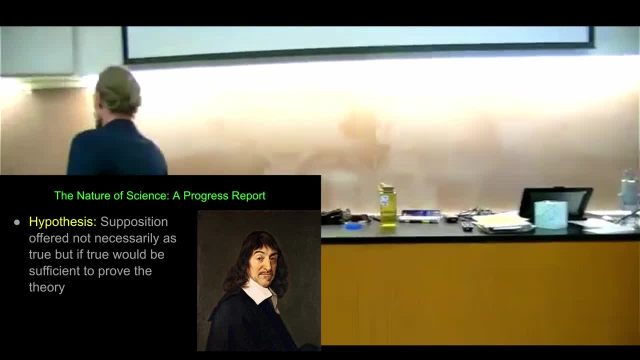 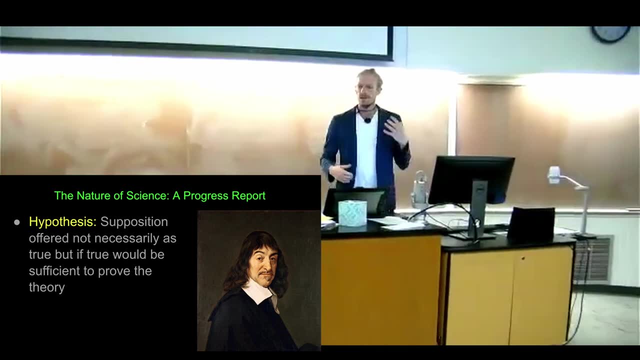 it would be sufficient to prove your theory. So- and we'll see why- this has been confused with theories and predictions and all of this. It's a real mess. but if we separate out all of these ideas, we can actually get somewhere. 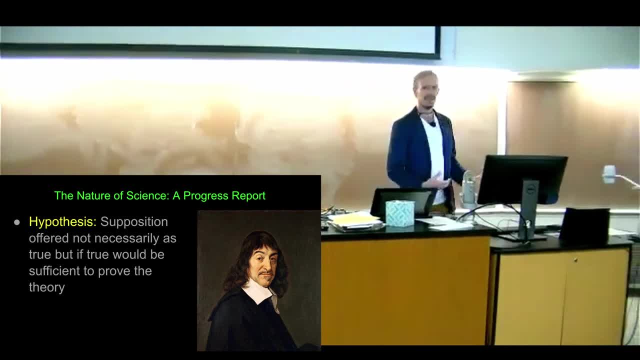 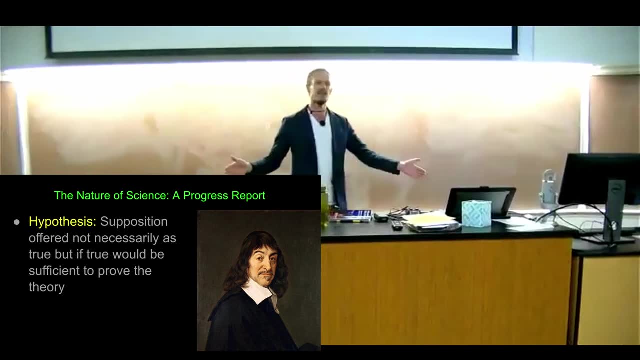 and I think we can have a better appreciation for what science actually is and how it stands with respect to technology. You know many universities have a science and technology department. Why do they say that, if it's all just the same thing, They're not the same thing. 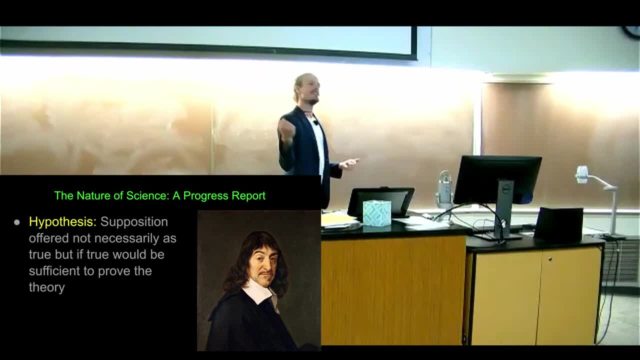 They're very different actually, And we live in a very technologically driven civilization. In fact, if you're a research scientist, it's almost impossible to get funding to do basic science. If you just want to know how something works, forget about it. 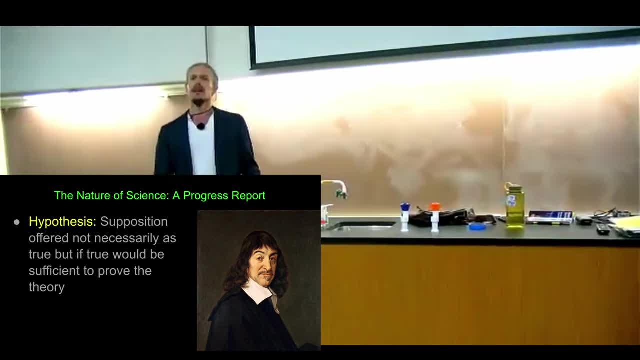 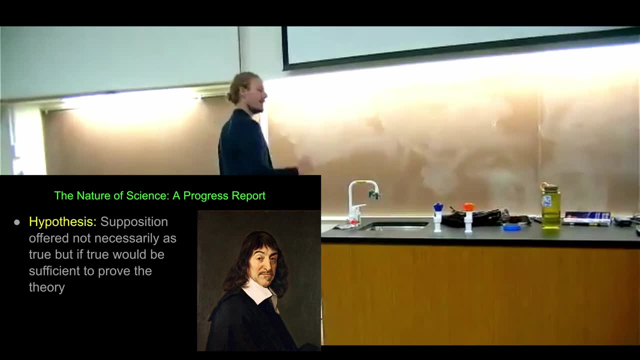 You need to tell the government or whoever's funding you, not only why you're going to study, why it's cool, what you want to study, but you need to tell them how you're going to instrumentalize it right, How you're going to do something for humanity with it. 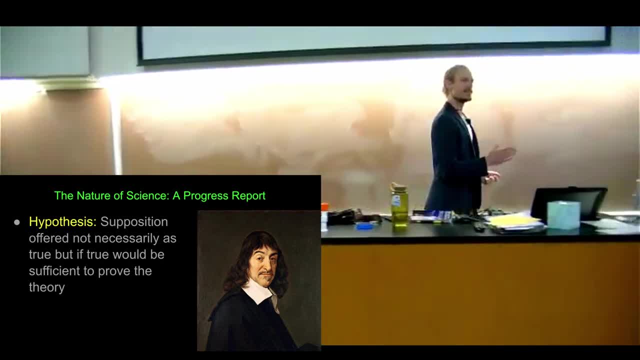 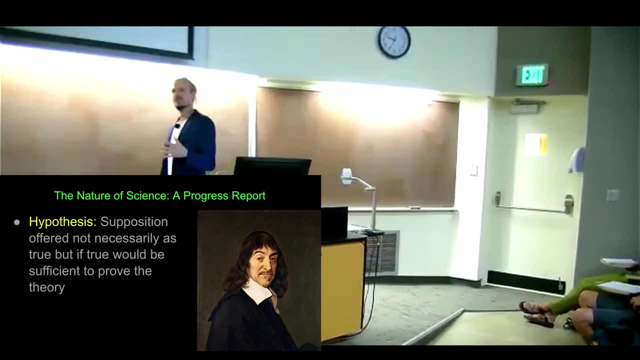 and that's the technological side, And sometimes, if you're purely motivated by technology, you might not be looking for the answers. that won't give you technological solutions, and I think that's led to a number of extraordinary blind spots in the history of science. 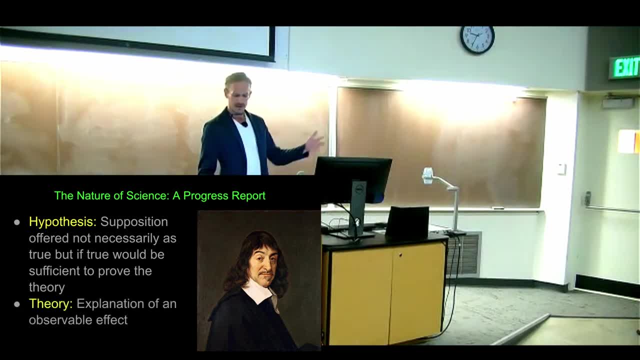 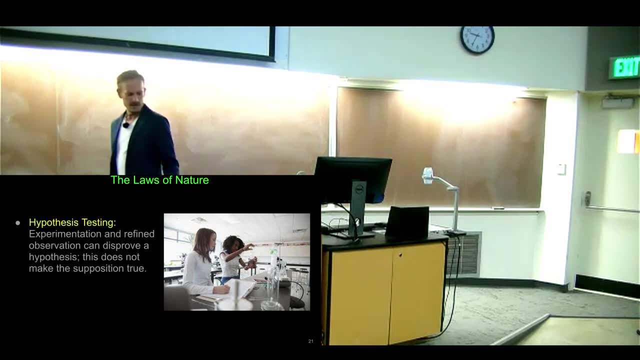 and we'll see those as we go through this course. Again, a theory is the explanation of the effect. All right, so what's a law of nature? Well, let's go back for a second. So laws precede both science and technology. 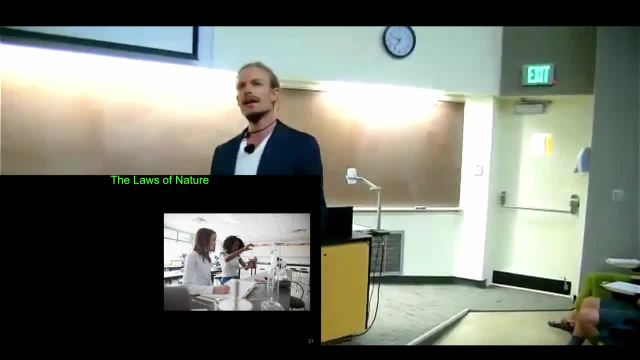 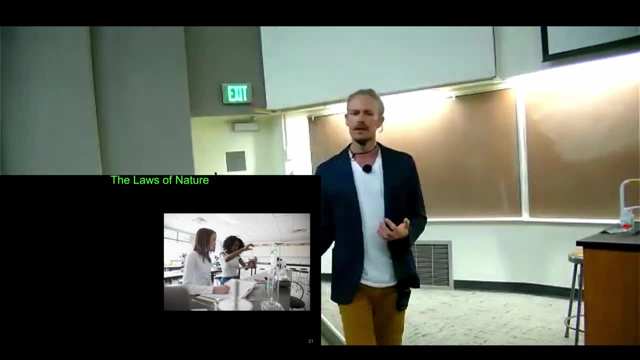 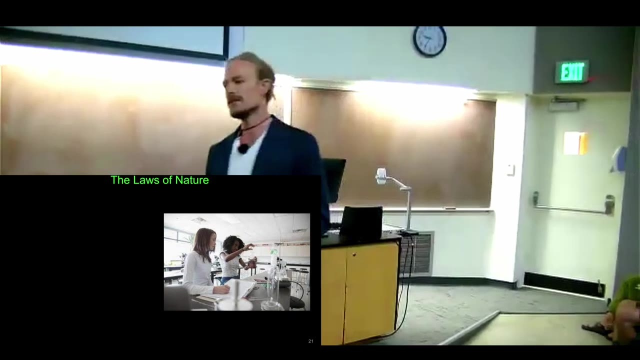 both hypothesis and theory. The law is simply a quantitative description of how things happen. That's it okay. So you know, an infant understands gravity, right? An infant understands that if they push a ball off of a table it's going to fall in a predictable fashion. 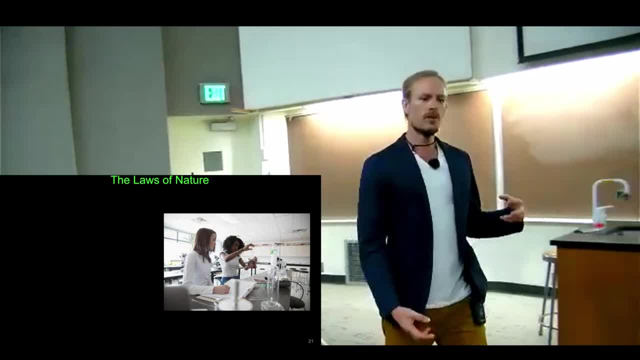 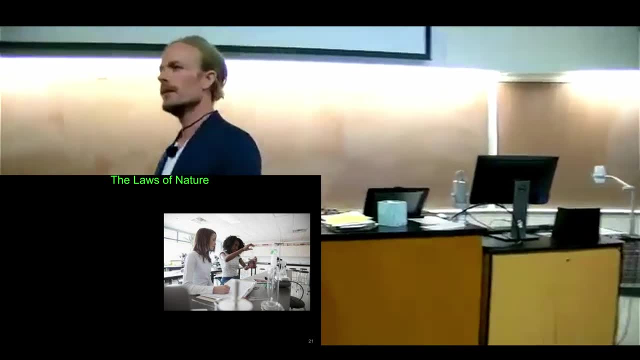 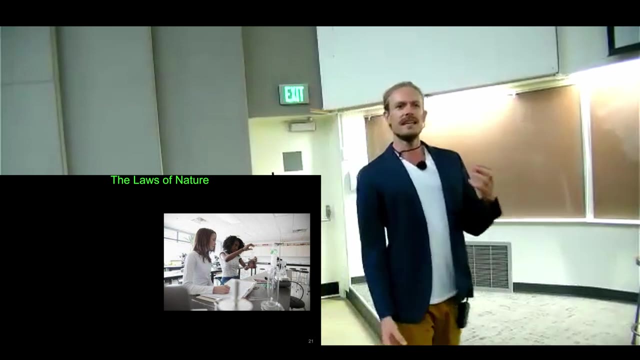 It always does it the same. So what the different thinker classes of people over the years have done- and particularly since the Enlightenment with all of this Newtonian dynamics that you're all probably well acquainted with- is they have ascribed the quantitative patterns. 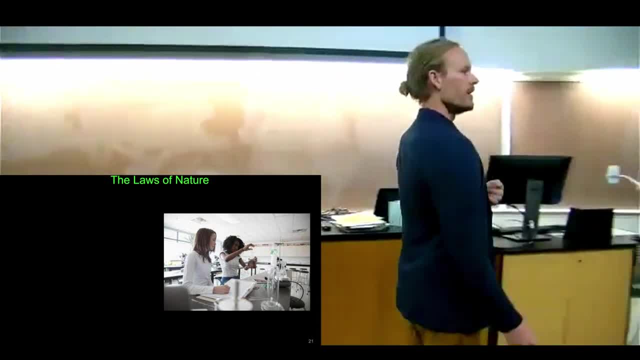 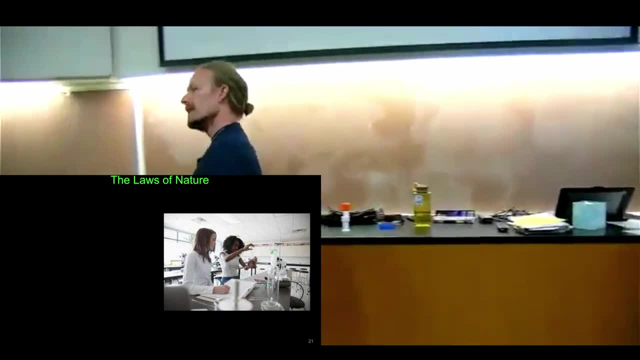 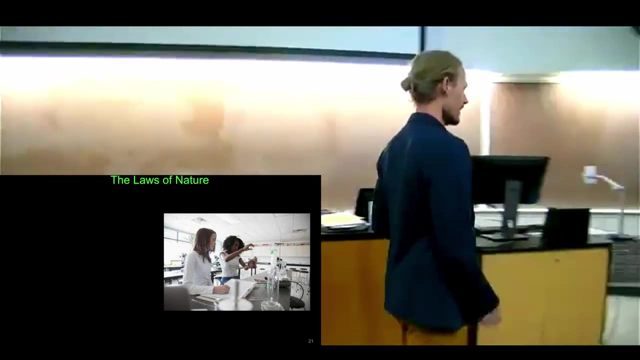 to those phenomena. So, gravity, Things fall off a table. Well, it turns out, they fall off the table the same way every time, And the way that it falls has to do with all sorts of things, right, And we can parameterize that and create laws out of them. 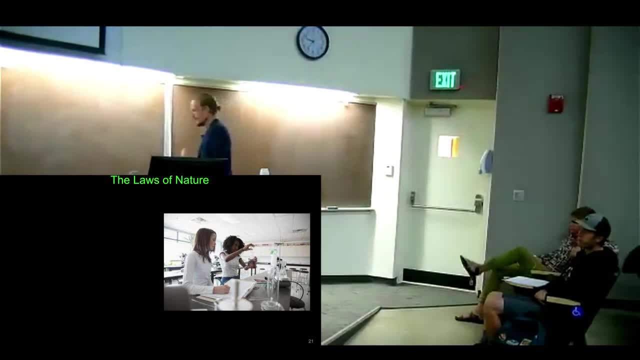 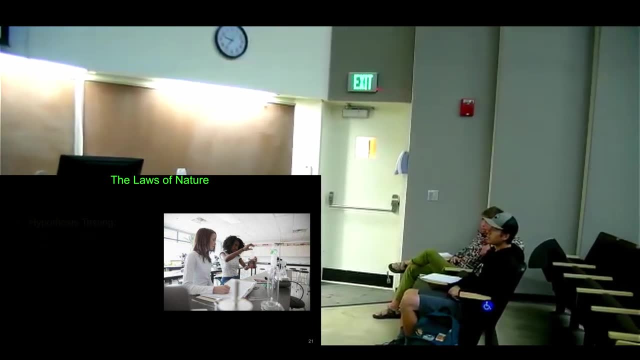 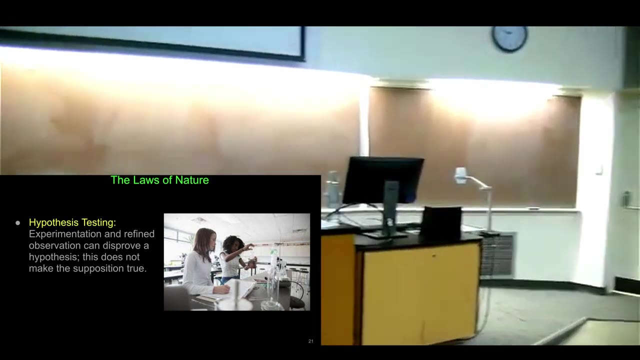 And the laws have some sort of symmetry with respect to one another. We can learn from one law, we might be able to learn how other things work And, of course, by putting things into laws, we can then be able to start to ask questions about. 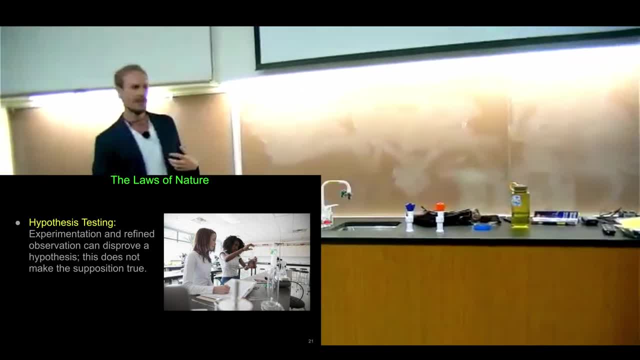 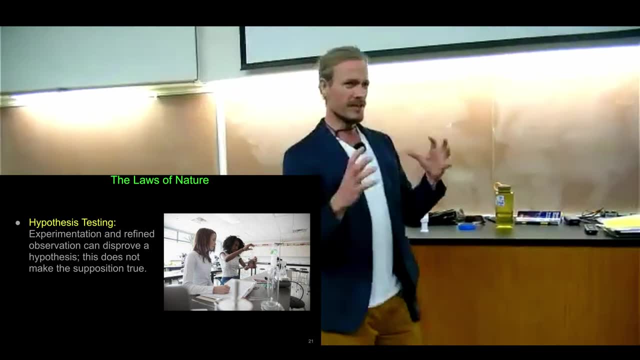 well, if this is exactly how this works, if the Earth is actually at the center of the Universe and we can describe that motion with this relationship, an equation, then we can begin to ask questions of it, We can begin to test that hypothesis. 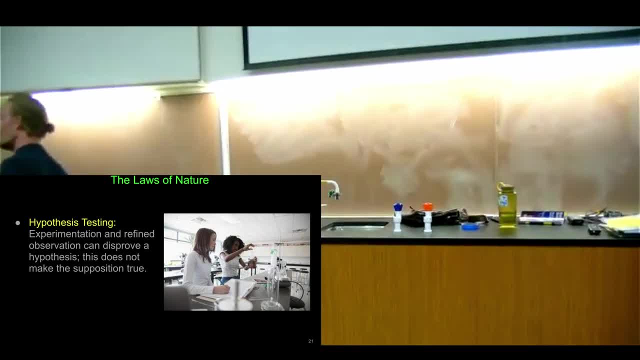 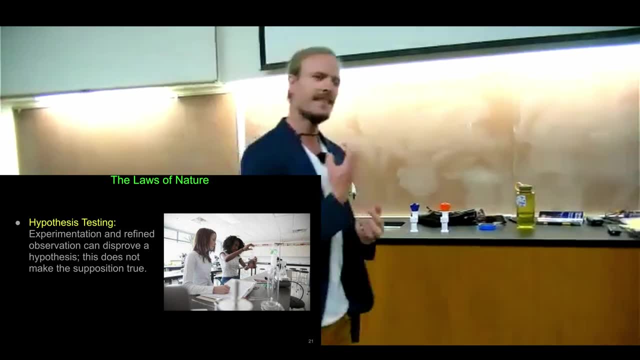 And this is really important in terms of getting rid of bad laws that don't actually work- And we're going to see a number of them fall by the wayside in this course- Getting rid of bad theories, right. So ideally, when a theory 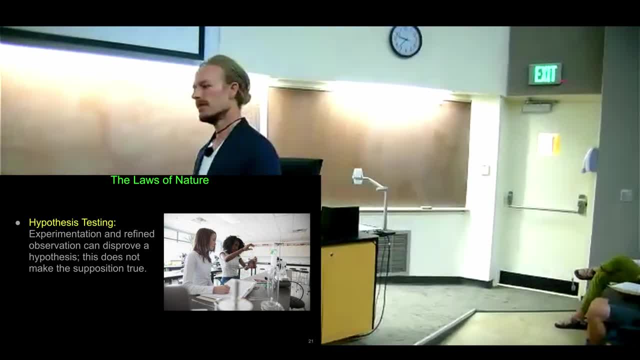 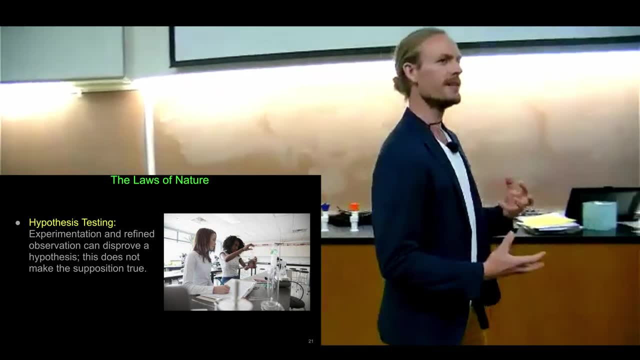 has an observation that contradicts it, the theory gets thrown out. Of course, this isn't how it actually works, unfortunately, Perhaps. unfortunately, perhaps it's because it's a very stable bureaucracy, Right? You don't want the whole of science being thrown out. 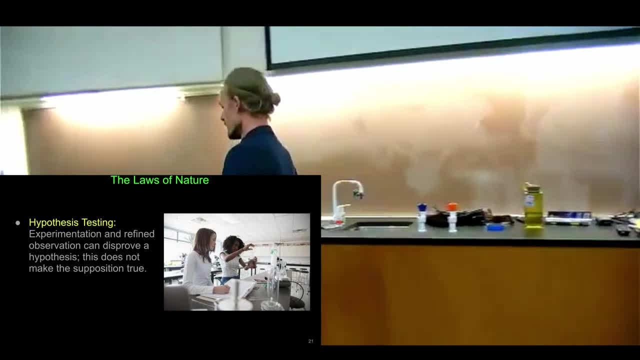 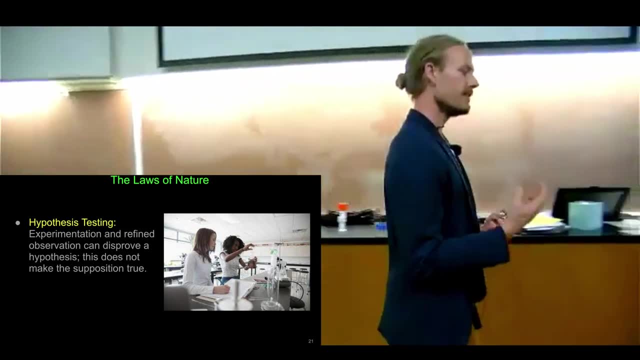 because something doesn't make sense all of a sudden. So epicycles get tacked on right, The laws get adjusted, The theory gets adjusted, And often the theory can be adjusted for many, many years, maybe thousands of years before. 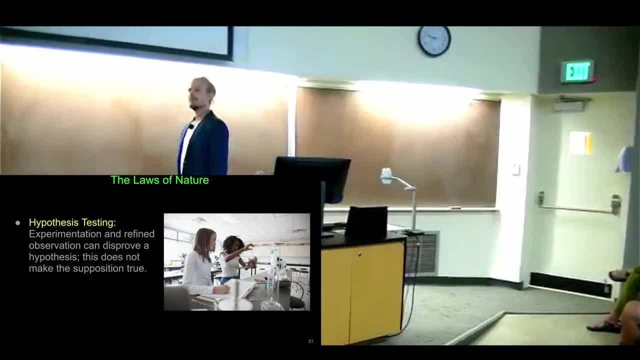 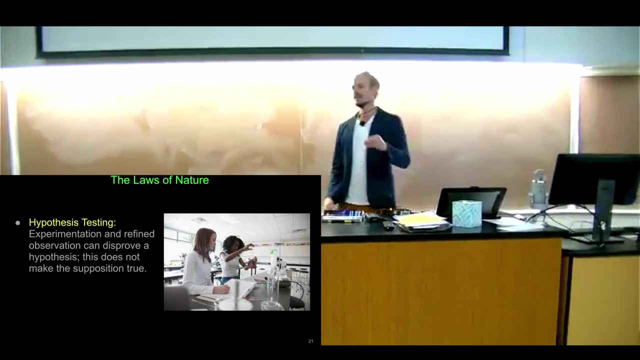 it finally comes to the point that somebody has a better idea And they say: you know what? This is way too complicated, This is just nuts. What if it just works like this? What if we just stick the Earth over here and the Sun over here? 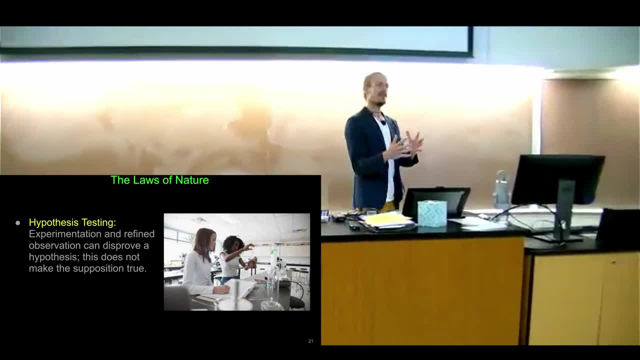 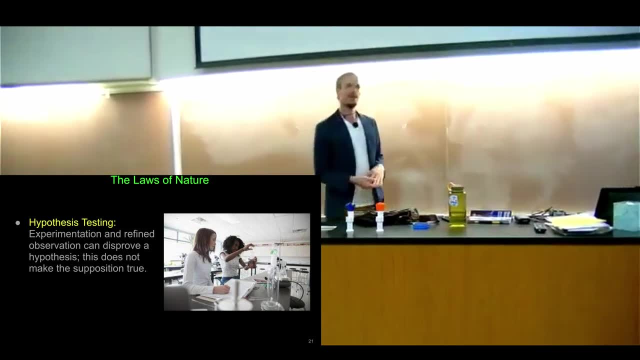 Well, now our equations simplify down. Now we don't need to add all of these different orbits. I don't know if it's correct or not, but it's easier and it seems to make sense to me, And people by and large eventually say: you know what? 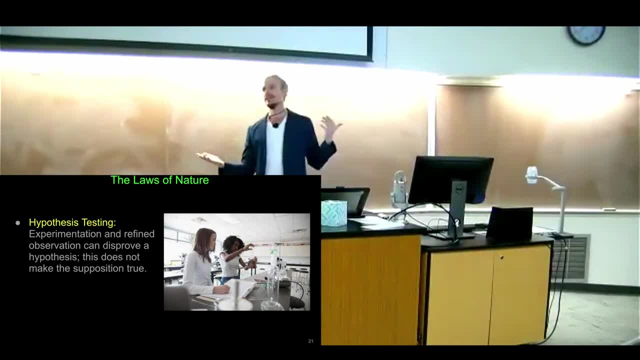 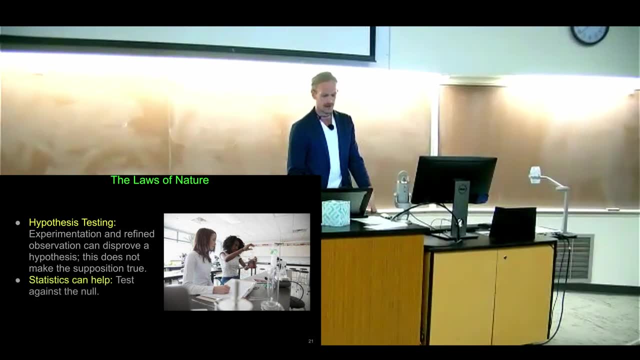 I think you know, I think that makes that works. for me anyways, That's a lot easier to remember. It works So you know, and today we used statistics to figure a lot of this out. We tested against the possibility that. 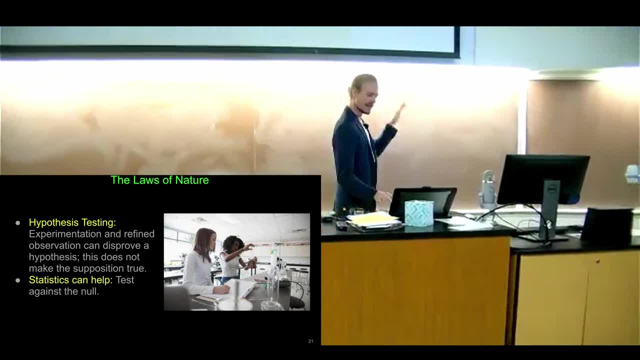 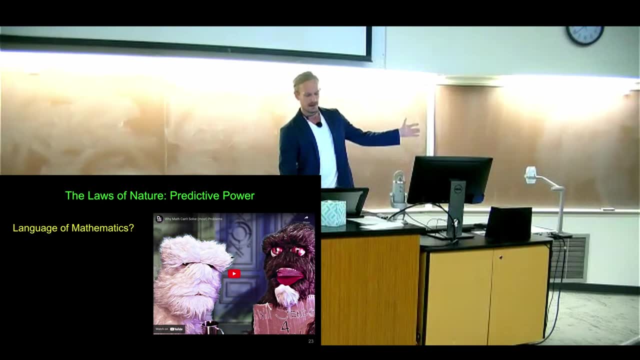 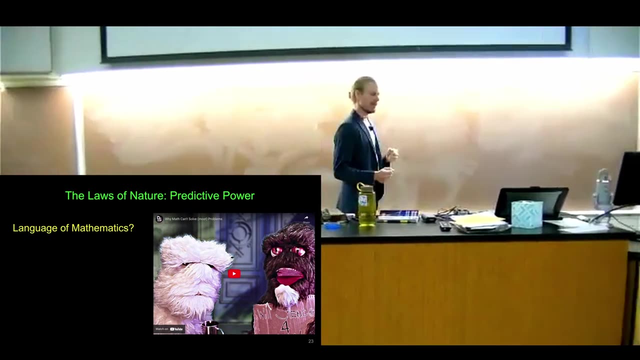 the phenomena is just due to chance. This isn't entirely important for right now. I just want to mention it. So, oh, it's often said that the way that we describe these laws is in the language of mathematics. Okay, Now. 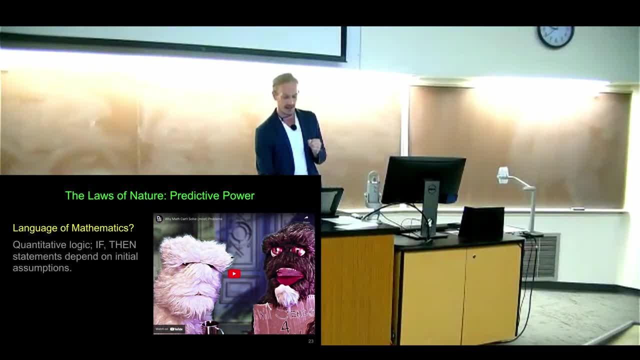 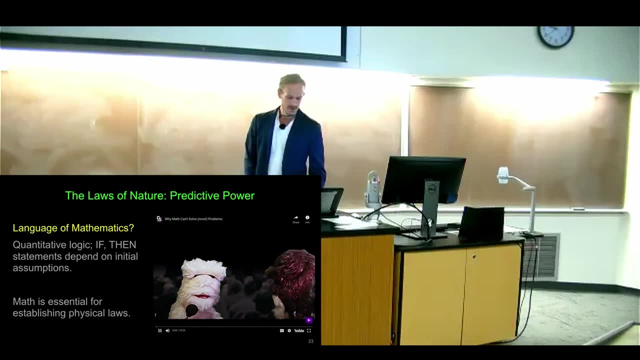 there's some problems with thinking about this. I actually put a. I actually put a video. I'm going to pull it up first. Oops, I don't actually want to play this yet. All right, I made this little, but if I could only stop it. 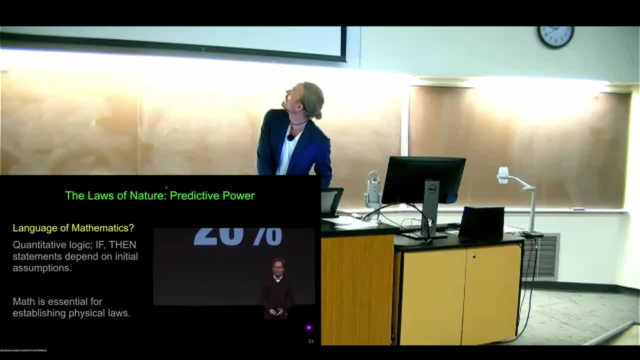 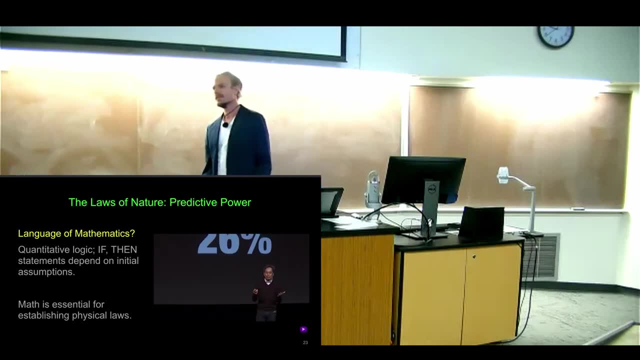 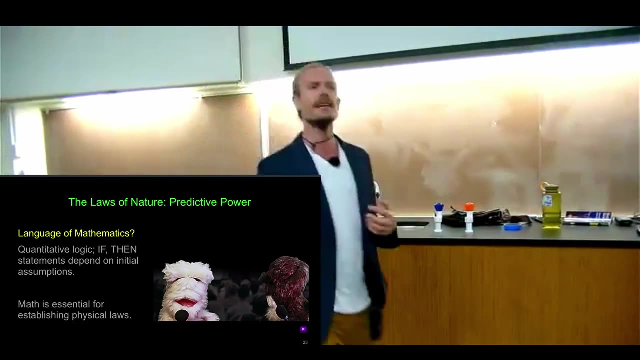 Okay, Look, I made a little movie about this. I want you guys to watch it. It's in your watch list. My wife and I did this. We used little puppets that are alien scientists and we're investigating the idea. Is math a language? 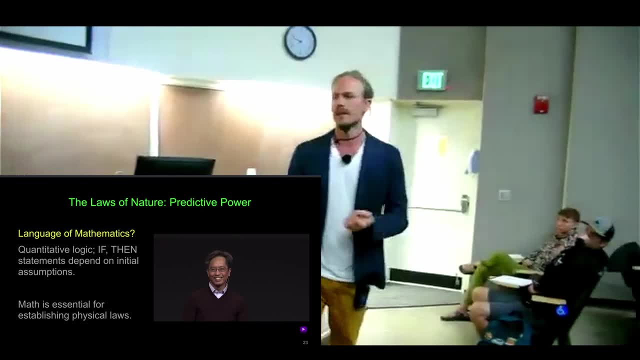 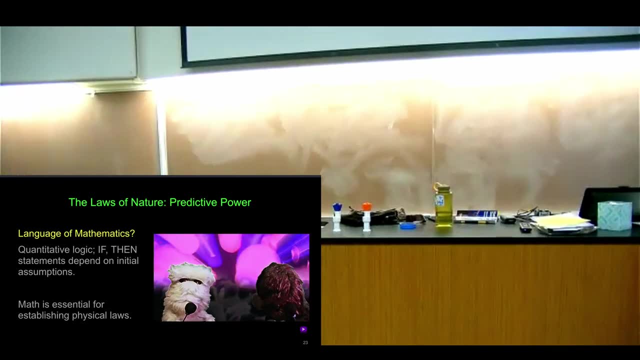 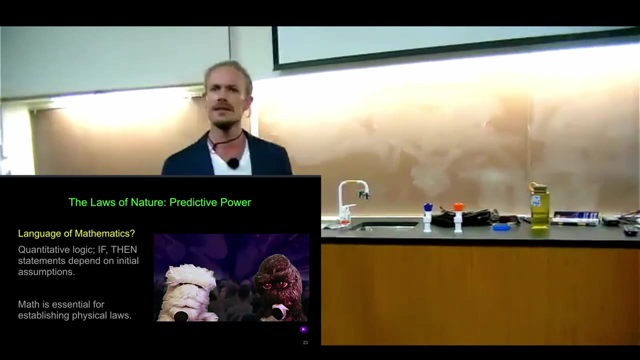 It might seem trivial, like who cares if math is a language or not. Well, I think that the fact that we treat math as a language when it is not a language has led us to make some very difficult confusion between what an explanation is. 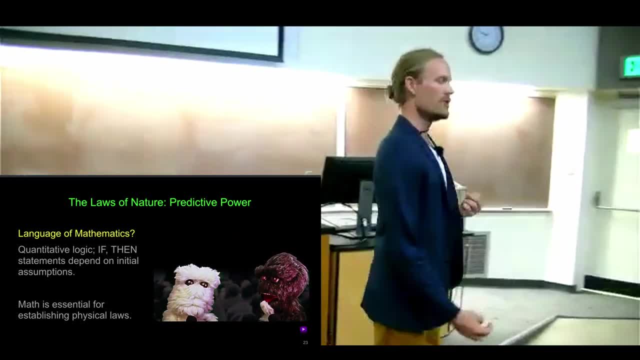 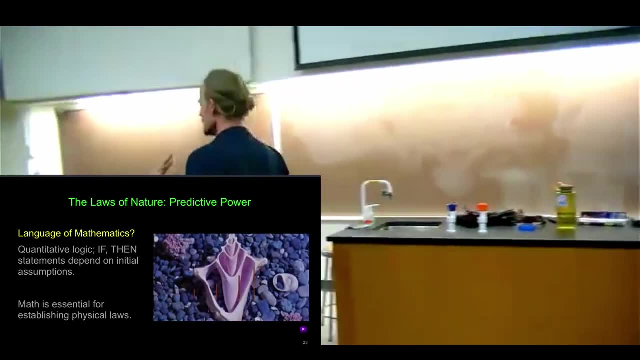 and what a law is Okay, Because just because I can make a law for how the planets move doesn't mean that I understand how the planets move, And this is becoming a really big problem in fundamental physics as well as astronomy, right. 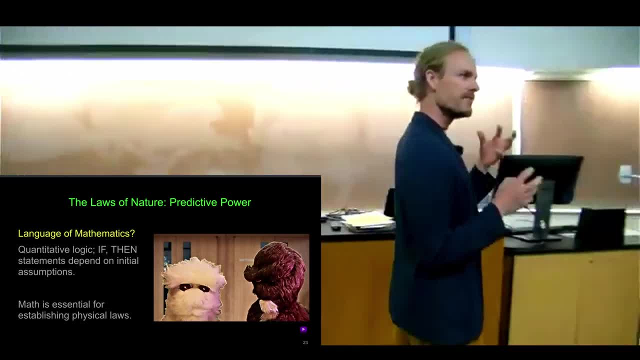 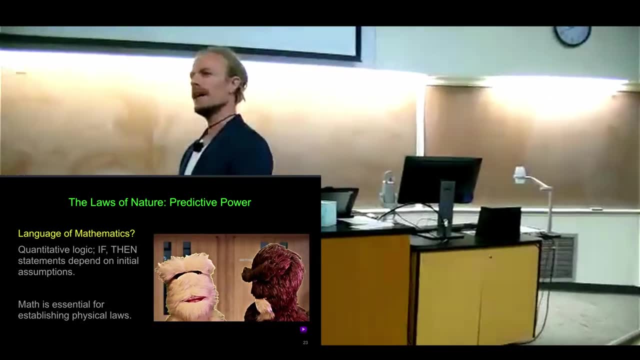 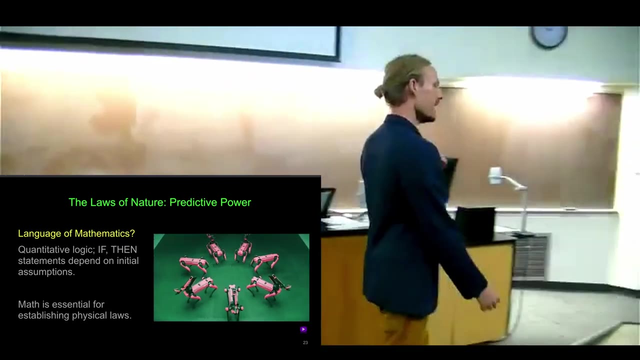 We have incredibly powerful laws for the way that quantum behaviors unfold, But we don't have a real mechanical picture of the atom. You can't draw me a picture of an atom and tell me how it pulls on another atom to produce gravity, And I think this comes down to our obsession. 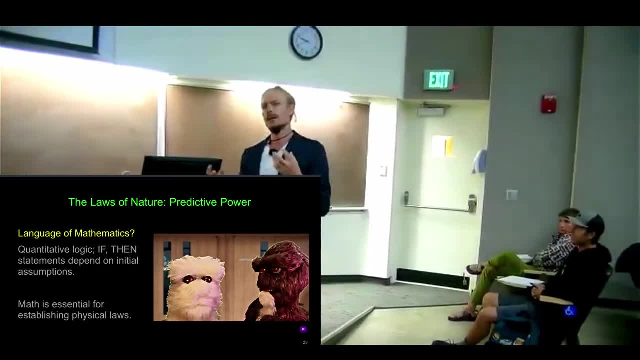 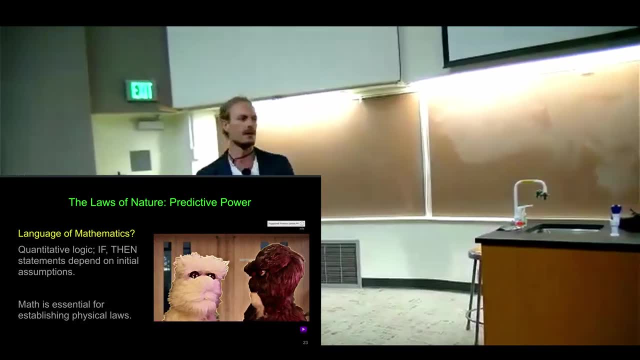 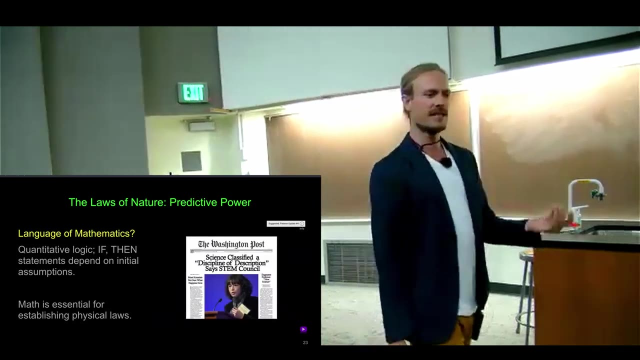 with the predictive power of these laws right, Not to say that that's worthless, That's extraordinarily important for technological- you know the magic of technology for these laptops that you're using. They all rely upon laws right, Which are predictable behaviors that we can tweak. 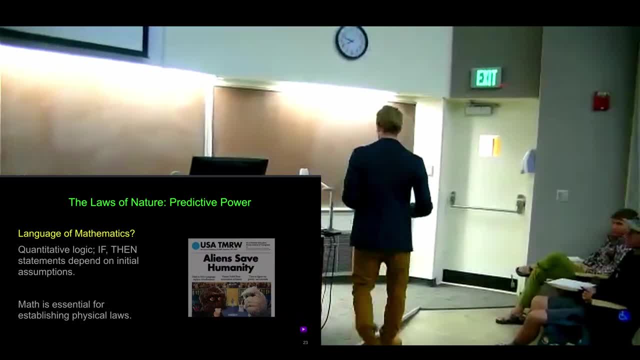 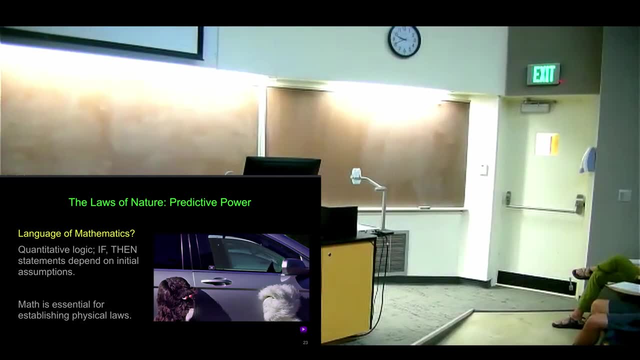 But they don't explain anything about it. Right, You don't actually have to understand how your computer works. In fact, if you're concerning yourself with how your computer works, it's probably broken. That's the only time you'd be worrying about it. 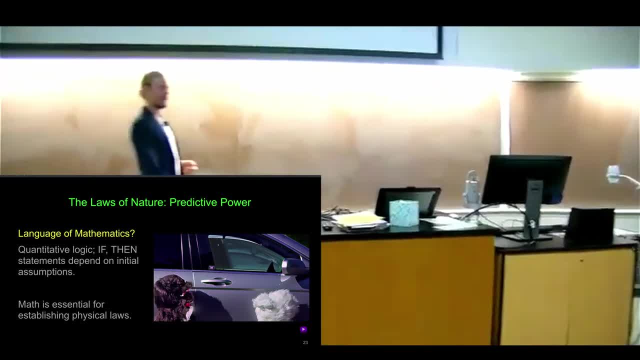 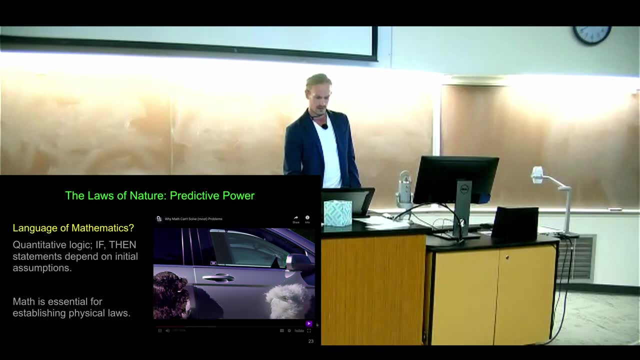 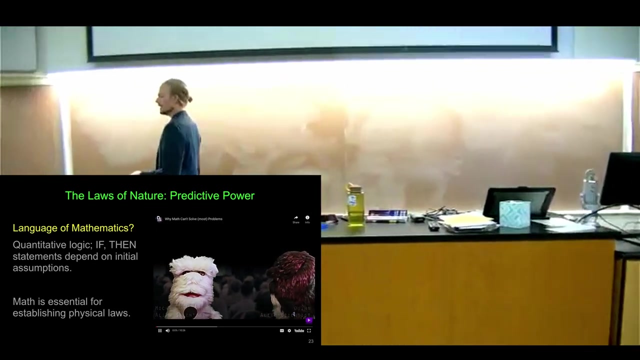 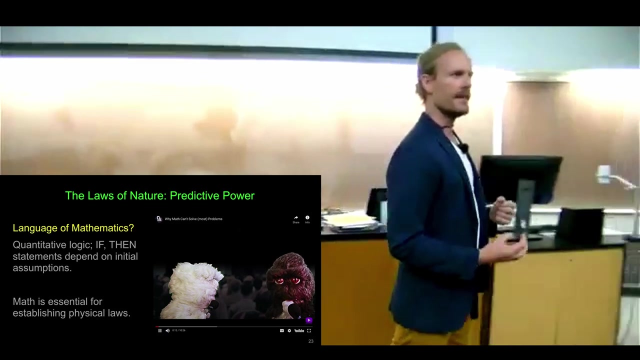 Otherwise, you're just interacting with material, And that's best So. So math is actually quantitative logic, And what that means is that it's a series of if-then statements, Right, And the problem with if-then statements is that they require you to make assumptions. 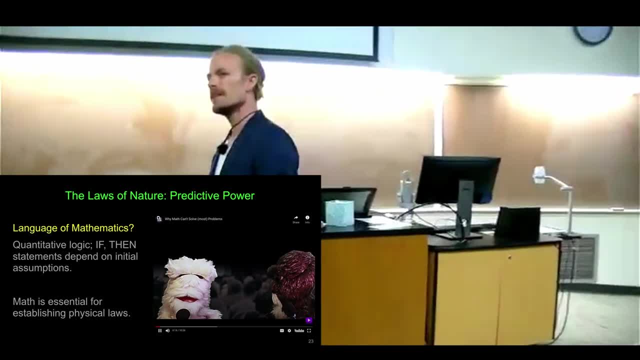 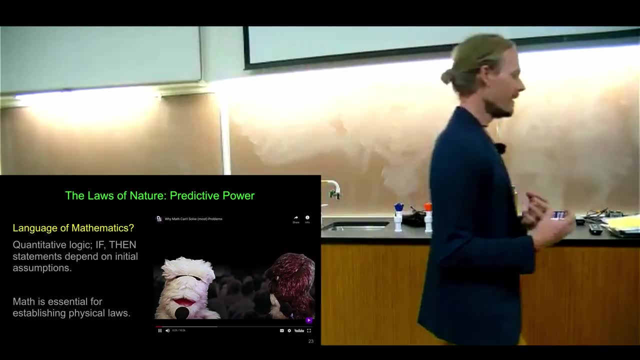 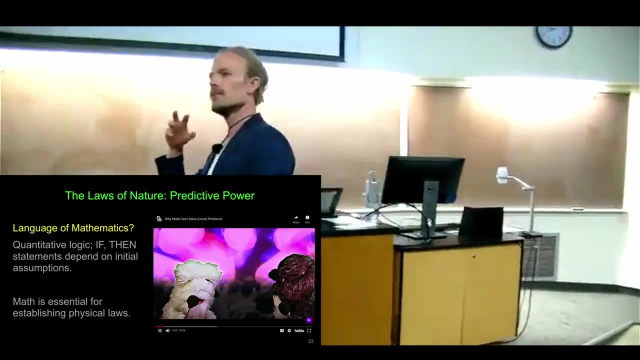 Let's assume this is the case, And if it is the case, then we can make all of these deductions downstream from it. That's fantastic. It's wonderful. It allows us to make these computers, It allows us to understand how things will. 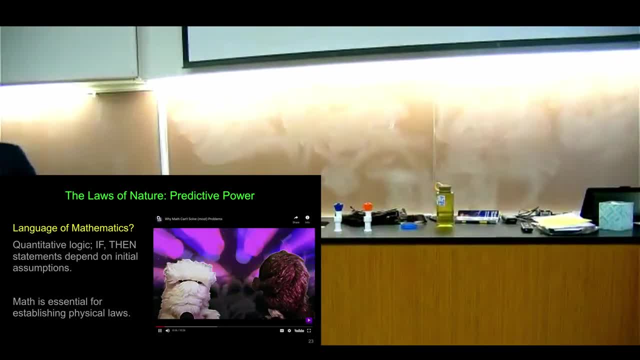 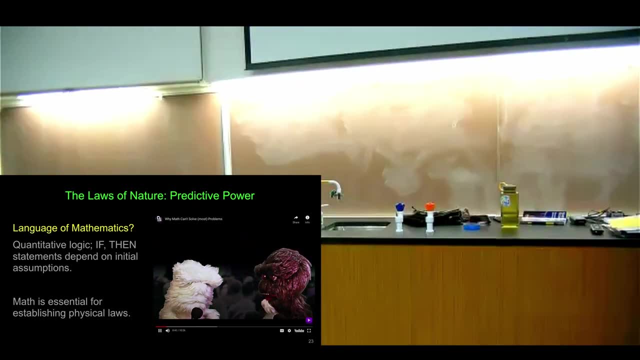 unfold if we launch a spaceship into the sky, But it's never, ever going to explain anything to us. Okay, So this isn't going to be a very math-heavy course. There's a little bit of math, And I think that's really important, because 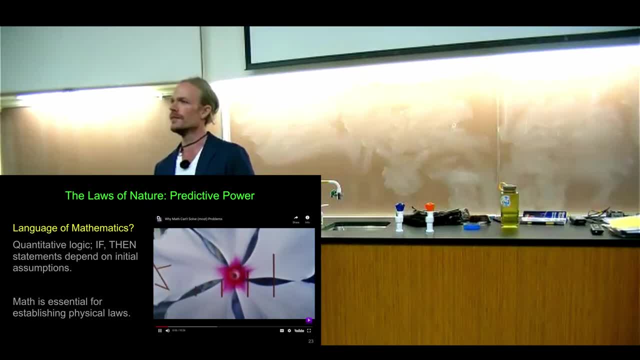 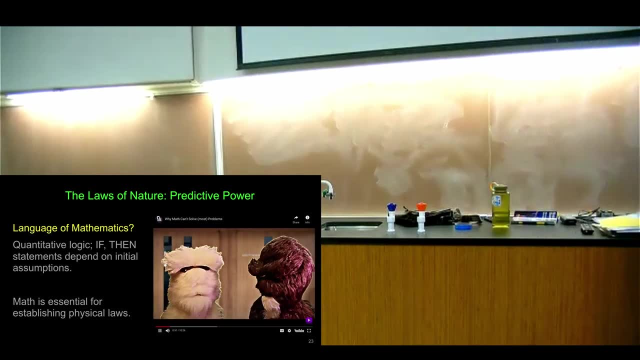 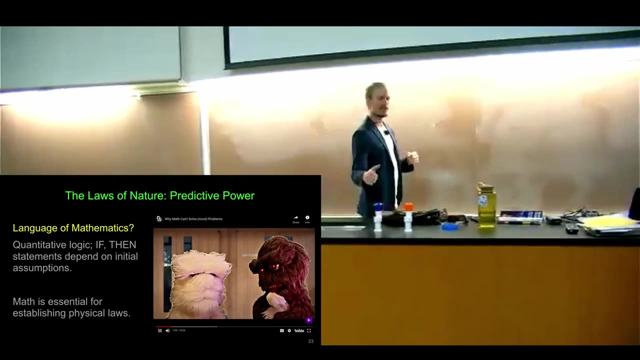 ultimately, science is about explanation. It's not just about saying how things unfold with increasing precision. Again, that's fantastic For technological progress, But at its heart, it has very little to do with explanation. It's just the first step. 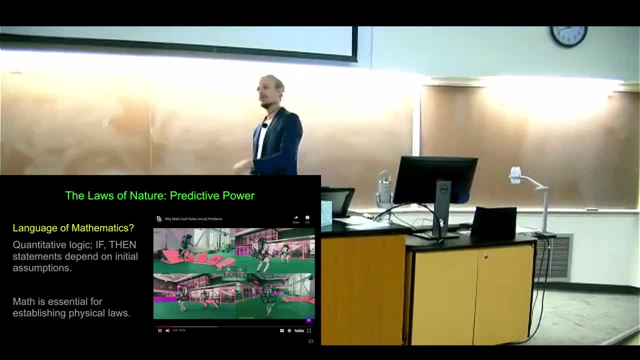 The first step is saying: okay, this is how this unfolds. The ball falls off the table. Why does it fall? Why does it fall? What's causing it to do that? Well, we don't really know, And we're still working on that. 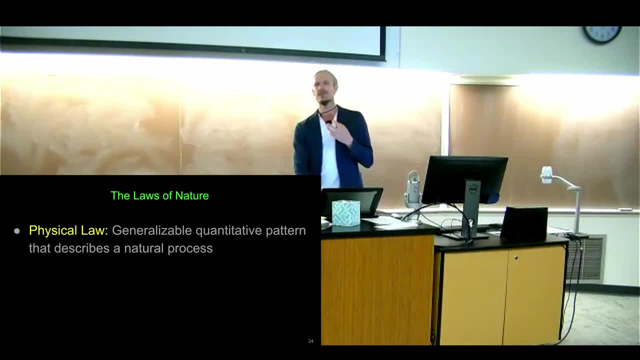 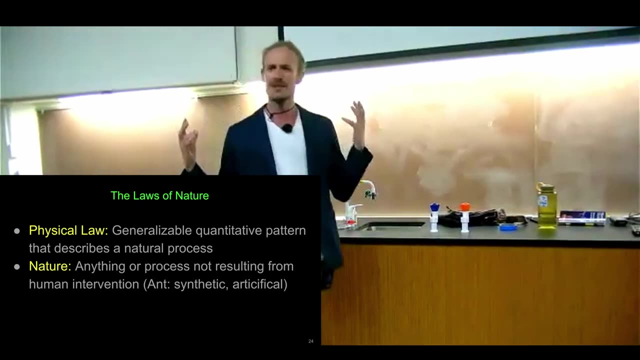 Talked about physical laws. which are these generalizable quantitative patterns Right? This is the first step to creating science. By the way, what is nature? Might seem obvious, Right, Nature is such a big concept it almost means nothing. 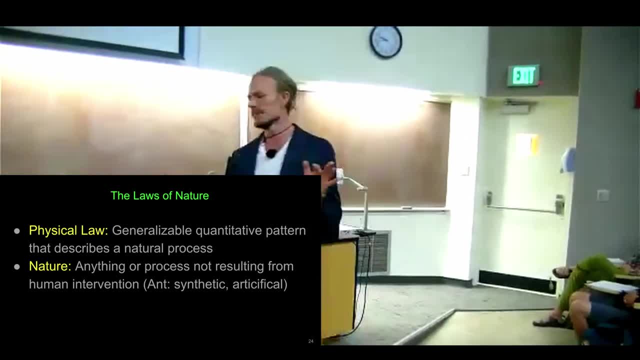 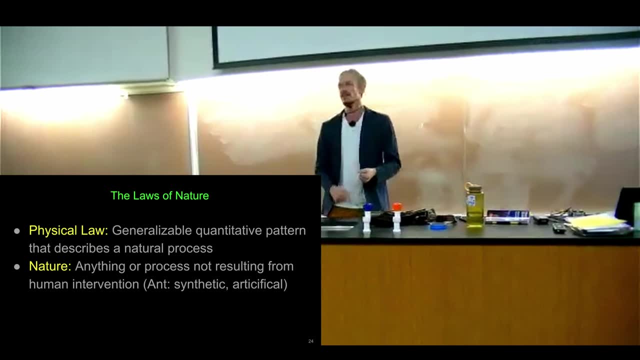 So I'm going to say that nature is everything except for you, Right? Everything except for stuff that humans make, Everything except for the world around us. And that's what we're trying to understand in science. Science is about nature, Right. 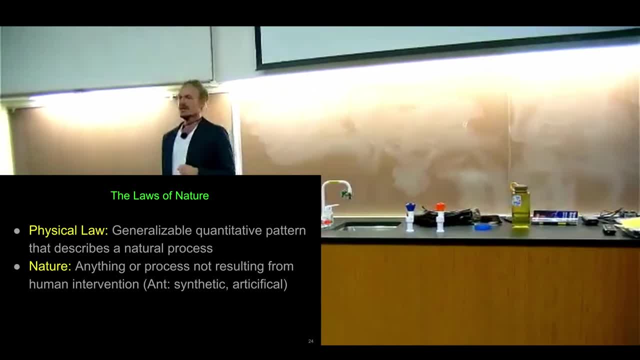 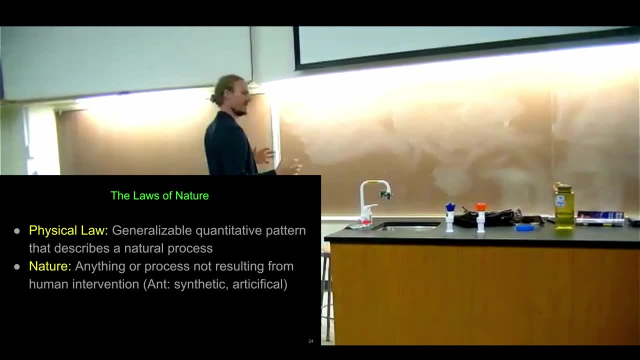 The biggest science journal in the world is called Nature Magazine. If you are at the top of your field, you're trying to publish in this journal, Right? It's about everything outside of humans And, of course, technology has made its way into it as well. 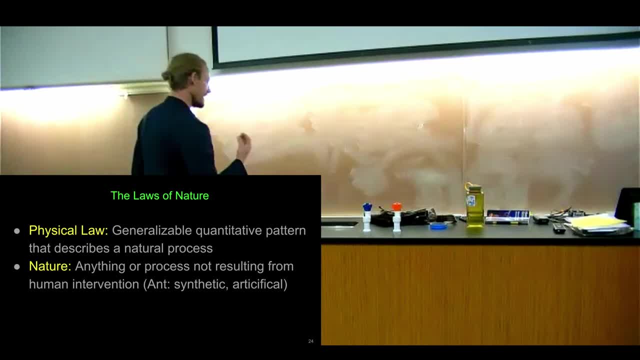 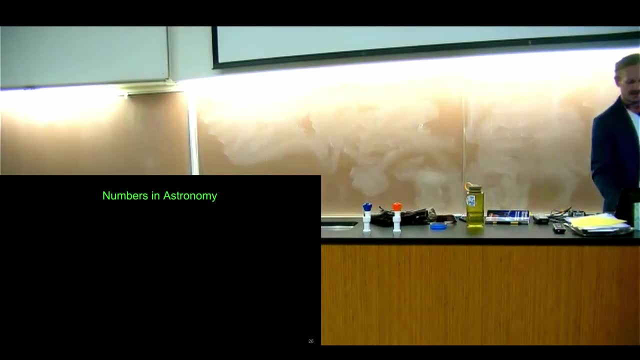 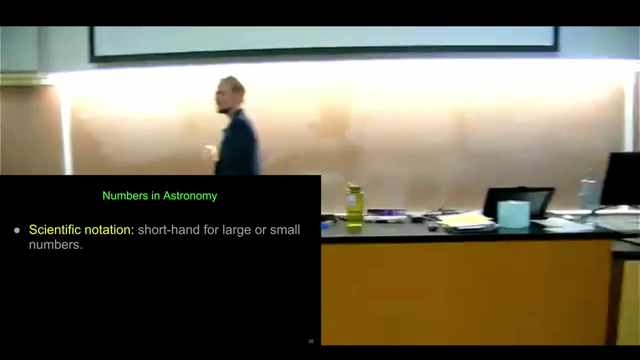 Synthetic, artificial things. But for the most part, science is concerned with how things unfold in the absence of us. I'm going to skip that, All right. I did want to make a very short excursion into scientific notation. You're going to encounter this throughout the book. 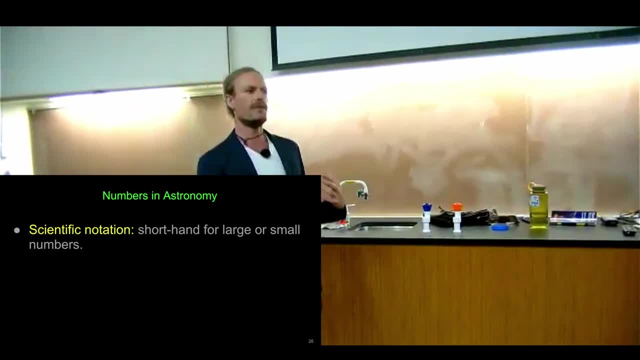 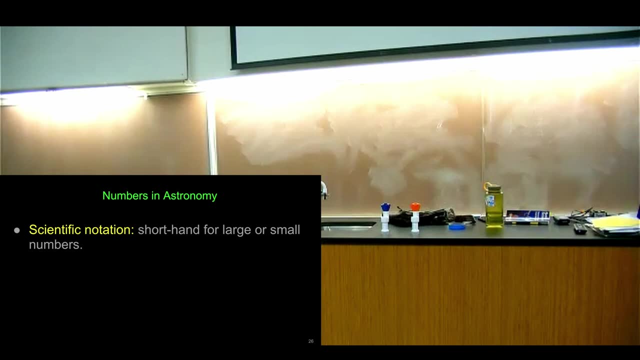 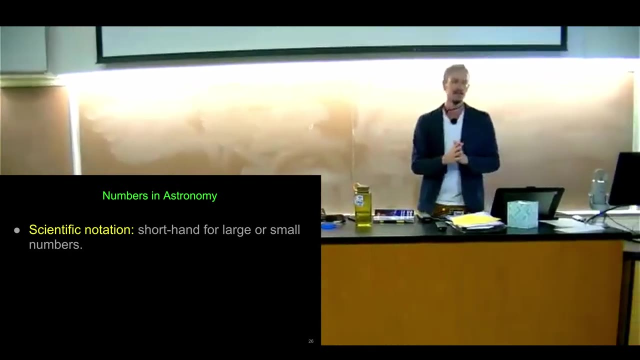 Many of you are probably somewhat familiar with science, Right, You're somewhat familiar with scientific notation. It's simply a way for us to cross enormous chasms of distance and scale without having to write a million zeros behind us. Right, So we use the base 10 in the West. 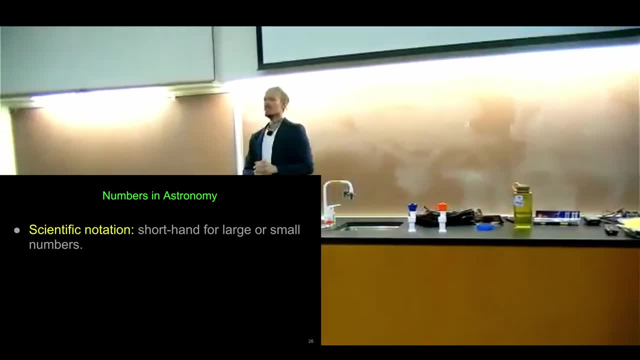 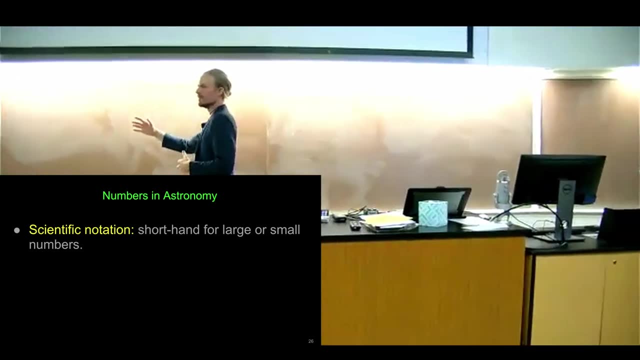 unlike the Babylonians, And this means that any number, however large or small, can be written as something times 10 to the power of whatever. So this will prove really important. I don't want to waste a ton of time on it. 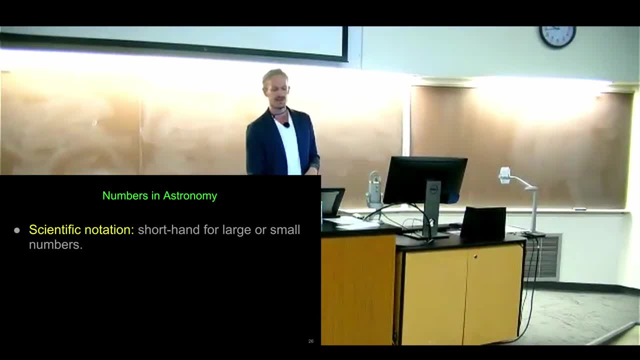 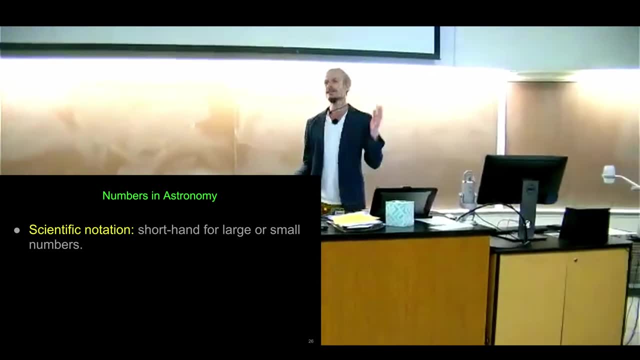 It's in your textbook. If you have issues translating between the two, you know it's quite simple The way that you do it. if you see something like 8 times 10 to the 18th, all it means is there's 18 zeros after that first digit. 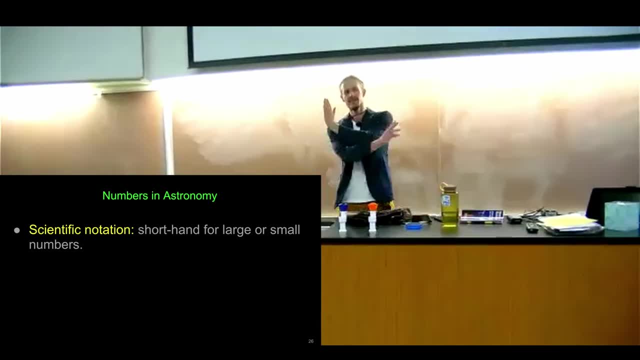 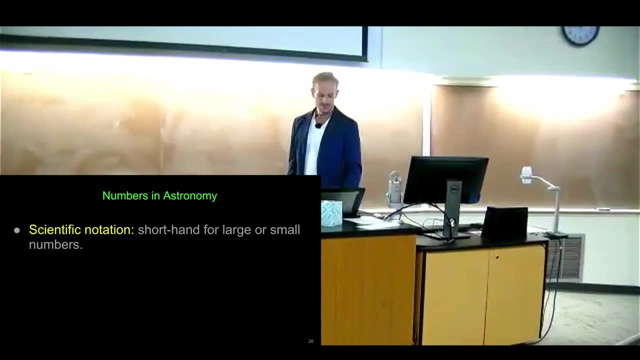 If it's to the negative power, you're going to move that decimal, place the same number of zeros in the opposite direction. Okay, This is just a simple shorthand. We're also going to be dealing with SI, which is System International Units. 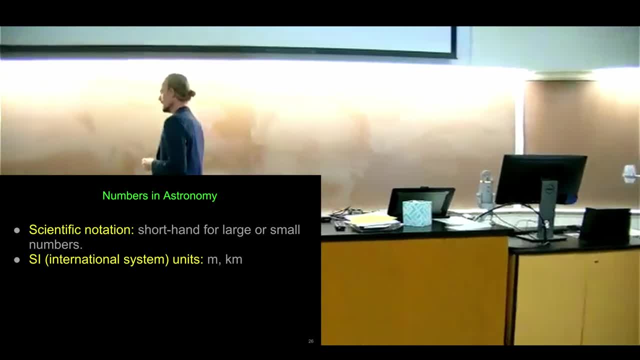 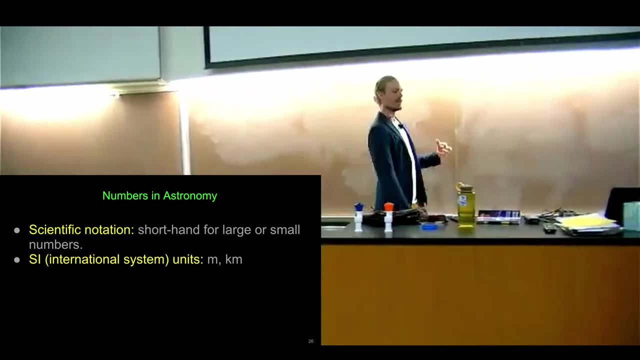 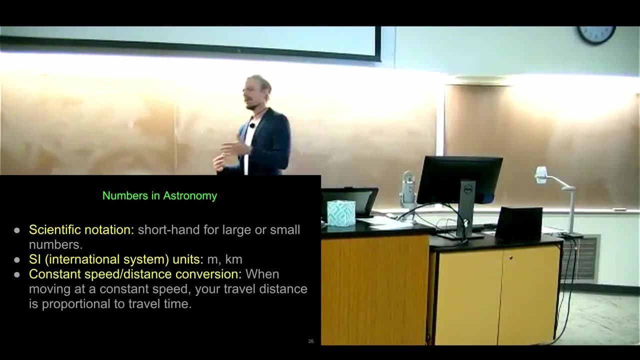 These are meters and kilometers. If you want to go between, say, miles and kilometers, you just multiply it by 0.6. if you want a quick conversion, Right, More kilometers in a mile. And then, of course, this concept that we're going to keep coming back to. 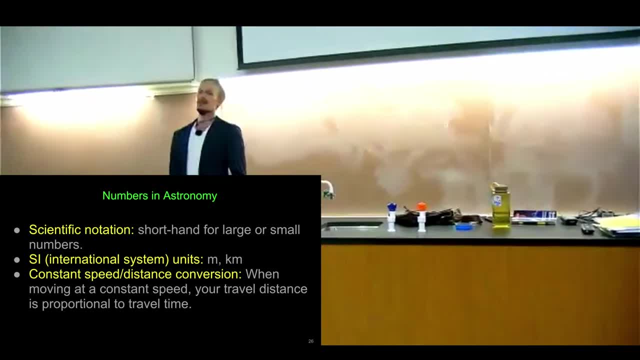 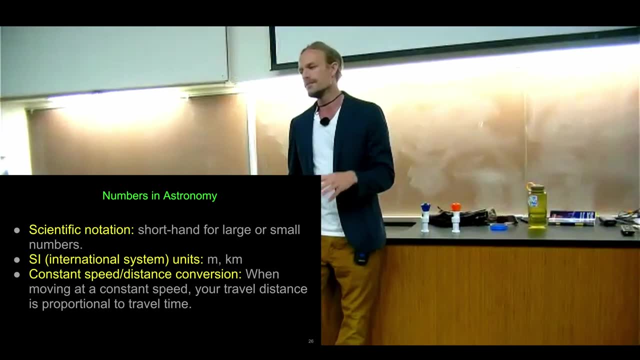 is the speed-distance conversion. So we assume that in astronomy that light is traveling at the same speed. It turns out it actually doesn't travel at the same speed everywhere, but we're going to assume that it does for all intensive purposes, If something is traveling at the same speed. 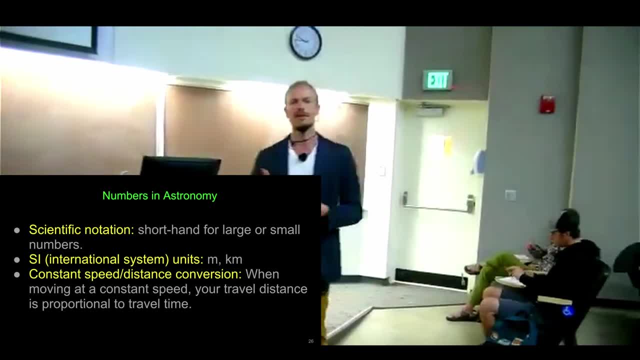 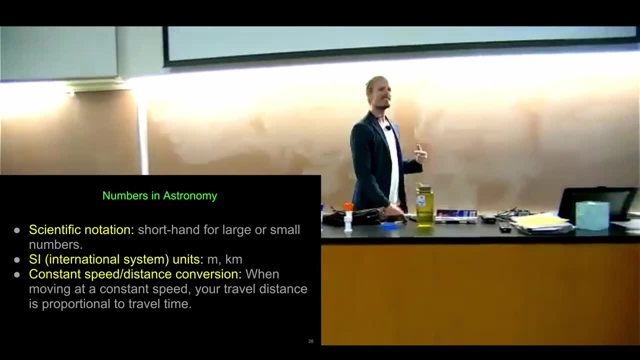 then, if we wait a certain amount of time, we can predict the distance that it travels. Right, This is pretty elementary. This is important because the distances are just so astronomical that writing them in kilometers gets to be preposterous, and we'll see that in a second. 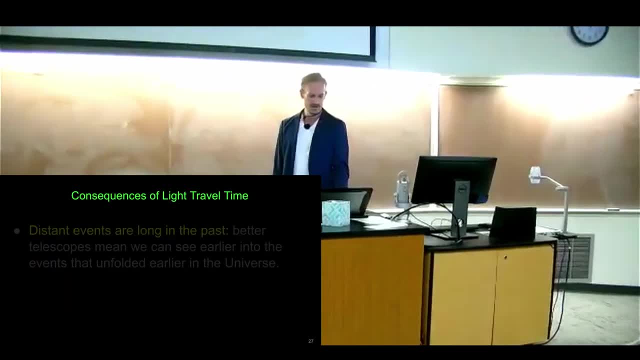 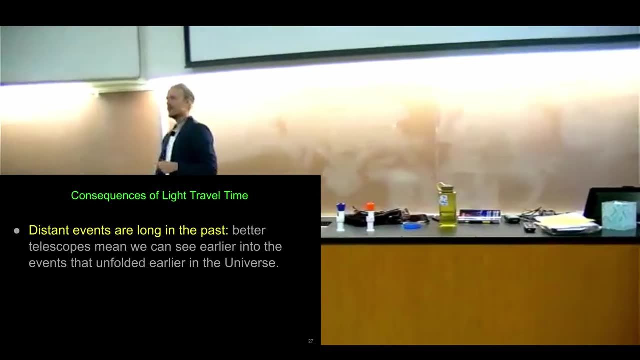 We're going to take a very fast tour of the universe. So the consequence of this is that when we look out into the night sky, the things that we see, they're not as they are today. We're seeing them as they happened millions of years in the past. 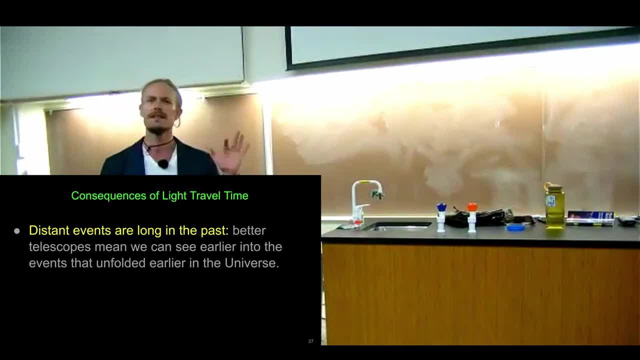 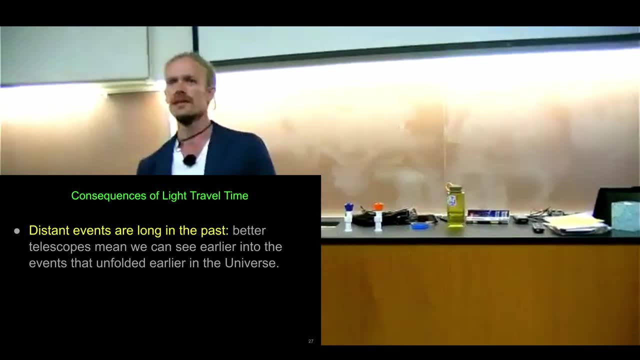 This is really, really crazy. Just go out in the night sky tonight if it's not raining and just look up and be like that's how things were 100 million years ago. That's pretty crazy. We don't have the ability to actually know what's happening right now. 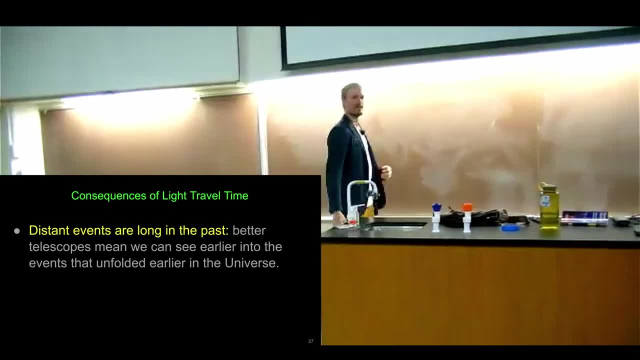 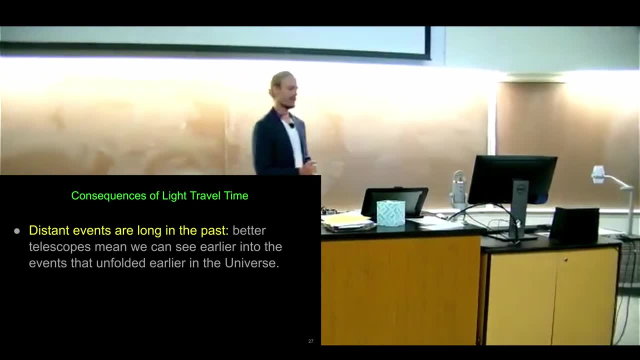 because the light that we use to understand them is traveling at a finite speed. Why it's traveling at a finite speed is a wonderful discussion that I hope we have time to have at some point too, but I want to get to this tour of the universe first. 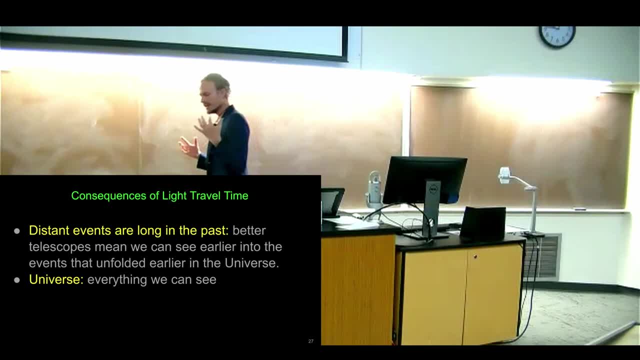 By the way, what's the universe? This is one that really hung me up for a while. The universe is just everything that we can see. okay, So oftentimes if you're in a philosophical context, you're just hanging out with people or whatever. 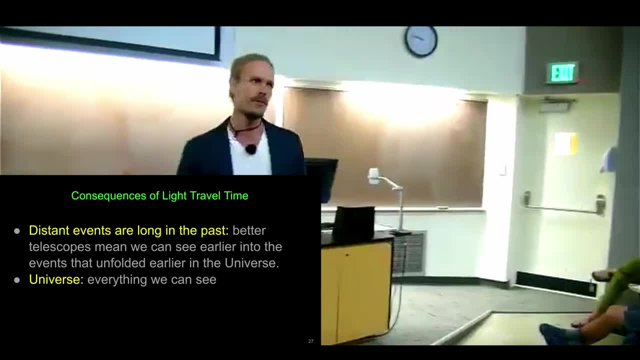 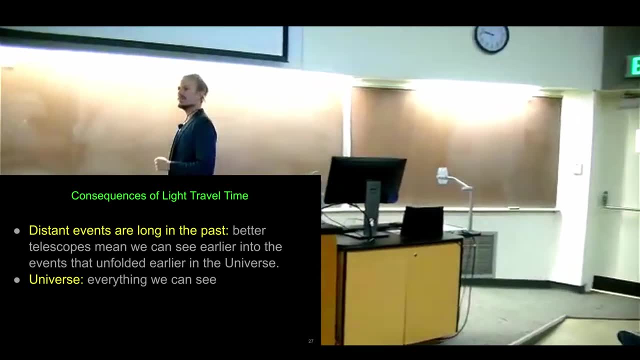 when we say universe, we actually mean everything In astronomy. when we say universe, we just mean the stuff that we can see Again, in the 1920s, the universe was just the Milky Way. Don't let that escape you. 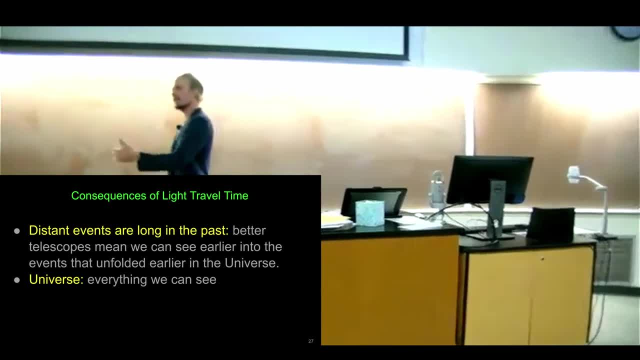 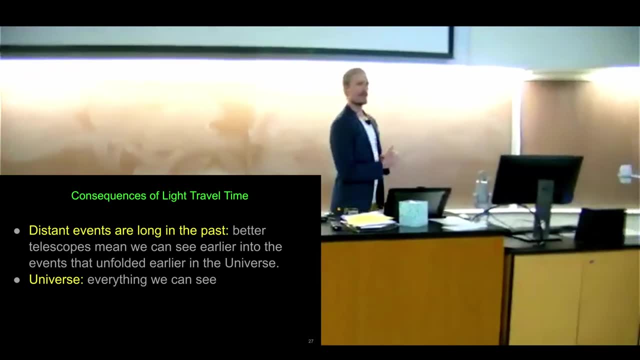 Today, the universe stretches out to about 14 billion light years from here. okay, Does that mean that that's the end of things? Almost certainly not, but that's as far as we can see right now, And actually there's a new telescope called the James Webb. 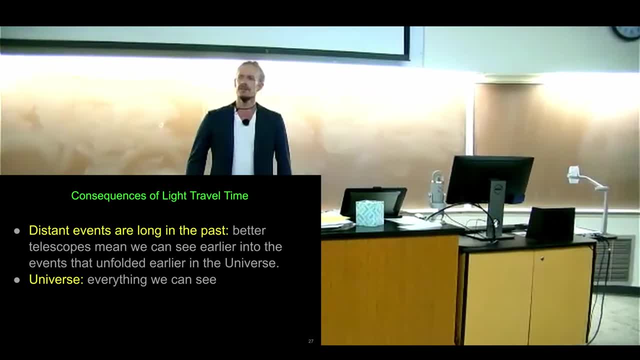 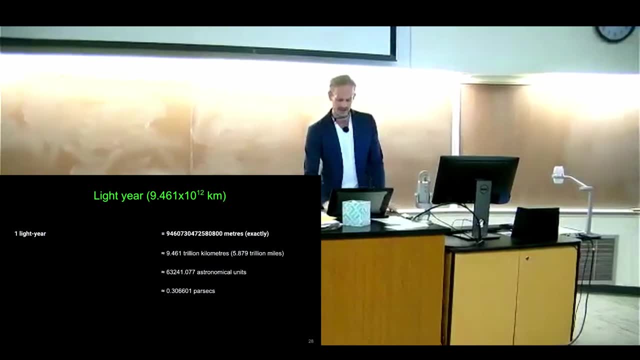 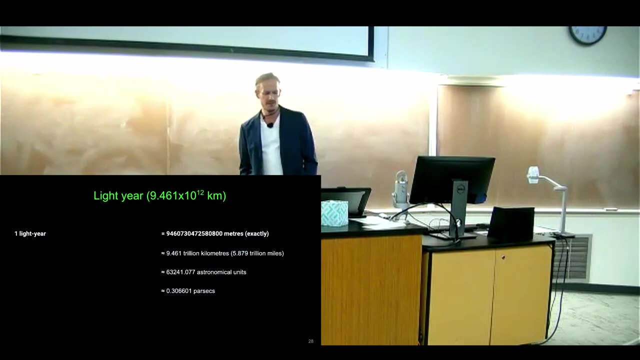 that's up in space and it's kind of crashing the party because it's seeing some things it shouldn't be seeing. All right, So light is very fast. okay, A light year is. I'm not even going to read this number for you. 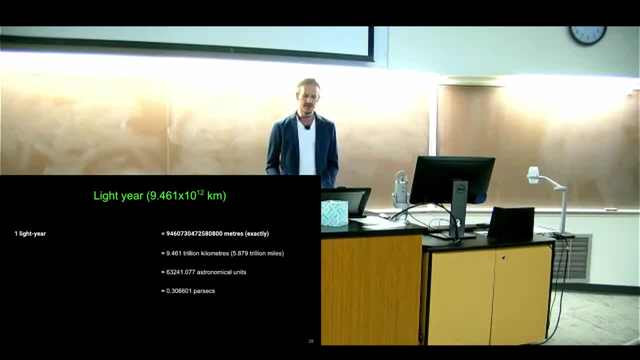 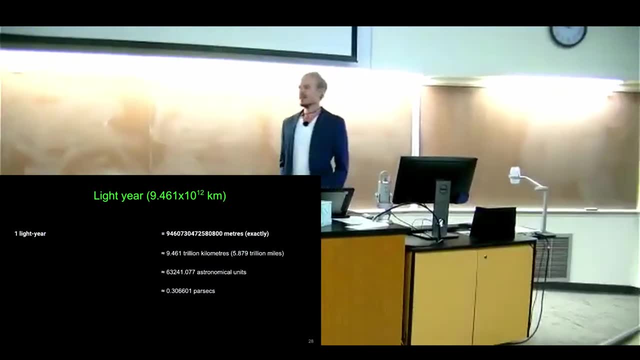 that many meters, which is about nine and a half trillion kilometers. A trillion is, of course, 10 to the 12th right. You can tack on all of those zeros to it. This is an unimaginable distance actually. 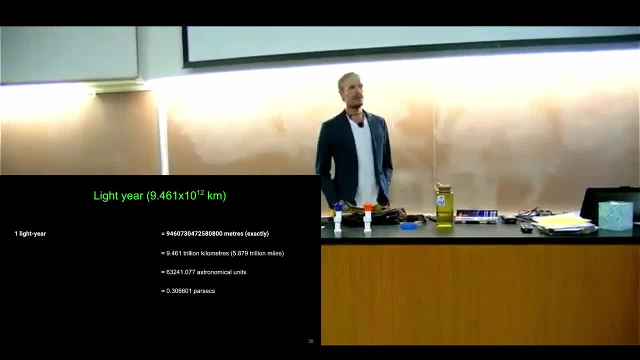 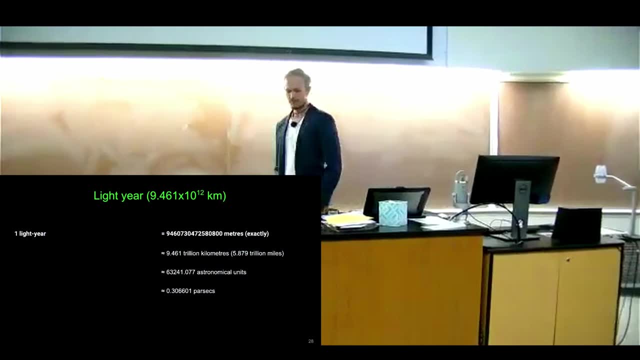 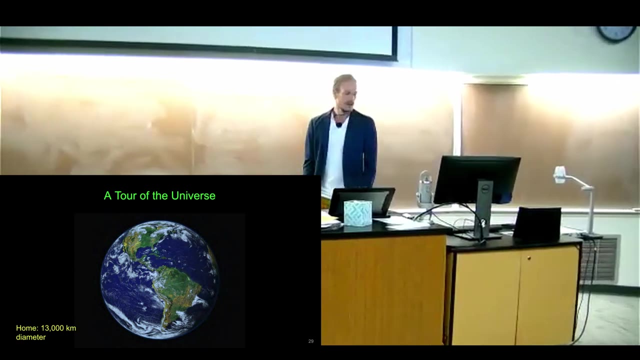 This is somewhat around the size of here, to the edge of the Earth, To the edge of the known solar system. as far as we understand it, It's very, very far. We'll come back to that. All right, So we got about 10 minutes left. 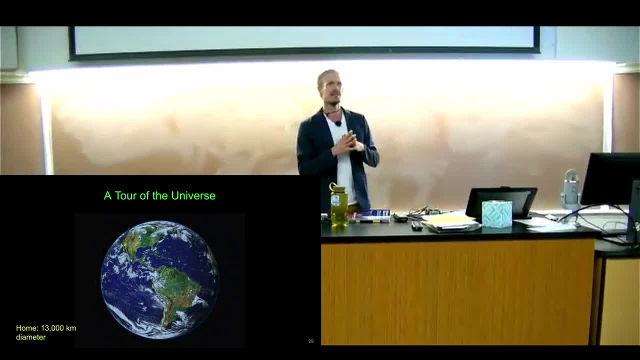 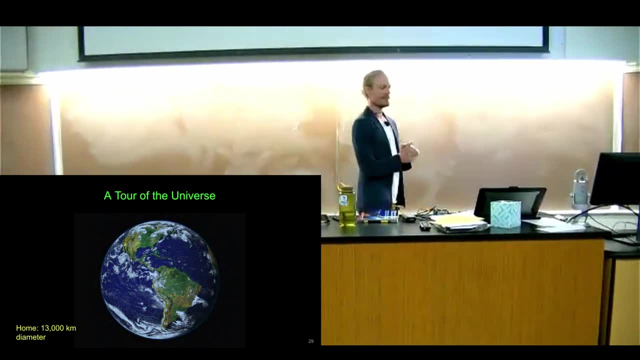 Do we have 10 minutes left? This class ends at 50.. All right, I'm going to give you five minutes. I'm sorry I'm going over. I just want to blast through this. This is really important. I want to show you where you are. 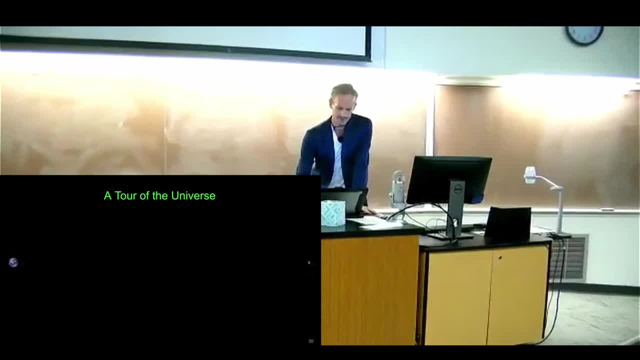 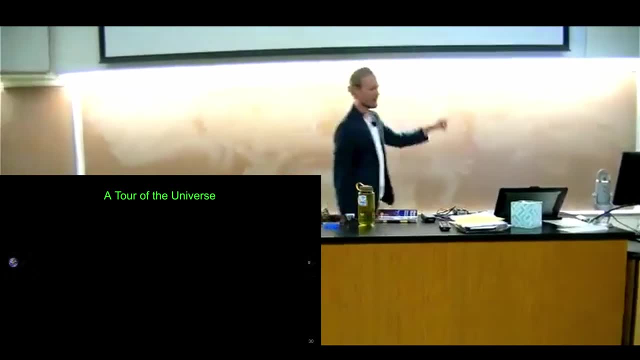 This is the Earth. It's 13,000 kilometers across. This is the Moon to scale. It's much farther than it's usually drawn in pictures. right, That's the Moon over there. The Moon happens to be, oh, about 30 times the diameter of the Earth away from us. 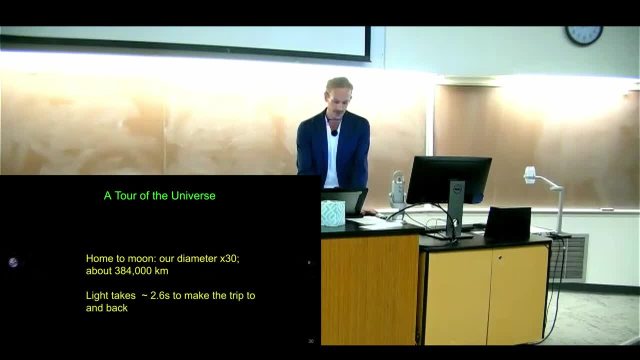 There's 60 Earth radii. Go a little bit further. By the way, light takes about two and a half seconds to go to the Moon and back, So by the time it's reflecting to you, it's taken quite a journey. 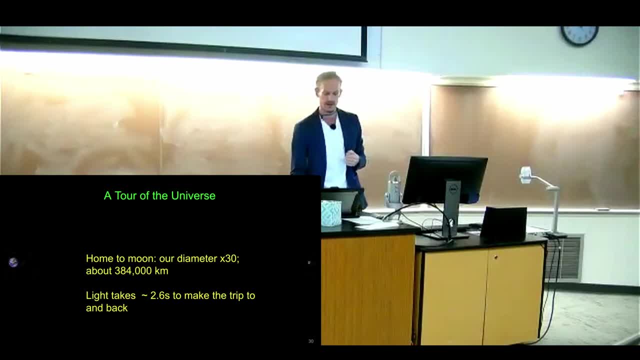 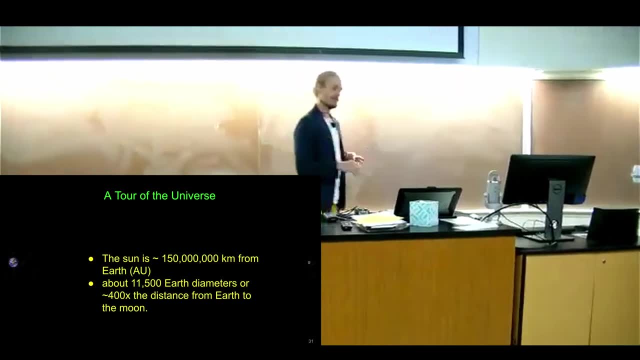 Again, seeing it in the past, which is difficult to comprehend. You know, if the Moon suddenly were to be vaporized, you would only notice it about a second later. All right, The Sun, then, is actually 150 million kilometers from Earth. 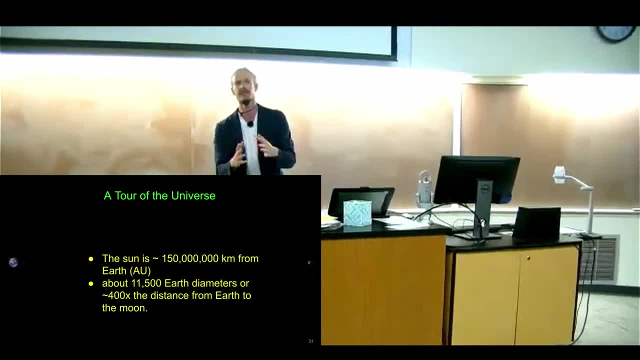 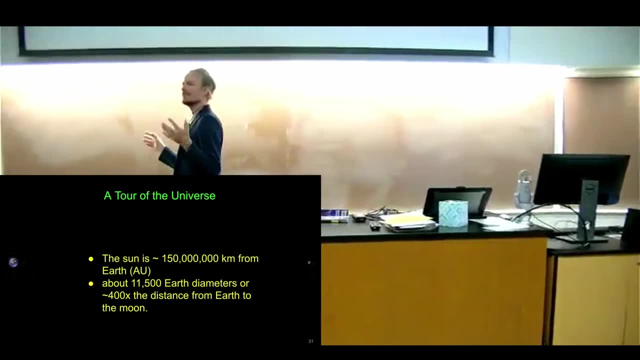 We call this an astronomical unit. Again, we're simplifying things, because if we had to talk about kilometers all the time it would be preposterous. We would just be sitting here just spouting all these ridiculously long numbers. It just doesn't make sense. 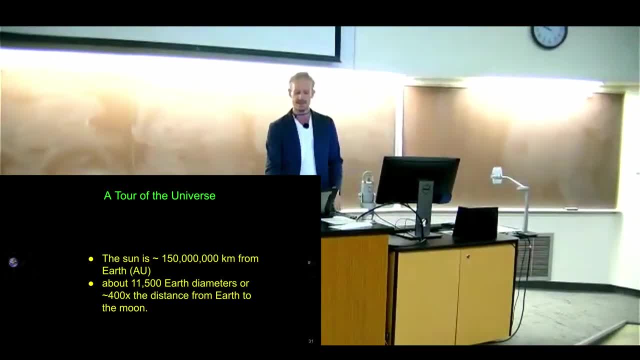 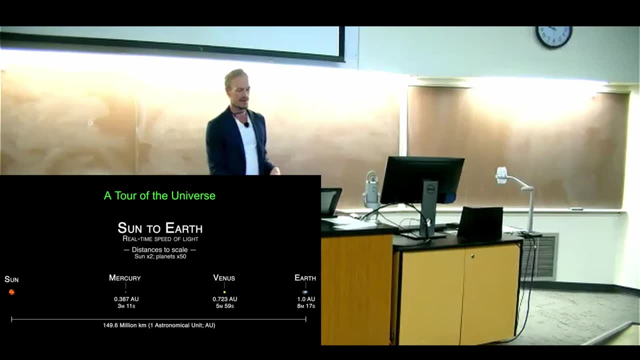 So in astronomy you'll often encounter the concept of astronomical units. That's the distance to the Sun, And there you have it. There's a couple of planets in between us. We're going to talk about those in great detail later. 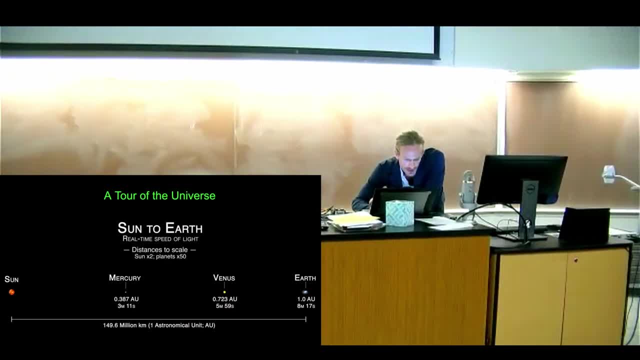 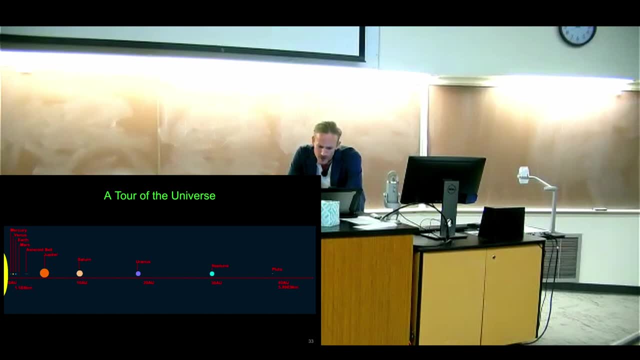 But that's one astronomical unit And again that's something like 150 million kilometers. Now, as we stretch out even further, we can see that Saturn is actually about 10 times that distance that we have between us and the Earth. 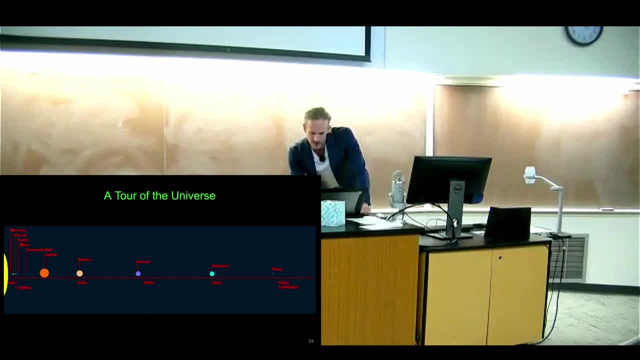 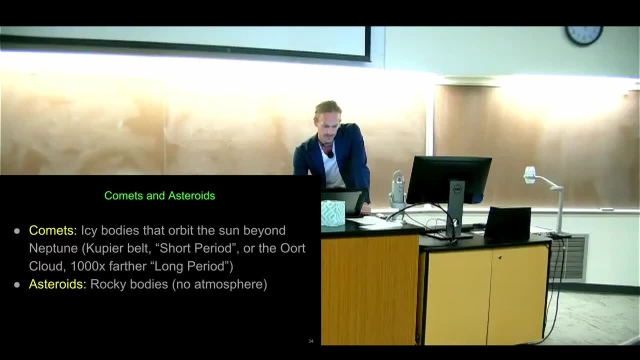 By the way this you know- Pluto is about 40 times that. If we go even further out, we're going to encounter something called the Kupyat Belt, which is where a bunch of comets and asteroids are appearing beyond these gas giants. 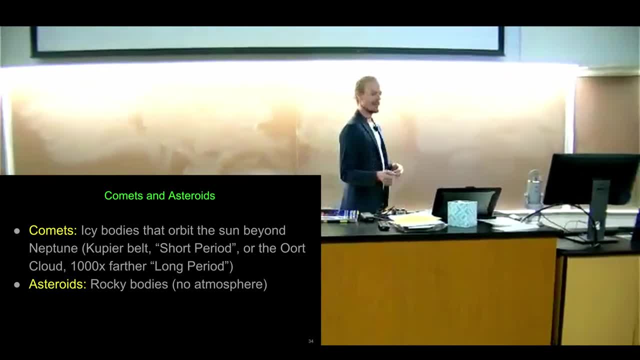 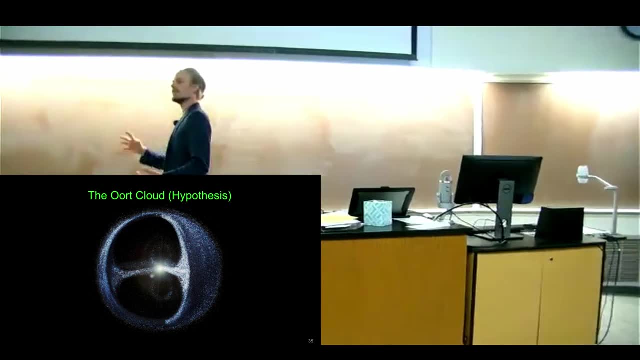 Go a little bit further out, we encounter this thing called the Oort cloud, which is a hypothetical cluster of comets and icy bodies that accumulates at the outside of the solar system, And it's not close at all. In fact, these are asteroids. 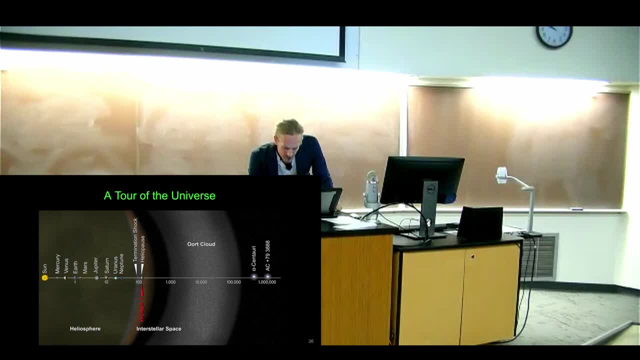 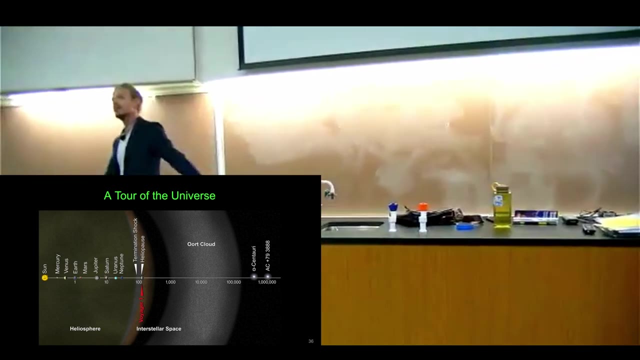 that have been in the atmosphere for a long time. These are AUs, right, So you can see, the Earth is one AU. The Oort cloud is 10,000 times further than you are from the Sun. away from here, That is the outer limit. 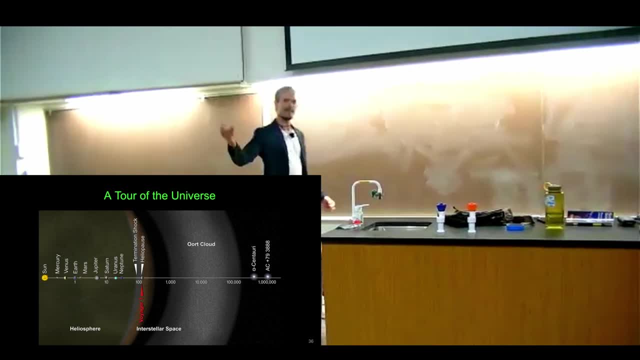 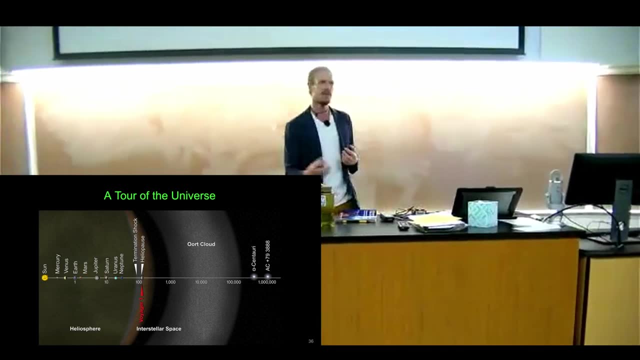 that is the shell of our solar system And periodically it seems like other stars come by and bump into our Oort cloud and they send planets, they send things hurtling towards the interior And we perceive these as comets and other celestial events. And since we've only been keeping record for a few thousand years, it's hard to say what sort of crazy things have been thrown at us since then. So let's keep moving. That Oort cloud is also about 1.6 light years away. If we actually look at our closest neighbors to the Sun, we can see that there's some other stars out there, About four light years away, our closest neighbor, Alpha Centauri. I mean, these distances are unimaginable. It would take you four years. 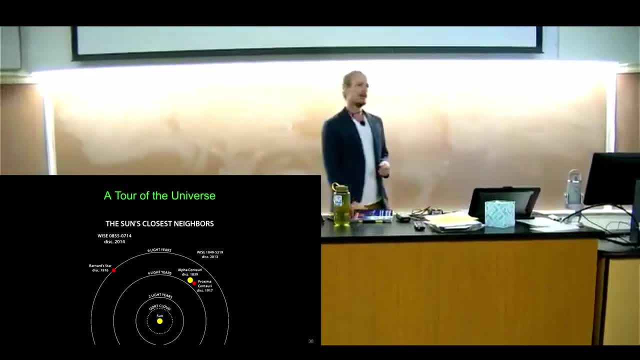 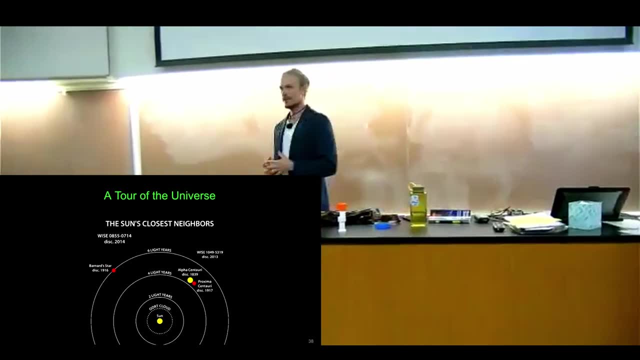 traveling at the speed of light to even get there. I mean, you know there's some doubt as to how close we'll ever even be able to come to this because of the physical limitations of how atoms work, But say we could go as fast as possible. 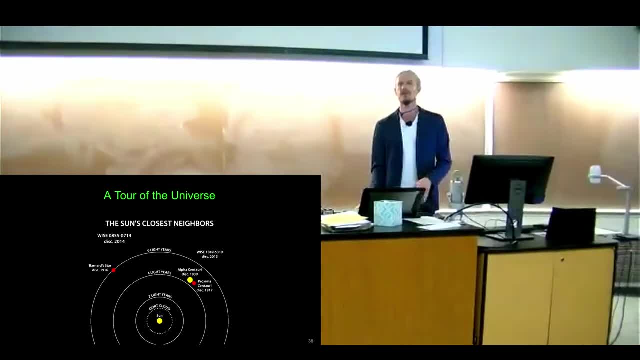 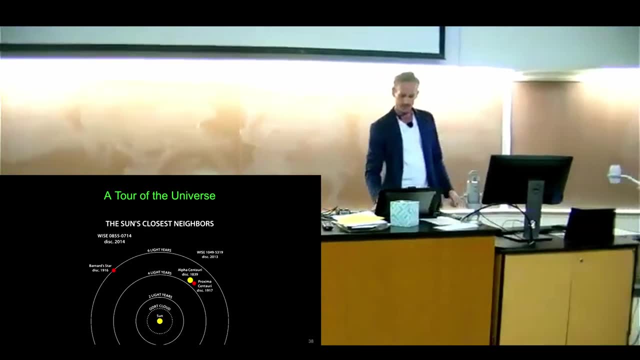 it would take us four years. In reality, if we're ever to travel there, it will almost certainly take a generation. It will take people to have children on a spaceship traveling out there to even reach that place. I'm going to skip this. 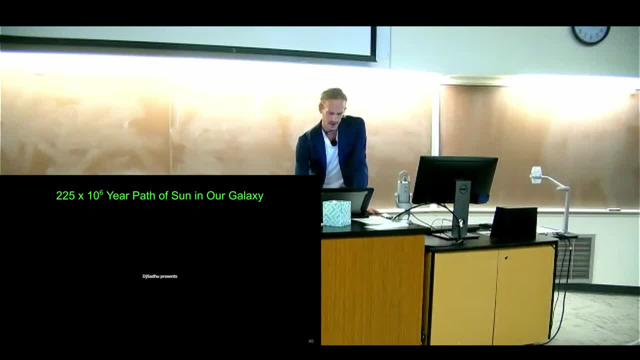 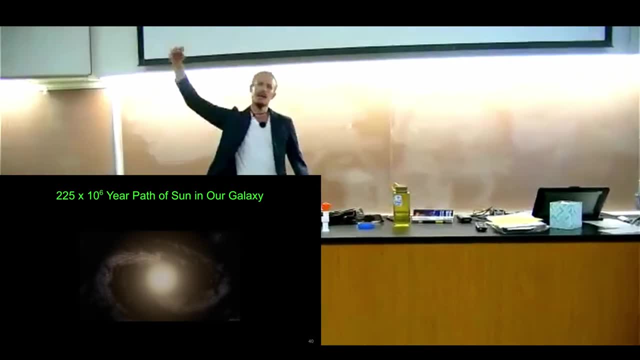 I had a little video here, but I think I think it's worth considering that as the Sun travels through the galaxy, it's actually going up and down throughout the galaxy. like this, It's corkscrewing The center of mass for the solar system. 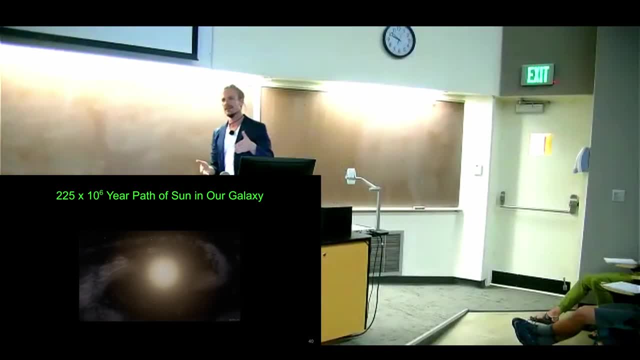 isn't actually at the Sun, It's slightly outside of the Sun. All of the other planets are tugging on it. The Sun wobbles. It makes this helical path as it travels around the galaxy- which, by the way, 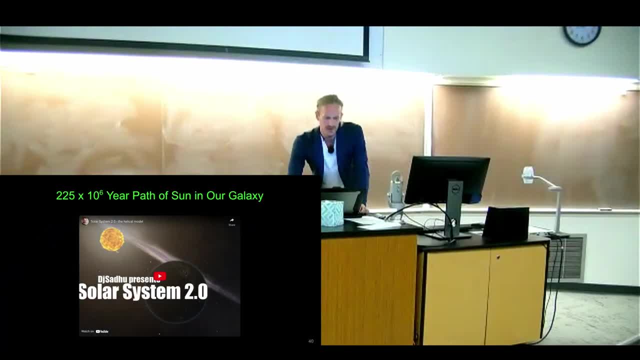 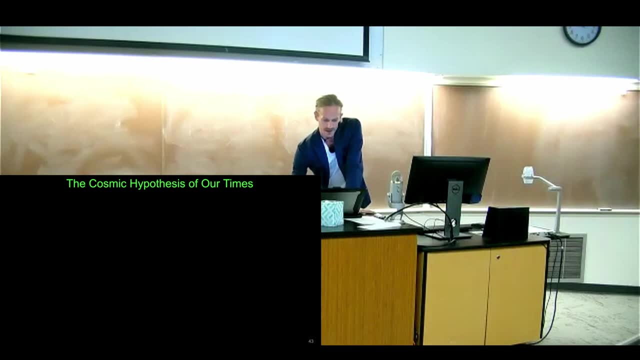 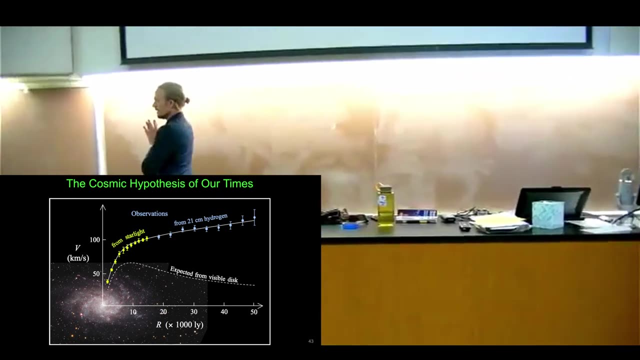 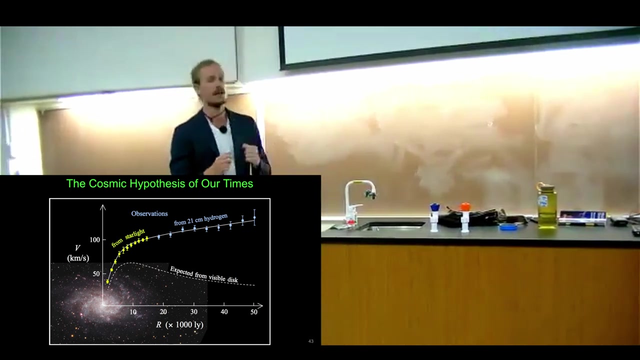 takes 225 million years to go around the galaxy. And I'm going to stop there. Well, no, Let's say one more thing before we stop. One more thing: Today, our astronomy is principled on this cosmology, which is called Lambda CDM.